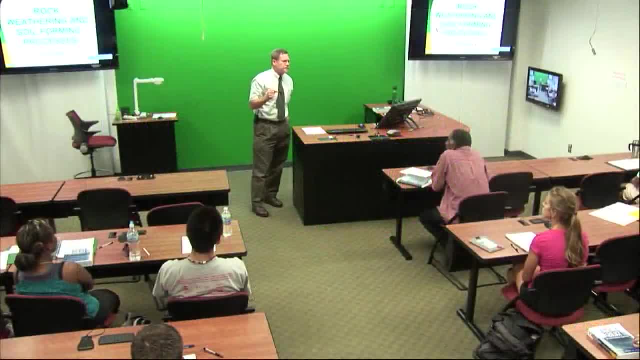 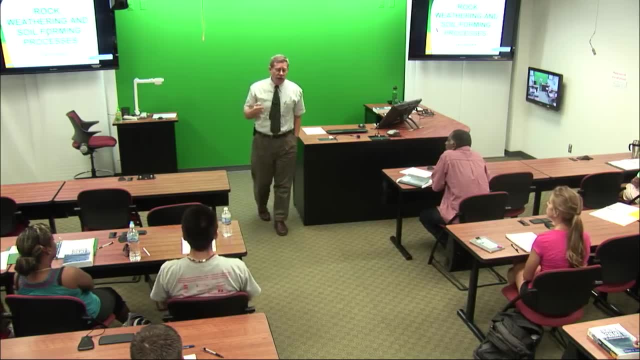 Any engineering problem out there. there's a hundred different ways to fix it. There's no one way. that's right. There's just the ways that you're most familiar with. You're not going to make money fixing anything until you've done it about 12 times. 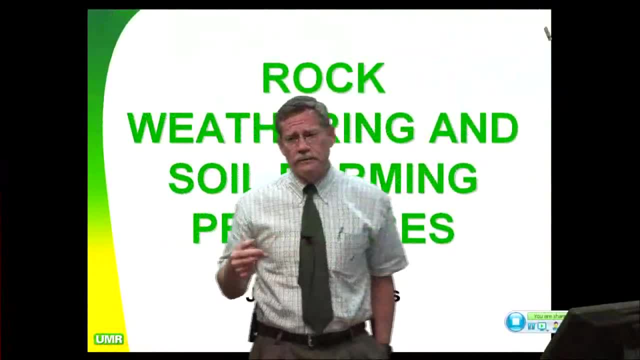 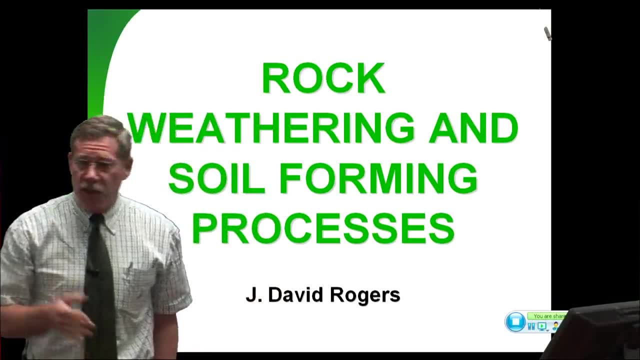 If you're smart enough to learn from all your mistakes. So nobody comes out of the starting blocks, goes out there and does something and makes a ton of money on it the first time out, You're lucky, You're blessed, You're walking with Jesus. if you can just break even the first time out, You don't lose your shorts. How long does a general engineering contracting firm last? in the United States, The average length of their life is seven years. That includes the guys like Guy F Atkinson, Bechtel, the ones who've been out there a hundred plus years. That's including everybody. The average time they last Seven years. Why? Very competitive business. You make one mistake, you're done. Make one mistake on something. didn't carry this decimal over. you're off by order of magnitude. You could lose a million dollars. 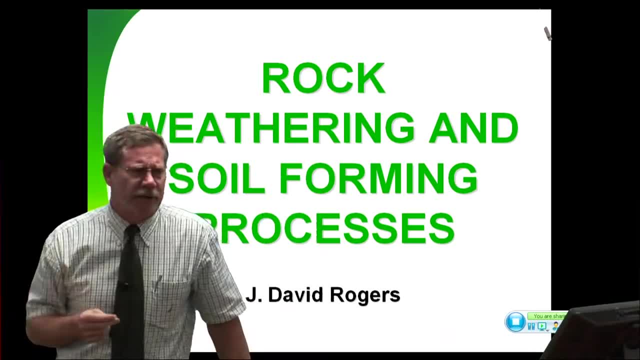 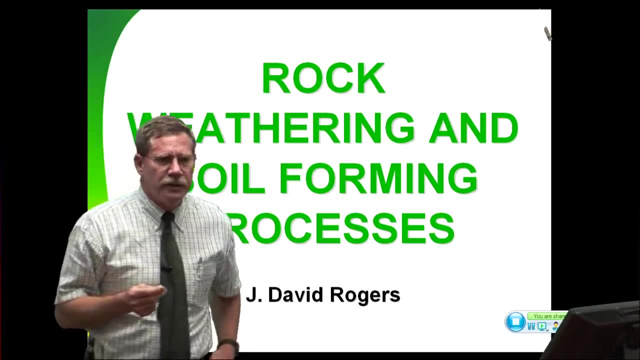 You could lose two or three or four or five million dollars Very, very quickly. Once you lose that much money, you're not going to be able to get bonded for your next job, So it's a very unforgiving business. It's a lot of fun. 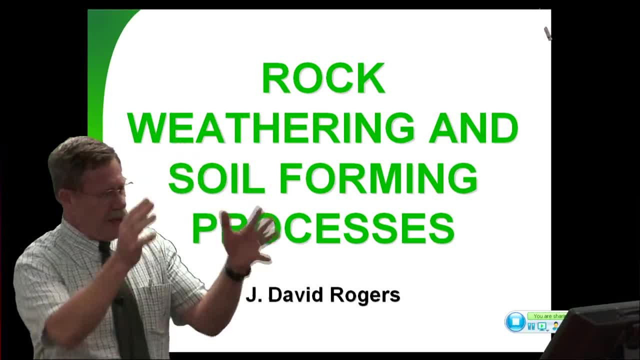 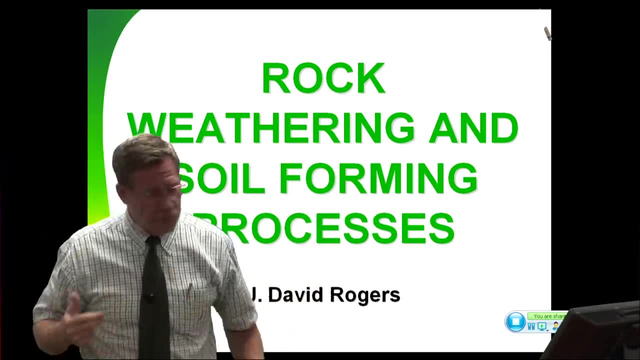 It's a lot of fun to go out somewhere, see a highway or a bridge or something that's just gone, and they say to you, Help us Do something, Get this back open. And you get it back open And you go back out there. 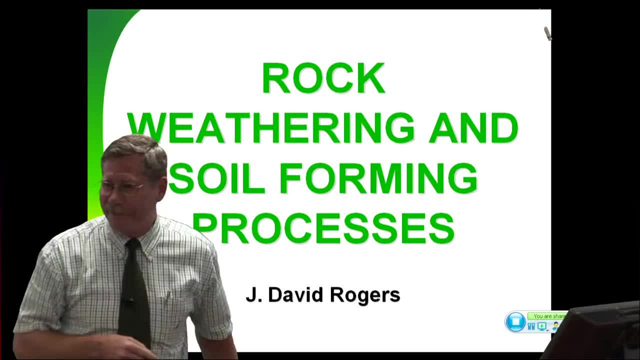 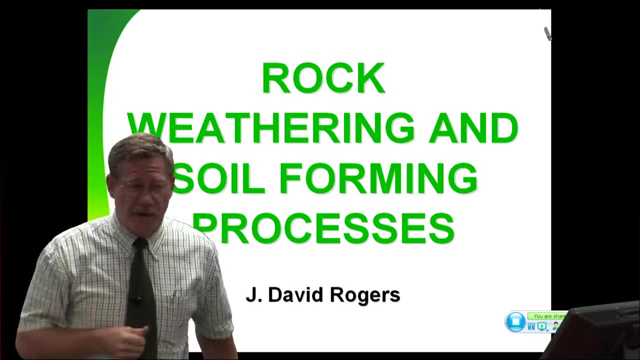 20,, 30 years later and you see your handiwork A lot better than being a parent. believe me, I've got five kids. None of them have turned out that good yet, But it's fun to go out there and say: 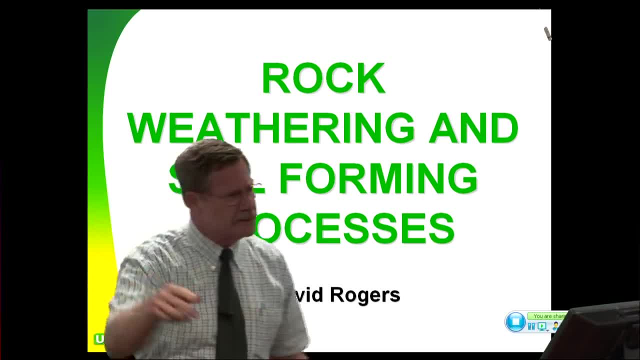 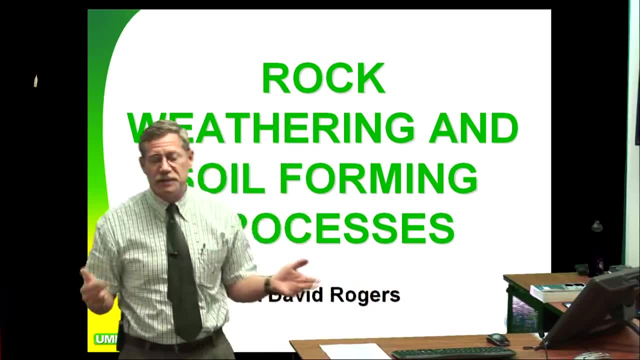 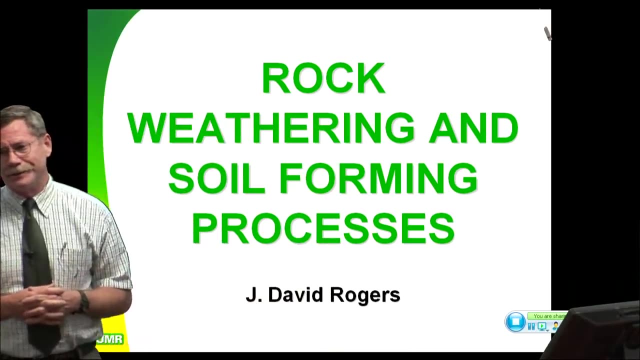 I designed this. I came up with this concept. I built this in a very short period of time. And look at it. It's working. Everybody's depending on it. It's providing something for my culture, my society. It's very, very fulfilling to be a civil engineer. 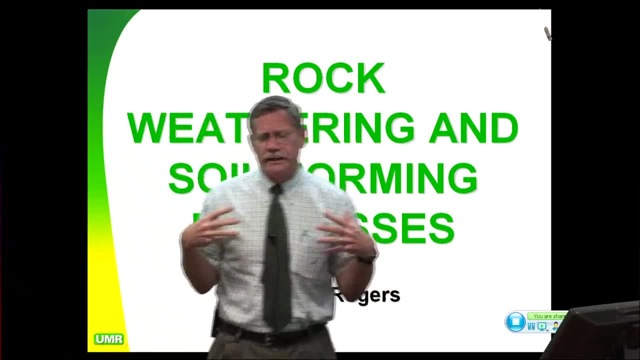 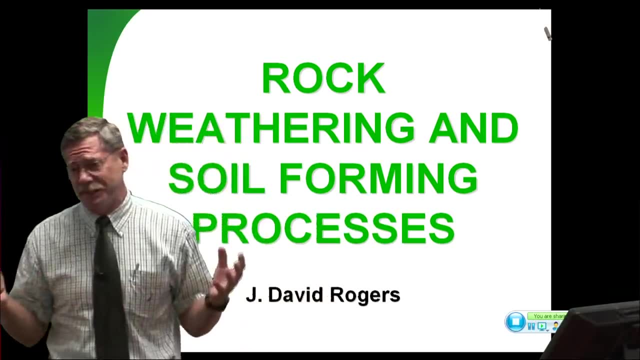 and to do civil engineering work, And that's what my job is in the geological engineering department. I'm the geotechnical guy, I'm the civil application representative. So I'm basically a civil engineer by training. Got registered back in 1983.. 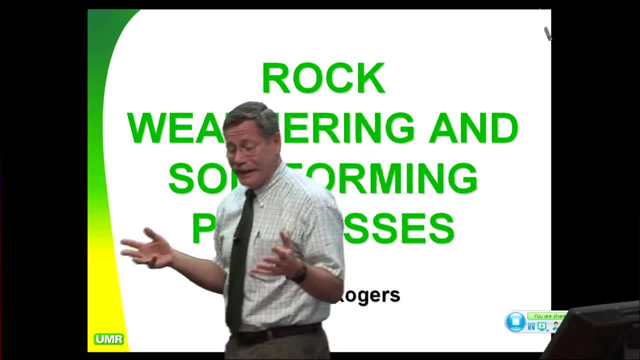 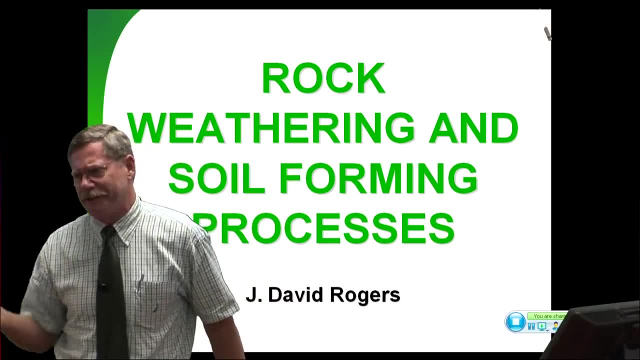 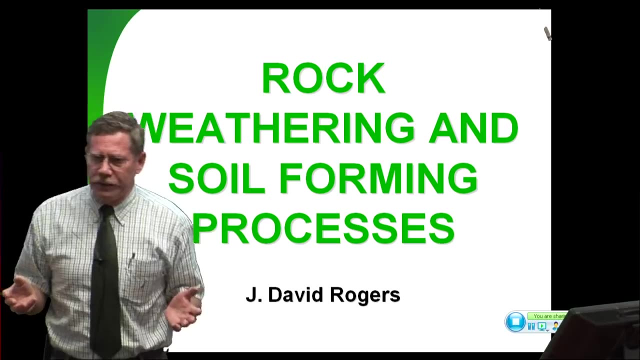 And got other registrations like geotechnical engineering. I have registered in geology, professional geologists, certified engineering geologists, certified hydrogeologists- all by examination, So I love taking tests. I came to Berkeley with an undergraduate degree in geology. 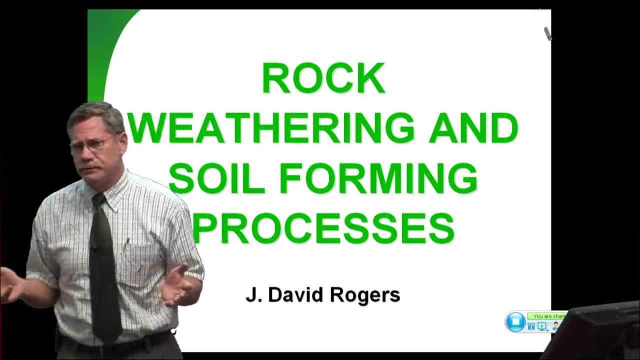 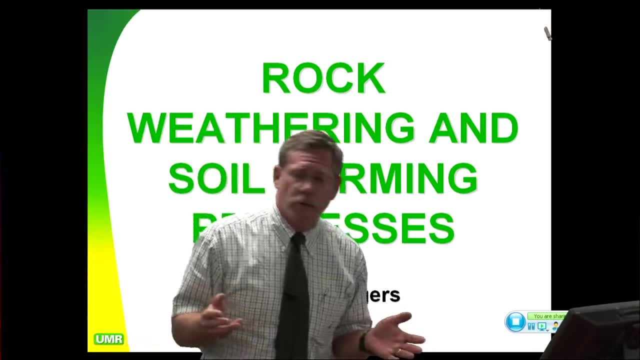 I didn't even graduate from high school with honors, So a lot of you are here. You don't have big ACT scores. I don't care what your ACT score is. All I care is how hard you want to work. You want to work hard. 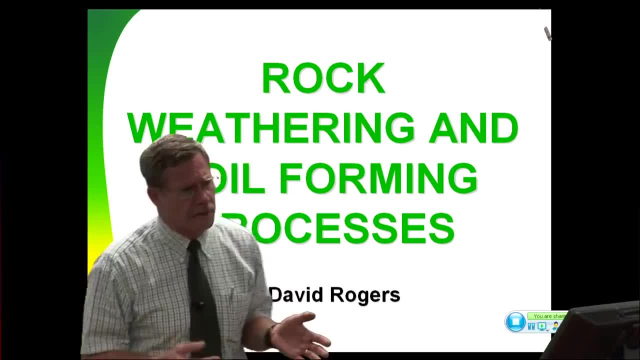 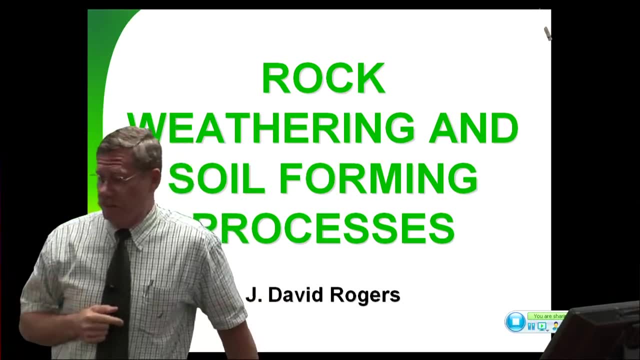 That's what employers look for. We basically look for somebody who'll walk in the door and say, hey, I want to work for you. You don't even have to pay me, I want to work for you. Those are the people you go. huh really. 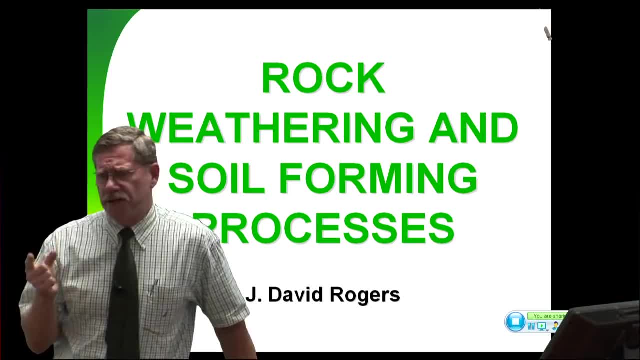 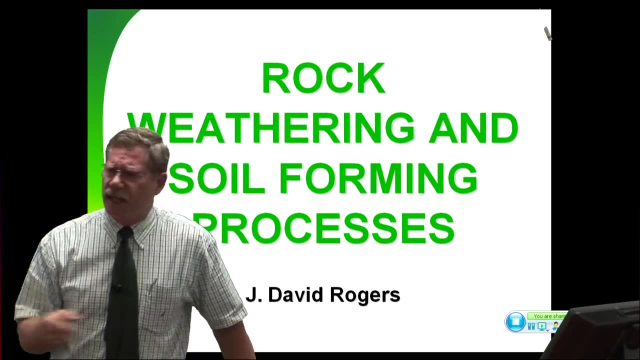 Show me, Show how hard you want to work. What every employer is looking for is this: Somebody who sees what needs doing and does it without being asked And doesn't come up with a whole bunch of lame excuses Saying: well, I didn't get training in that. 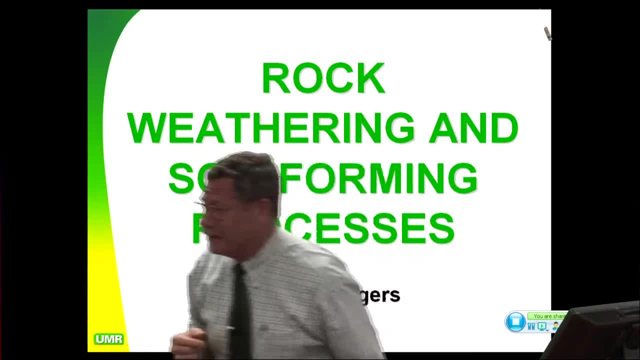 I couldn't do that. You know there's mosquitoes out there. Oh, there's muddy out there. You want me to get muddy? I mean, I don't know, I got Italian suede shoes, I don't know. Those guys send them off to structural engineering school. 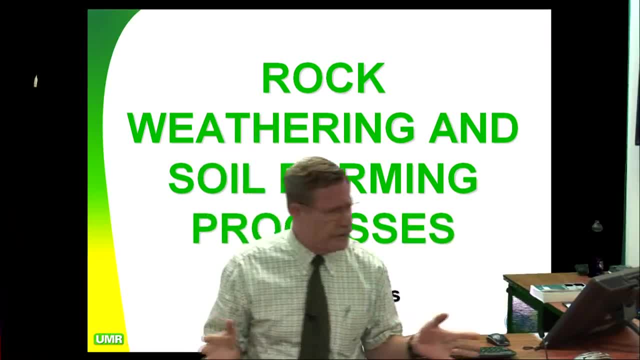 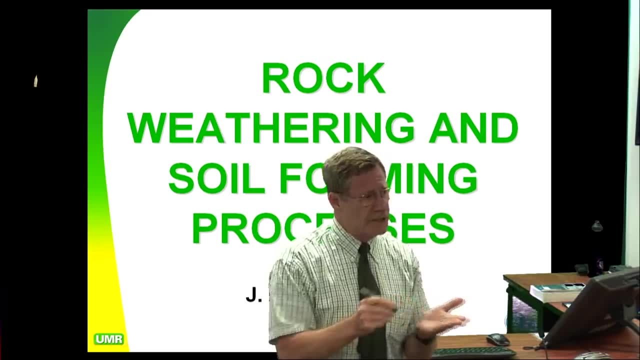 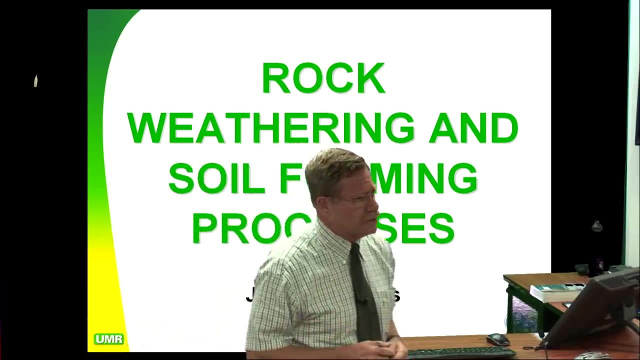 That's where they need to be. Structural engineers can calculate strains to half a percent. They are engineers' engineers. They can cut it nice and fine because they're dealing with materials that come out of Pennsylvania steel mills with ASTM certifications, And I would always have conversations with structural engineers. 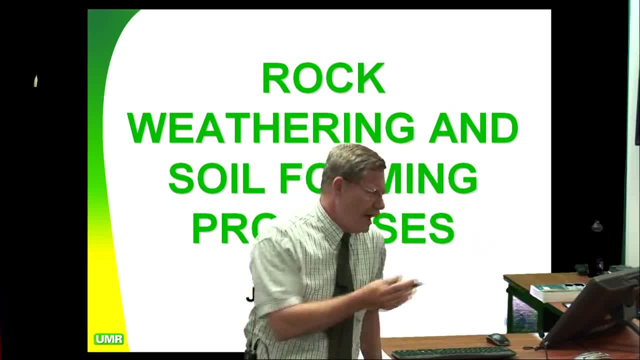 when it's something like this: They'd be calling me up about one of my geotechnical reports And I'd have some clause in there saying you know you can expect settlement on this embankment of anywhere between three and nine inches. 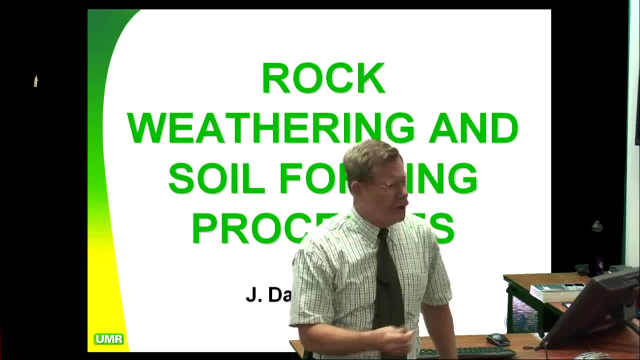 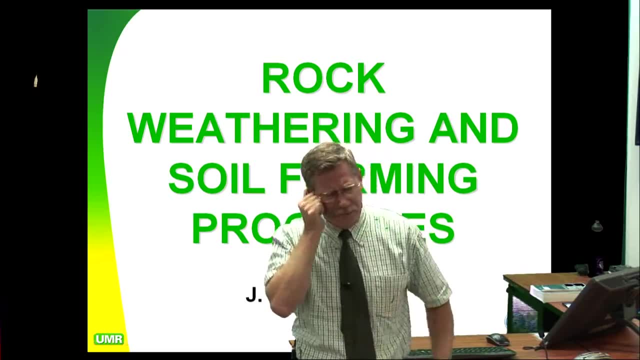 in the long term. so six-inch variance. Structural engineer would call you up and go. hey riders. Yes sir, What is this stuff here? You know it's about three, nine inches. Is it three inches or nine inches? 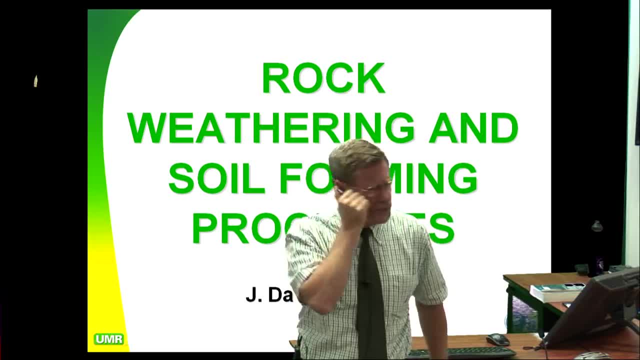 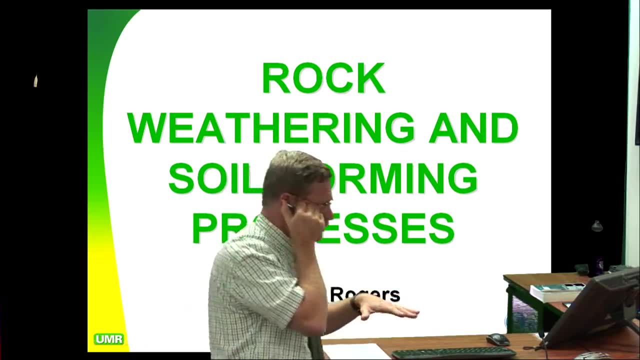 Do you know what you're doing over there? That's a big difference, That's 300% difference. Oh sir, it's anywhere between three and nine inches. Soil never settles uniformly like structures settle. It settles in a dimpled up-and-down type of fashion. 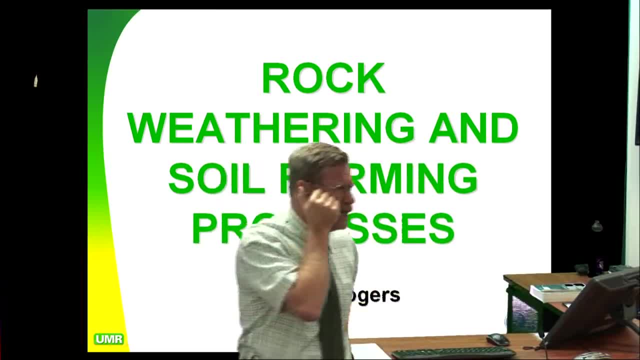 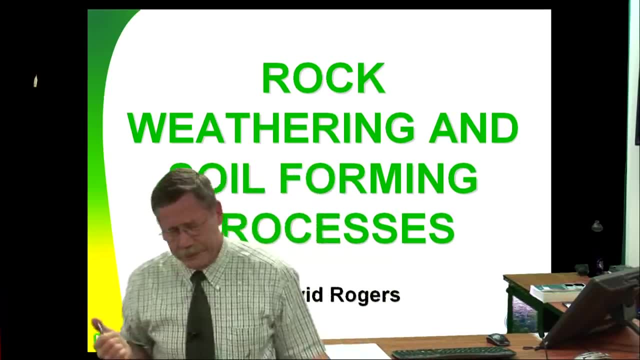 And the rates depend on drainage and effective stress, stress history, over-consolidation ratio, and you go on and on and on. He doesn't know what you're talking about. It's a bunch of you know, geotechnical gobbledygook. 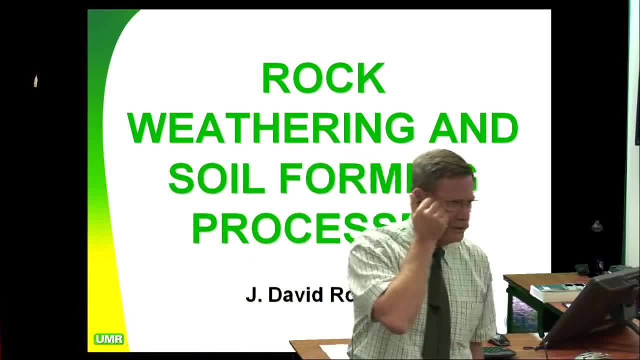 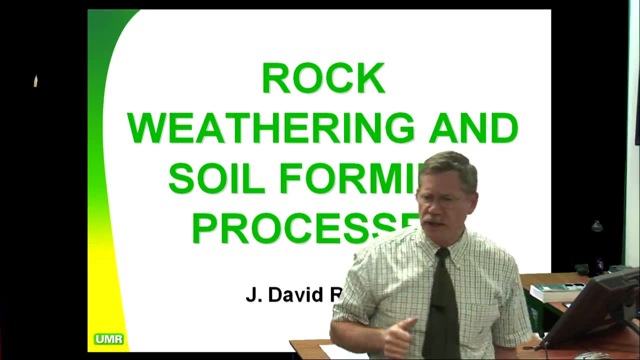 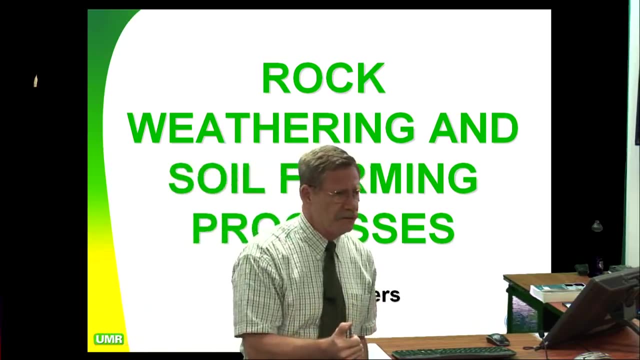 So finally he says, we over here the real engineers, structural engineering, we can calculate strains to half a percent. What can you do? Soil mechanics? the best we can do on strains is about 150%. So if you've got to do things with a lot of precision, 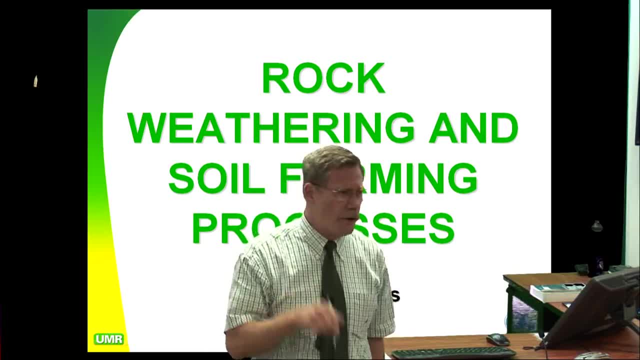 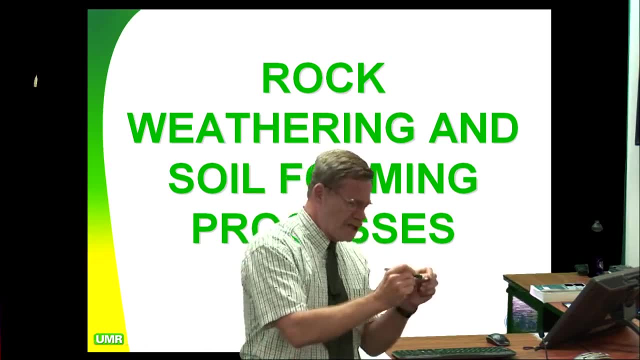 get out of this business. This is the business that takes an enormous amount of engineering, judgment and maturity. You want to be a pinhead and just run everything out of a computer to 74 decimal places, which isn't realistic. it doesn't mean anything but make you feel good. 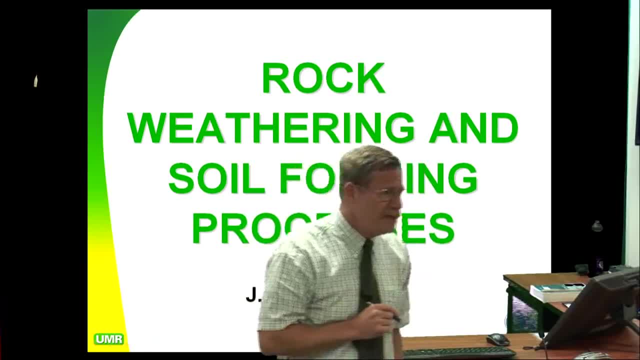 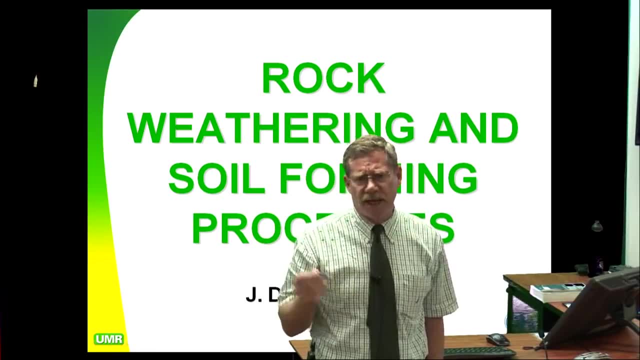 You sit down and your sphincter is nice and loose. Oh, I calculated it to seven decimal places. Who are you fooling? Go to structural engineering Now. rock mechanics, much worse Rock mechanics. you're lucky to predict strains. 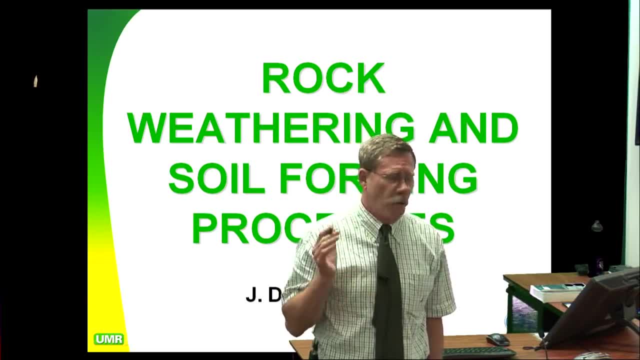 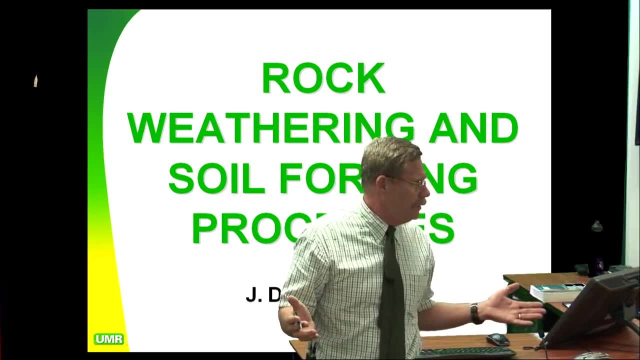 You're lucky to predict strains within 300%. That's on a good day with a world-class field of people. Now why? Because we're dealing with things that were made in the ground. They are incredibly heterogeneous. They are orthotropic. 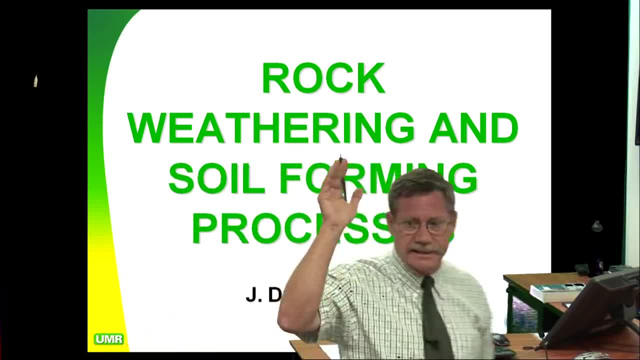 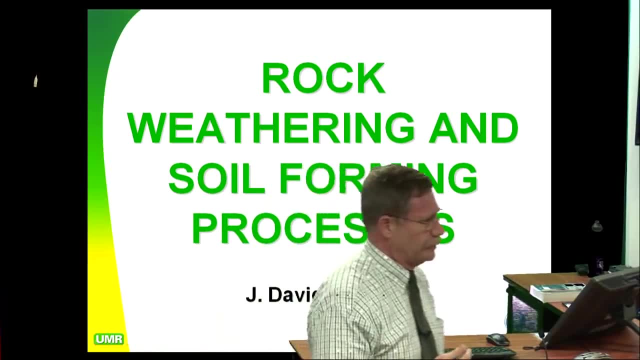 Have you ever heard that word? Orthotropic? Anybody take timber design? yet Probably not. That's not sexy. Timber design is what you want to have. You're going to work in bread and butter civil engineering. Most of the structures in the world are made out of timber. 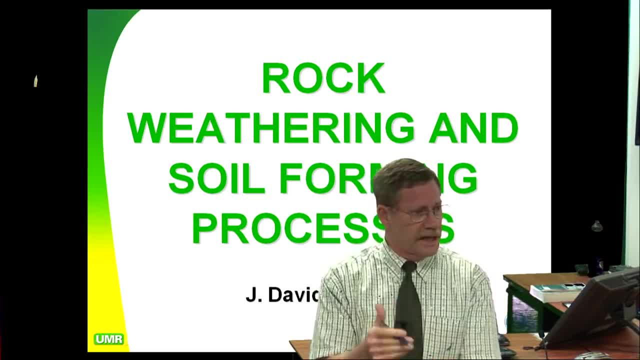 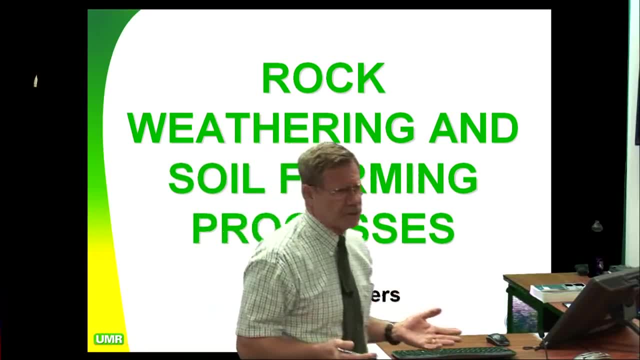 Timber is orthotropic. It has different properties in all three axes: X, Y, Z. That's what rocks are like, Now soils- a lot of soils- are transversely anisotropic, which means they have different properties perpendicular to the bedding. 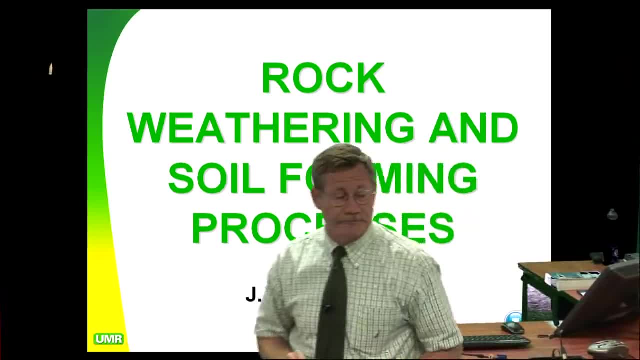 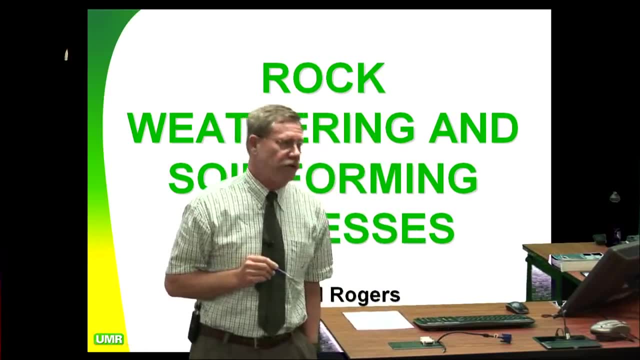 but in this direction in the bedding and that direction in the bedding, they're more or less the same, unless they were deposited in a channel like New Orleans. New Orleans, they're orthotropic. What does that mean? That means the permeability. 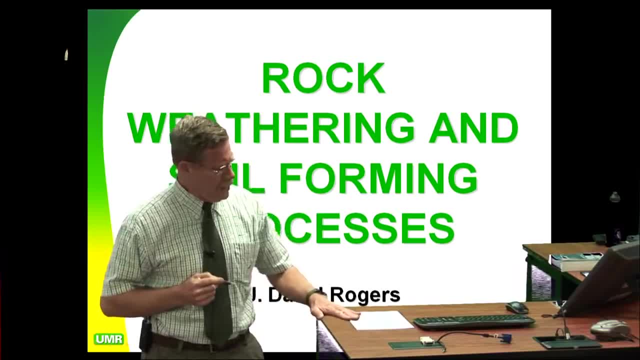 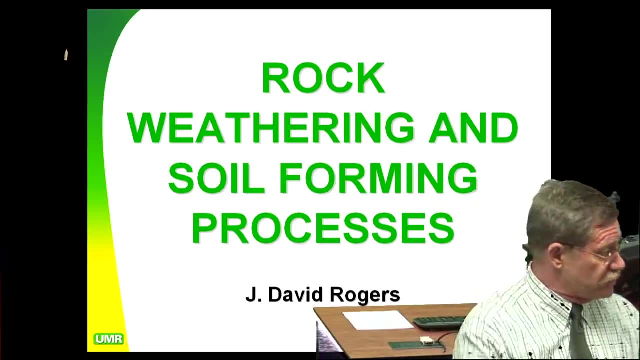 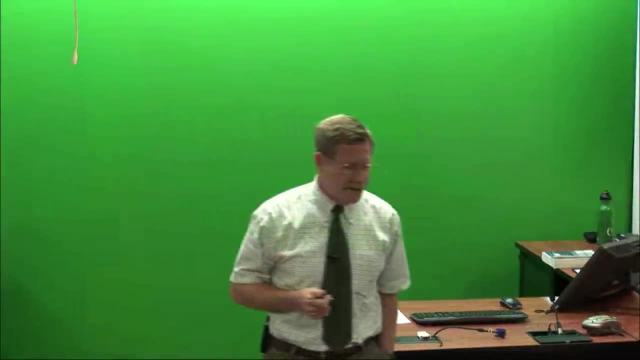 or hydraulic conductivity with respect to water in old channels is super high, very, very high. It's not as high going this direction and that direction. All the engineers down there assume it's all the same, but it's not. I had a whole bunch of professionals down there- Army guys tell me. 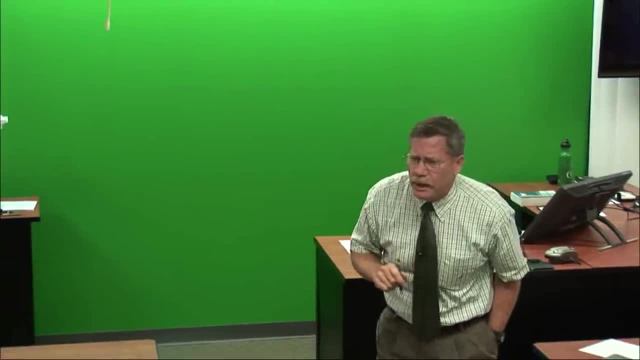 you know the peats are not pervious. Oh, do tell. Why is that? Well, because we have data showing that. Where's the data from? Oh, back in the 1960s. How much data do you have? 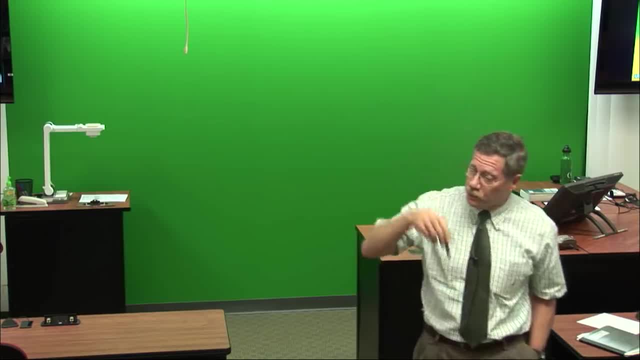 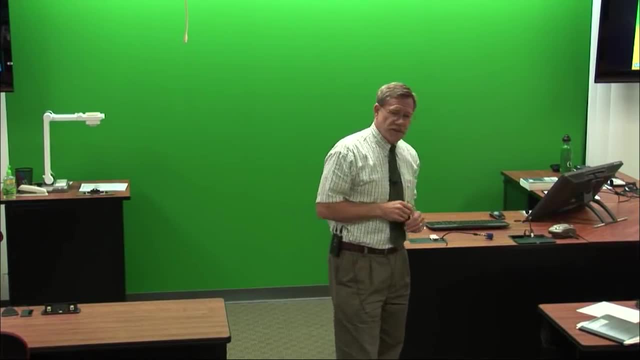 Five tests. What kind of tests did you do? Well, we drilled vertical holes through horizontal shale and peats, beds, silts. So right away, you're going down this direction and then you're going to tell me what the permeability is in that direction. 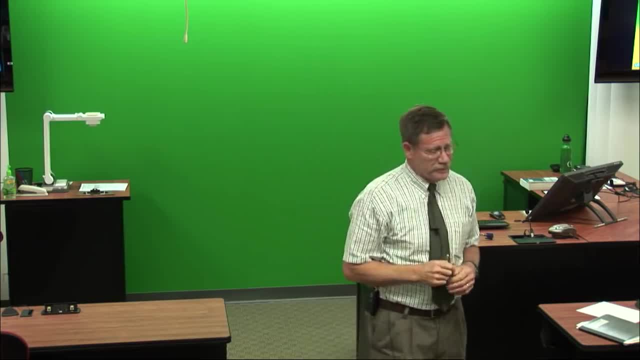 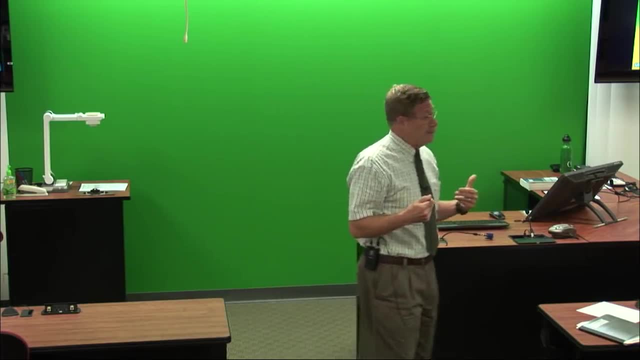 That doesn't work. You've got the sample going the wrong way. Now how did I get to my opinion? Oh, Festus, I'm one of those guys that sits on drill rigs. I was probably the only guy after Hurricane Katrina sitting on a drill rig. 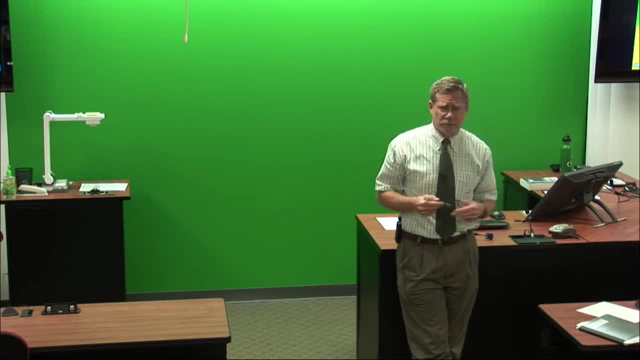 who was over 50 years old, who was down there for any meaningful period of time. Everybody else drilling holes was young kids pulled from all over the country and all these different consulting companies. Now you sit on a drill rig. you learn a lot and you learn about behavior. 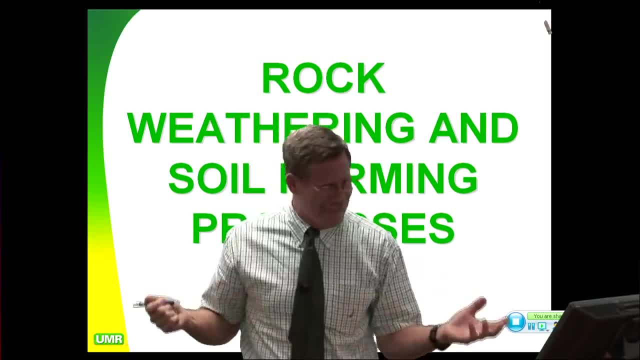 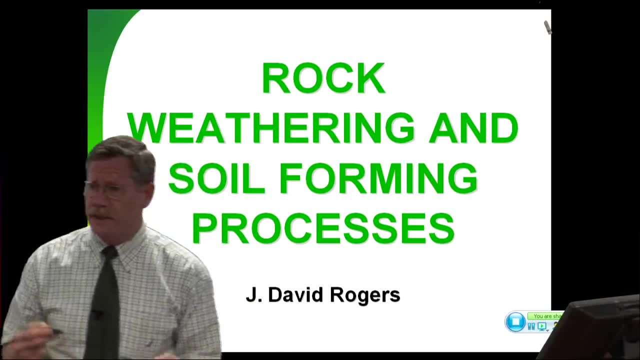 We extract properties from behavior, and behavior controls everything, As we're going to learn when we get to Chapter 5, we talk about rock mechanics. Differential strain is everything in rock mechanics. You don't care about stress, It's a strain that kills you. 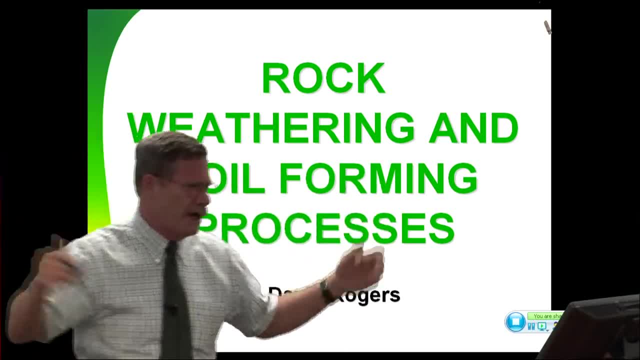 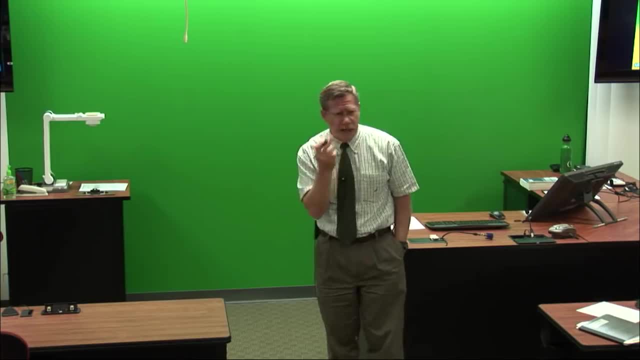 We talk about stress because it comes from solid mechanics and mechanical engineering. We love to talk about stress and calculate things to four decimal places, But in the real world what you're going to be looking for with your Mark 1 eyeballs is evidence of strain, things like dilation, cracks, opening up, stuff like that. 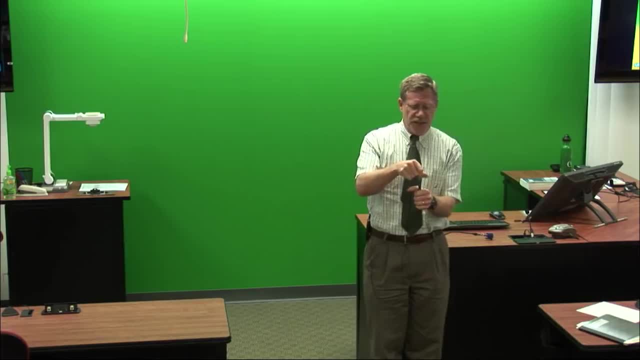 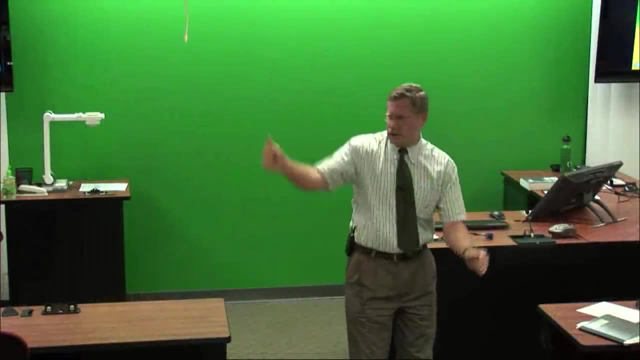 Okay, it's not that hard. I get down there and I'm pushing samples through this stuff, through this impermeable piece. They're impermeable And as I'm pushing the Shelby right here, water's squirting up out of all the adjacent holes. 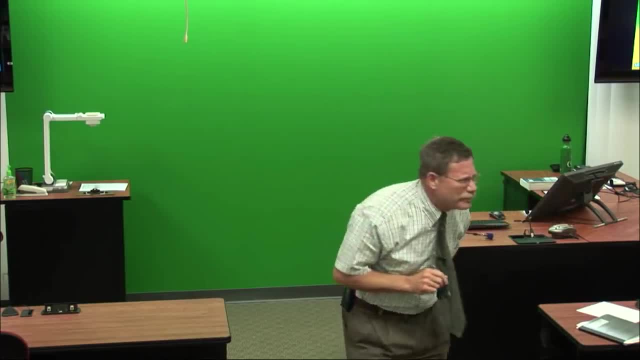 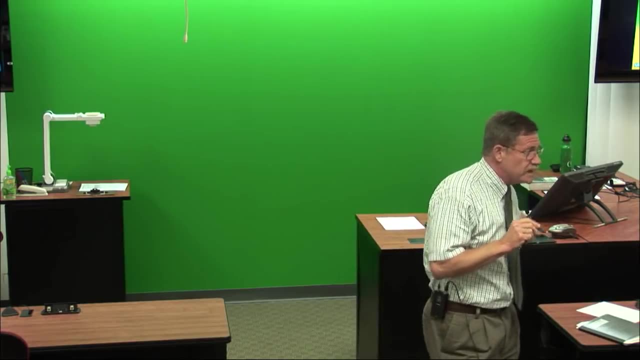 Because I'm Swiss-cheesing the place with holes. Now how permeable is something if I push right here and the water squirts up 30 feet away? That's called a BAP- big-ass permeability, Pretty permeable. 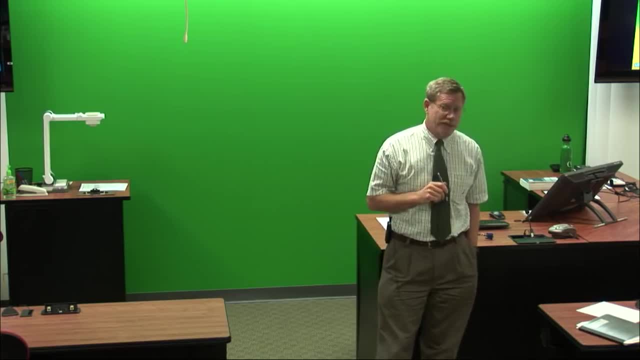 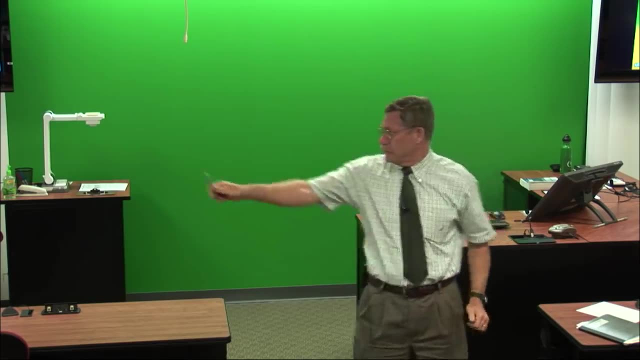 Can't put a number on that one. It's way up there above one centimeter per second. And what we notice too is when we're pushing it. water went higher right there and right there than it did over here and over here. 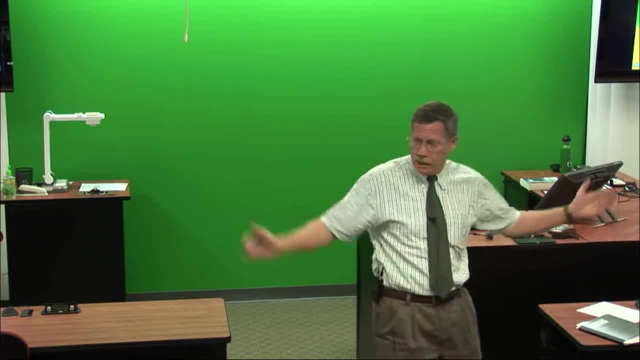 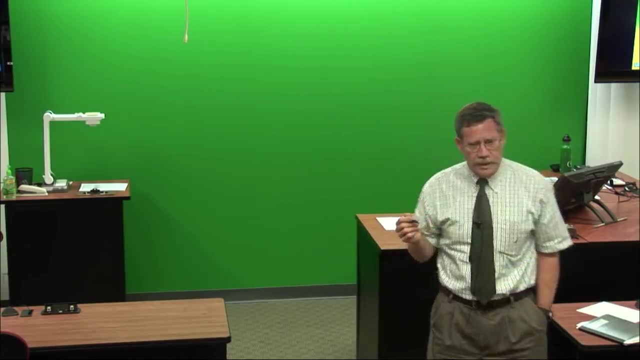 So right away, I see I got some anisotropy. Welcome to geology. Everything about geology is anisotropic. Now, another fundamental axiom we're going to learn today is when you are working on developing a cross-section. 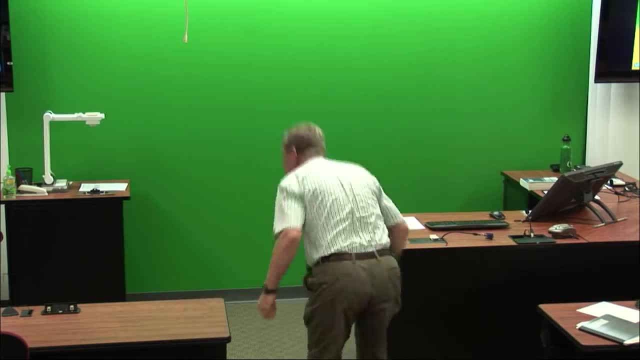 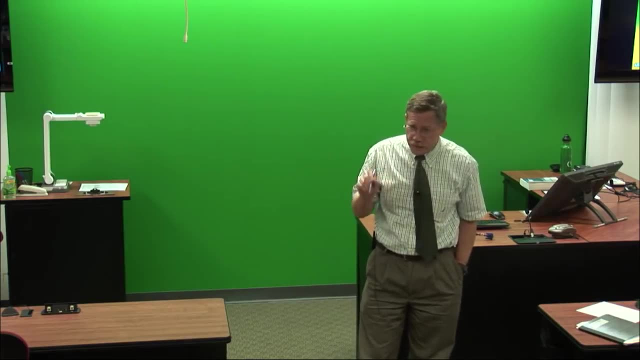 you can embarrass yourself. show the world how much you don't know by drawing cross-sections with rulers. There ain't no rulers in geology. Rulers are over in the civil engineering department. From architecture. Draw everything with rulers. So if you give me two borings, 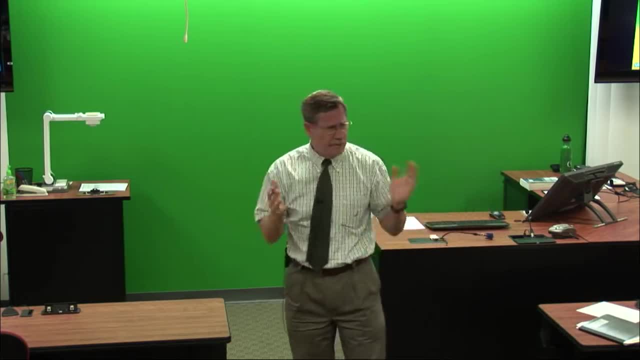 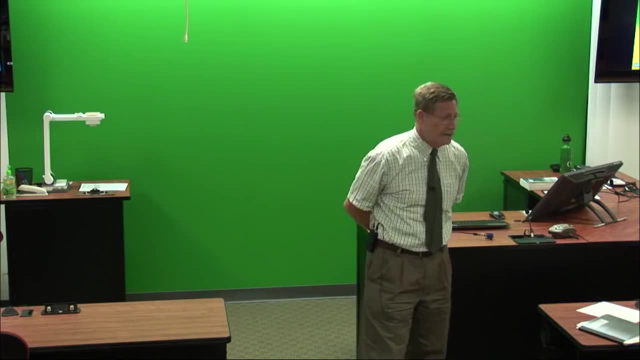 and you're drawing things with a ruler between them. all that tells me is: I'm dealing with a freshman, I'm dealing with somebody who doesn't have much experience. Don't you dare use a ruler. You went through my class. You can get yourself one of those flexible curves. 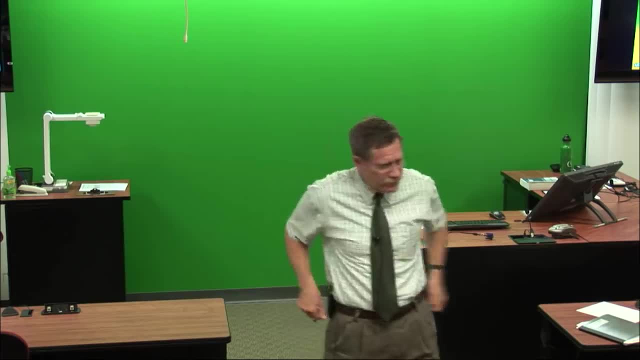 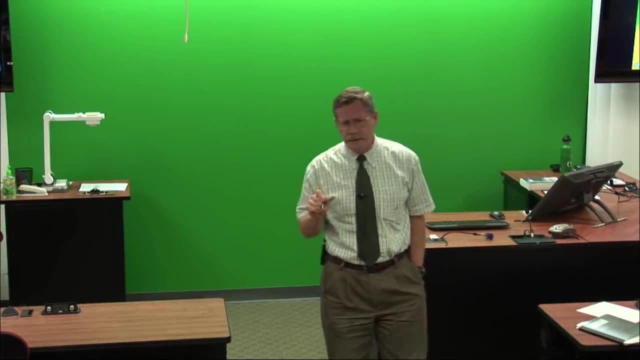 They're nice to try on a date some night, They're nice. You can measure everything And you use a flexible curve, because that's how things are in the real world. There are no straight lines in geotechnical engineering. geology- 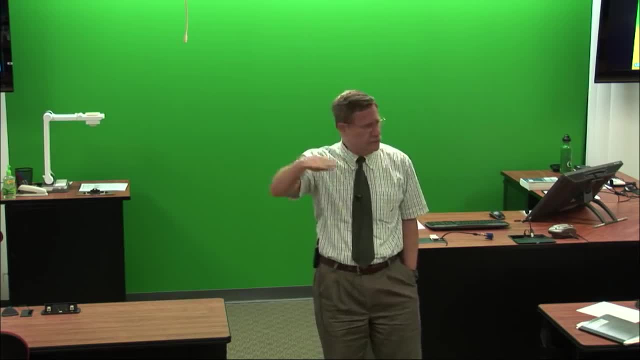 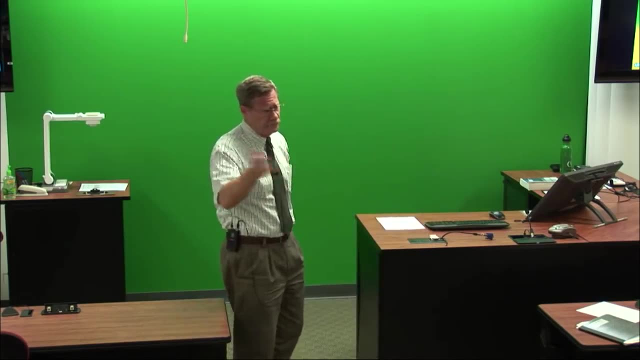 Only when the lake, the lake surface, Got some lake out there. that's relatively flat, but it's got chop on it too, So you don't have constant pore pressure, even under a lake when you have wind blowing. So that's some of the stuff. 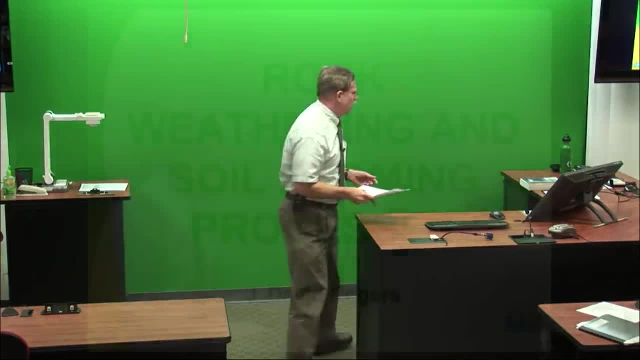 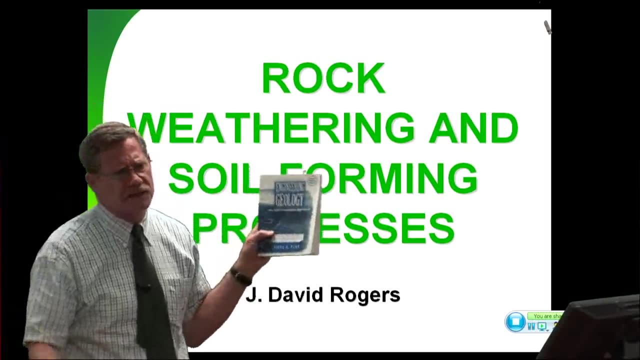 just kind of giving you an overview. We're going to start out by doing about half this book. We're not going to do the whole book. If I do the whole book, I'm going to cram way too much stuff down your throat. 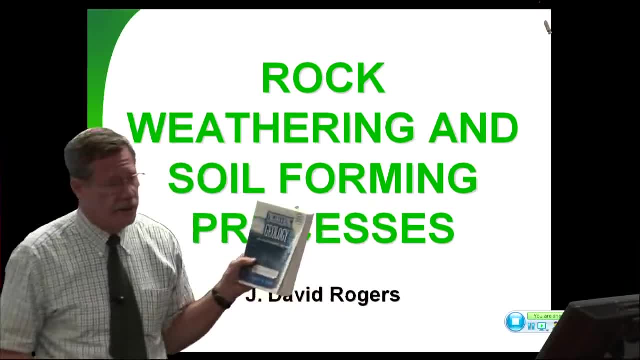 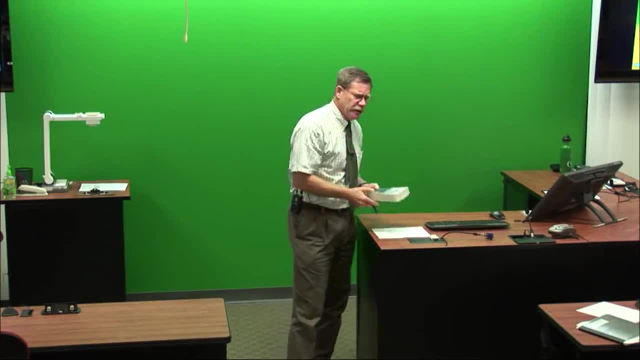 That's how my schooling was. I had 10 years of schooling and they just crammed me down. They crammed all the stuff down my throat And I found out pretty quick. I really didn't enjoy being an undergraduate. I just had to take all these different classes. 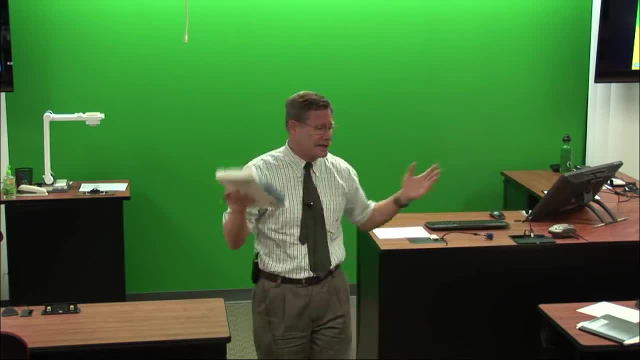 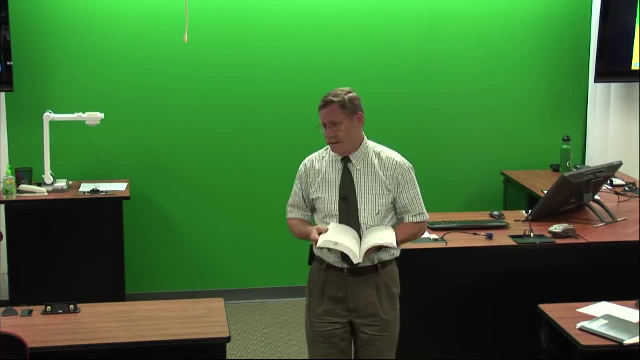 I was doing sports, I was doing military, I was flying, I was doing all these different things. I never had time to crack the books open and read the things. Only the nerds on scholarship got time to do that. I was working all the time. 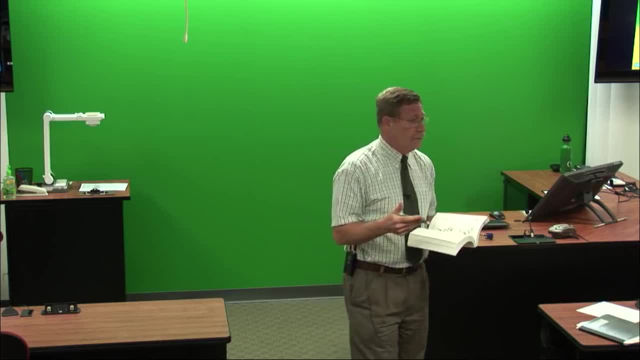 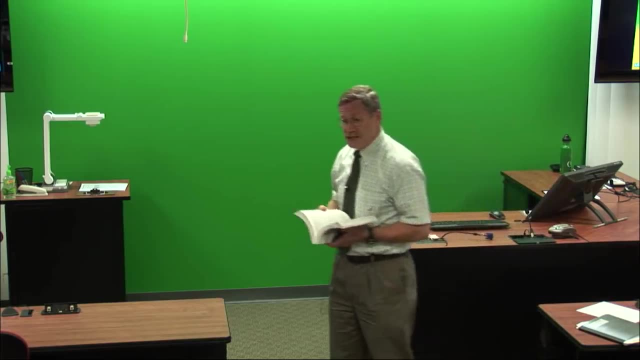 Didn't get to do that. So what I loved was grad school. After I went down to flight school and got out of the Marine Corps, I went to Berkeley, Got to go to grad school, Took two classes. I'd always taken 17 to 23 units. 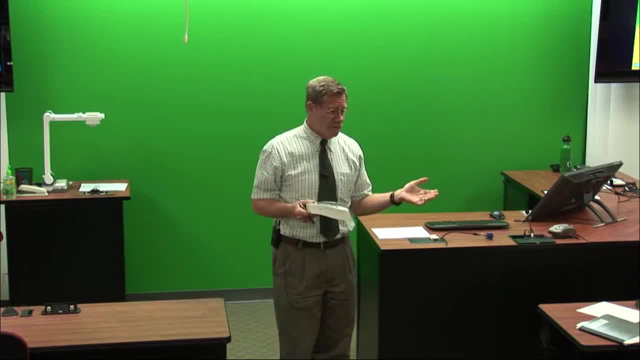 every single quarter. We were on a quarter system. So I go to Berkeley and they say: take two classes, Six units. I could actually open the book up and read the book and enjoy the class. It was a lot of fun. 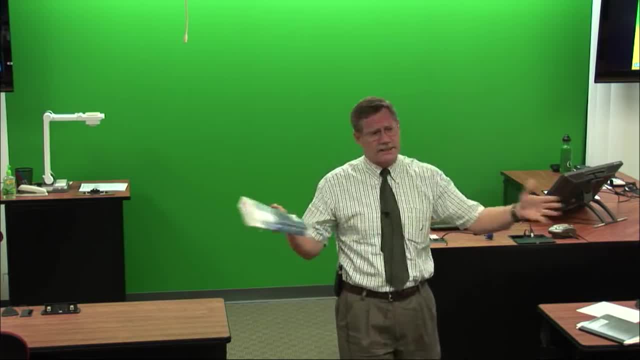 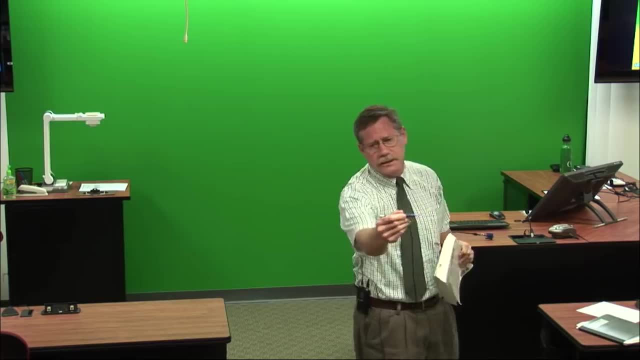 And I ended up staying six years taking just about every class they had in civil engineering program. because my undergraduate degree is in geology. I wanted to get the depth in civil engineering so I could go take the PE exam. The PE exam is the exam that counts. 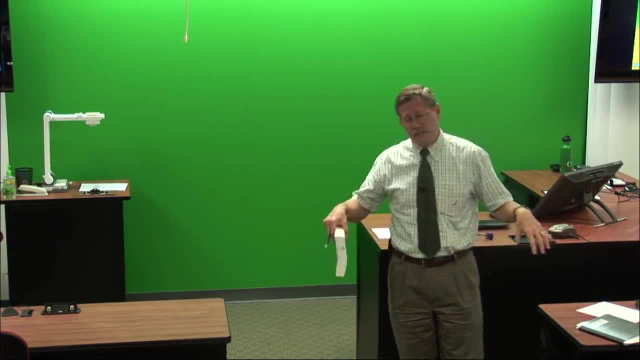 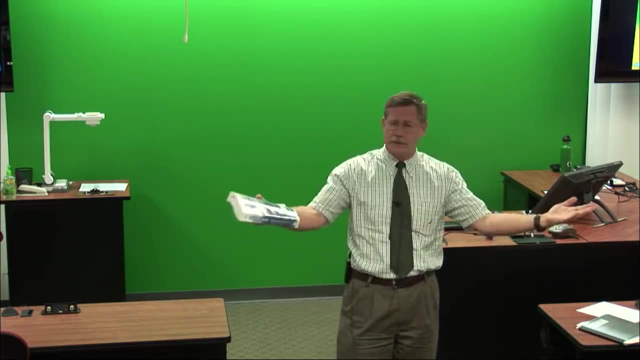 That's the exam you want to go take Now in this program. in Missouri you get double credit. They don't do that in California. Here you actually get double credit towards PE and RG registration. California you got to pick one or the other. 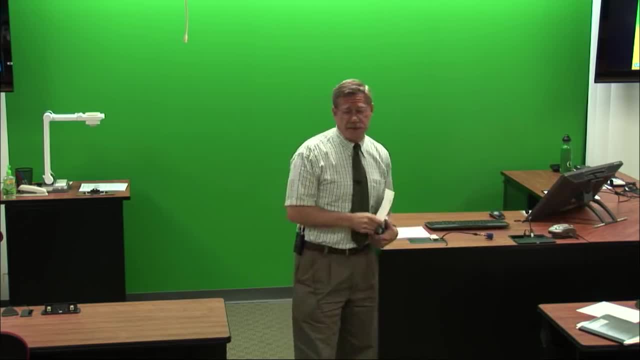 So it took me many more years to get my geology registration in California because I was already a PE. So every time I would apply to take the exam, they'd say, hey, you're not a geologist, You're the enemy. 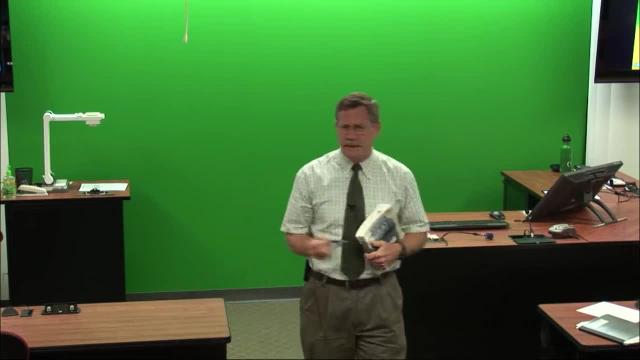 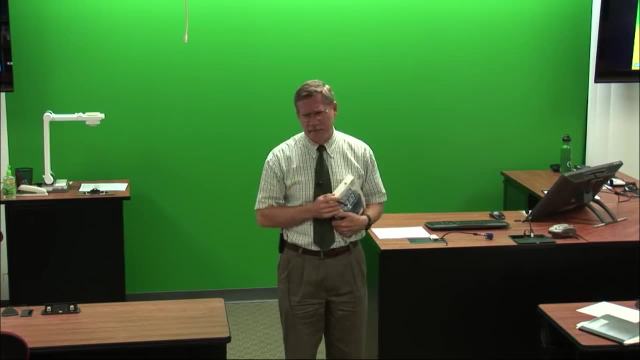 You got P behind your name, Isn't that for physical education, Petroleum engineering? No, You're an engineer. You're the enemy. I go what? Yeah, we don't want you taking the exam. I have an undergraduate degree in geology. 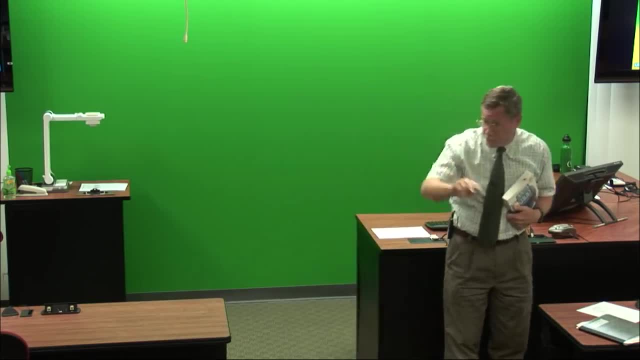 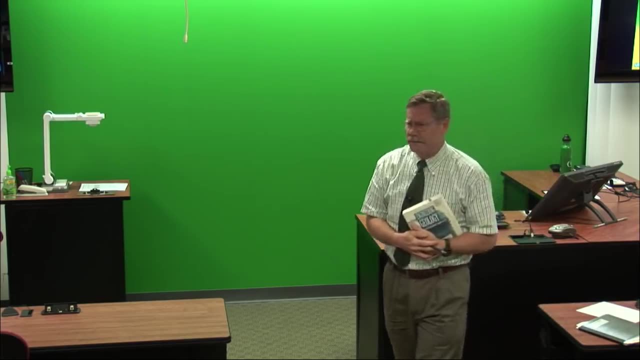 Yeah, but you're practicing engineering. You're not a geologist anymore, You're a trader. You went to the other side, the dark side. Probably don't even drink beer anymore. No, I don't drink much beer. It makes me fat. 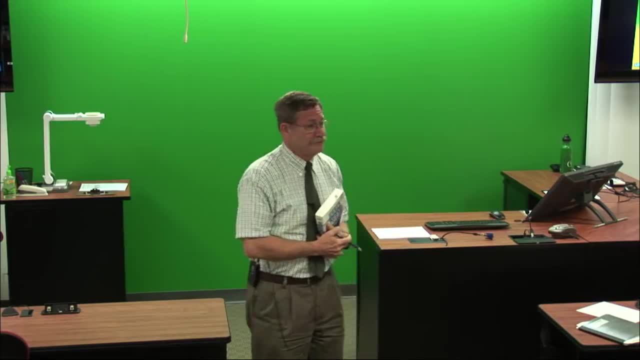 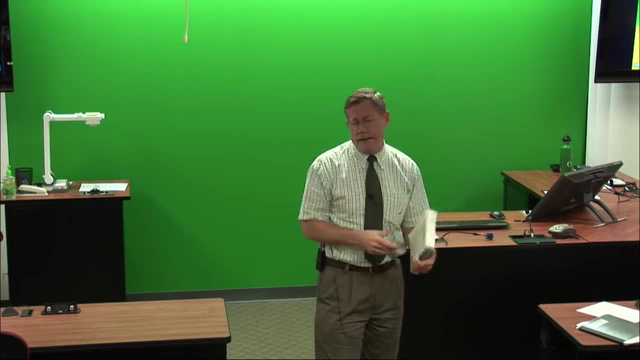 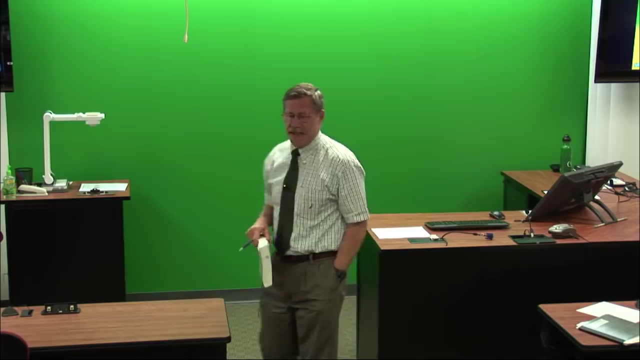 So I drink goat's milk- Really weird. So I decided to take all these CE courses so I could pass the PE. Now California had a real tough PE exam prior to 1976. It was very much structures-oriented. They didn't have the national exam yet. 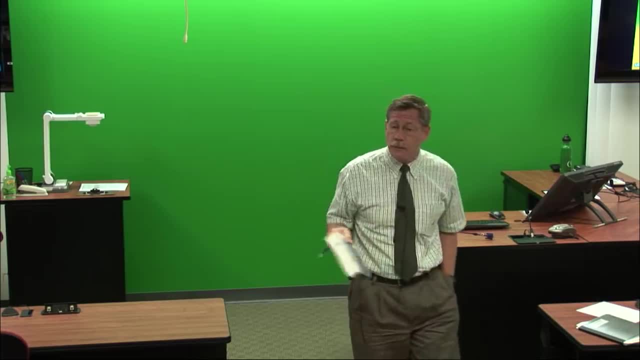 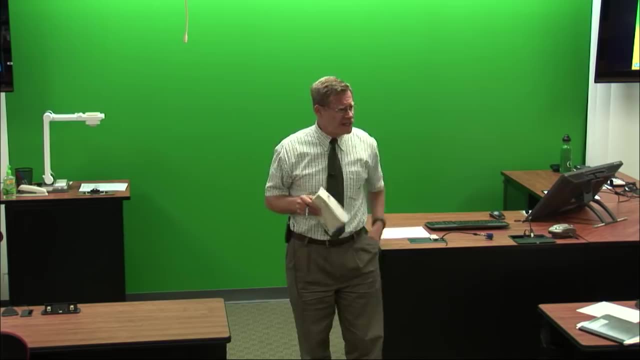 And so I minored in structures and took all these structures classes, And that's really where I learned dynamics, especially in structural modeling. You get a chance to take structural modeling and you're going to go into earthquake work. That's the place. 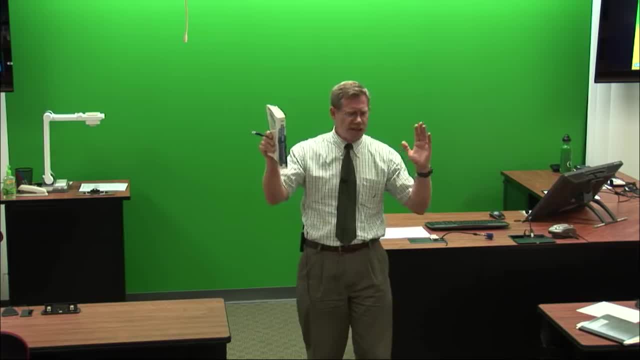 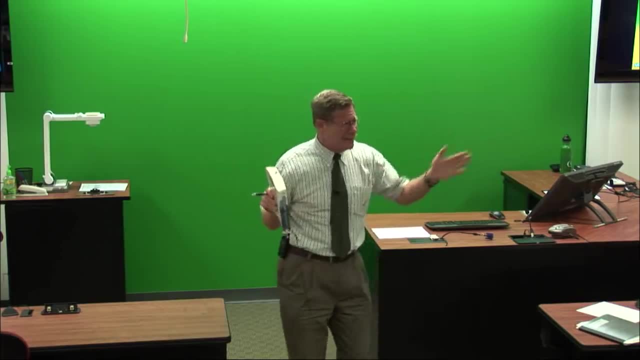 using the strobes and the shaking tables, where you actually get to see dynamics. Dynamics is impossible to teach on a static board. Dynamics is about things moving. It's like watching the babes in the bikini at the beach. I can't do that one for you on the board. 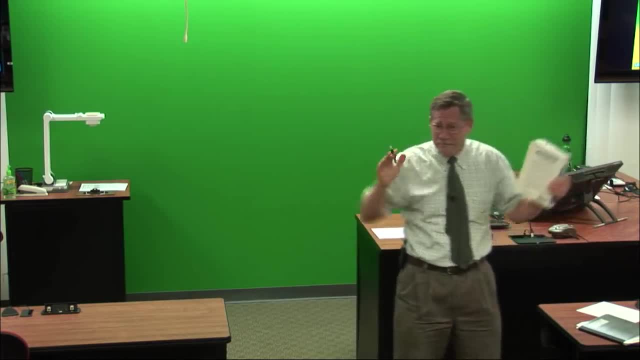 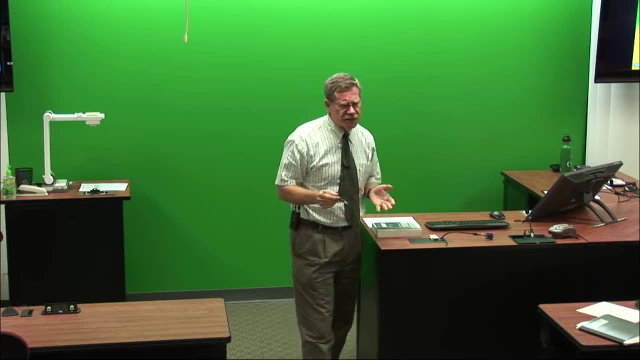 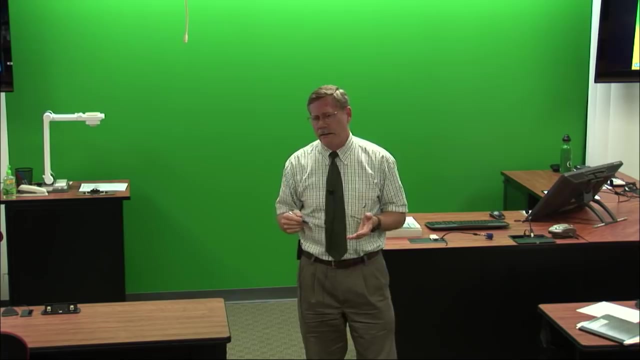 It just isn't the same. Things are moving around, They're oscillating And anyway, what I learned through all that was you're going to use everything you learn at somewhere in your career- you don't know where The structural engineering I learned. 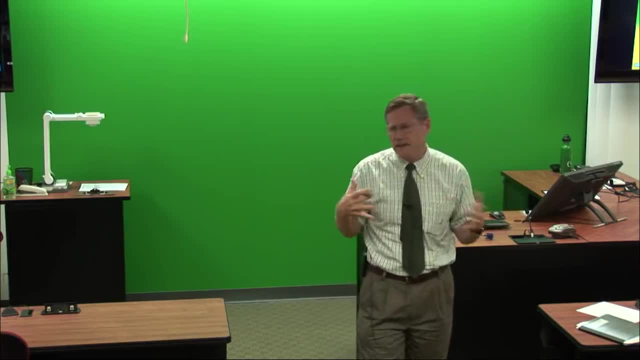 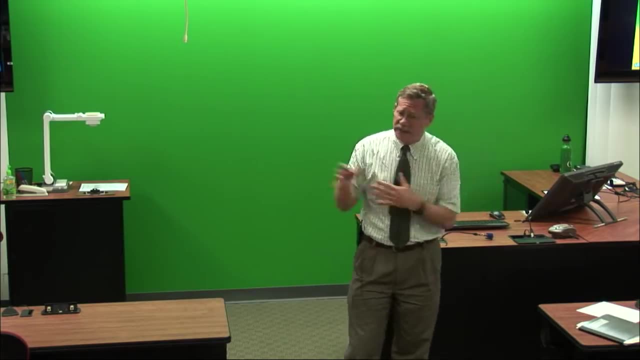 was fantastic, Because all of my biggest arguments that I had in my professional career were not with my clients. I'm a pretty fast-talking guy. I can make people feel good, I can tell jokes. I'm a great guy. I don't play golf. 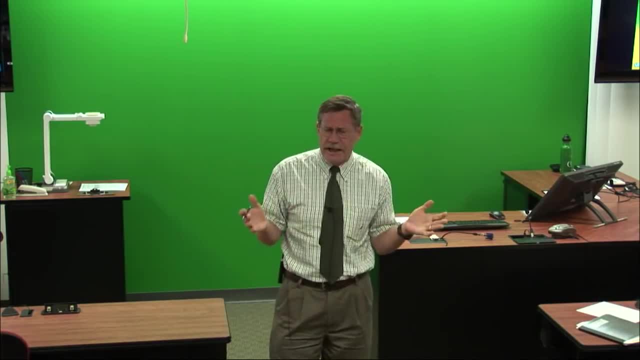 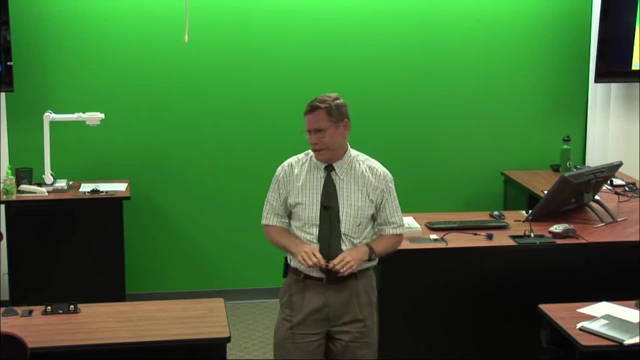 I don't do any of those things, But the biggest arguments I had were with structural engineers, Especially structural engineers designing shoring, temporary shoring, working for a contractor, Usually with only an undergraduate degree and usually with one class in soil mechanics. 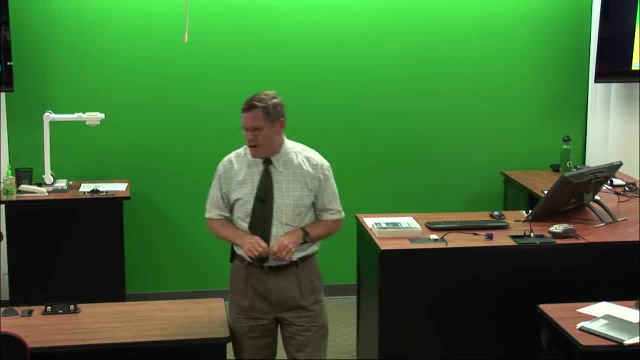 In 1947.. Wasn't Terzoggi? wasn't he one of those soil guys? Yeah, that's about it, And they'd be telling you what to do And you're sitting there going. now wait a minute. 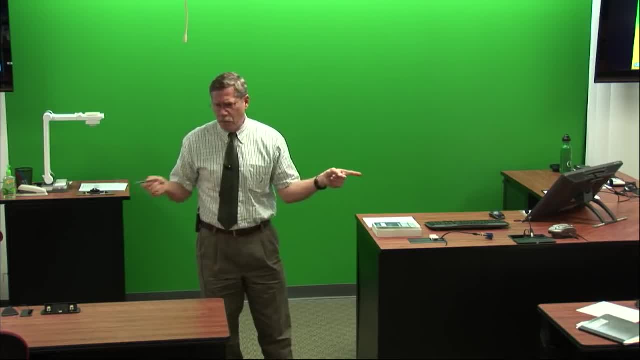 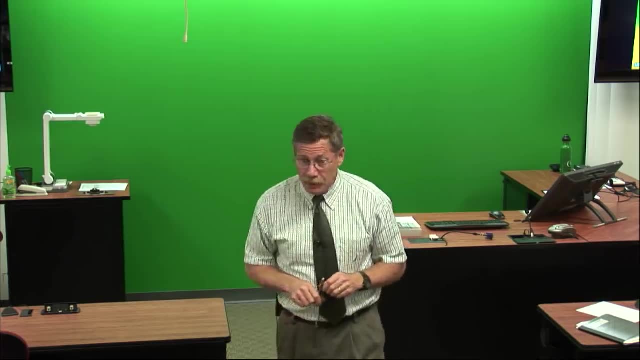 You've got one course in soil mechanics. I've got 37. Why are you telling me what to do? Because I was designing these things when you were a boy scout And I don't like what you have to say: Yeah, You're going to get that. 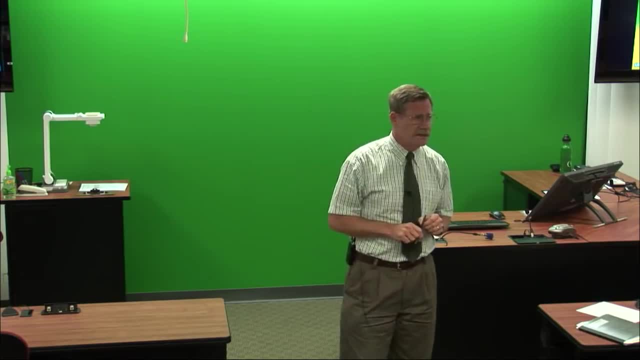 Especially your first few years out of college. You're going to get some of that kind of stuff And you've got to be respectful And you've got to become a teacher And you've got to try and teach the person. So one of the things that I learned to do- 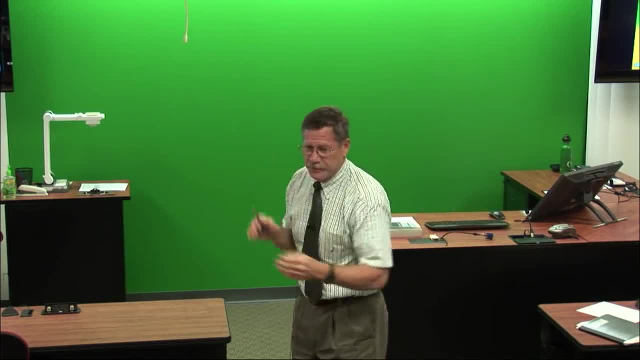 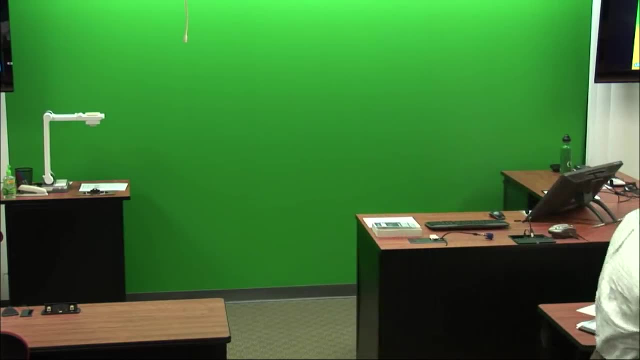 is. I have a big library of disaster pictures. That's porno for civil engineers. man, Show the disaster pictures. Look at this. Try to build a wall, just like you're doing it. You can see the guys going. I don't want that. 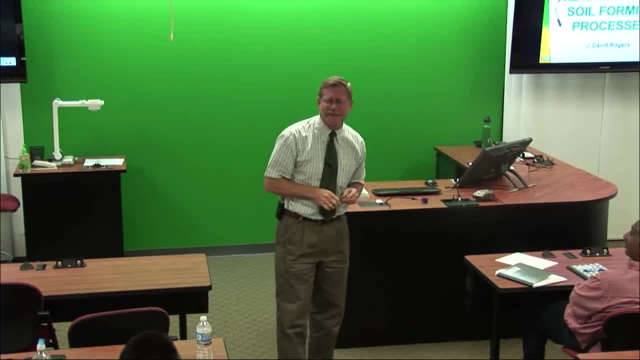 How'd that happen? Probably had a geologist in the project somewhere. That's what it was. So you have to be able to be convincing, And you have to do it with images. We live in a visual society, So you can talk a lot about things. 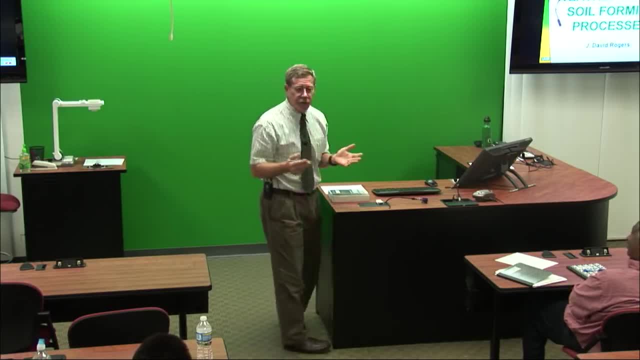 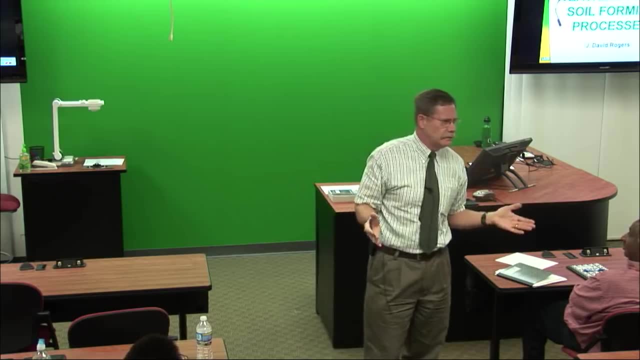 You can talk fast about things, But you have to be able to show people. here's why I'm concerned about this. Let's walk out here and let's look at how this project performed. That was always my strongest straw Whenever I went to work in a new area. 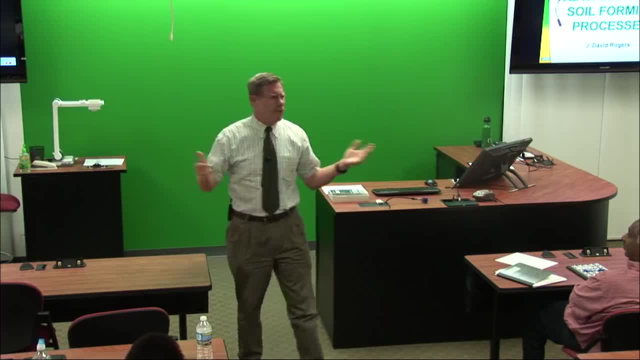 I remember I got a job once down near Porterville. It was in the San Joaquin Valley. They don't do soil mechanics in the San Joaquin Valley. It's flat, It's all sand. I mean, what do you need soil mechanics for? 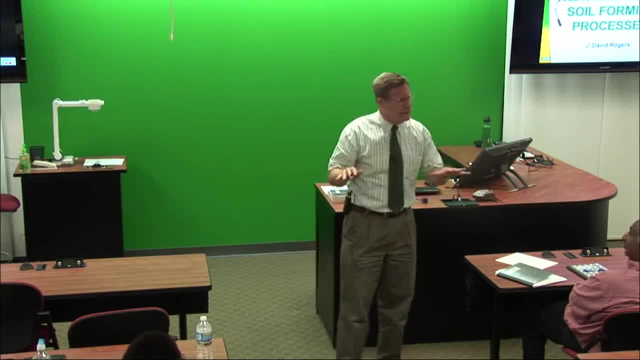 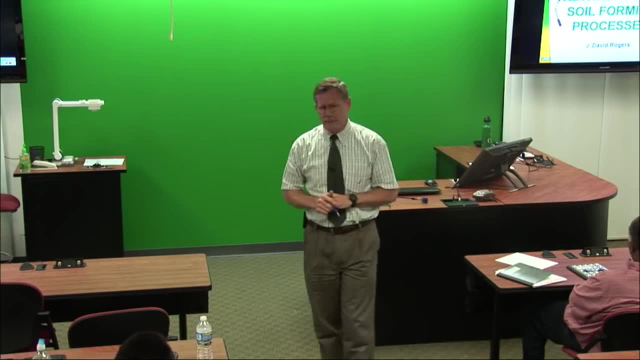 That's what these guys were asking. Well, they were in a pocket area that had expansive soils And they didn't have the sand there. And this guy with the bank was concerned and said: we think you need a soils report because we've had a lot of problems. 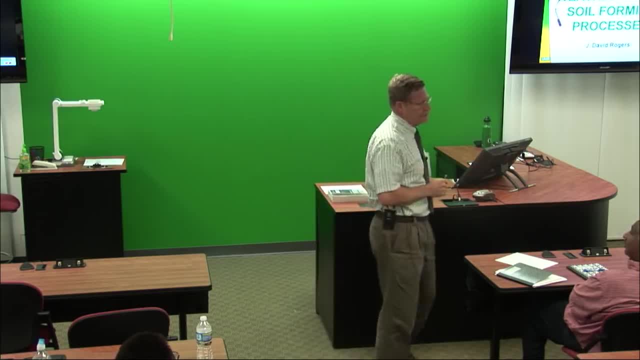 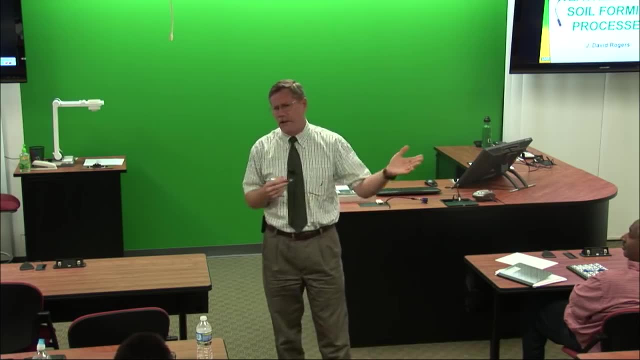 with property casualty losses in that area. So we want you to hire this Rogers guy down in LA. And Bob said, well, I don't want to do that. Well, he got forced to. So, yeah, you're going up here with a hostile client, basically. 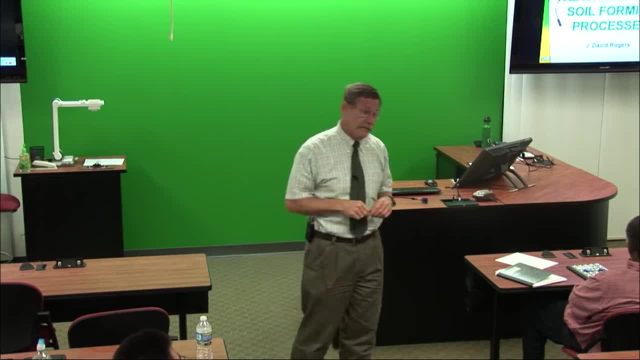 It's like a hostile date And you go up there just looking forward to it And I went up there and I go up a day early. What do I want to do? I want to cruise every street around, you know, within a couple miles. 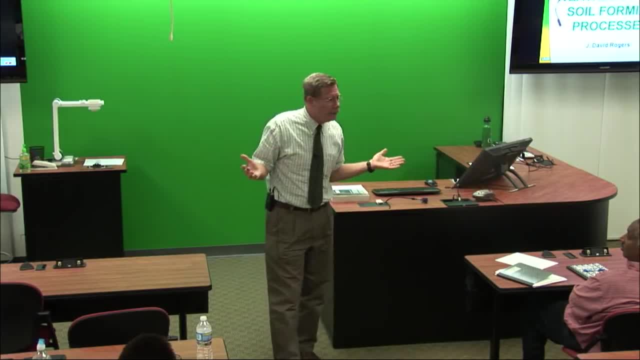 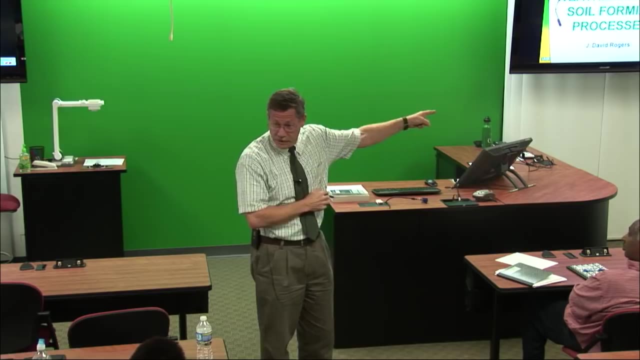 of where his project was going to be. and look at what. What do I want to look at as a civil engineer: Performance. Look at the street. Is it even? Does it have cracks in it? Are the cracks showing offset? We've got some dandies right out here on US 63, on Bishop Avenue, right here. 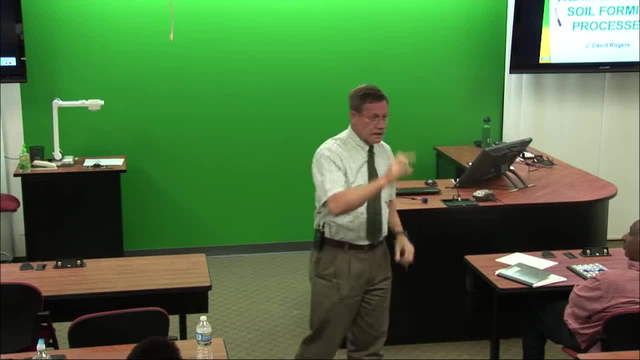 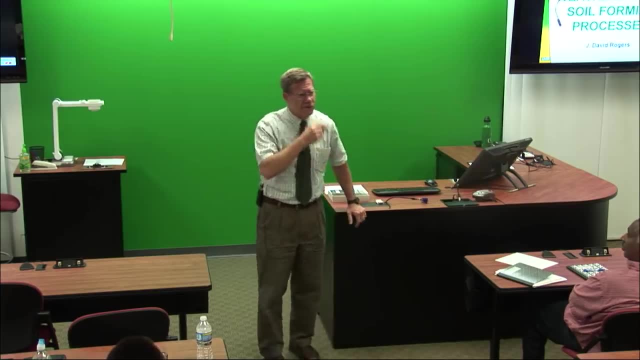 right by the light that just showed up last spring Settled about three inches. You ought to go out there and look at it, Nice and straight. Come back here and tell me. I'll give you five bucks if you tell me what it is, because I know what it is. 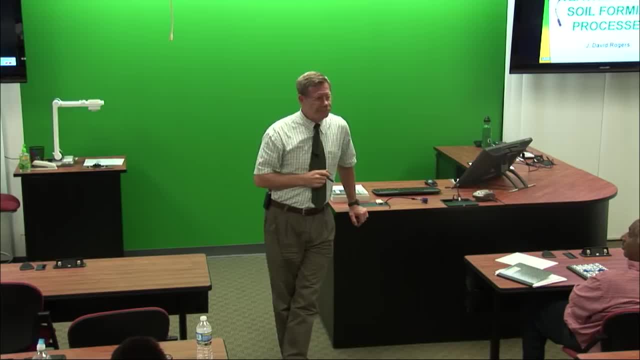 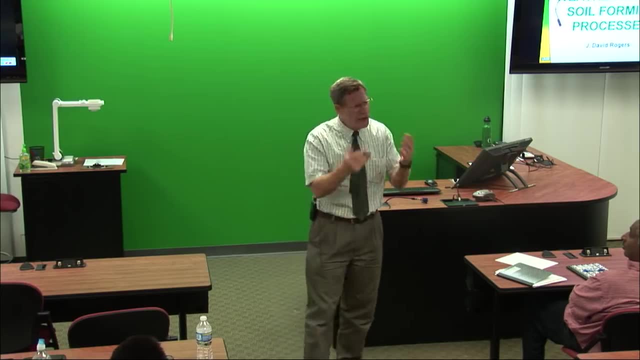 And it's from only four and a half years ago. That's why you have to compact things. If you don't compact things, oh I don't need to compact. I'm only putting in this: much Great, Try it, See what happens. 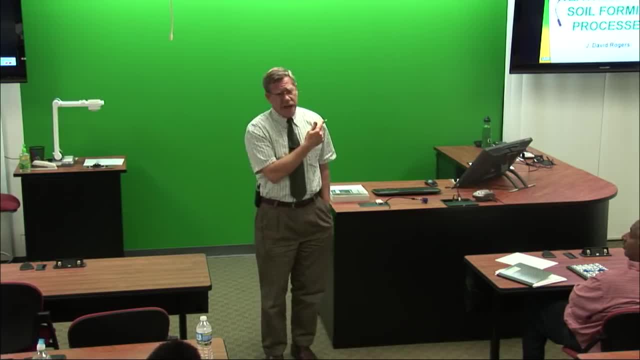 You get a nice big crack going down the street. Now, if a truck hit that at 45, 55 miles an hour, it could cause a load shift, It could cause a fatal accident. You know that if you take your transportation engineering courses. 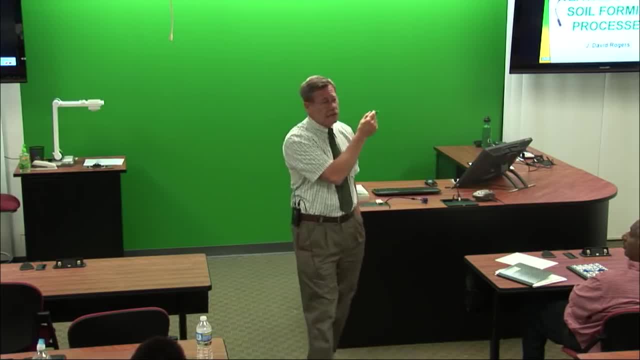 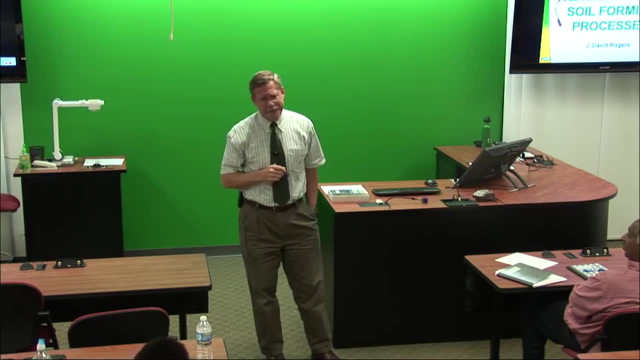 That's a real. The only reason this hasn't caused any big grief yet is it's got a stoplight right there and it's about a 30-mile-an-hour turn. It's a tight turn on old 66.. Okay, So you go out there and you look at performance. 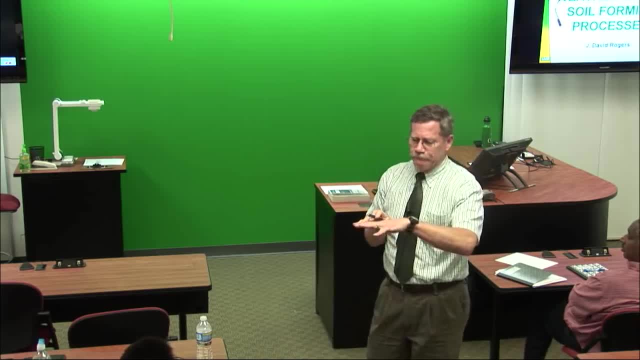 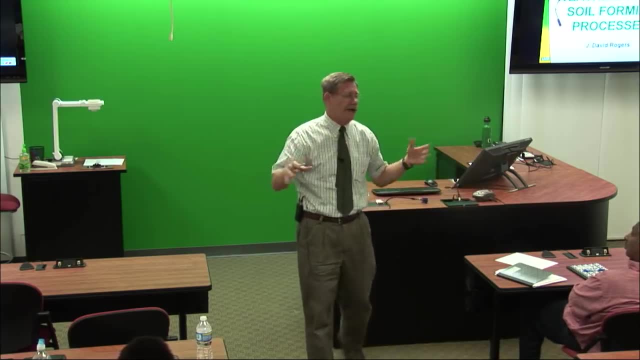 You look at the driveways, You look at the garages, You look at all the flat work. If you're on expansive soils, you're going to see all this stuff moving around, cracking, breaking up. So the next day I meet the client. 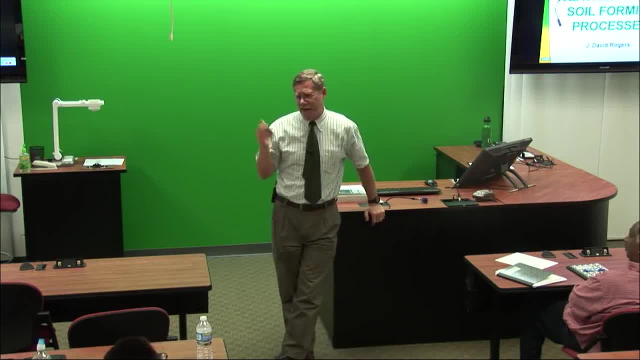 He's a man out there bright and early. He's a contractor, so I meet him at 7 o'clock, breakfast at 5 and go out at 7.. It's the middle of the day for a contractor at 8 o'clock. 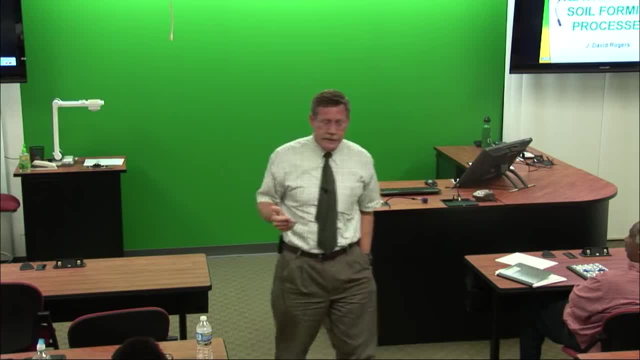 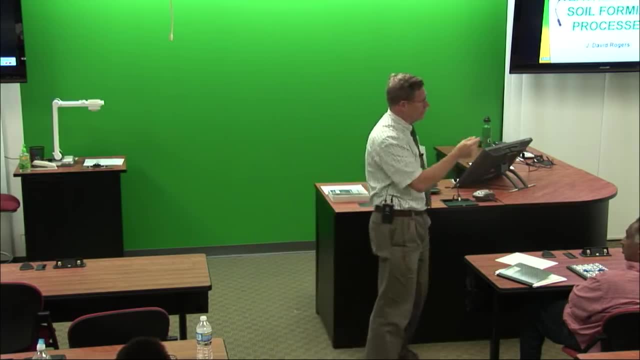 So you go out there and what do I do? He goes out and shows me his project. I'm very respectful, I listen to everything he has to say. Then I say I want to show you some subdivisions over here on the same geologic materials as right here. 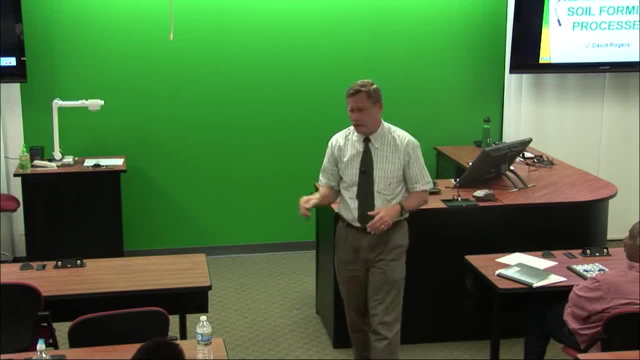 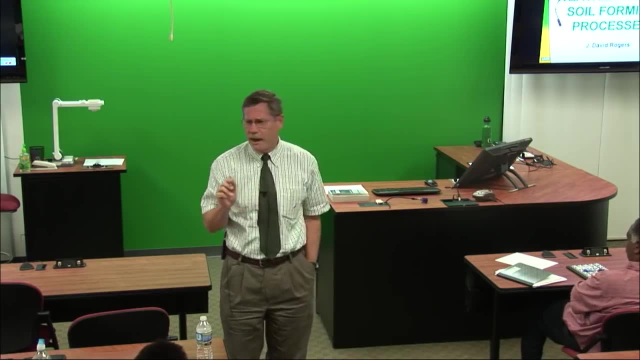 Here's my soil map I got from the Soil Conservation Service. I want to walk around over here. I'll show you a nice身etized soil map and let you see what all of these pieces have, And then take a quick look at the rest of the soil ones. 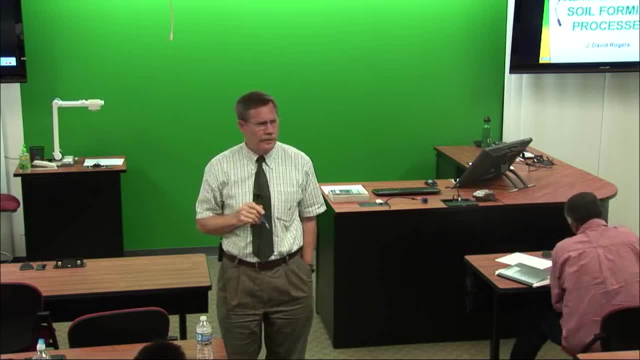 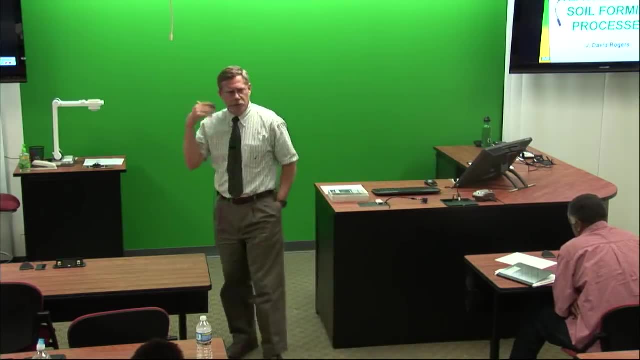 This one is stupid. This is what I've got here. That's where I put in all the pulp. It's red. That's why you have to turn it up. See all the soil here. I got them done right here. 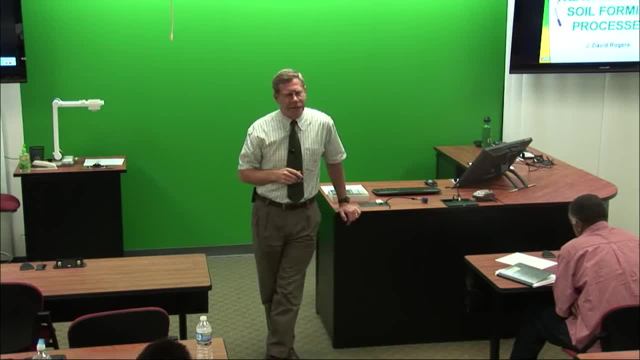 Do the same with the available pans Isolated soil. It will make it save me some money. I'll get my composed soil to repower the multiplexing Awesome to your boss or to your client. you got to look for stuff like that. you got to. 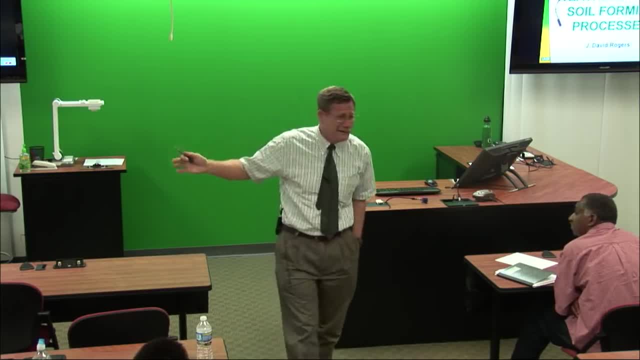 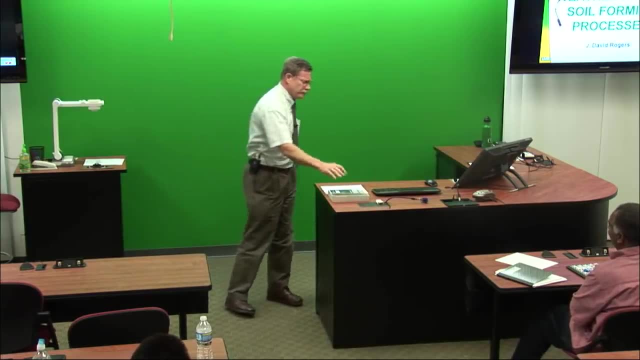 take them out there and show the real world. I can't show pictures of Nigeria someplace in on this out of the world. I got to show them something that's right there and their back door right on their back door. okay, so this is the book we're. 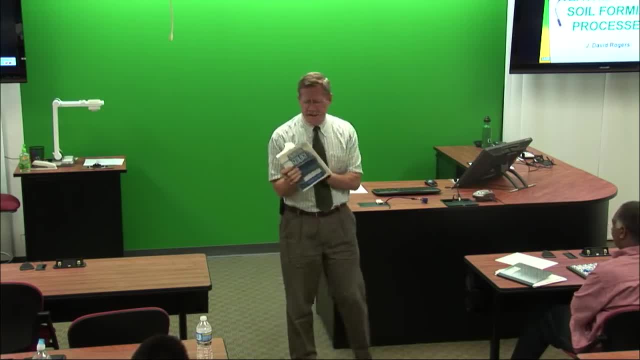 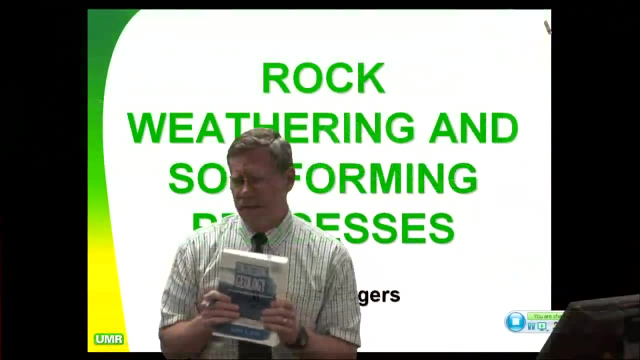 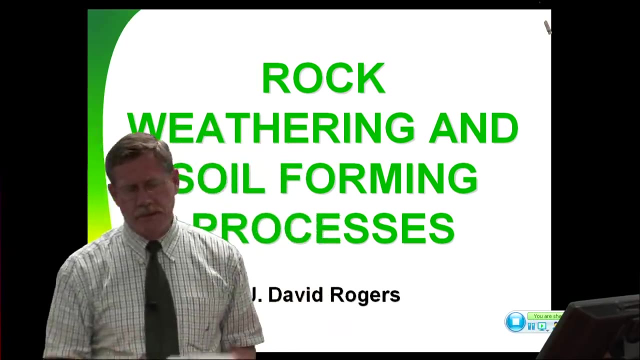 going to use. it's Perry Ron's second edition engineering geology- terrible pictures in this thing. pictures are terrible. the problems they have in it are good. that's why we use it. we're gonna probably look at less than half of the book, so I want you to read the chapters I'm going to assign and this: 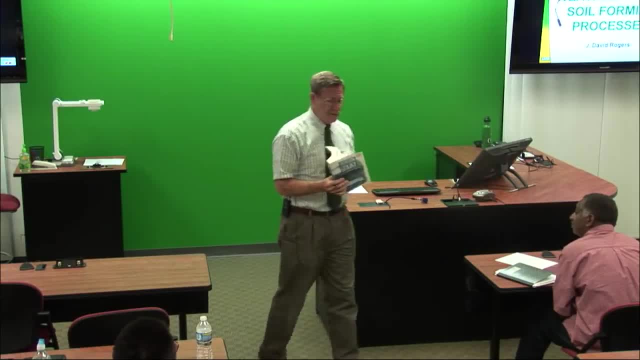 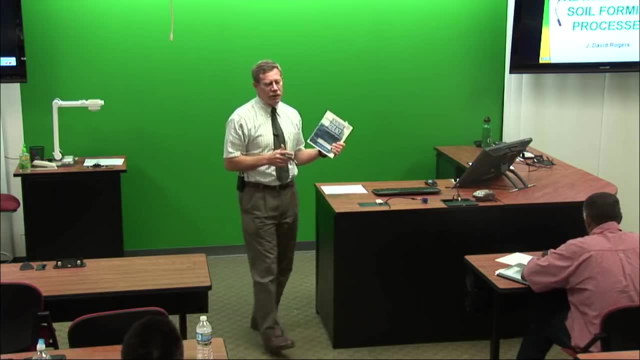 week we're going to do weathering of rocks, which is chapter 3. chapter 3 doesn't have any problems in the back, so I'm going to give you an assignment on weathering. it's posted on blackboard, so it's the first assignment on blackboard. 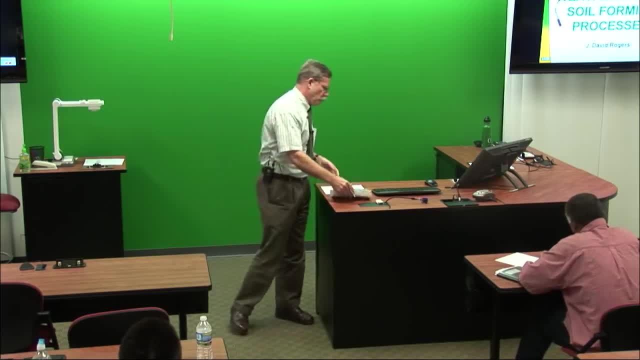 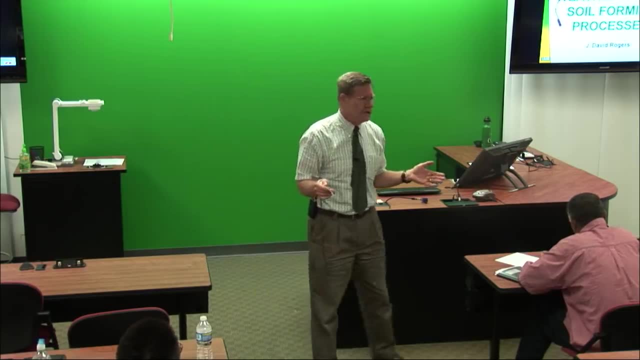 under assignments, weathering. and then after that one, there's one- you on a drawing, a sample cross-section. so that's gonna be your two for this week. now the sample cross-section, I don't want you to kill yourself. that's a real world example from Budapest, Hungary. it's a real case. some of you who don't have 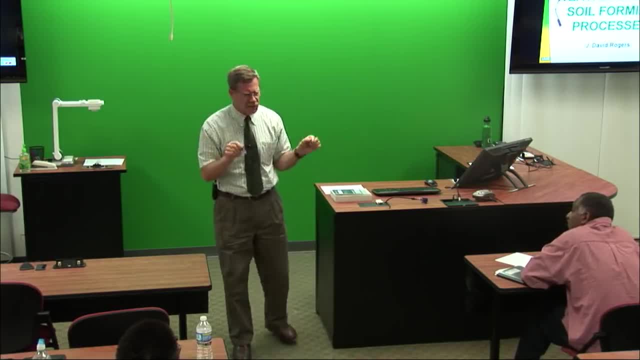 any geology background I can be able to figure out the strikes and dips on the thing. but I just want you to try and do crosshole correlation. don't spend more than two hours on it because you won't get it anyway. it's real difficult, but I 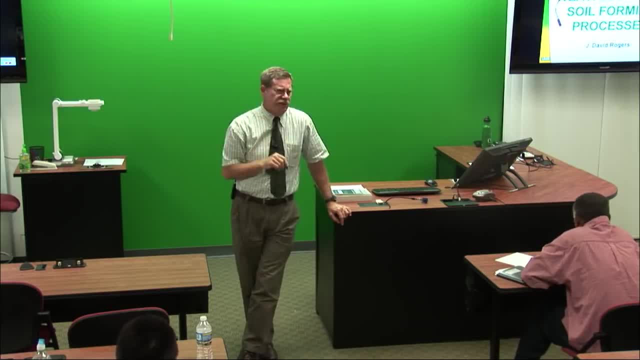 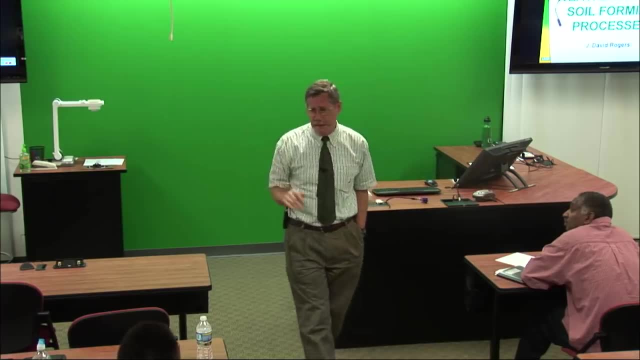 want you to appreciate how difficult it is by trying to do the correlations yourself. and then I'm going to show you, after everybody turns it in, I'm going to show you the actual cross-section when they and they, when they gutted the place out, I'm going to show you what they. 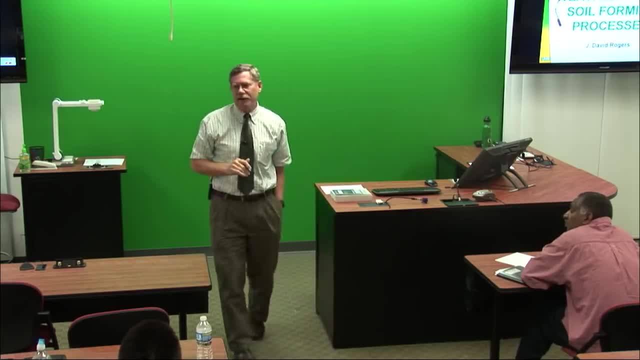 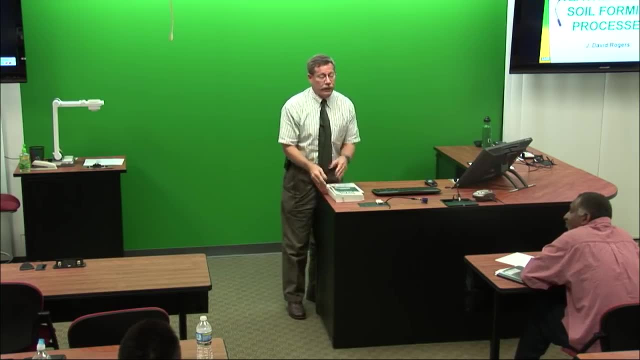 guessed ahead of time and what it turned out to be. oh and if that doesn't scare you, there's nothing I'm saying up here is gonna scare you, but you try to characterize weathered sites that had a lot of weathering. there's a high degree. 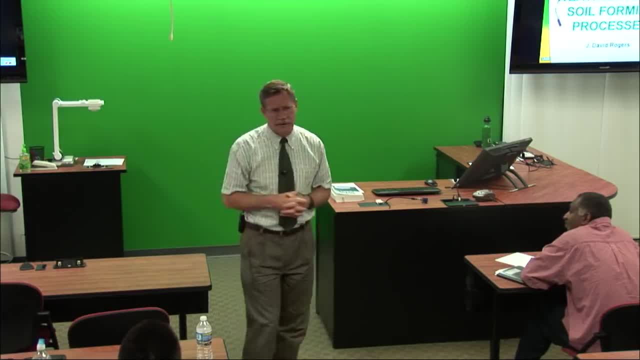 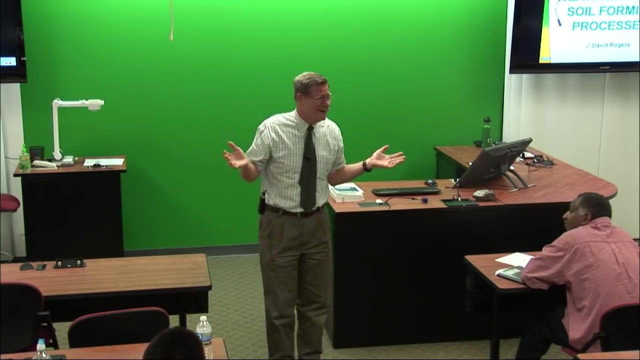 of heterogeneity. that's college talk, for things are way more messed up than you were ever led to believe in school. in school, we do everything hunky-dory simply dimply. that's because we got people teaching foundation engineering who've never built foundations. maybe I. 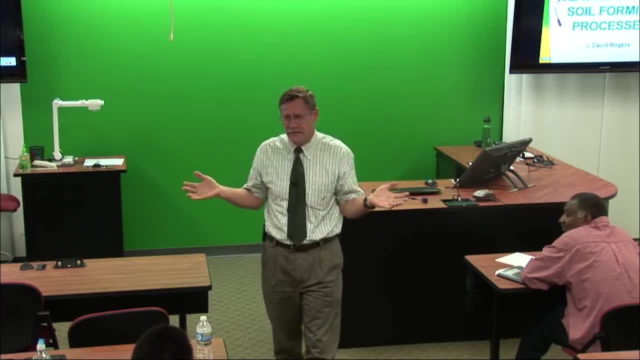 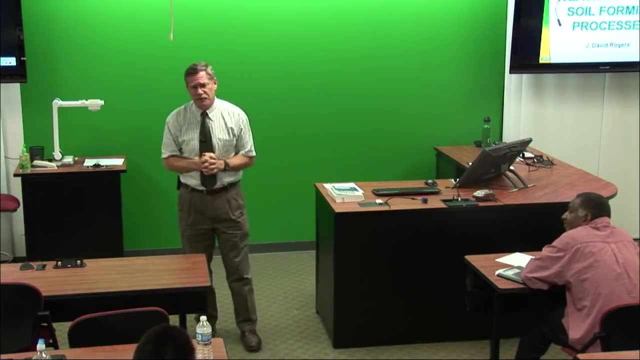 go into West Point taking a class in artillery from some clown has never fired a cannon, but that's the system we have. so I'm gonna give you a real world stuff. I'm gonna show you a real world stuff. there's a high degree of heterogeneity and you need to be designing things to account for that. 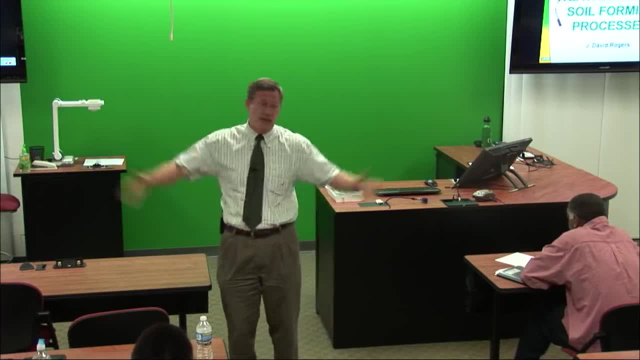 heterogeneity. so when you hit something you didn't expect, you don't have to change the design of the building and cause a bunch of claims, extra lawsuits and all this kind of stuff, because that's what will happen, you know. the poop will hit the fan and your client will not be happy with you. so 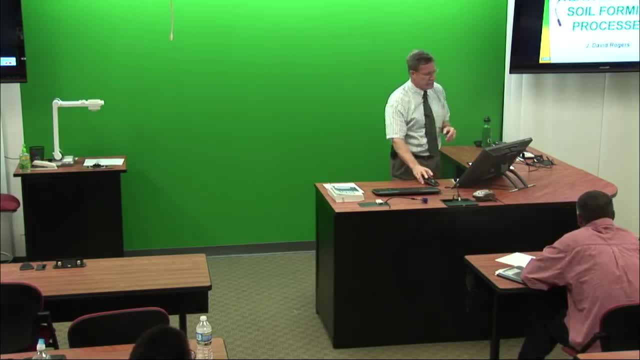 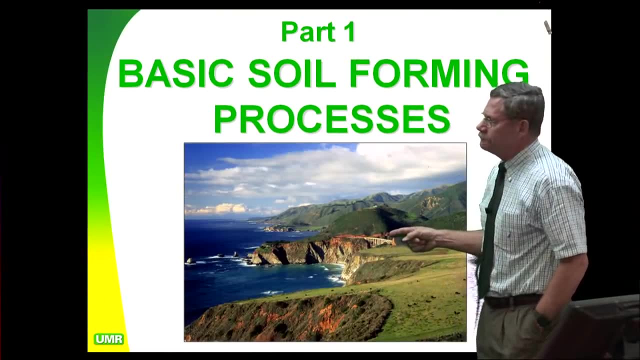 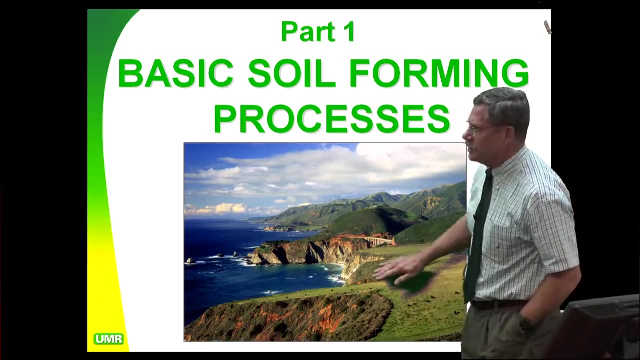 we're going to start here with rock weathering, soil forming processes, and I'm gonna start right here by showing you. this is a Bixby Creek bridge on California. route 1 is a sloping erosional surface here And that surface is an erosional surface from when? 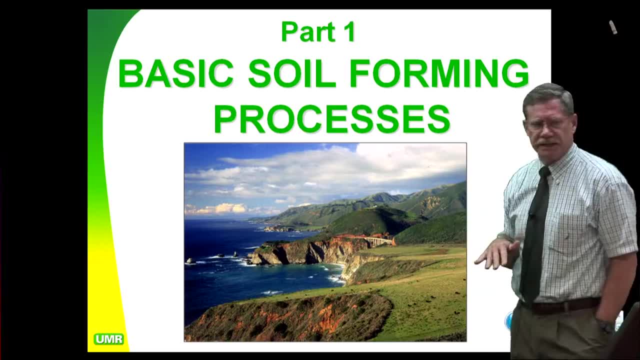 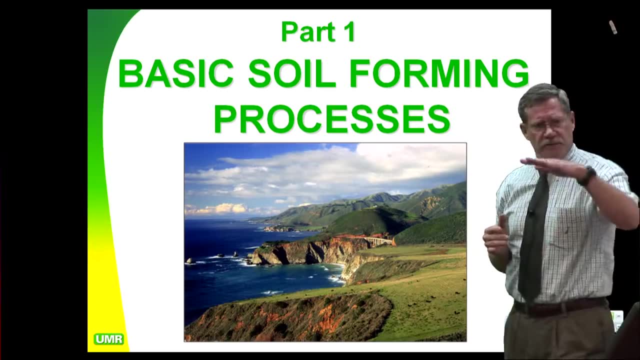 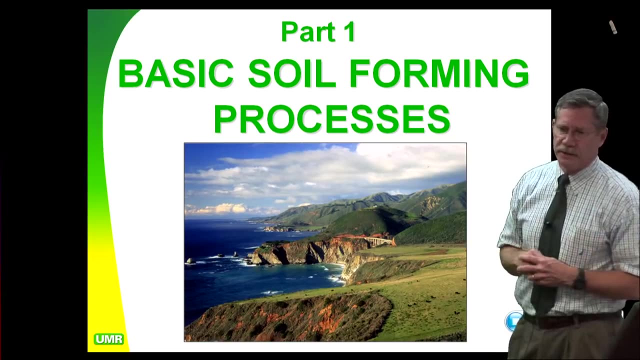 sea level was 360 feet lower than it is today. Now off the California coast- very dynamic coastlines and active tectonic margin- sea level was 360 feet lower than it is today for 90 percent of the last 1.6 million years, So 90 percent of the time sea level was out. 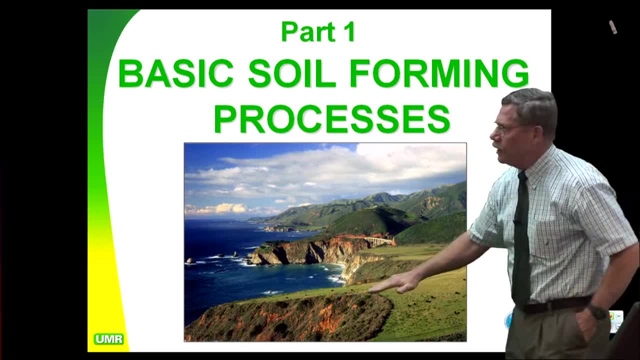 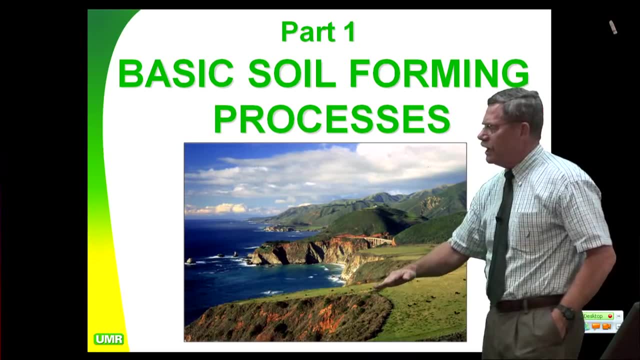 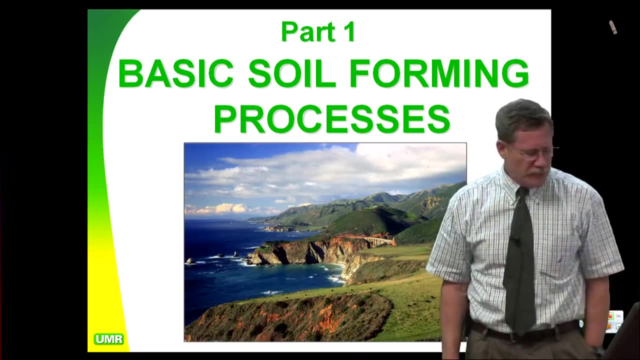 there much lower, and you have these very well-developed erosion surfaces. They're very, very planar. And this one, if you take the strike, if you take the dip of it and you project it, it goes off shore about five and a half miles And that's about right. And 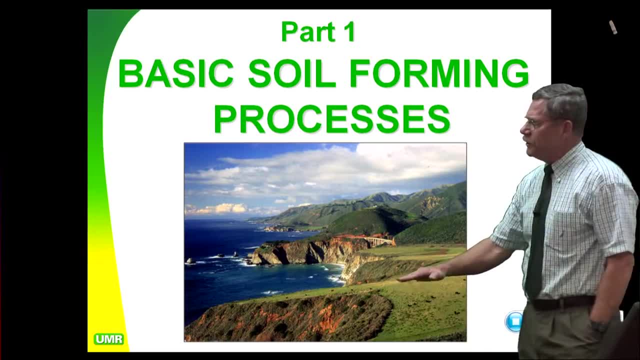 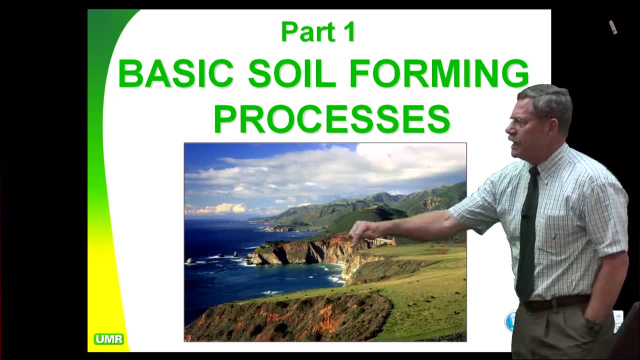 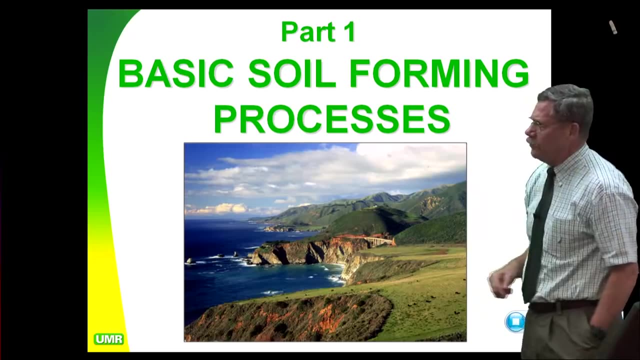 so if we look at that surface, this has been under sub-aerial weathering for a much longer period of time than areas that are like down in here, where it's very, very, very flat, And that's where you actually see a lot more active erosion. So this is California Route. 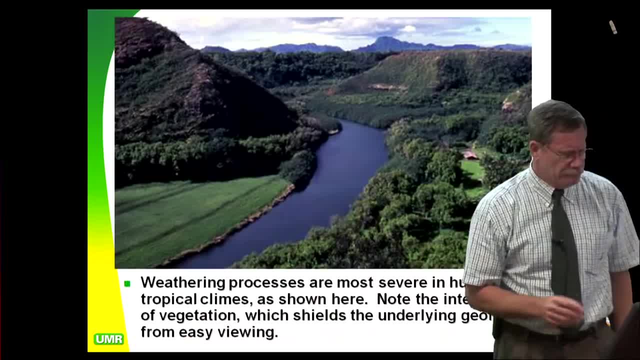 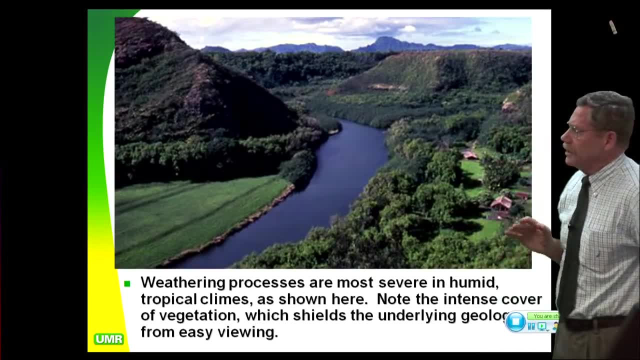 1 north of Big Sur. If we go to some place like Panama. I've done a lot of work in Panama with the canal down there and here we're in a tropical environment and we have very, very active weathering processes. It's very, very humid. It's very, very warm. You're going. 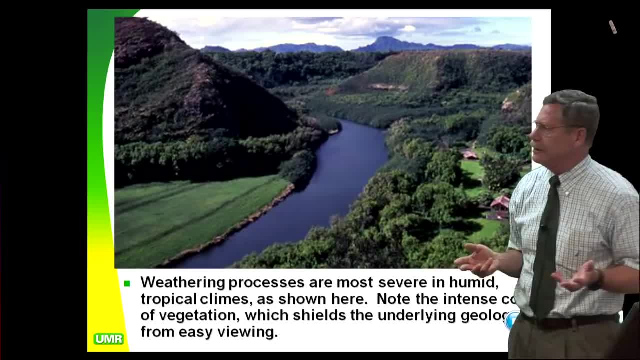 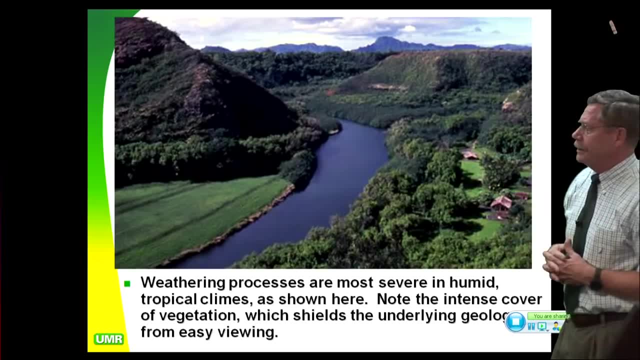 to get more redox reduction reactions here. So that's what we're going to do, And so it's in a shorter amount of time than you're going to get in a temperate climate like we have here in Central Northern America. So here it's very hard to see what's going on with the geology. 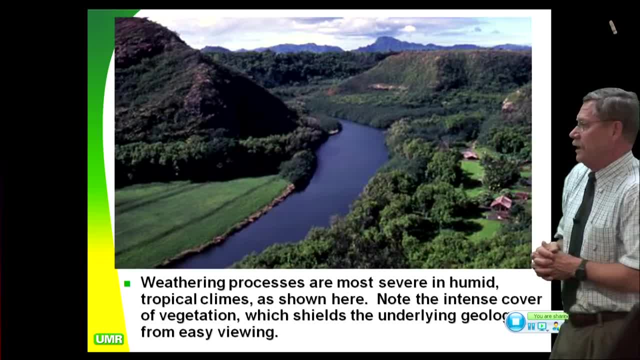 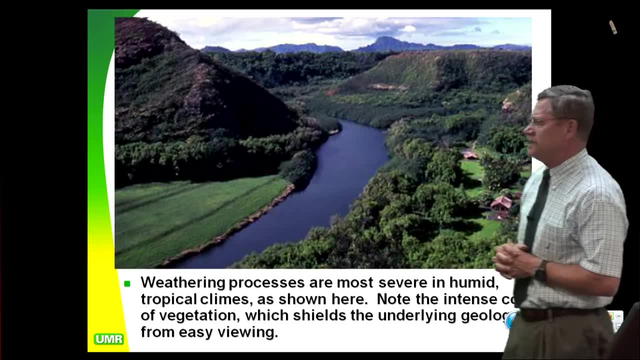 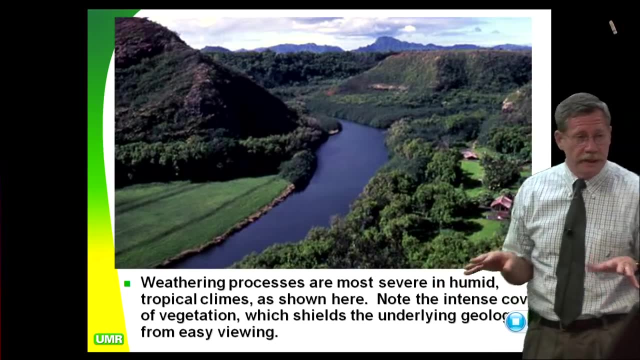 Everything is covered by jungle or water or something else and you have lots of decaying organic matter everywhere and lots and lots of acid that is out there from decaying organic matter dissolving anything that's dissolvable. So it's a completely different environment when you go to the tropics. 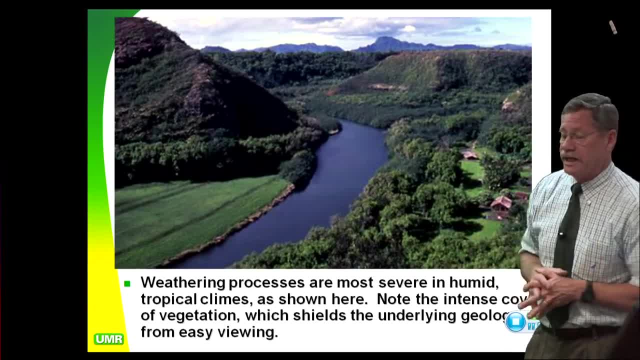 from what you're dealing with with American soil mechanics. I just want to make that clear. So when you go working in the tropics, you forget everything you learned in Missouri and start learning some extra things, because you're going to need the extra things. 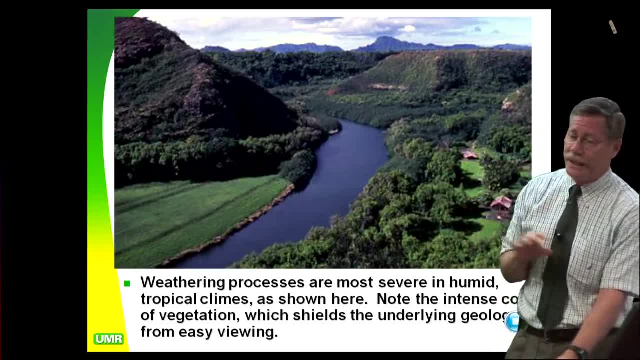 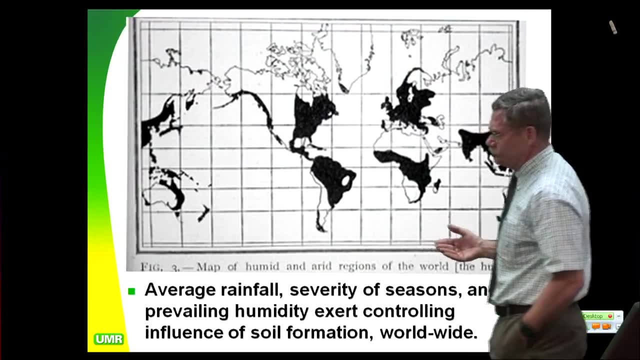 My firm did a lot of work in Taiwan, Panama and Hawaii. We even had an office in Hawaii for a while because we had a lot of consultations there. Now, if we look at the soils around the earth that have formed- and this is from a book that's over 100 years old- 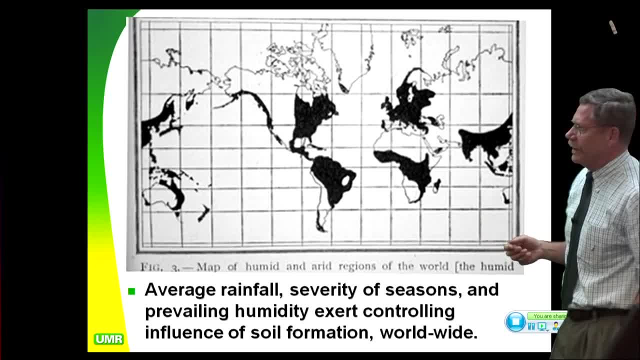 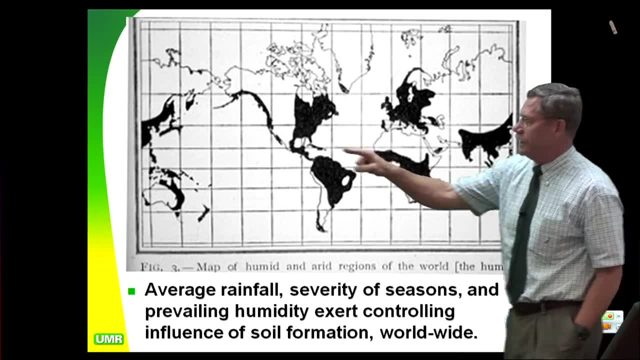 And you look at average rainfall, the severity of the seasons, the prevailing humidity, they all exert controlling influence on the soils And the dark areas you see here, the dark areas like here's up in central or eastern United States. these dark areas are humid areas. 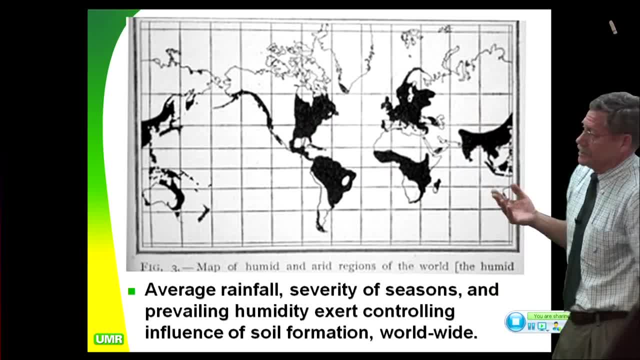 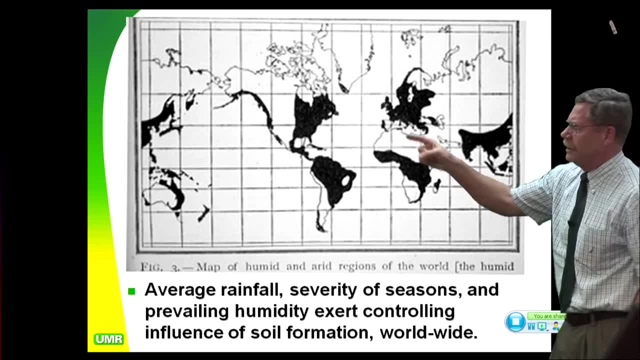 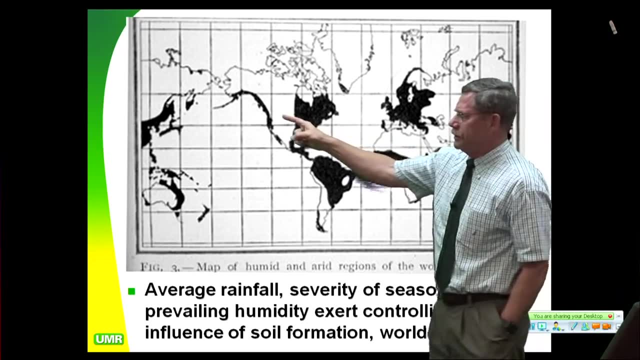 areas that have high humidity, And areas of high humidity or semi-high humidity have completely different soils from areas that are more arid and semi-arid, like the Sahara, The Gobi Desert and places like that, And so western United States. you'll notice completely different west of what? 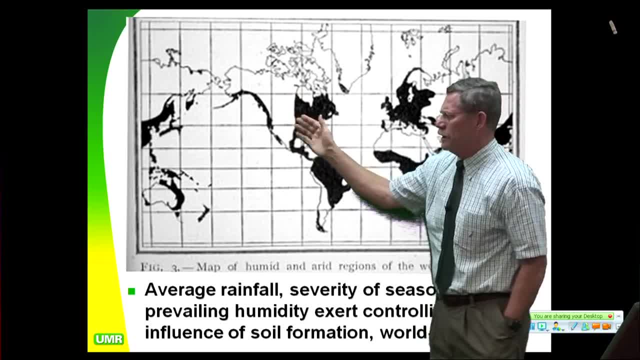 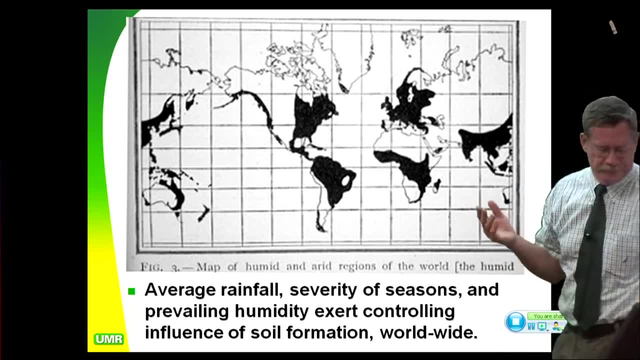 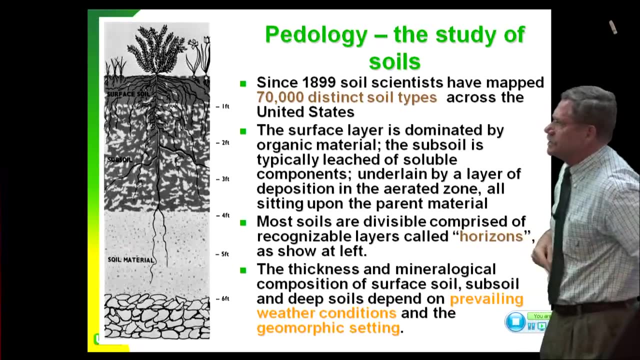 The 100th Meridian, You go west of the 100th Meridian, you have calc-alkali soils. You have lots and lots of calcium and carbonate, just carbonate, calcium carbonate. All right. So podology is soil science, the study of soils. 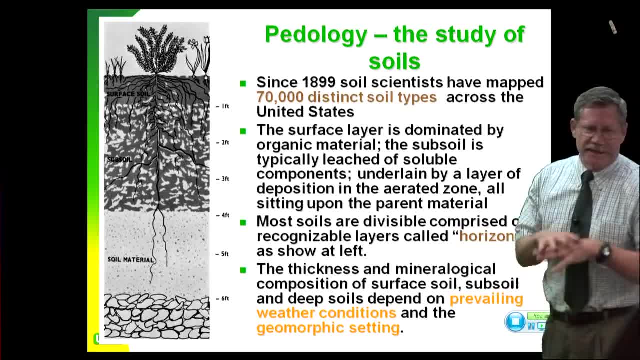 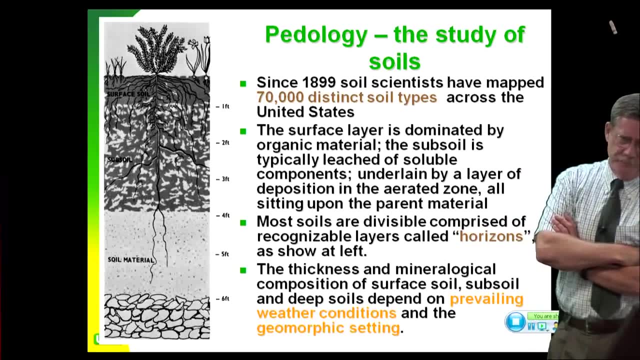 And since 1899.. Soil scientists have mapped about 70,000 different kinds of soils across the United States alone, not to mention the whole world. And this was all driven by agriculture. And they're mapping the upper four feet. They're not going down very deep because that's what the crops grow in. 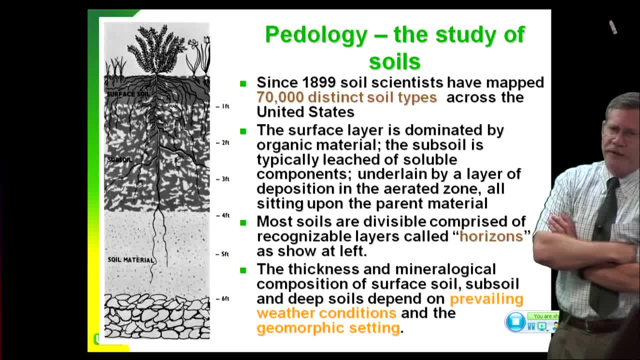 The crops and the orchards grow in the upper four feet, So 1.3 meters, not very deep. The surficial layer is usually dominated by organic material- We sometimes colloquially call that the topsoil- And it's typically leached of soluble components. 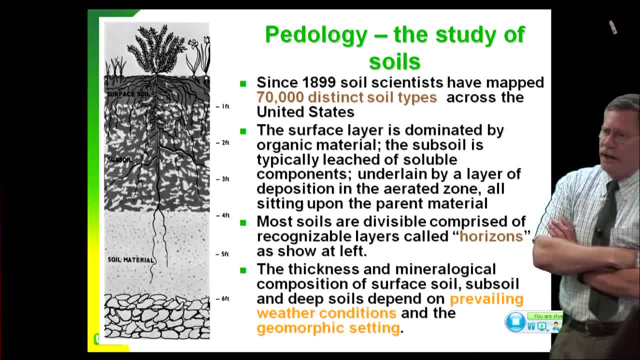 Anything that's easily soluble is generally gone, unless you're in those dry areas where you have less than 20 inches of rainfall a year. That's kind of the magic number 20.. Here in Rolla we're at 38.. 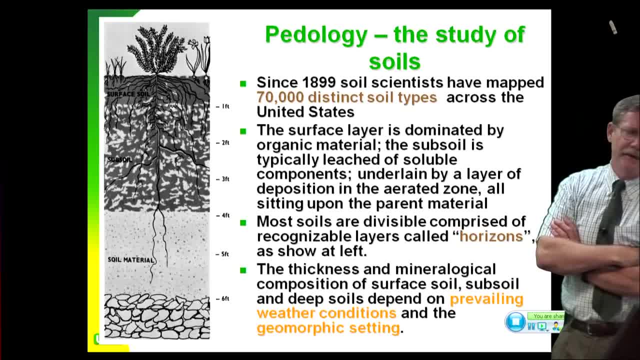 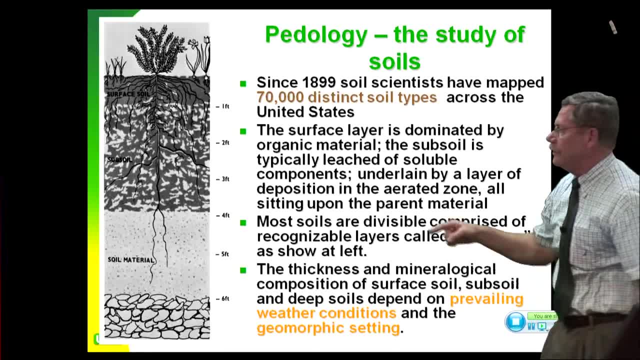 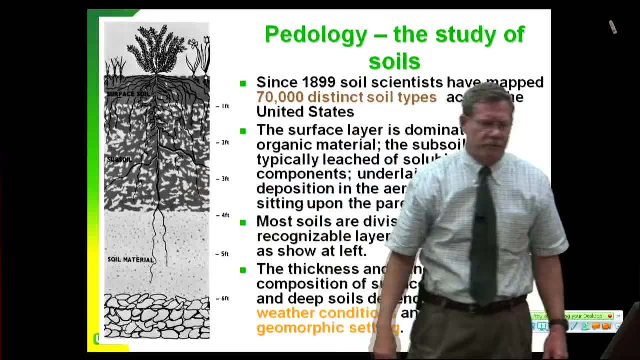 That's the average iso height, average rainfall here. Underneath that zone is a layer of deposition which we call the aerated zone. So that'd be right here. This is the aerated zone. Sometimes we refer to it as the argillic B horizon because it has argillite. 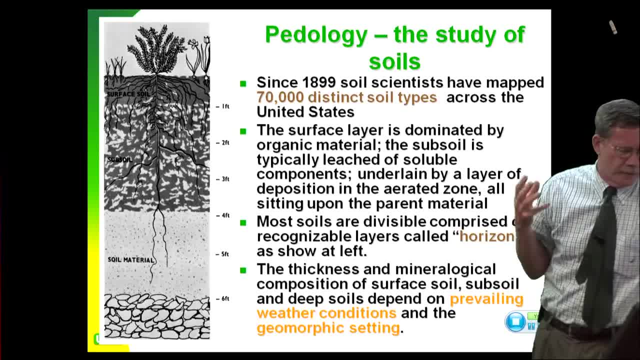 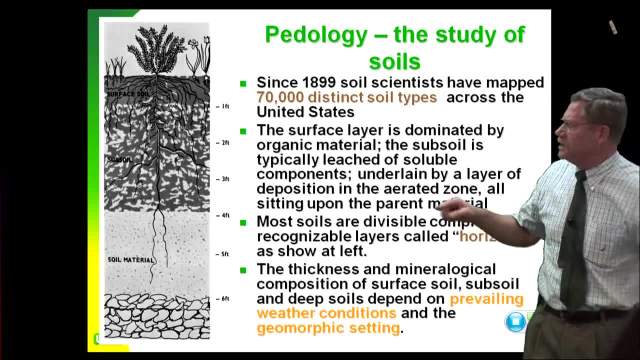 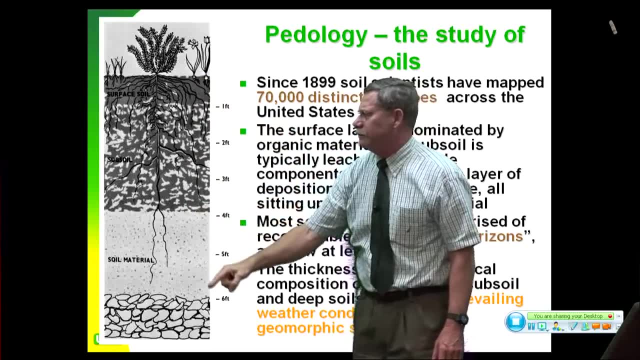 It has clay formation, clay starting to form. We call it the subsoil in classics podology, And we call these divisions horizons. So we have A horizon up here- This is the B horizon, And then down here we actually have a C horizon. 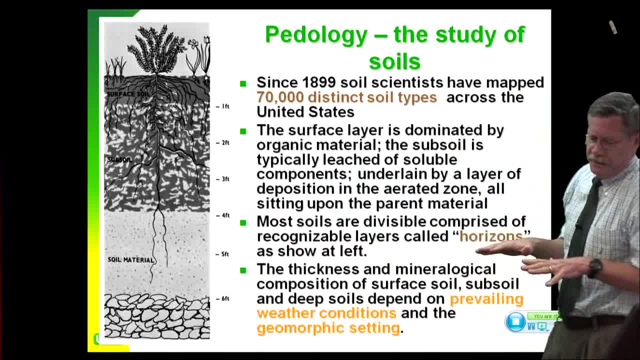 And that's the weathered in place zone, The weathered in place material, the weathered soil, rock, bedrock. The thickness of all these depends on the prevailing weather conditions and the geomorphic setting. Geomorphic setting- what's that, the big word for? 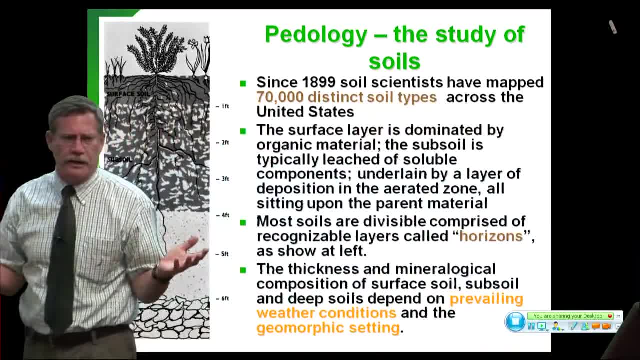 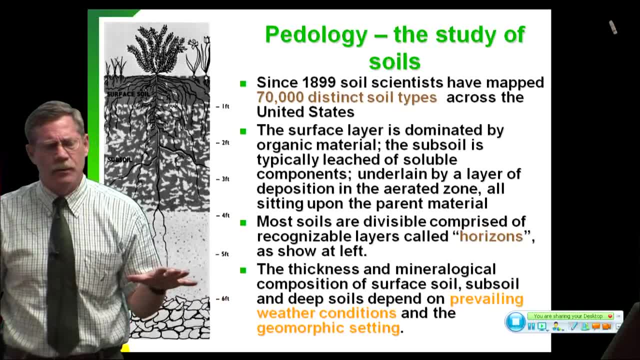 Geomorphic setting is the big picture, view the geography. Are you down in a floodplain? If you're down here in the Missouri River floodplain, that's a whole different game, groundwater-wise, from being on the lust-covered elevated uplands. They're going to be different. 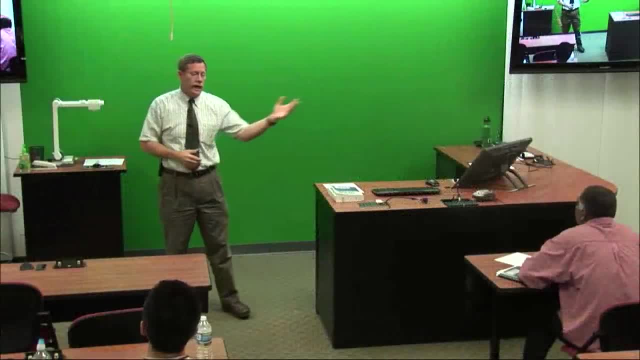 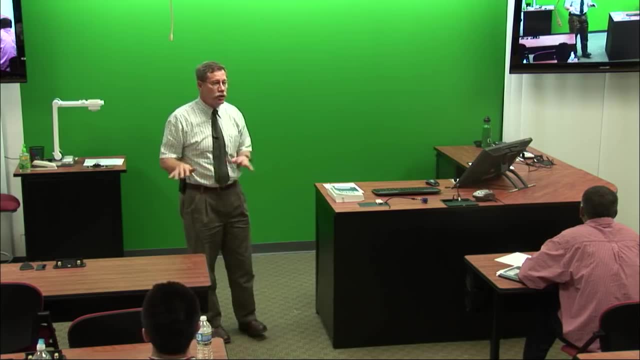 They're going to be much drier, much more prone to self-drainage. You get out there on the floodplain, you don't have to drill very far to hit water and you have very low bearing capacity, very soft, youthful soils. 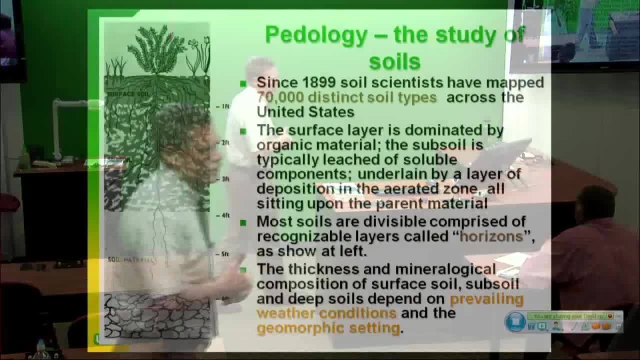 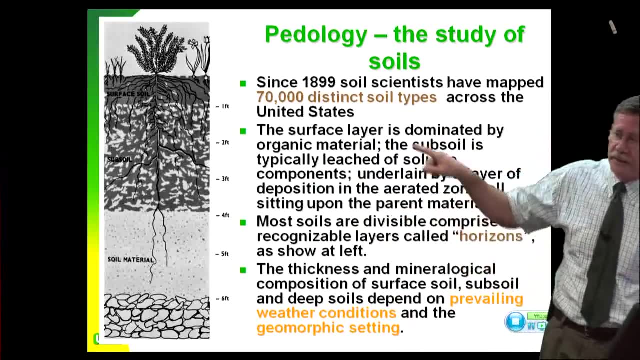 They just got put there 15, 20 years ago, In our case 1993 flood. It's the last big flood around here. Most of the floodplains around here, even Big Piney Creek, are all 1993 floodplains. 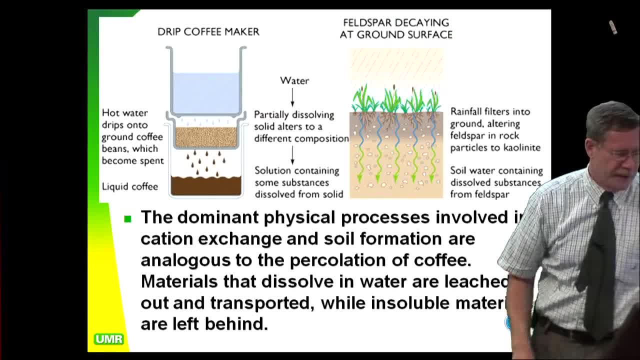 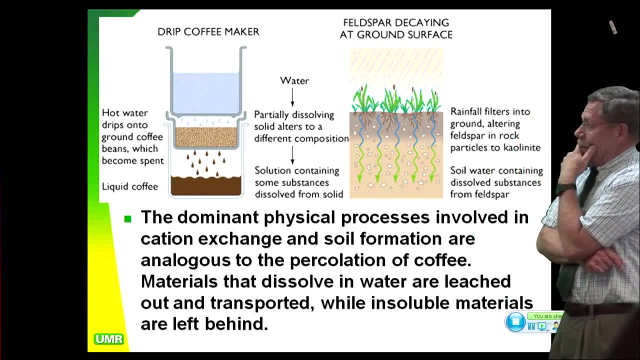 They date from the big year. We had a lot of flooding that year. Now, I like this analogy. This comes out of a physical geology text I used to use at Berkeley. At Berkeley we make all the civil engineers take an engineering geology course. 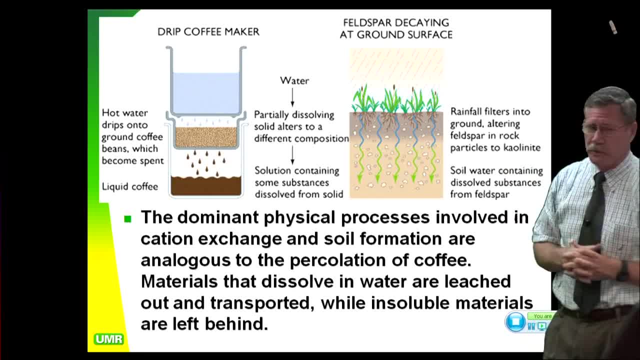 They say: well, how can you fit that in the curriculum? They keep bringing the curriculum down. Well, Berkeley's ranked number one in civil. So what they do? they took a four-unit course, dropped it to three and then dropped it to two. 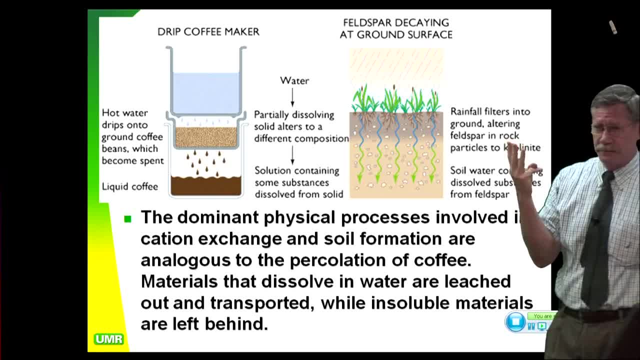 Two units, three hours lecture, three hours lab. You don't like that? Go to MS&T, Go to Columbia, Go somewhere else. They can get away with it there. Hardest class we had in the undergraduate click room there was AutoCAD. 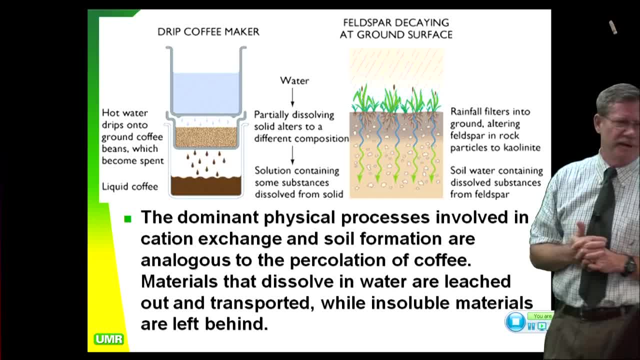 AutoCAD. I think we gave them half a unit and it was about six units of work, depending on how good you are at that kind of stuff. But this is a good analogy. I like good pictures because pictures are how we teach and pictures are how we remember things. 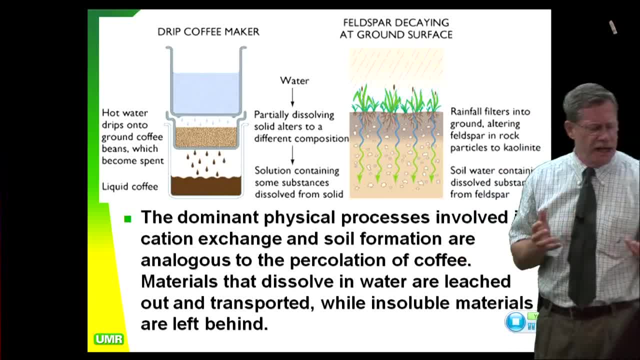 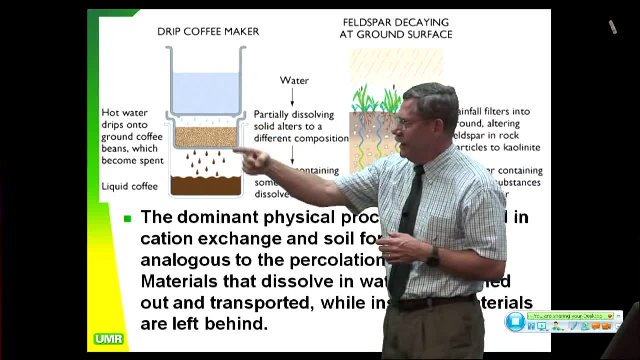 And so, if you look at this, it's saying here that soil formation is akin to what? To a drip coffee maker. Yeah, This is just what's going on in a landfill too. In a landfill, we call this leachate. 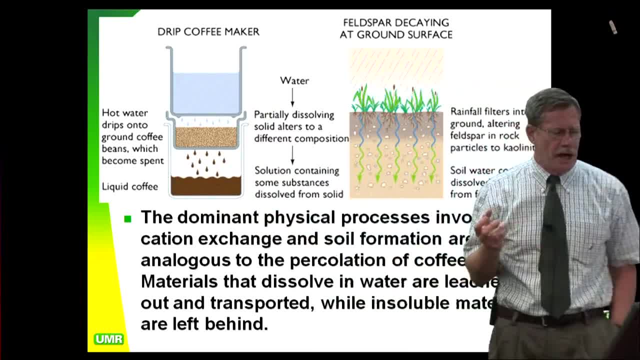 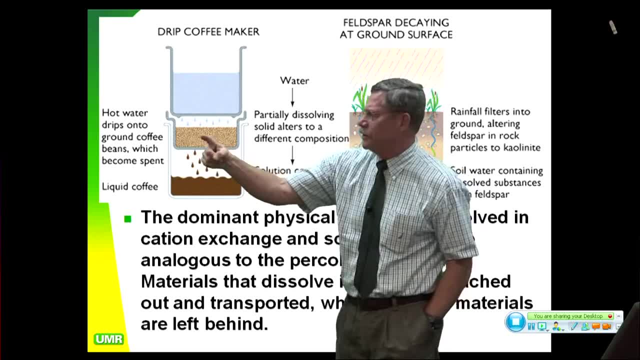 Here we call it liquid coffee, But same kind of thing. What's going on there is we're dropping water through a system And as we drop water through a system, the soluble components, depending on their coefficients of solubility, are going to be picked up and brought down. 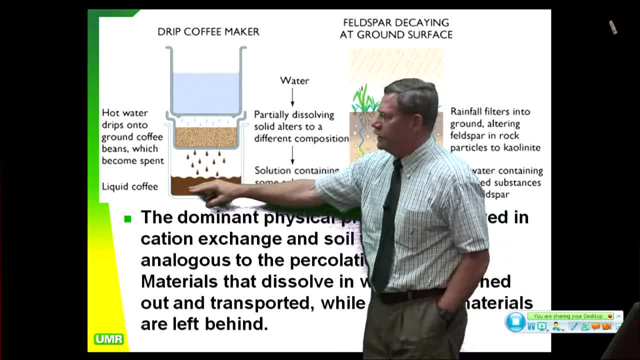 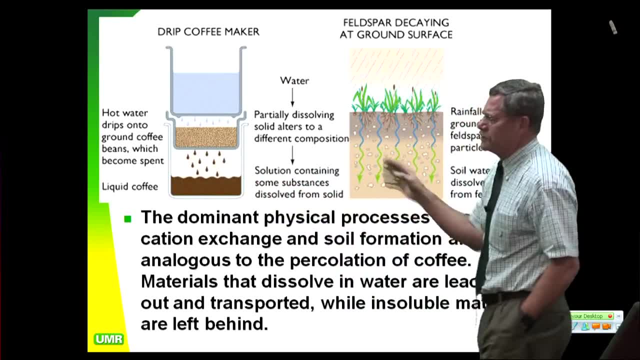 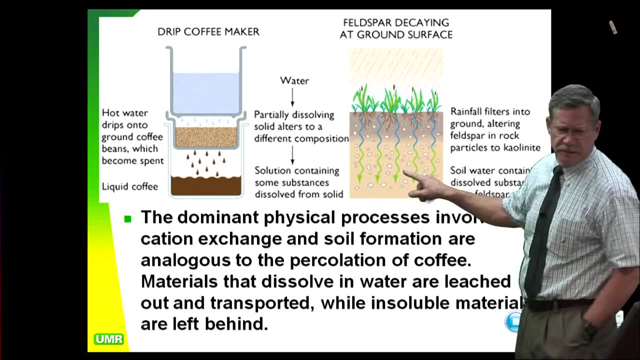 And so, as those things are picked up and brought down here, you have a solute down here that has other constituents in it. All the free cations are going to get pulled out of here and dragged down, And in the long run that's why you see things here like dissolved materials are all gone and leached out. And then you'll see. these nodules of carbonate are very common, which we call caliche out in the West, And of course it's a big problem in agriculture Because as we get this progressive drying out, that's occurred over the last 11,000 years. 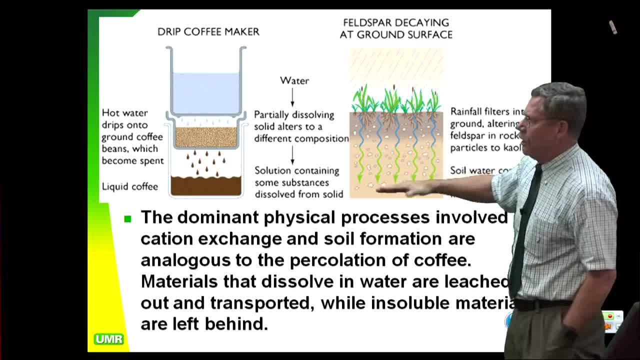 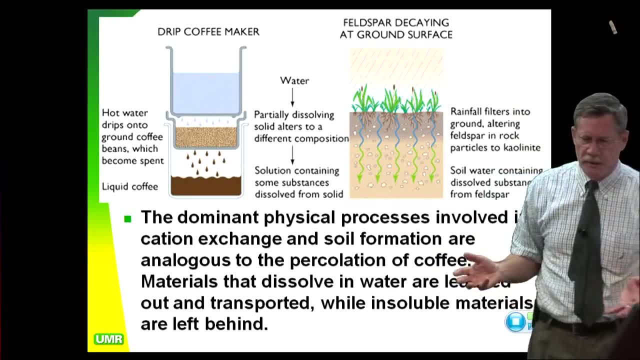 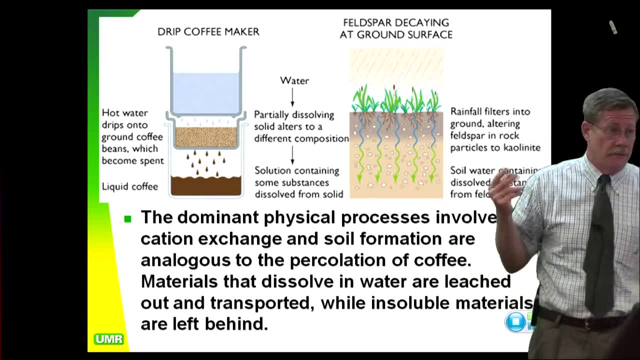 especially the last 7,000 years in North America. we get a hard pan layer down here, a hard pan of caliche, And if you don't break through that hard pan, the irrigation you do gets hung up on top of it and ends up causing fungus and rot of your roots. 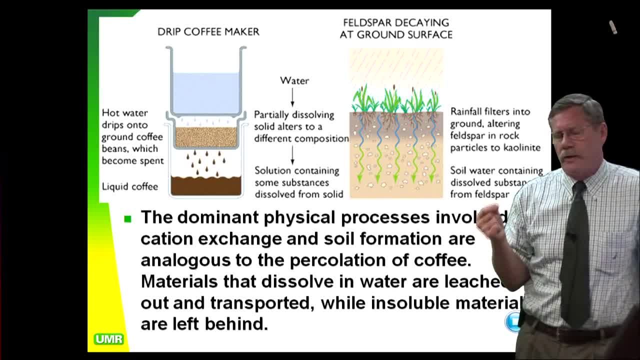 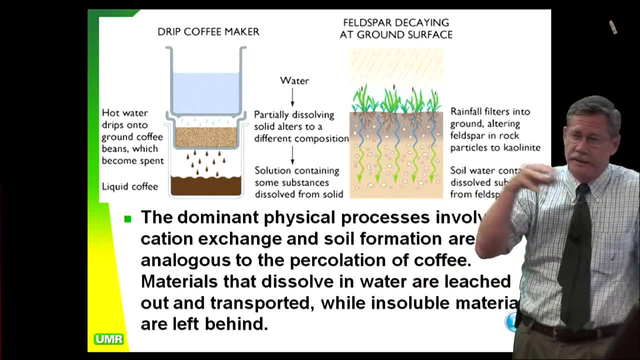 And so what they had to do to be able to ranch a lot of these areas west of the 100th meridian was develop giant plows, like on the Imperial Valley in southeastern California. It's in the delta of the Colorado River. They had steel plows eight feet high. 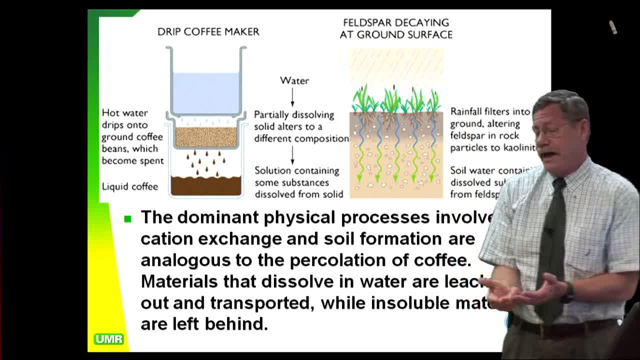 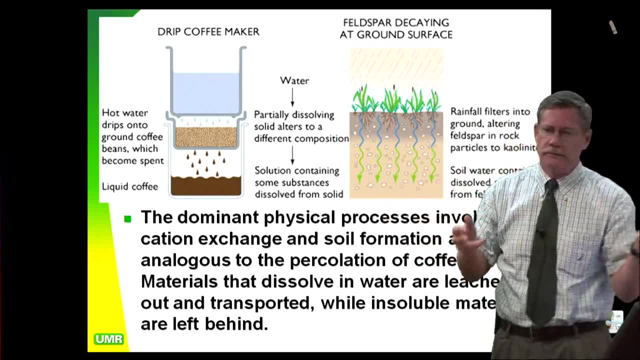 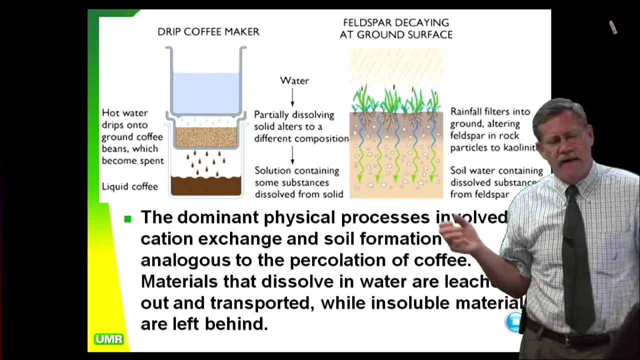 They dig down and pull up and break through that hard pan and turn it over. And then what they do? they flush the carbonate salts out. So for every gallon of water that the plant gets, they have to push three gallons just to wash the salts out into the salt and sink. 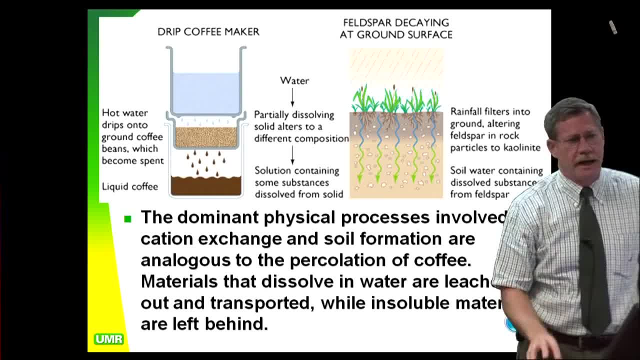 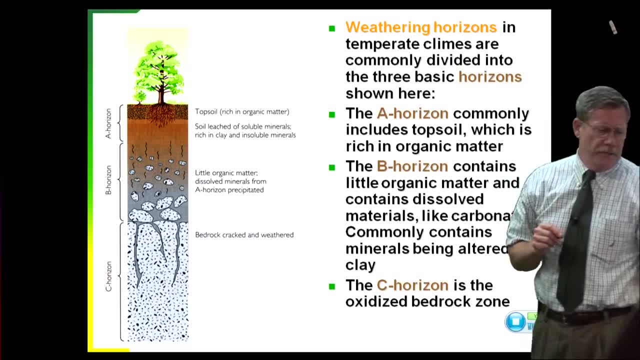 So that's a problem with doing agriculture in dry areas. You have to have an excess of water. It's not a real, effective use of the water. Now, weathering horizons in temperate climes are typically divided into three basic horizons. 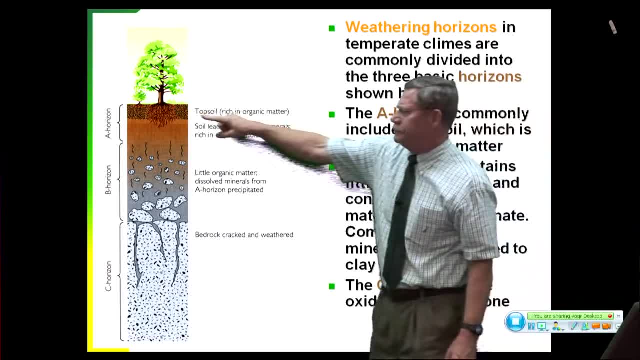 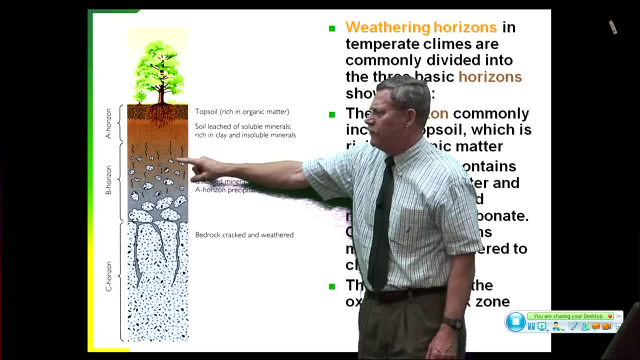 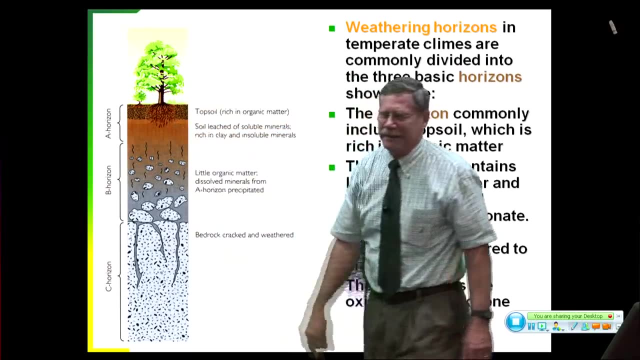 I mentioned previously. You have the A horizon. up here at the top You have the argillic rich- typically rich in clay B horizon. Then you have the weathered bedrock horizon in C. Now this stuff is pretty straightforward. 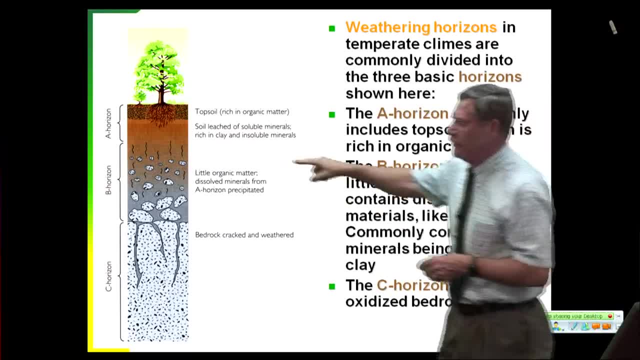 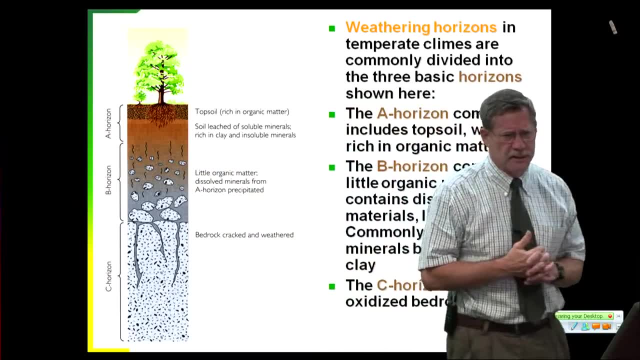 All the problems that occur in practice. kids are with this one. This C one is a pain in the hoo-hoo. Put that in your notes. Rogers says C horizon is a pain in the A-S-S. Why? Because it's so highly variable. 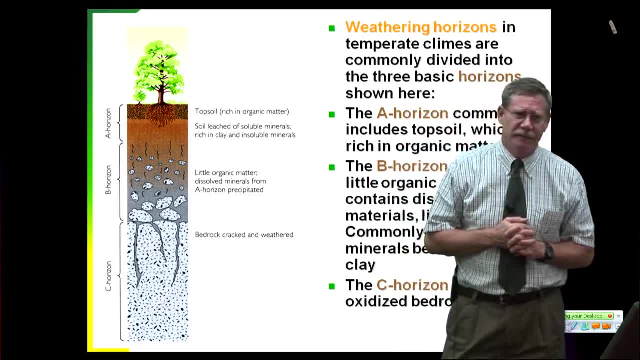 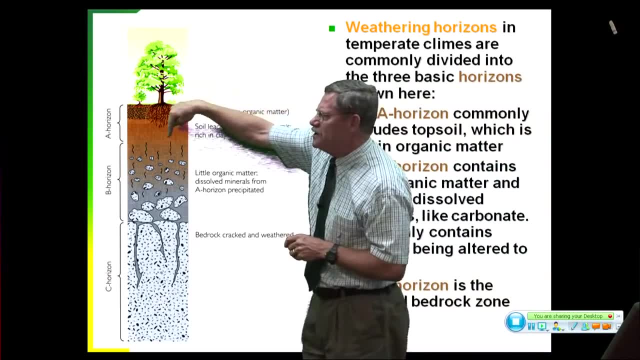 It's worse than going to a dating center or a service trying to find a wife. It is just highly, highly variable. So you're going to come along here and you're going to drill a hole. Oh, this is easy, easy, easy. 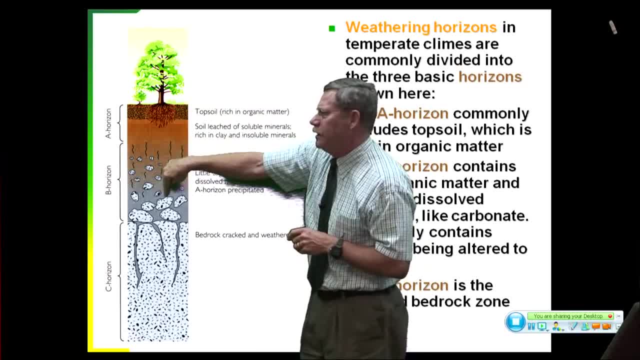 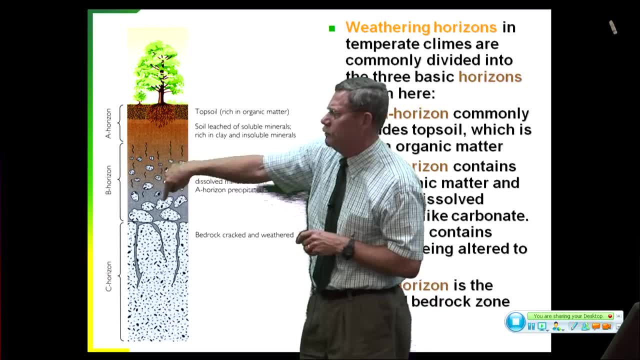 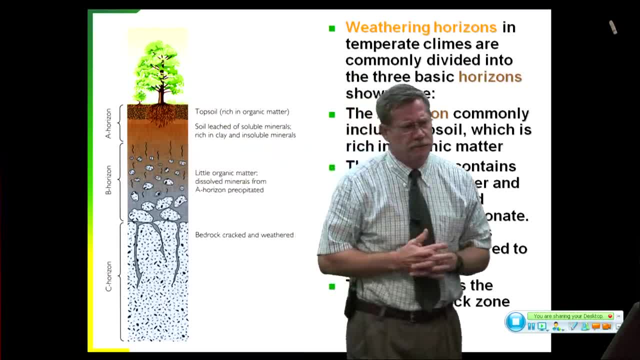 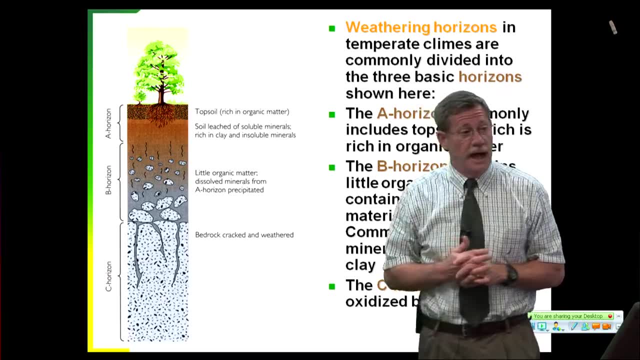 Ah, minus 23 feet 6 inches, You get out there with your subway excavation. You're 10 feet above the bedrock Because you didn't drill far enough. Now, believe it or not, Missouri DOT Department of Transportation. 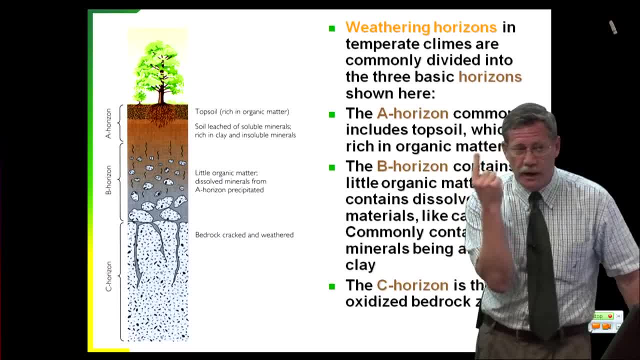 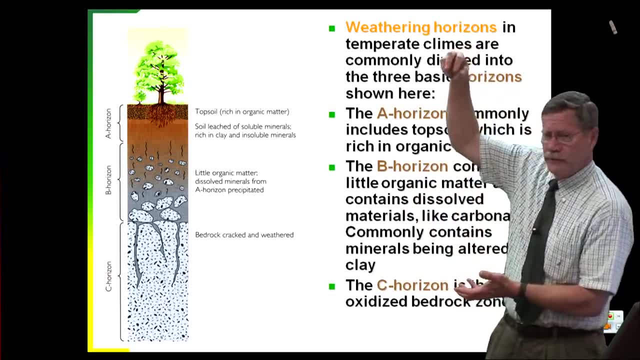 they have a requirement. You cannot call anything in a borehole bedrock unless you core 10 feet into it and you get 10 feet of core out of it. You recover all 10 feet. Then you can call it bedrock, but not until then. 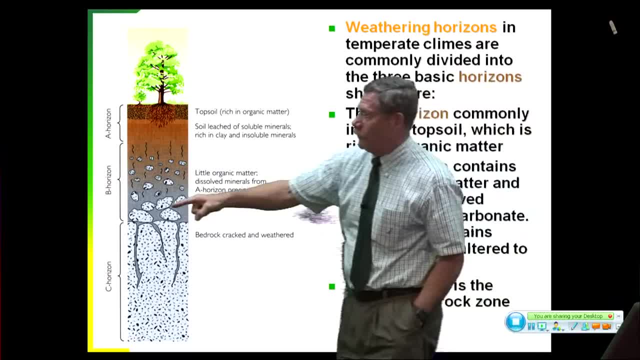 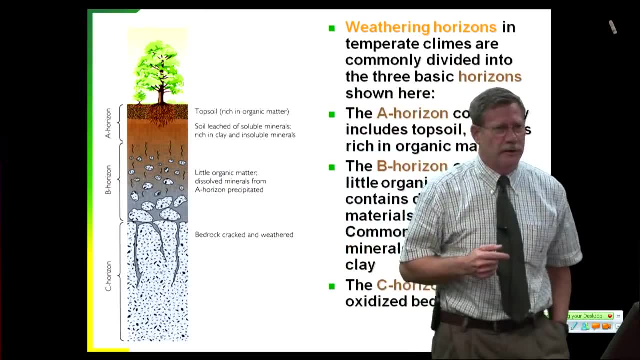 Why do they have that standard? Because this is what Missouri looks like. That's why You've got all these weathered floaters. These are called floaters or knockers. Knockers is not a politically correct term anymore. I guess Hooters took that one out of the dictionary, or something. 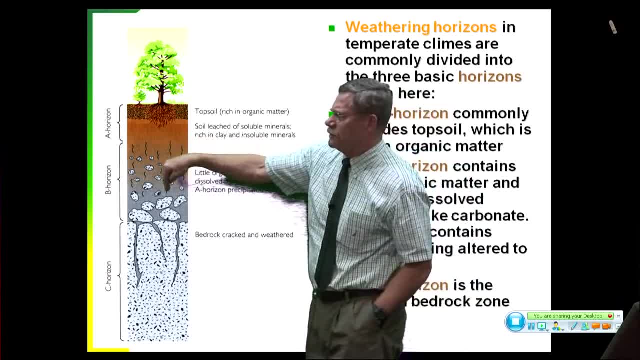 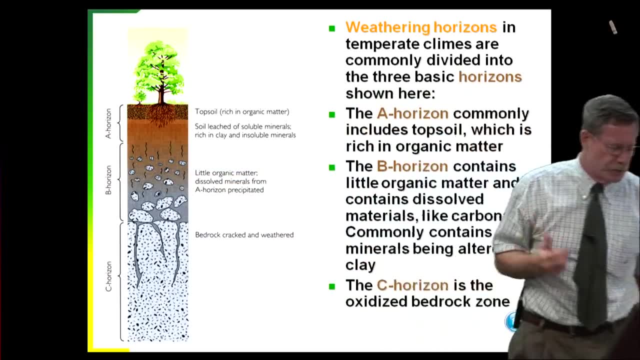 But anyway, these are called knockers. and they call them that because when the drill comes down, if he gets near the edge of them he can actually get stuck in there And they can be a real pain to drill through if you're not just doing diamond coring. 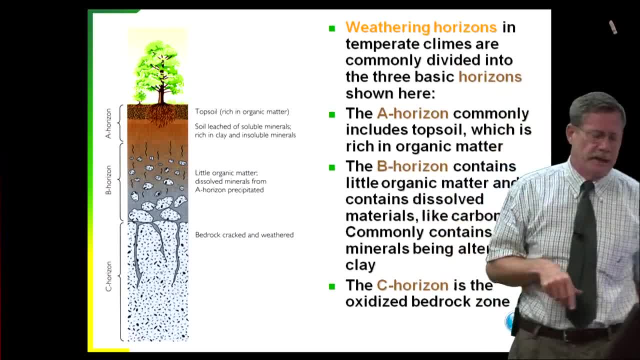 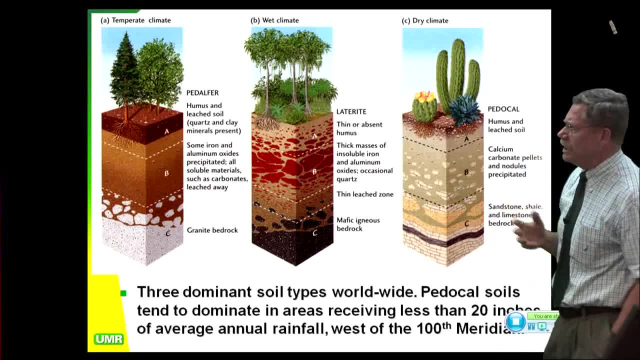 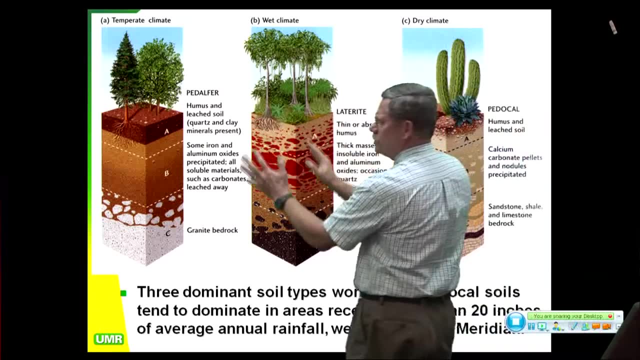 So Missouri, as soon as we hit the rock we diamond core, because there's too many unknowns trying to just auger through it Now. go to another geology textbook and we see the three dominant soil types worldwide. Now these guys got all kinds of cousins and progeny. 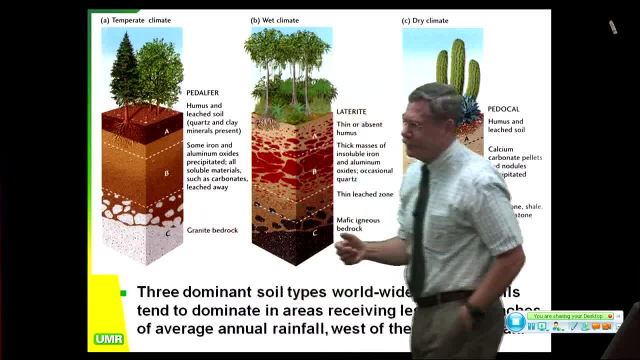 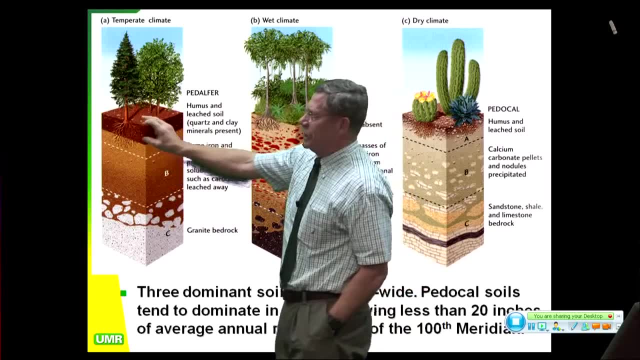 within their respective areas. So if we go out to Washington State, we typically see something like this: a pedulfer soil. That's pretty typical. And what do we see there? We see a real nice organic-rich, humus-rich. 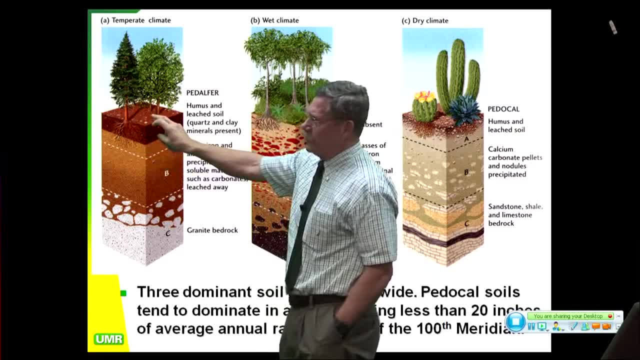 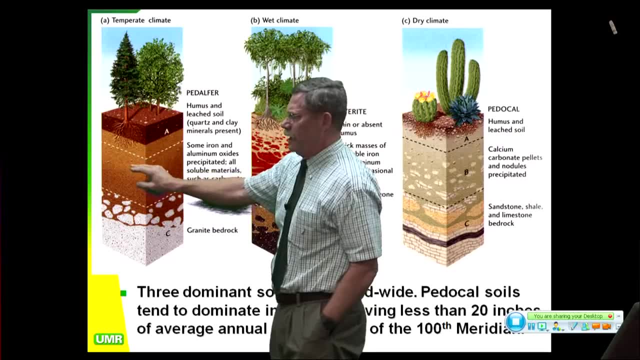 leach, soil litter on the forest floor And then under that we're going to get some iron and aluminum oxides that have precipitated out. You're going to get typically it depends how much the water table fluctuates in here. 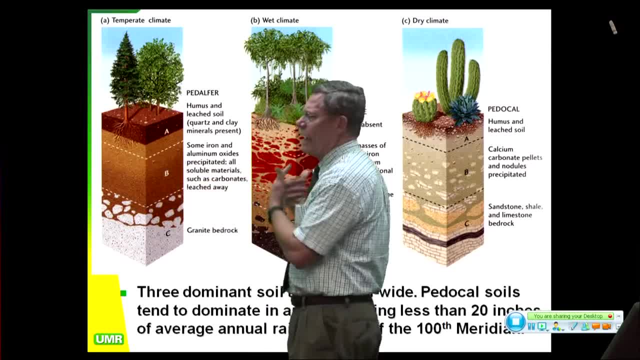 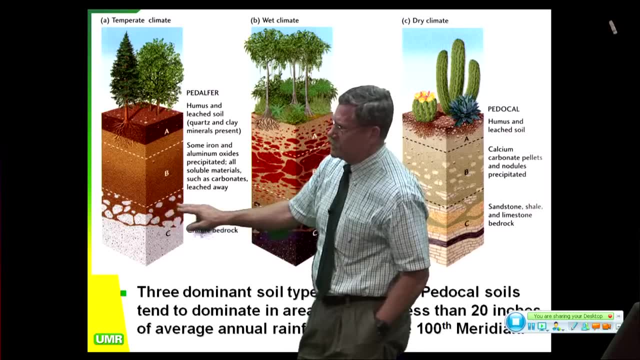 The higher the water table, the more that's going to migrate out of there by leaching, And then you get down here in the sea horizon and this is where all the problems occur. This is where you can actually have soil around the rocks. 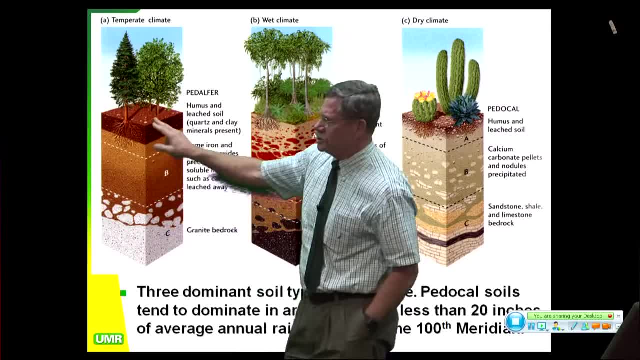 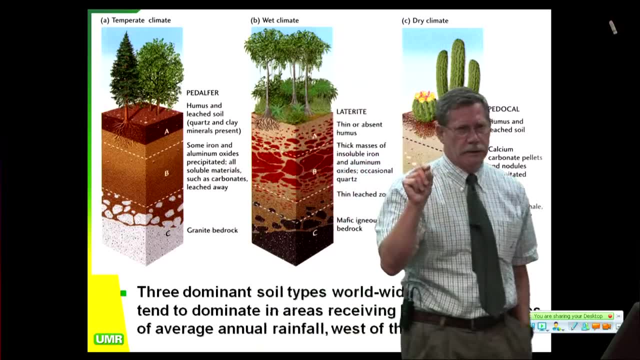 and you can really get fooled down here. So if you're actually showing a boring in this area and you say, oh, I hit bedrock here, you're always going to dash that contact and put a query on it. A query is a question mark. 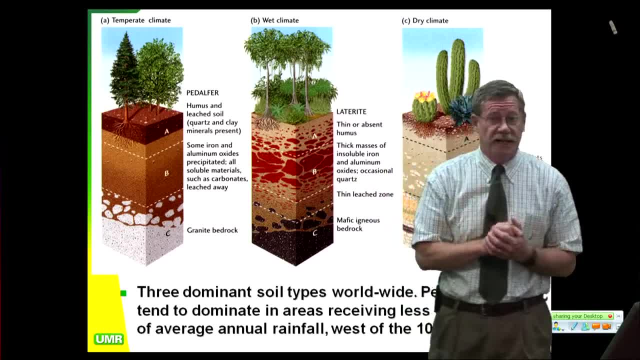 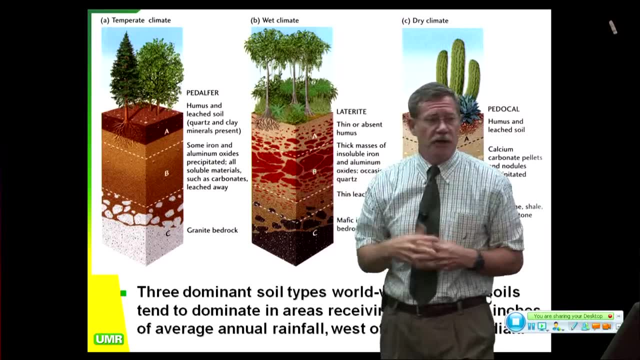 That's called covering yourself, covering your ass. You're covering your ass. You're saying, well, we drilled it and we think the bedrock's in this vicinity and we're going to put some mush language And you're going to get introduced to all kinds of mush language. 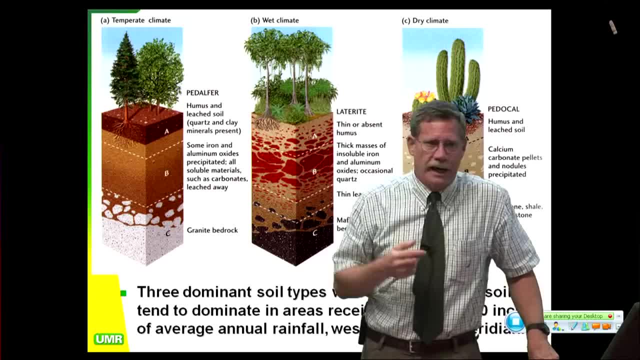 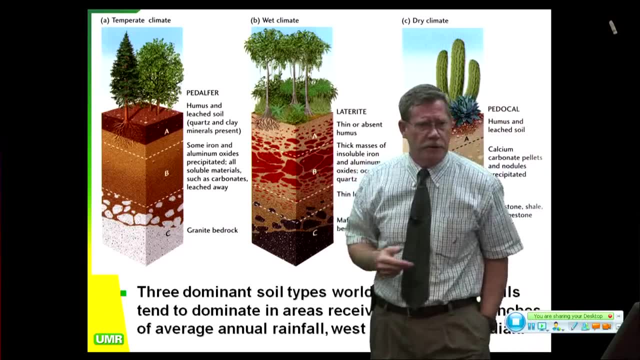 in this course because I was the master of mush language in California and I have that up on my website. It's called Limitation of Liability Clauses. that you're going to put on the paragraphs in your report and say, well, this is how it was the day we drilled it. 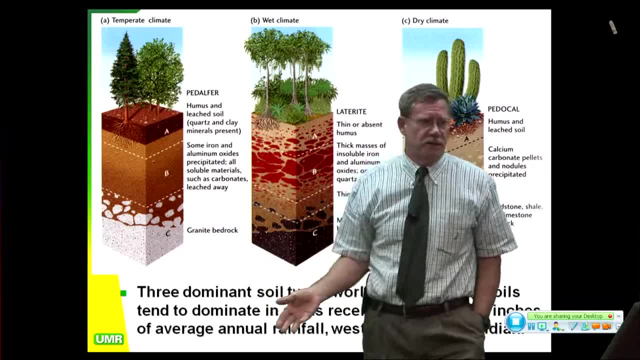 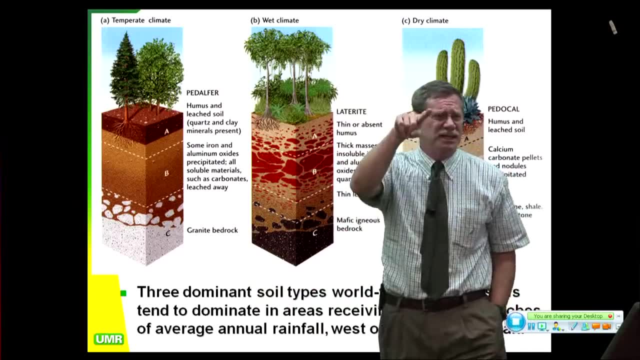 but we drilled it in the dry season. Substantial fluctuations could occur With the passage of time. conditions can change. Groundwater's always a dangerous one. Out here in the Mississippi River, right across the river from St Louis, we watched the groundwater go down 3, 4 meters. 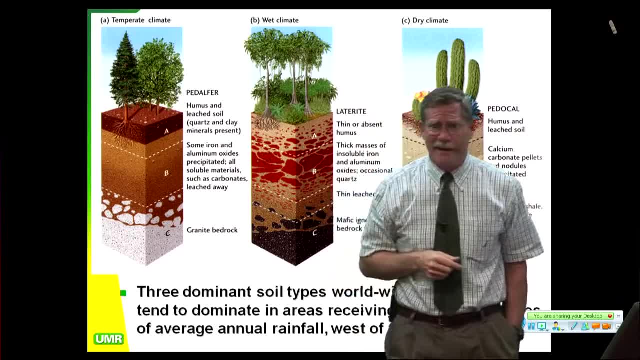 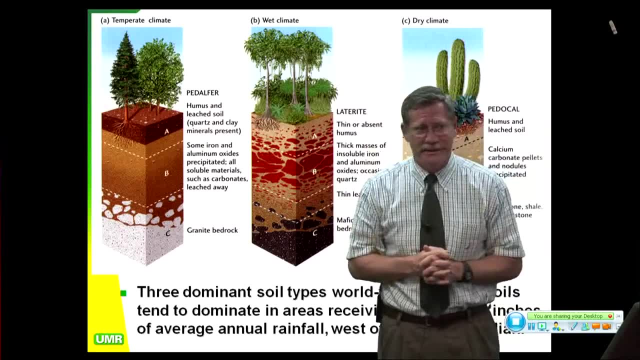 over a period of 5,, 6,, 7 years. That's a lot When you're in a big flood plain like that. you wouldn't think it would change that much. Yeah, they're out there drafting water for industrial use like crazy. 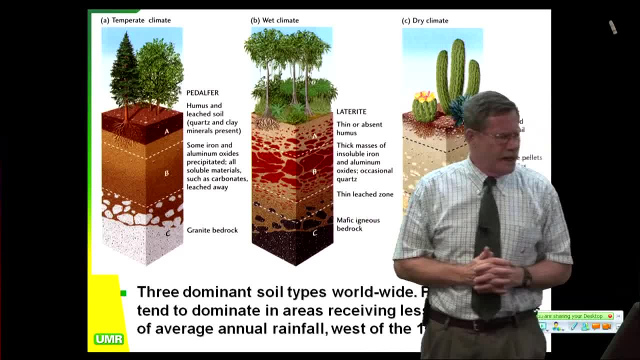 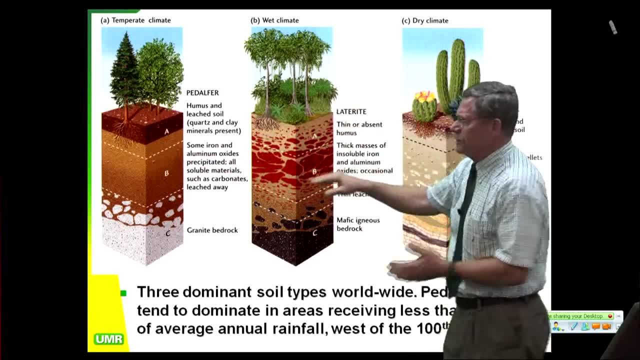 So it doesn't rain for a while, They draw the water table down. Okay, so Pidalfer, pretty straightforward, That's a pretty easy one. Let's skip over here. This is not in the United States, this middle one. 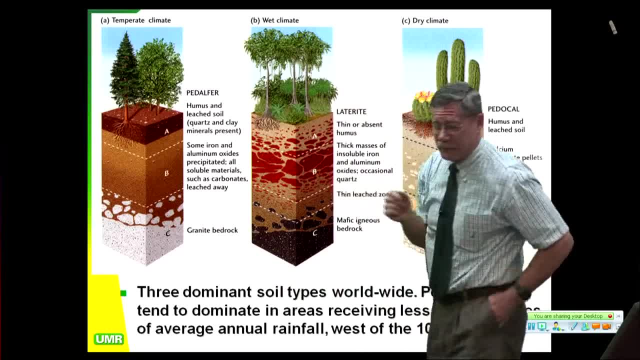 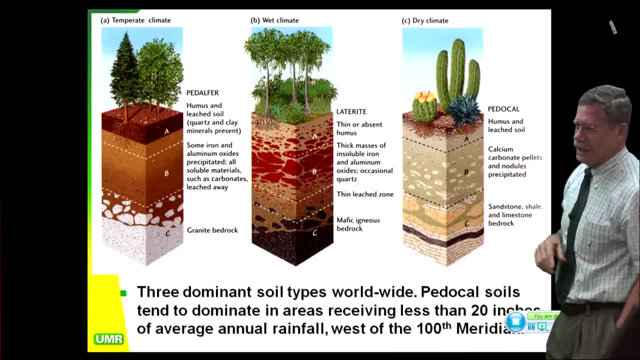 This is exotic stuff. Exotic, and that's more like what we're talking about with Venezuela and Colombia. So we're going to go over here and see the desert? Yeah, so we go to the southwest, and how far do we have to go? 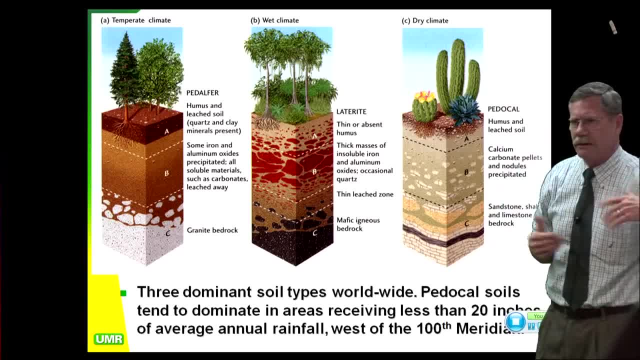 If we drive out Interstate 44,, we go out Interstate 70, we get about halfway across Oklahoma, two-thirds of the way across Oklahoma. just west of Oklahoma City you cross the 100th Meridian, the old Chisholm Trail. 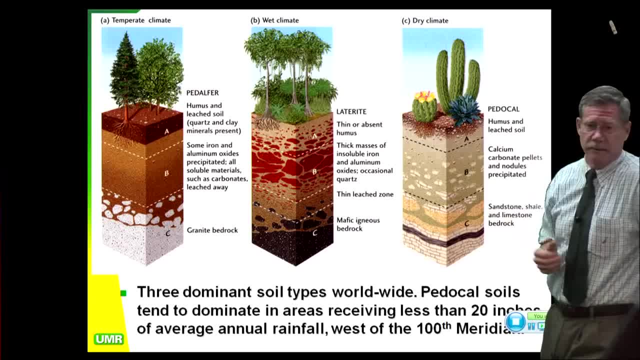 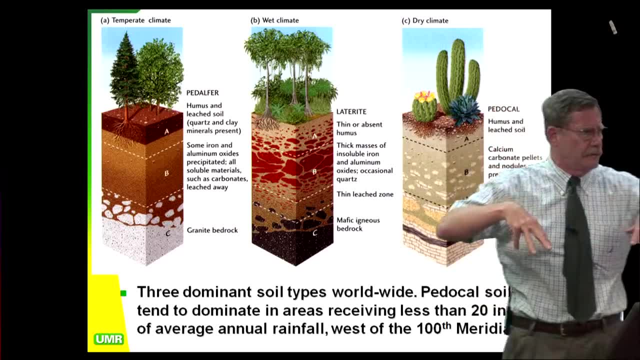 and you're in dry country. You don't see any trees anymore, except the ones that have been planted by man. Things get dry. What's going on there is: you've got less than 20 inches of rainfall a year, so the water that's raining down. 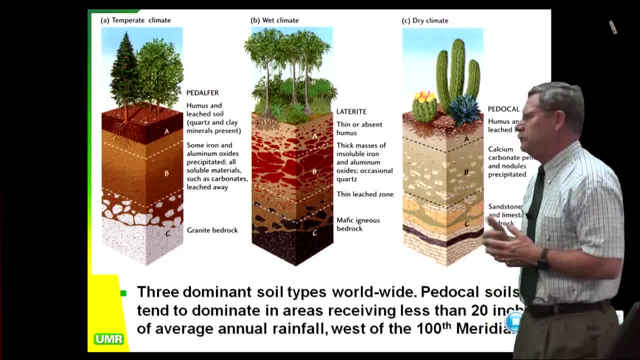 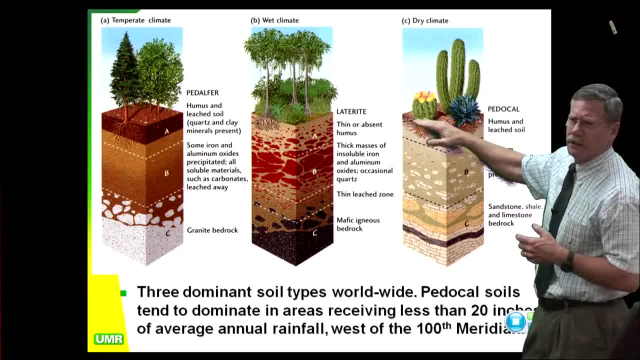 is getting evaporated back out. Now, if I'm out there in western Oklahoma, how much water would I have to have to keep my grass green? We have something called a lysimeter test that does that. We grow grass, fescue grass. 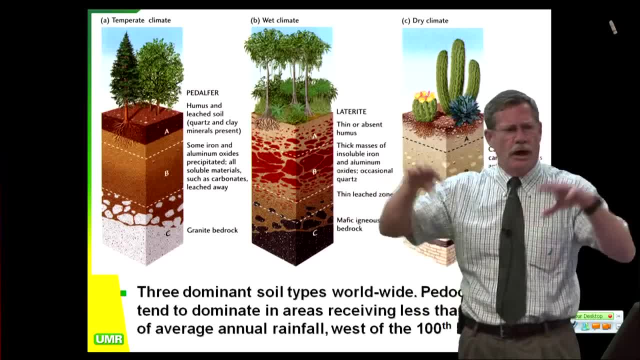 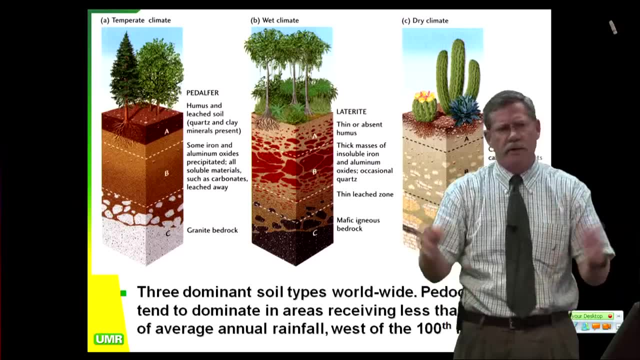 four to six inches high and we just water it and we keep watering it and there's holes in this big, huge table. it's a perforated table and the excess water is able to go out and we measure how much water. 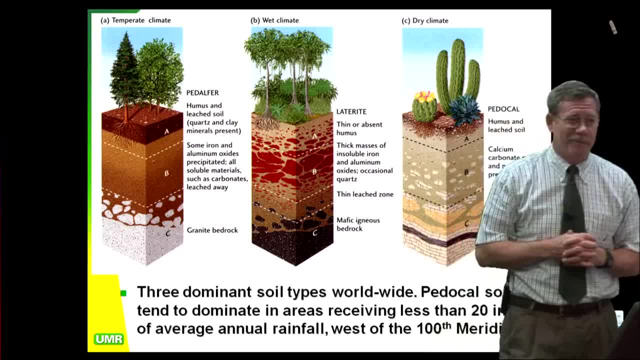 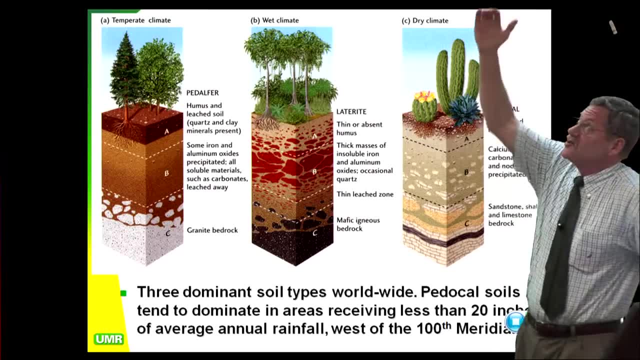 is taken up by the grass to keep it green. You want to guess how many inches to keep your grass green in western Oklahoma? Eighty-four inches. That's higher than Shaquille O'Neal. That's up there, babe. That's a lot of water. 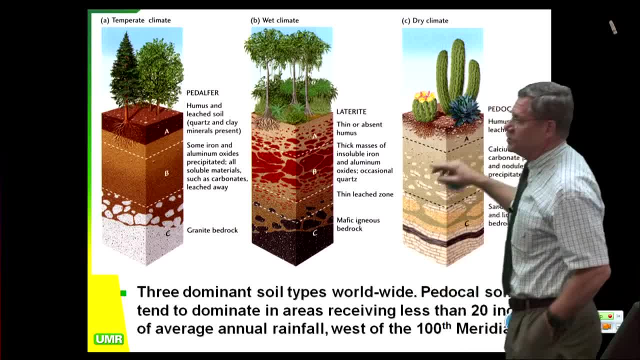 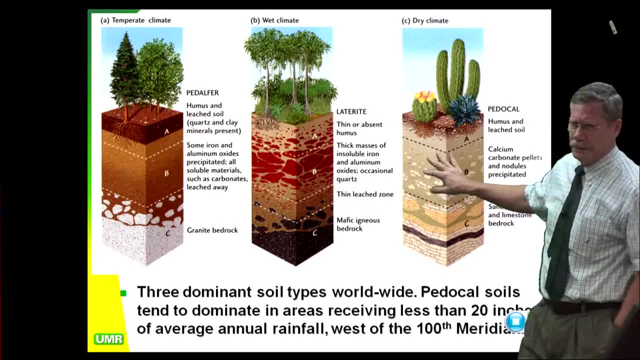 A lot of water. So what happens here is you get all kinds of carbonate nodules, all kinds of exotic. You get sulfates- Sulfates you got to watch out for because they attack concrete and they get underneath concrete. It's a big, huge problem with pavements in Las Vegas. I have, you know, Las Vegas- I'm going out there every couple of months- a lot of exotic problems with soluble salts. They put asphalt in because asphalt's cheap: $4.50,, you know, square foot for a three-inch asphalt overlay. 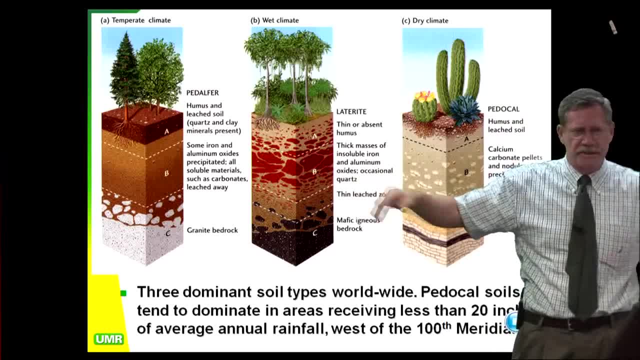 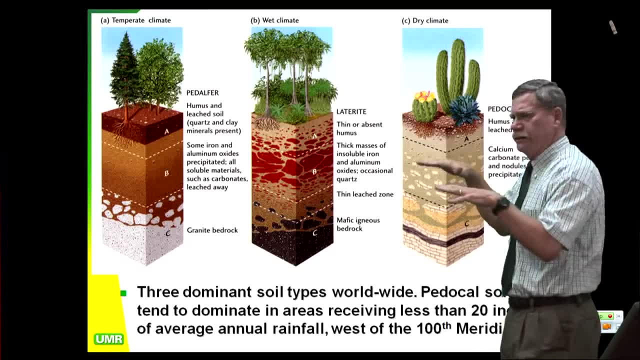 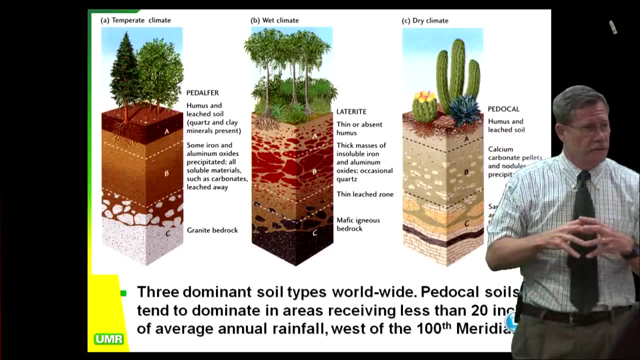 They put asphalt in, put down nice deep curbs on either side and then it heats up to 150 degrees during the day And then at night you get condensation of moisture underneath the pavements and you get etringite sulfates forming and expanding. 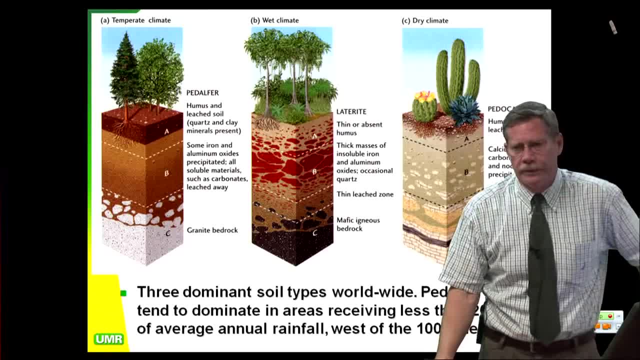 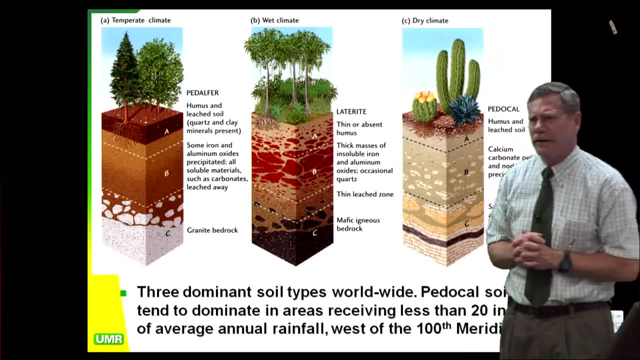 and busting the crap out of everything that's built on them. Just bust the heck out of everything. What kind of uplift pressures? 5,000 PSF- not uncommon at all. So north side of Las Vegas is expansive soils on old Lake Las Vegas. 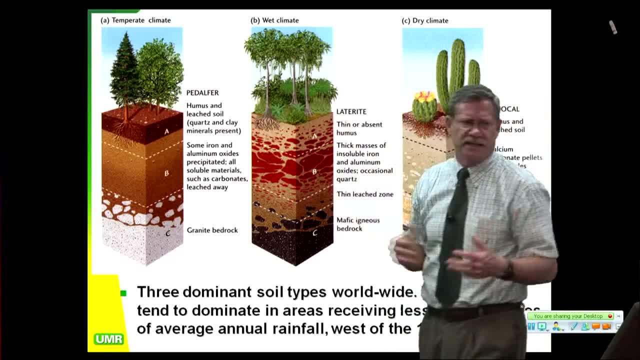 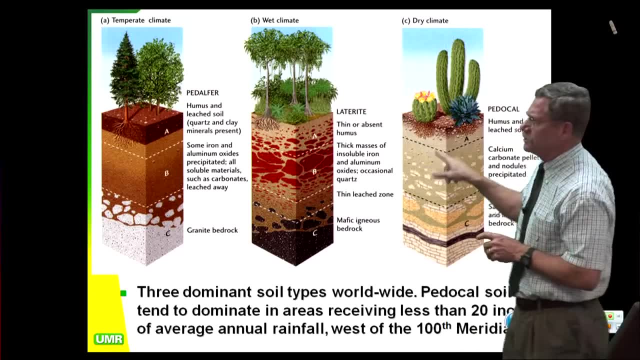 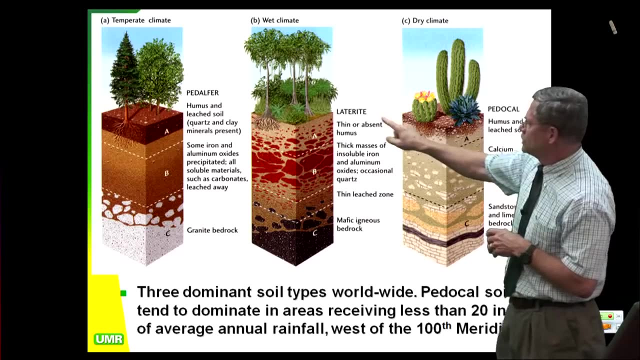 South side of Las Vegas is old debris flow fans lots and lots of gypsum, Gypsum's highly soluble, highly reactive, Bad news stuff. So these are pedical soils and they take a lot of experience: Very, very thin little discreet soil horizon. 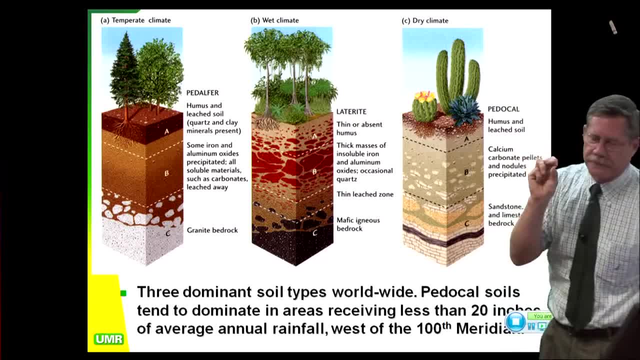 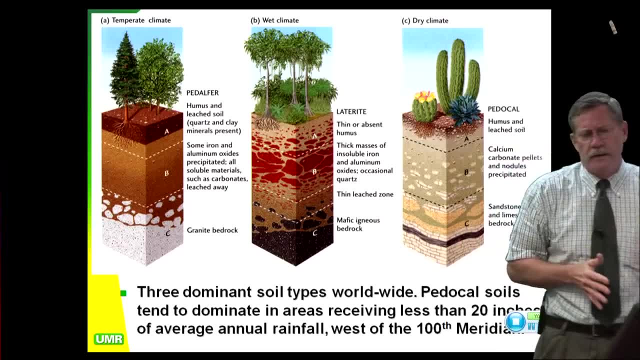 Out in the desert your soil horizon can be little as a quarter-inch thick. This is why we can actually get on satellite pictures and we can see all the way up there, all the ruts out in the Mojave Desert from Patton's army doing maneuvers out there in 1942,. 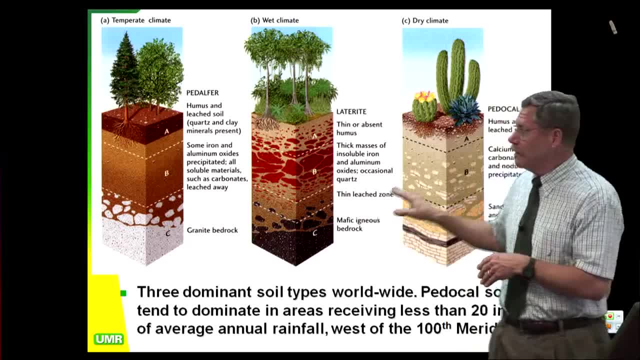 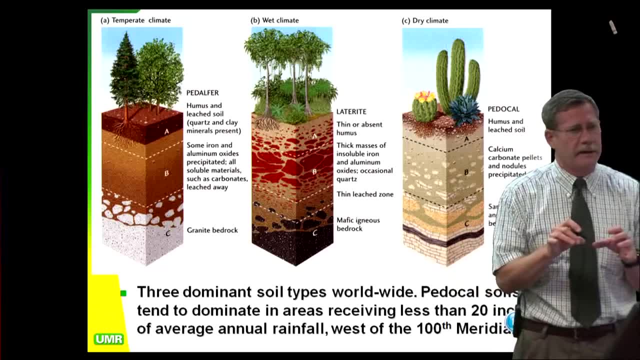 because they ran around a thing: they disturbed this very, very delicate soil horizon and then they got condensation of moisture in the cold nights and they got a little bit of carbonate cementation. We see that same thing in parts of the Middle East. 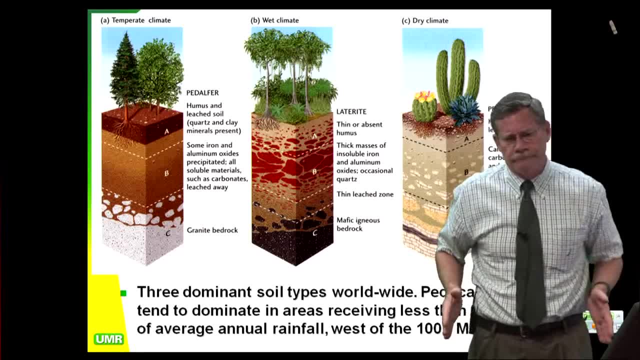 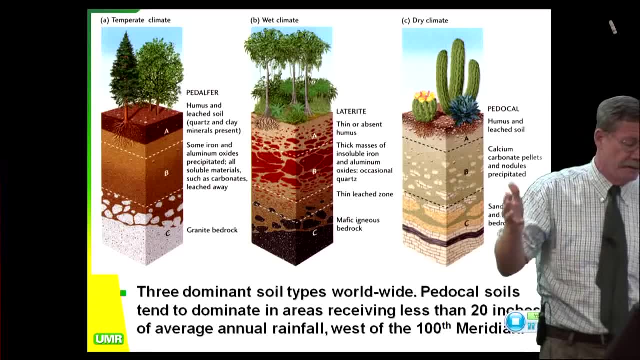 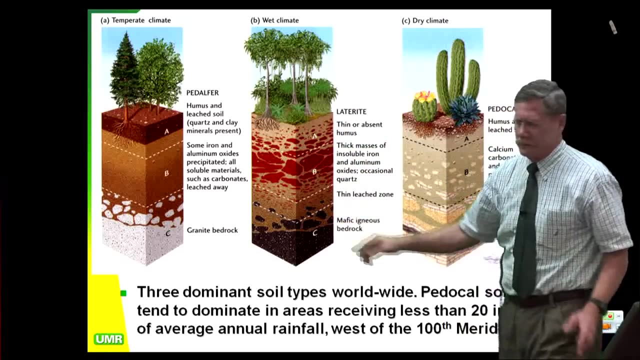 from even Egyptian chariot wheels made out of bronze, and they got through and left tracks that have been weakly cemented. Now, if we look in the tropics, the tropics, whoa- all bets are off. You've got to think completely differently here. 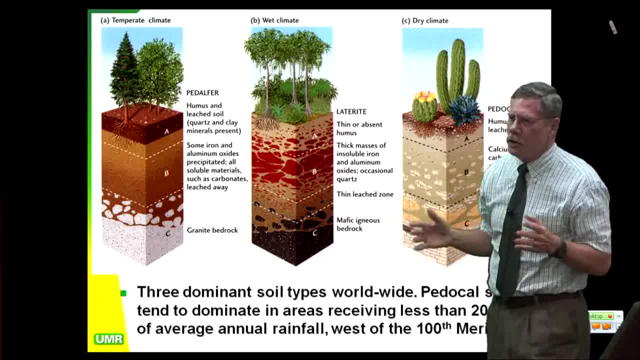 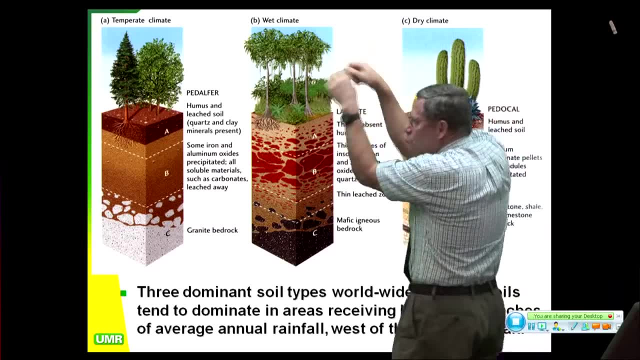 You've got to think like you're at Starbucks and you're making very strong coffee. Now you're just pouring water, hot water, through this stuff, just pouring, And the stuff's going down and it's just picking up. 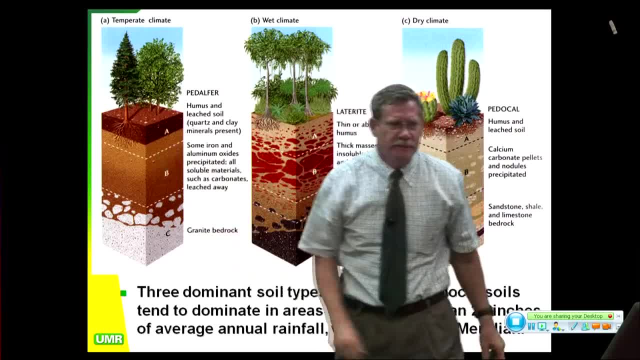 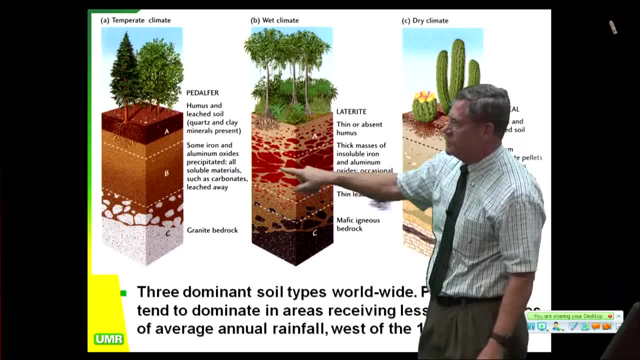 Everything it can find and doo-doo-doo-doo-doo, goodbye. So all your solubles are gone. So the things that are here, what's left here? These things that look like you know, kidneys and filet, mignons and stuff. 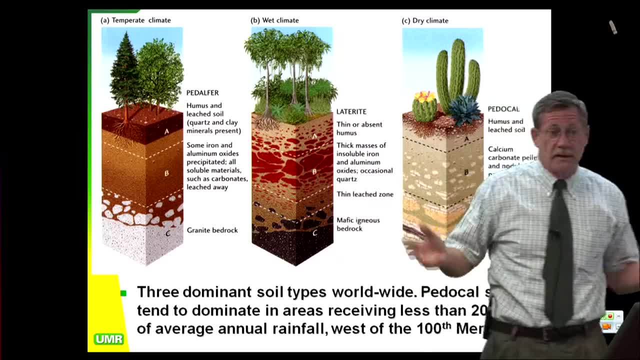 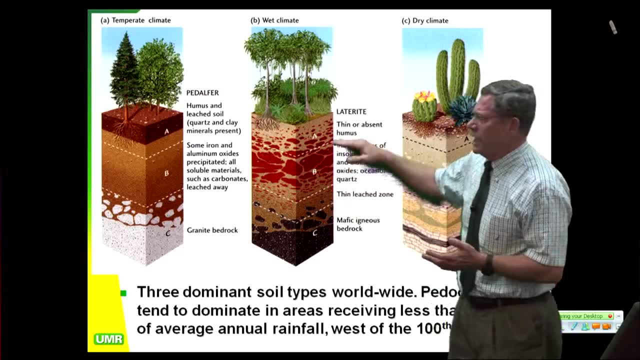 this stuff are insolubles- bauxite, you know, like aluminum ore. That's why bauxite comes from Venezuela, right down near the equator. So these guys are insolubles and these are really fun to work with. 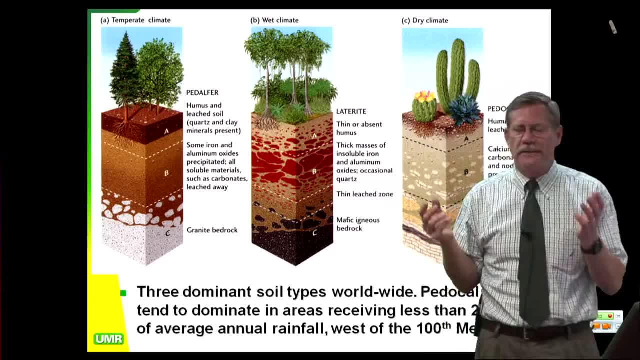 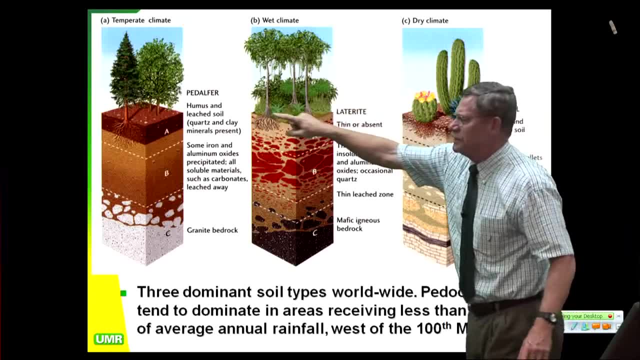 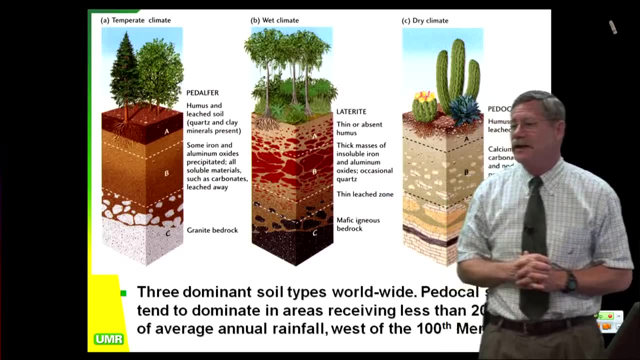 Again, highly variable condensation. One of the first building foundations I did consulting on down in Panama we had four holes on four sides of this bank building. Couldn't correlate any of the holes, So they brought in this American consultant from New York City. 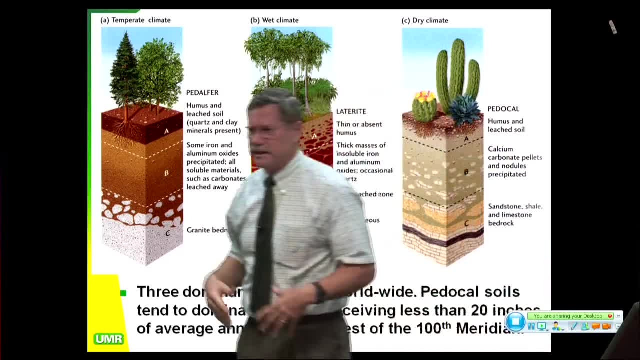 You always tell a person from New York City they're wearing all black because they all used to be in the Undertaker business or something. They're always wearing black. you know Now, a guy from California, how do we dress? 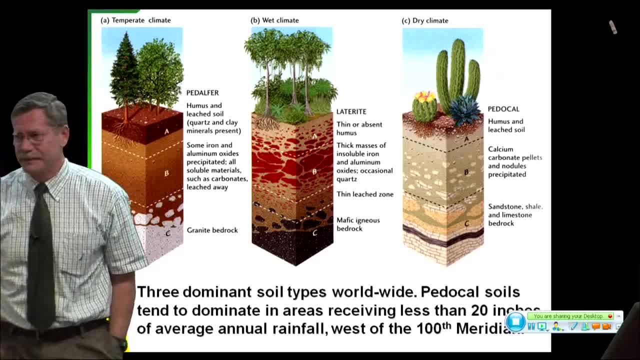 Yeah, Tevas and a Hawaiian shirt- right, Shirts, right. okay, I'm being nice to you, I'm wearing long pants today, okay, So anyway, this guy from New York comes in, He goes. well, this isn't very easy. 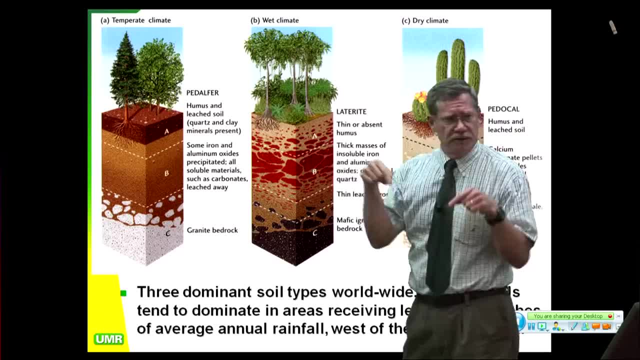 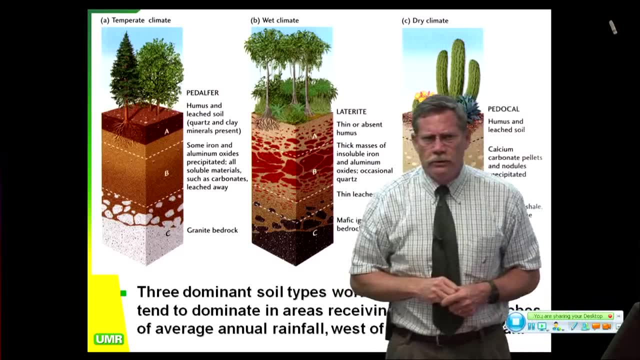 What you need to do is to drill a hole in the middle, and then you'll start seeing. you know what's going on. I drilled a hole in the middle. It only got worse And this guy goes. that's impossible. 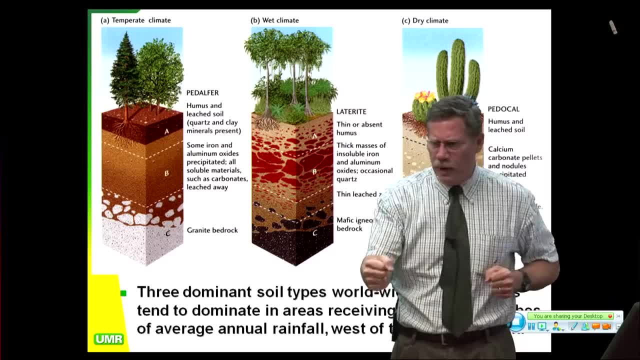 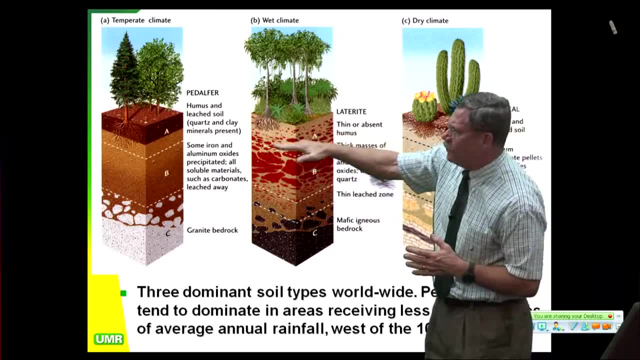 That's you know. we halved it by order of magnitude. We don't have as much distance between them. Well, the problem is you don't have a layered sedimentary system. All these things are getting there by leaching in place. 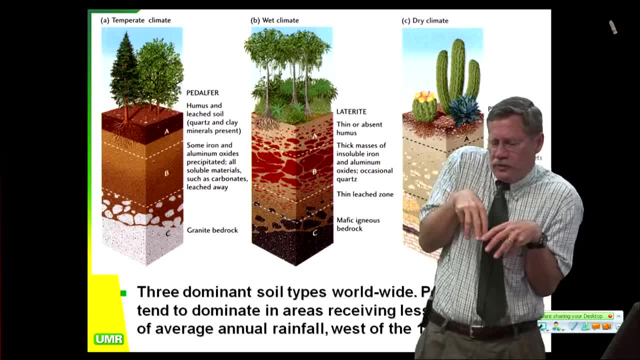 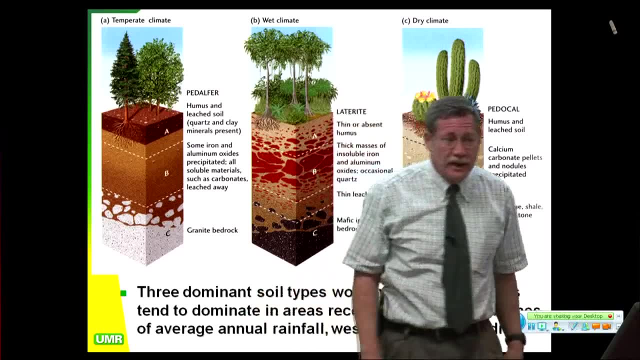 And you have little percolation corridors that look like gopher holes. Some of them are going over here, Some are going over there, Some are going out the rear over here, And you try to figure that out with a two-dimensional cross-section. 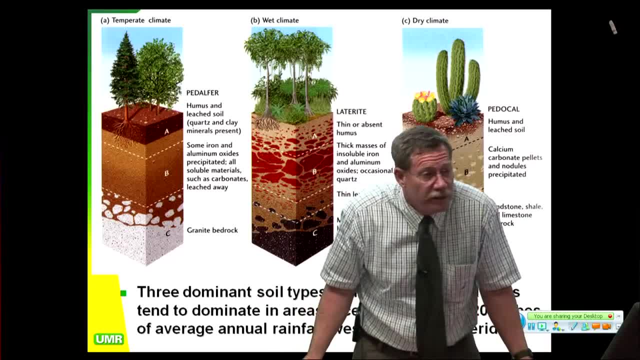 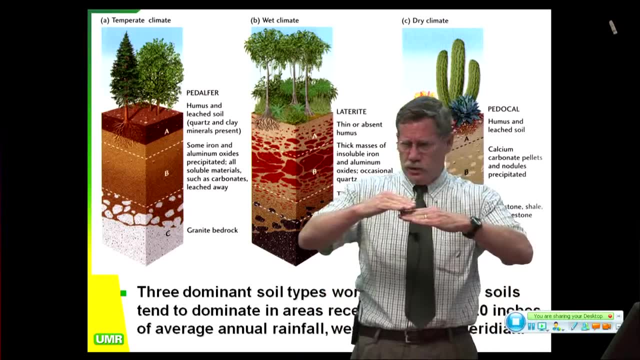 and guess what? You can't. You can't do it. So what do you do? Everybody asks me: well, what do you do, Dr Rogers? I say, well, you draw a dash line and you have big two-sigma lines. 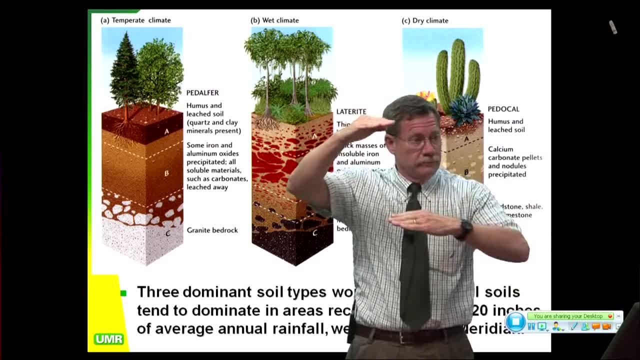 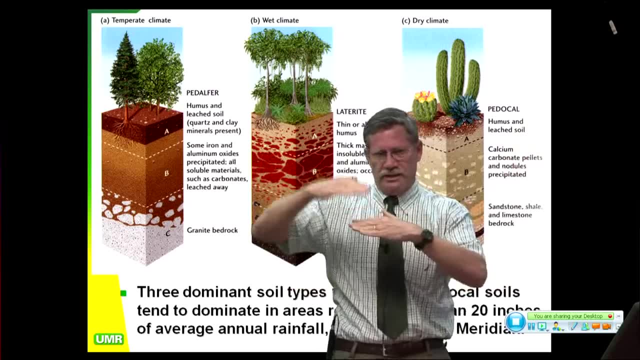 above it and below it, meaning the uncertainty is very great. Now you've got to realize: the closer the borings are together, the less uncertainty. The farther the borings get apart, the more uncertainty there is with where that geologic contact goes. 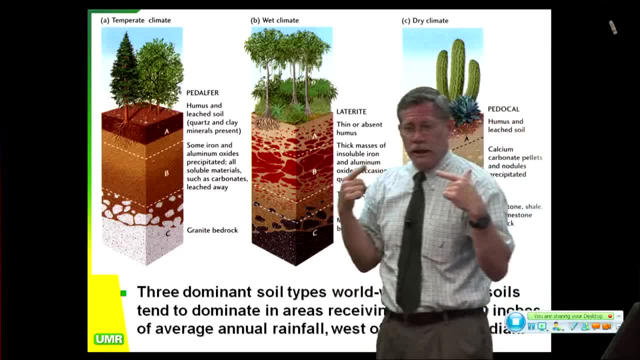 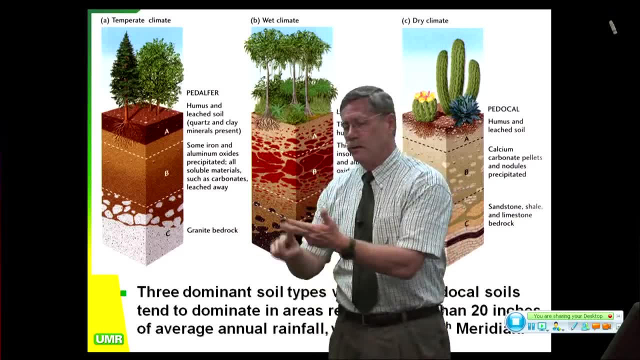 You've got to be careful, But you've got to be real aware of geotechnical uncertainty, because that's how you're going to sell your client to do more geophysical work or to do more cone penetrometers or, you know, do more borings. 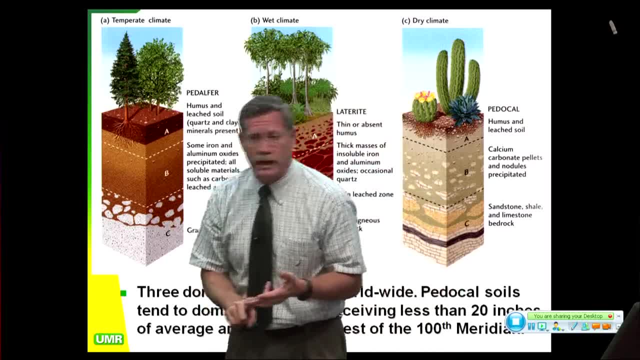 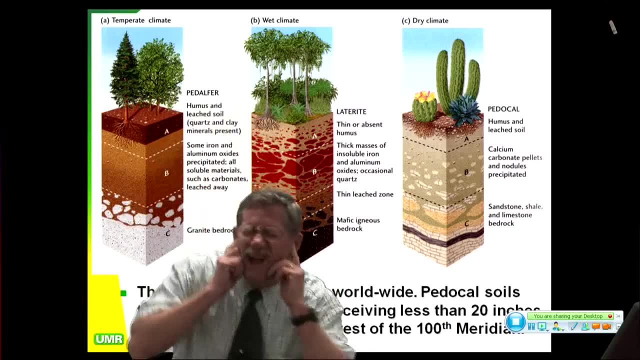 Borings are the last thing I do, folks. I mean, borings are like a Polish minesweeper. You ever seen a Polish minesweeper at work? You know what that is Ready? Okay, this is an Army thing. 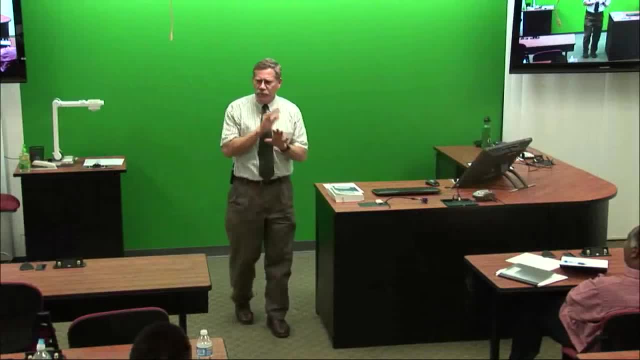 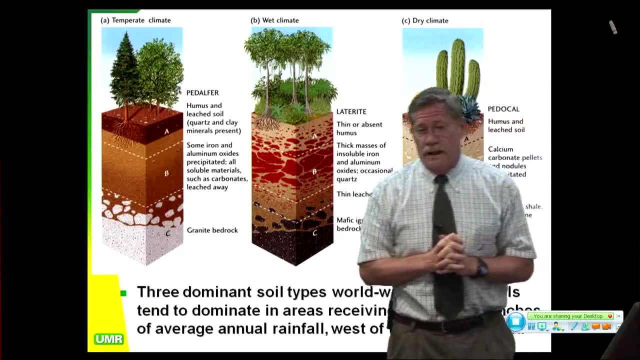 That's a Polish minesweeper. It is out there, bop, bop, bop, bop and you're hoping to hell. you hit something, but your chances of missing it are very, very great. I mean, borings are like little piano wires. 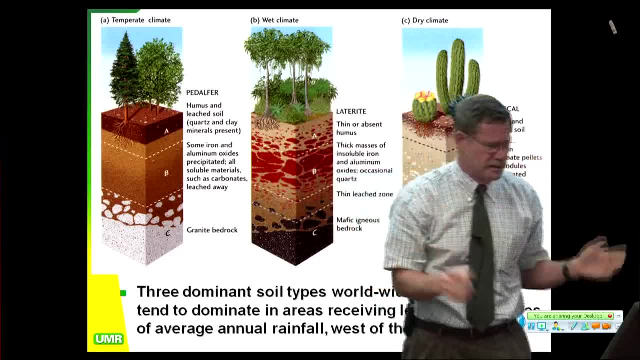 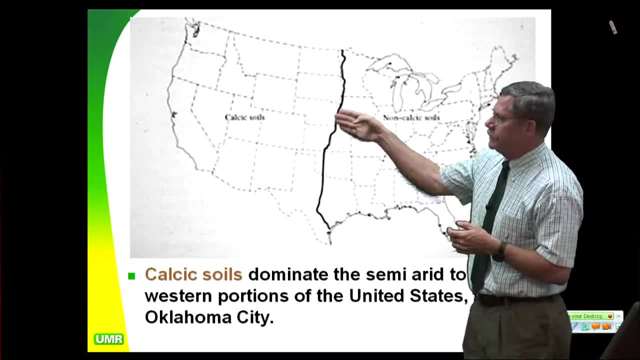 stuck around, It's very easy to miss things. All right, So if we look at that 100th meridian line, the rough 100th meridian line, it looks like this. It goes across: These are calcium-rich, calcite-rich soils. 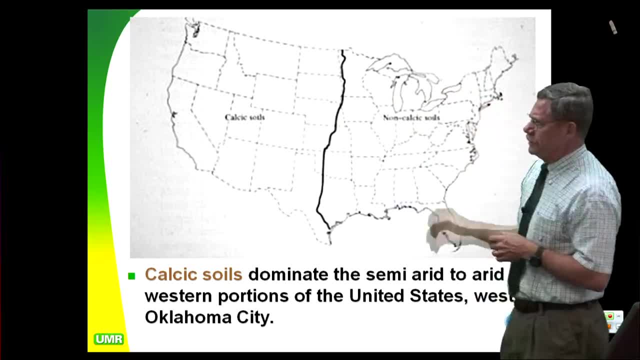 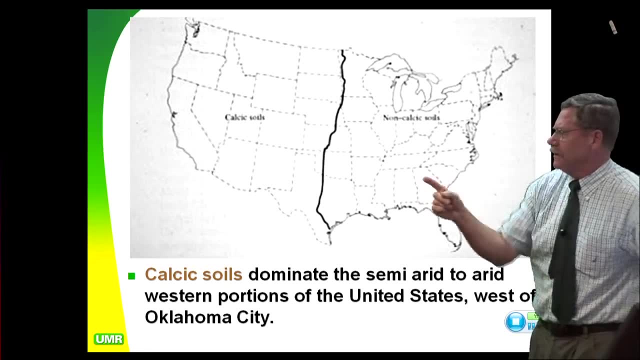 out in the western part of the United States and non-calcic soils in the eastern part of the United States, And so foundation conditions are going to tend to be very different depending what side of this line you're on. Now. the problem with out west is watering. 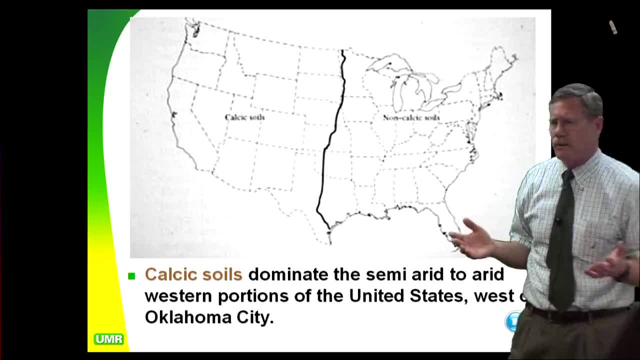 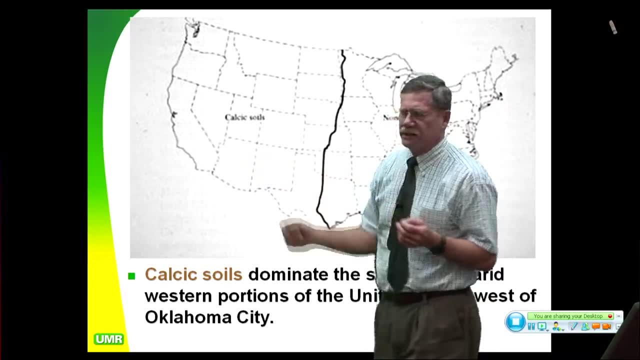 That is dry, dry area, They don't get as much water. But what if you go to Phoenix, Arizona right down here? If we go to Phoenix today, there's all kinds of green things growing. Where's that water coming from? 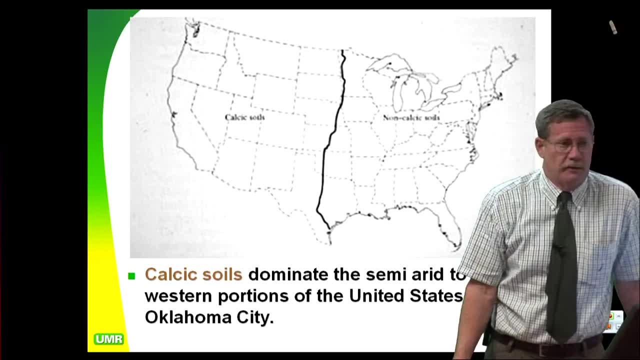 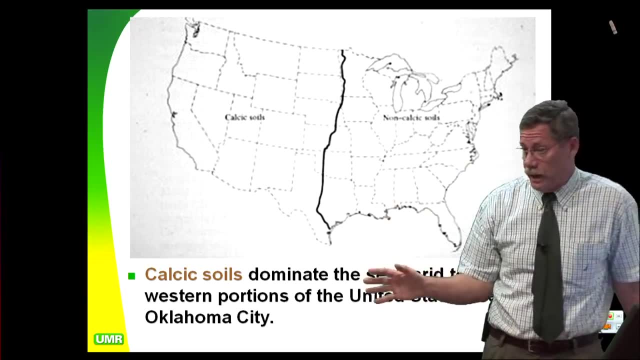 The Salt River and the Verde River and the Colorado River, So they're adding water to an area that used to be very dry. And there's a whole new area of soil mechanics, which is called unsaturated soil mechanics, where we deal with things like hydro compression. 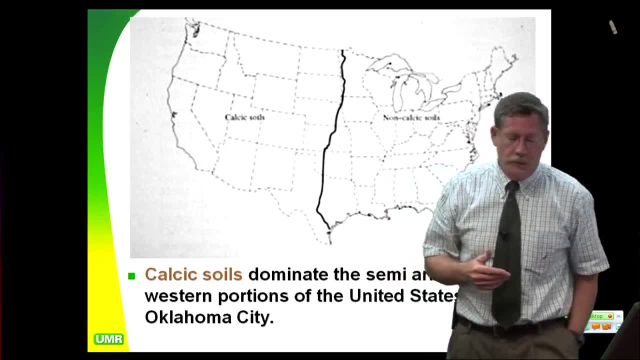 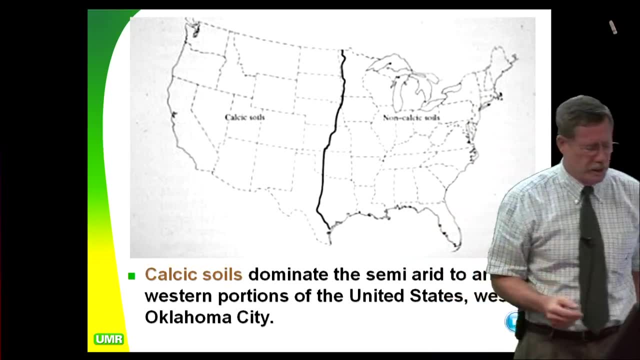 We're going to talk about more when we get to Chapter 4.. Those are issues that are going on, that are used to be completely missing from the geotechnical textbooks 20 years ago. They're a big issue today because in places like Phoenix and Las Vegas, 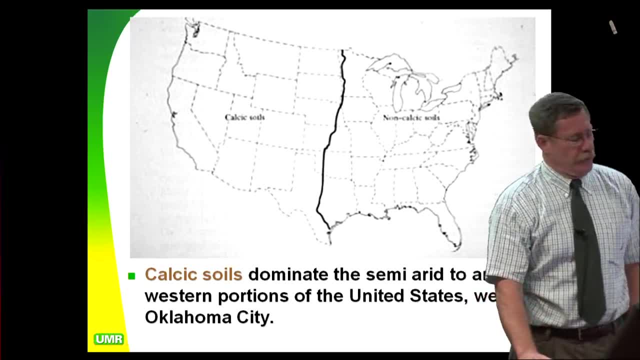 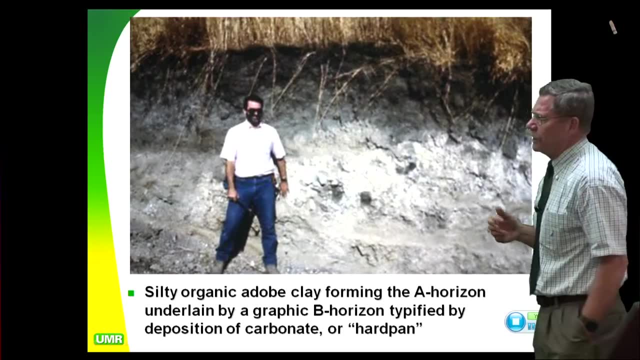 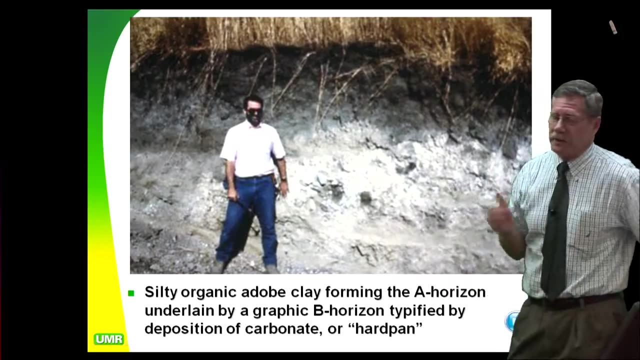 and Palm Springs and other parts of California. they play a huge role in damage. Now here's a typical kind of soil you see in coastal California, Coastal California- every mile I go in from the coast the soils change. It's not like around Phelps County. 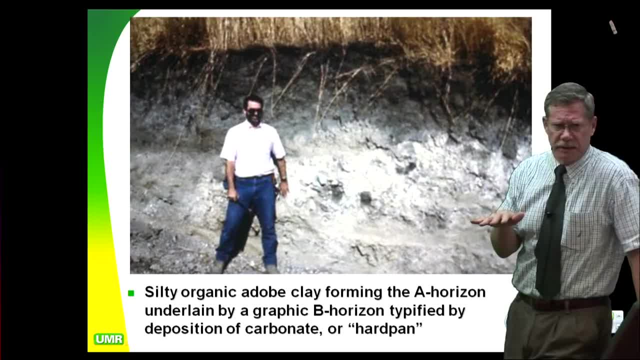 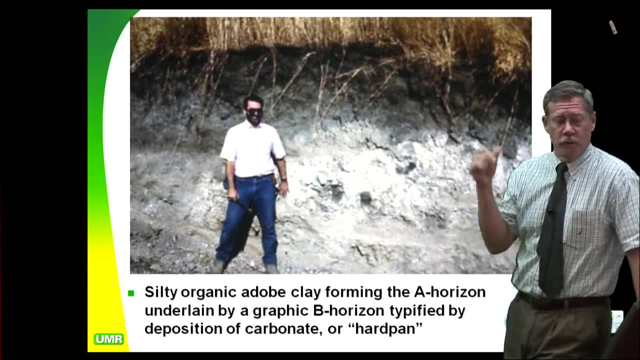 I'm in the most boring, in the most boring part geologically of the North American continent. right here This is the oldest erosional surface in North America, Over at Fort Wood. they've documented erosional surfaces over there and up here at Rolla Airport. that date back to late Middle Miocene. It hasn't been glaciated. It's not high enough to get a lot of erosion, Just not. a lot of exciting stuff has happened here in terms of geologic deposition and erosion, But in California you have that rain. you have moist air in the wet season coming off the ocean and that air bleeds off as you go inland. So you don't have to go but 20 miles inland and you're in a subarid environment. You go 40 miles inland. 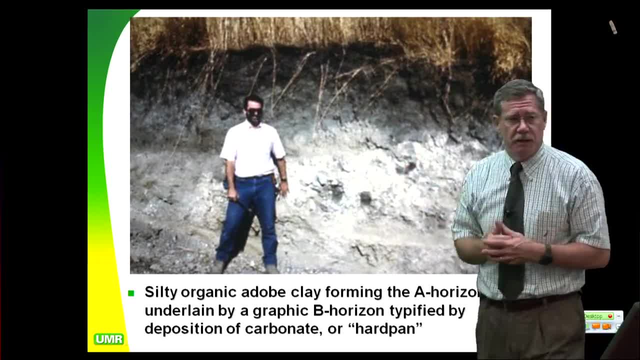 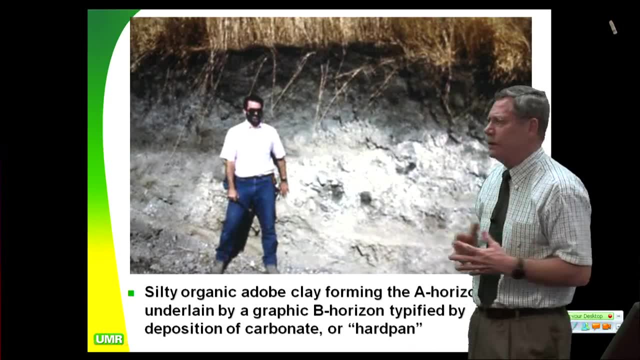 you're in an arid environment, So, but over in San Francisco you freeze your tush off in the summertime because you have this coastal inversion breeze coming in. It's real cold, clammy and chilly. So here we are, right here. 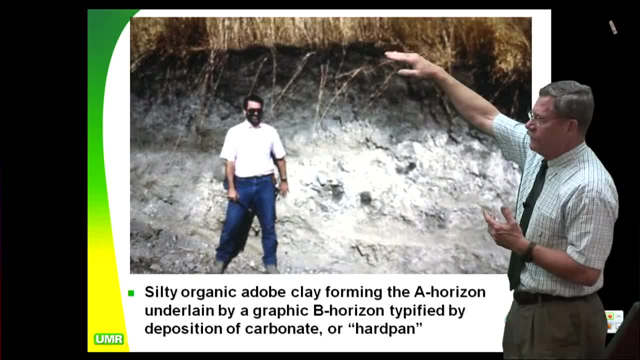 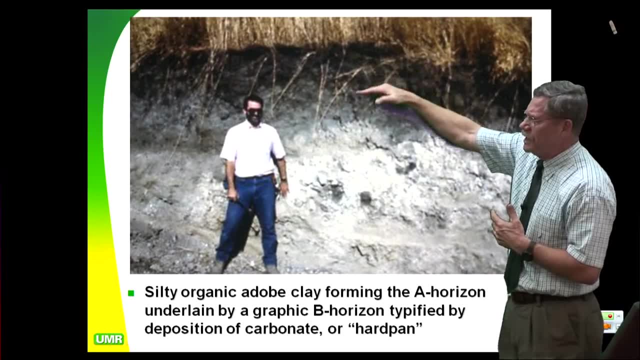 Now we're about 20 miles from the ocean. here We have a very, very highly plastic black silty, adobe clay. It's a CL And this stuff up in here, the PIs up in here are all 55 to 85.. 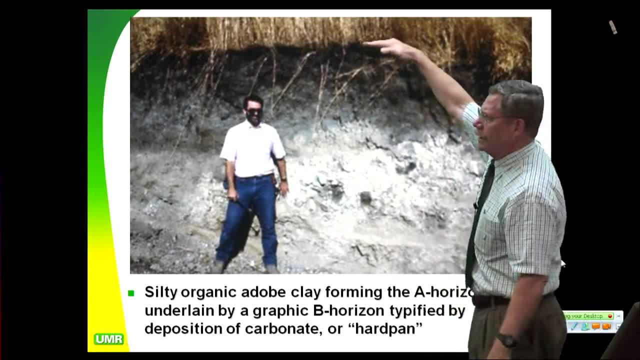 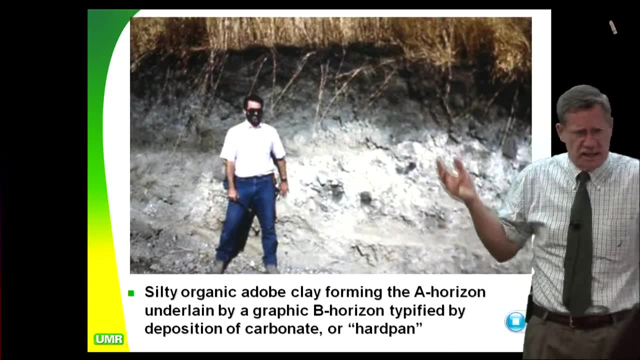 They're big time. You don't want to build anything on here unless you put a whole lot of water on this thing for a couple months and get it to suck up all the water it can and swell up and then build something on it. Now you have here is hardpan. 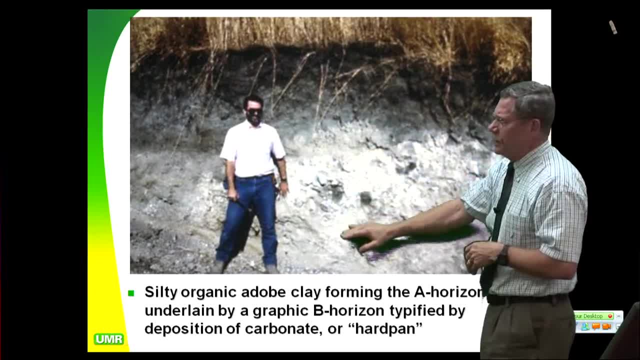 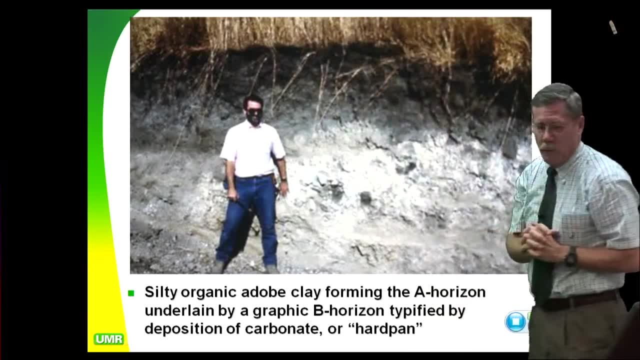 There's the hardpan. This is the caliche layer. This is the carbonate. Now, as the water percolated through here and it fed the grass, the grass was green during the wet season and it stops raining about the middle of April. and it doesn't start raining again until mid-October to mid-November. So you have six, seven months no rain, None, Zero Zilch, That's California Now around here. if you don't have rain for two weeks. 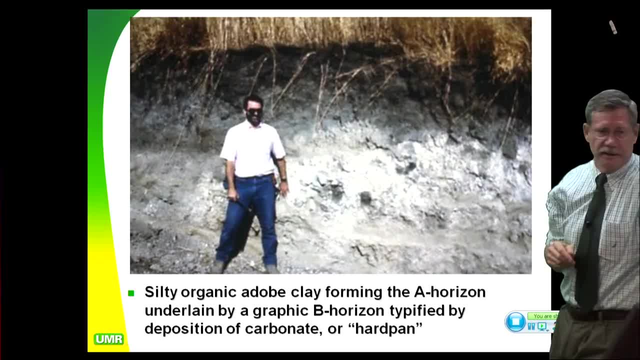 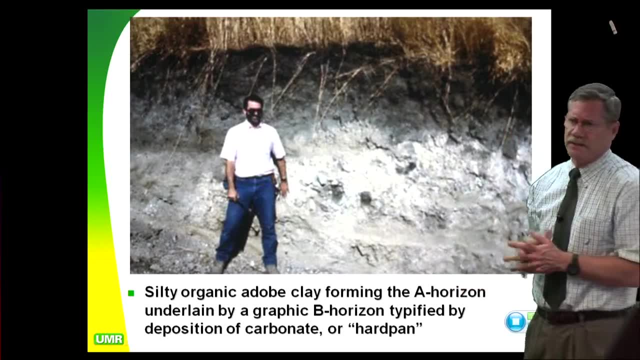 it's a drought. They're starting to call the president and trying to get a declaration and everything, And the ground does start cracking and everything, But it's nothing like what you have out west of the 100th Meridian in terms of a seasonal drought. that's just constant. 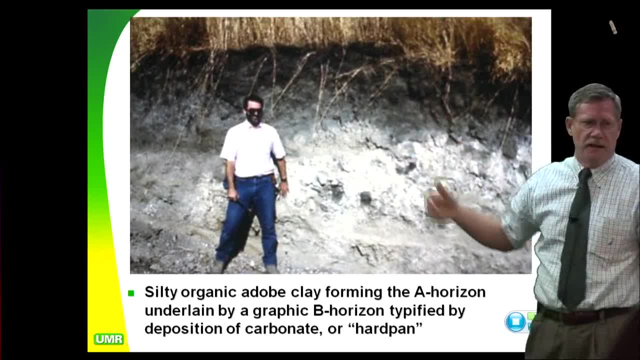 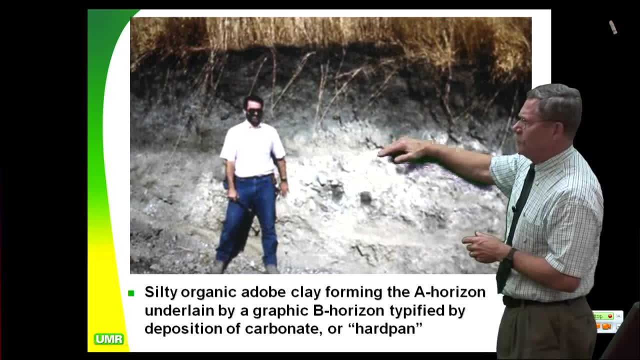 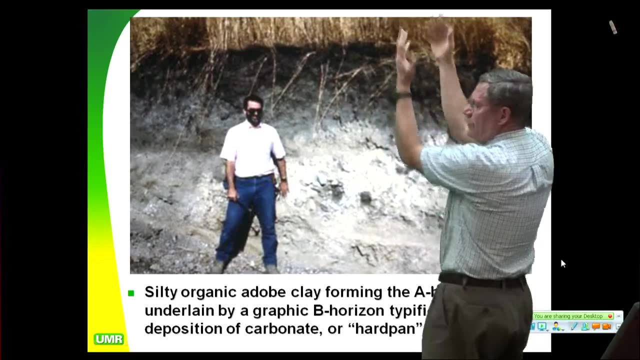 So that's why you don't do agriculture out here without dams, canals and irrigation or wells and irrigation. But these carbonate nodules here have formed over thousands and thousands of years because this ground is The water is being cooked off by the very high heat in the summertime. 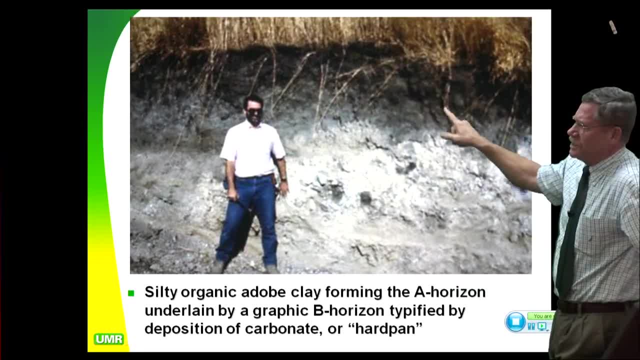 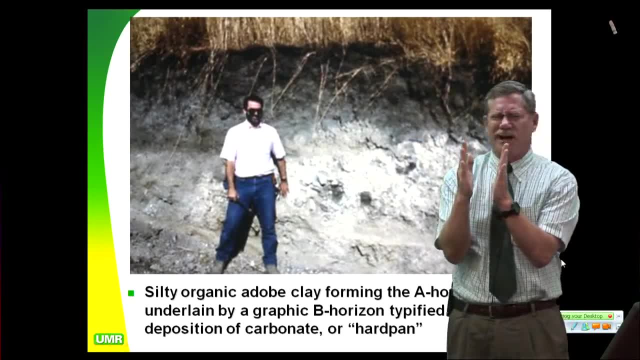 Now we always get into arguments: How deep do desiccation cracks go? I mean desiccation cracks are when you have the clay shrinking. We're going to talk a lot about that later. Clay is like a wife. It has a great memory. 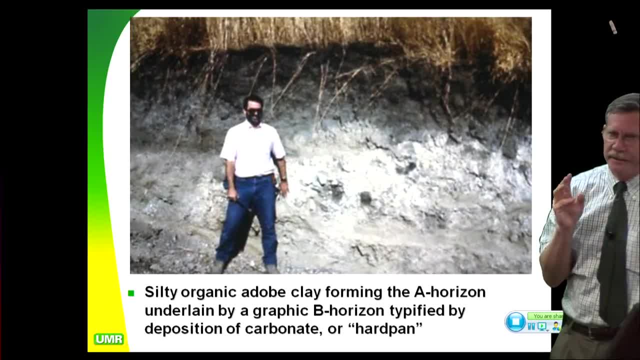 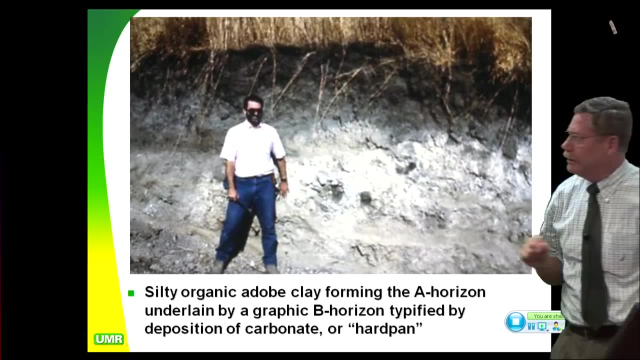 It remembers everything that's ever been done to it. So clay is the great. You can't take enough classes on clay mineralogy. Everyone you can scam out, go take it, because you're going to use it somewhere down the road. So these materials are really 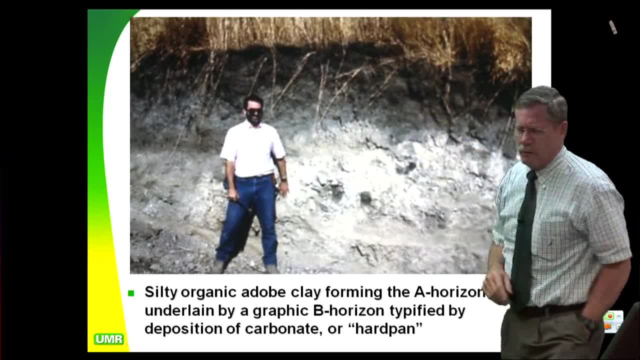 You know, we say, well, how deep is desiccation cracks? Most engineers will say, well, I'm going to assume 30 inches. You take a meter, stick out there, which is 39.4, and you just drop it right down. 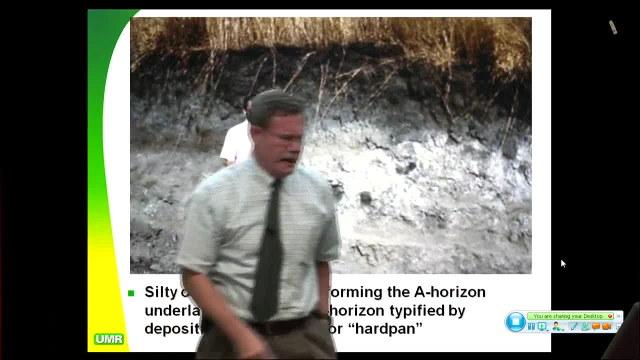 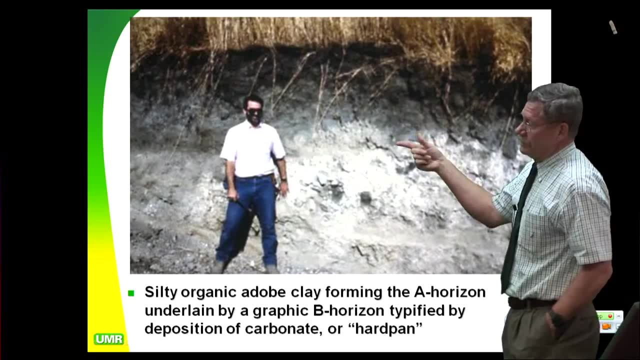 It disappears, You go: oh, it looks like a little deeper than Well. I can't design it for you know: 12 feet, How deep are these things? Well, there's actually documented cases in the San Joaquin Delta, back in 1880. 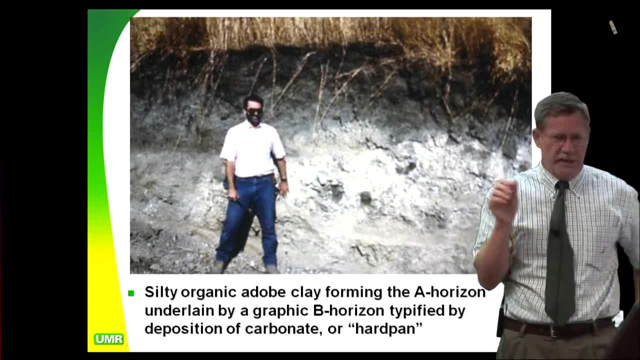 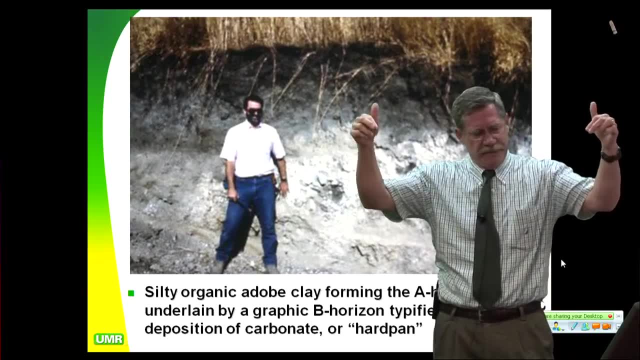 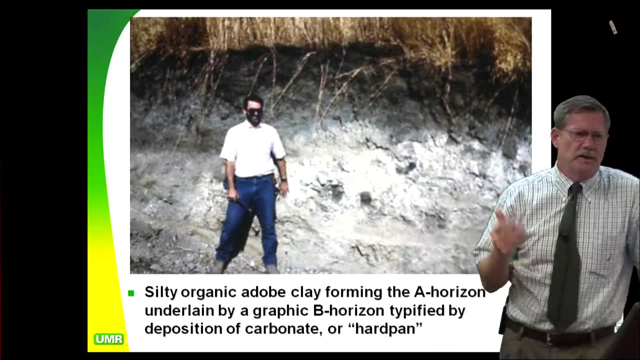 by John LeConte, professor of geology at Berkeley, where they did a big excavation out there in these peaty islands and they actually had these desiccation fractures filled with sand that went down 60, 80 feet And some of those we think. 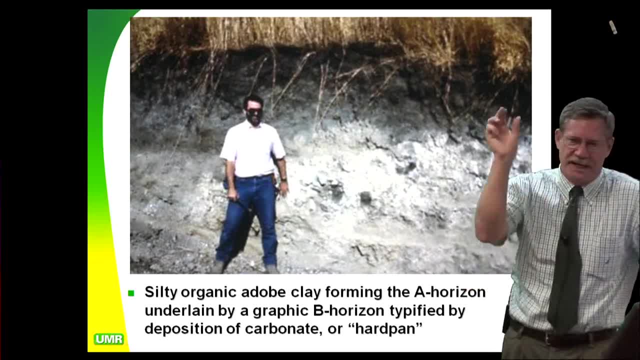 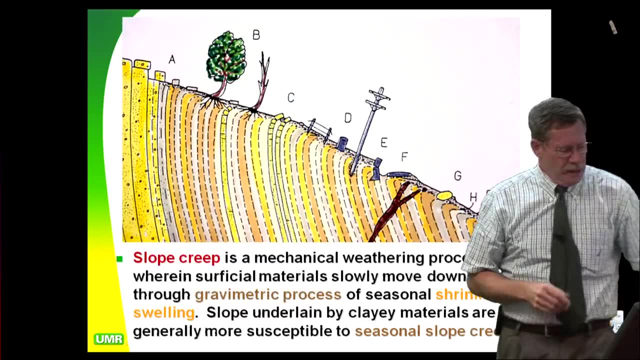 are due to liquefaction features. now, We don't think they're desiccation all the way down, They're probably liquefaction. But obviously these things can go a lot deeper than that. They can go up to 130 inches. Now, slope creep is something. 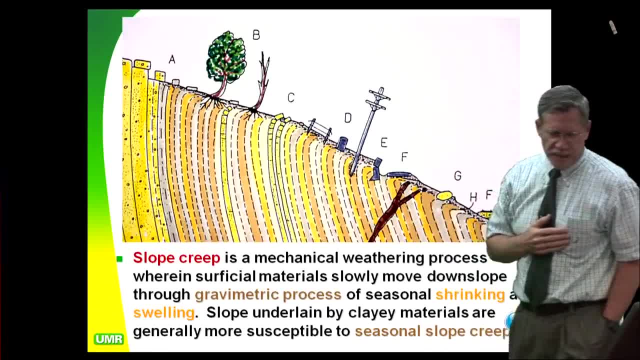 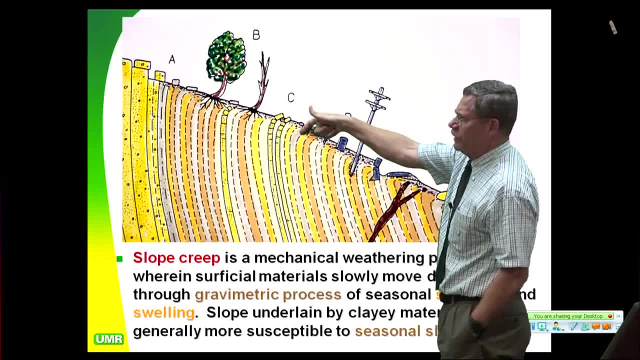 you really need to be aware of, especially if you're a geologist, because geologists go out in the field to places like this and they take a strike and dip right here and then they project it with a ruler And they go. eh, there's the strike and dip. 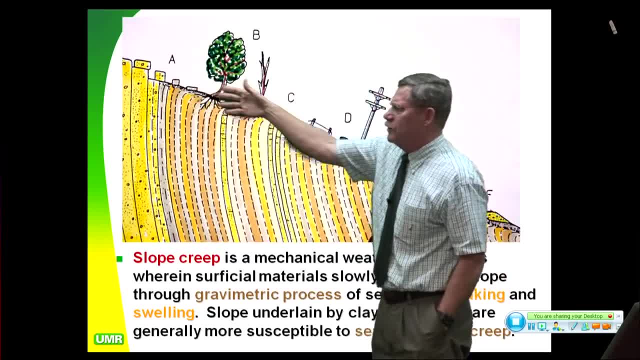 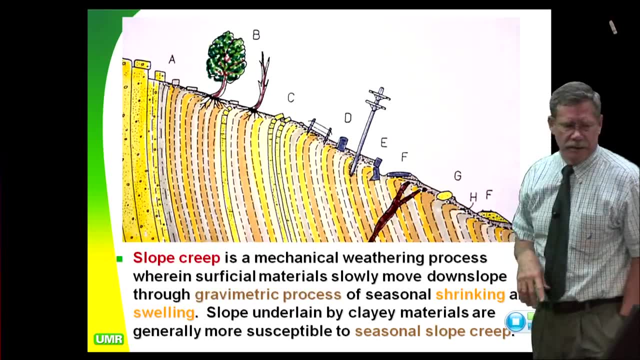 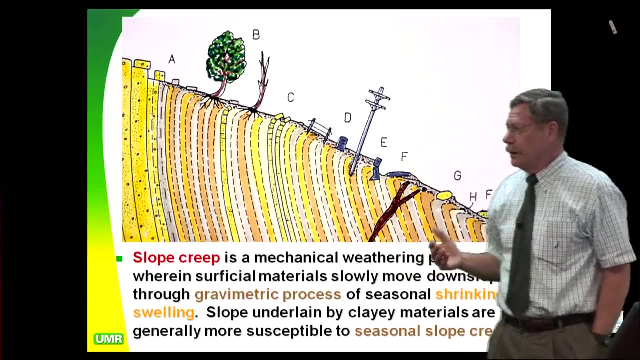 Wrong. There's no reliable strike and dip. you can take on a slope. See why This was published back in 1938. Because of slope creep. Creep is an engineering term. It means strain under sustained load. All slopes are subject to creep. 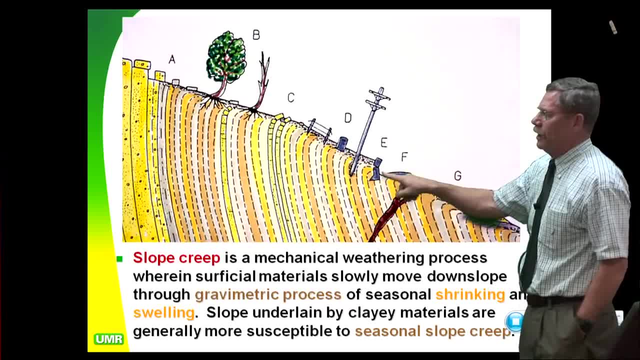 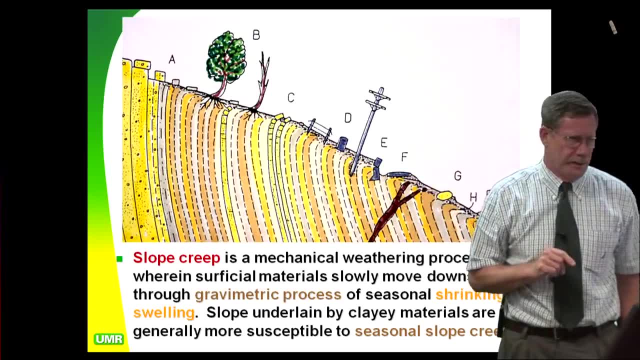 Creep is the hardest thing to design a retaining wall for Why? Because you're going to get passive pressures on the active side of the retaining wall. Nobody wants to do that one. Nobody wants to do that one. Come on. No, you don't believe me. 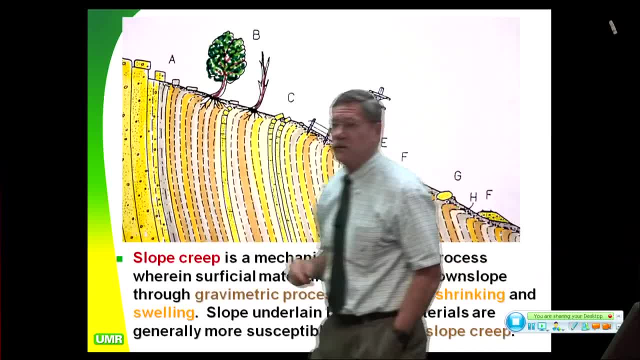 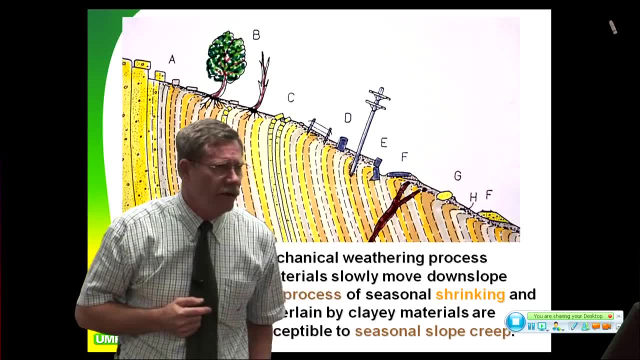 Walk around Rolla, Look at our retaining walls. If you find one over 6 feet high, that isn't failed. come see me. I got $5 for you. Okay, They're all failed. What's going on? Most of them don't have enough drainage. 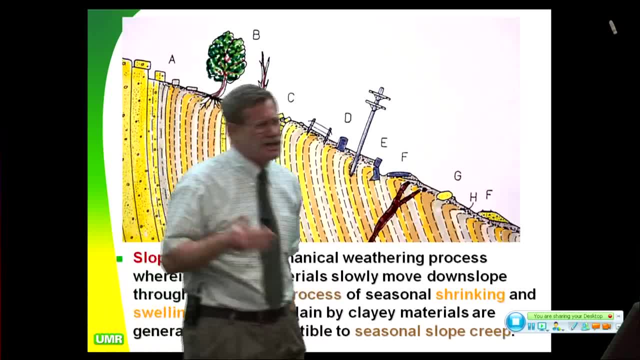 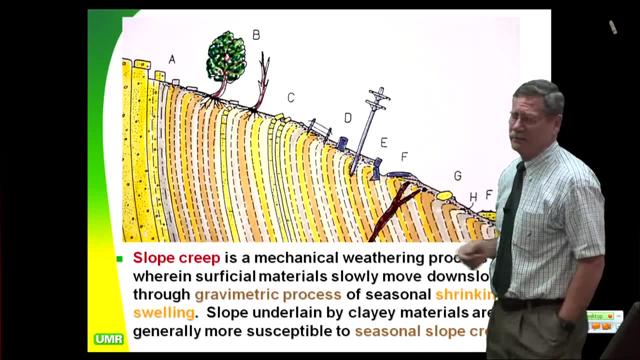 They put native soil behind them. You're going to go 6 feet with clay with no drainage. Yeah, It's going to be hard to do long term because of creep. It's going to be hard to do. You also have surcharging. 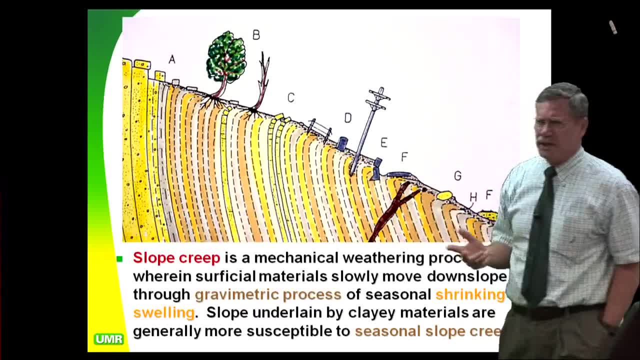 You have load on top of it. But if you go out- and what I want you to do, if nothing else you get out- of my course you say Roger's got a lot of sick jokes. He's kind of you know, blah, blah, blah. 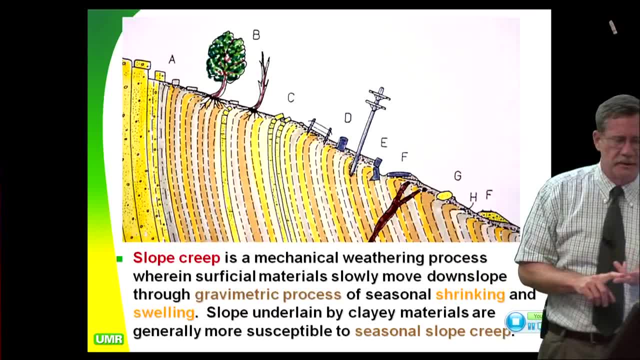 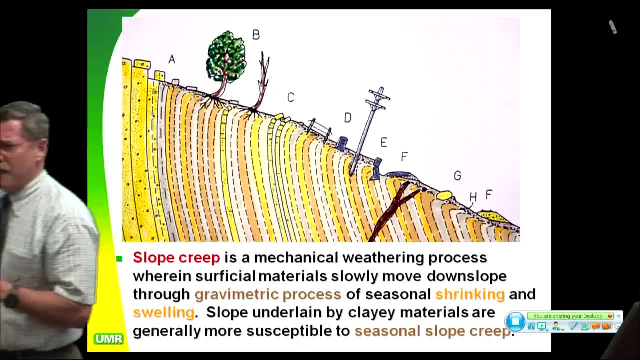 But I want you to become an astute observer of nature. It doesn't matter what I say. It doesn't matter, actually, what the lab data even says. Don't get overly enamored with lab data. Lab data used to drive me nuts in all the forensic consultations. 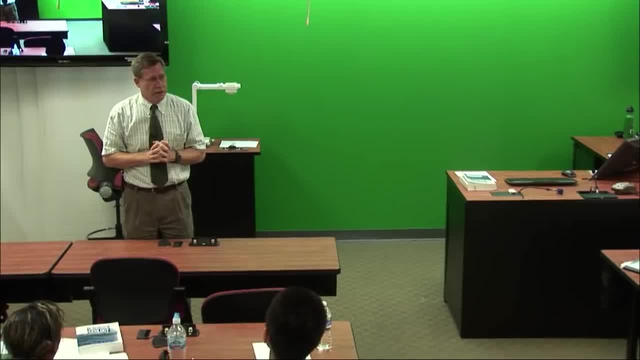 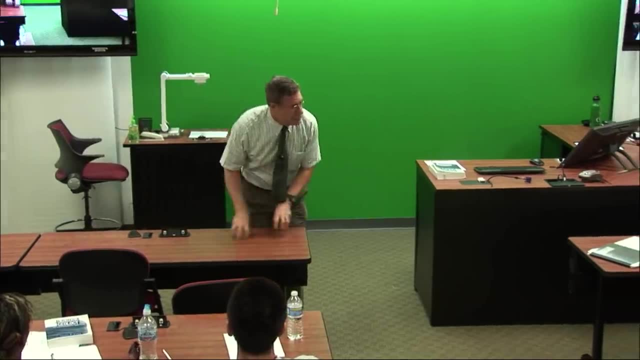 Roger's Pacific worked on Why? I'll tell you why. You want to have some fun, Take any job you want, Take samples- all the same samples- and then send them to 16 different soil labs or environmental labs for water samples. 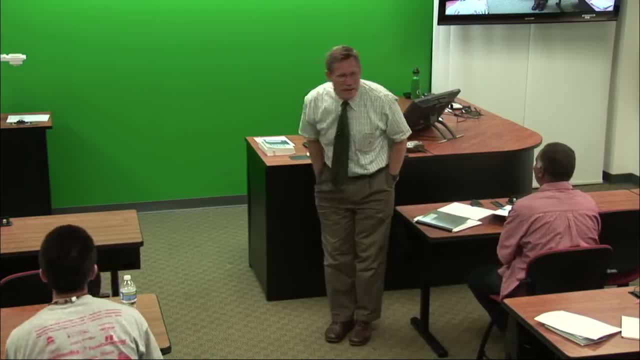 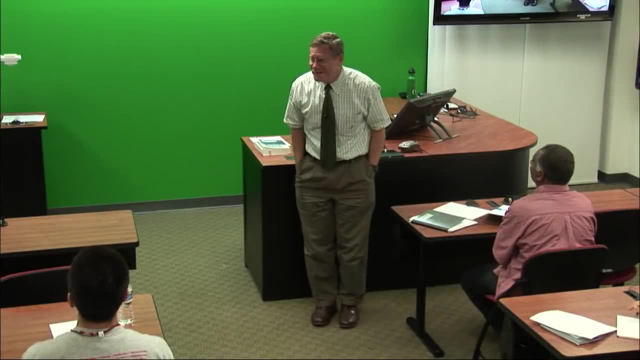 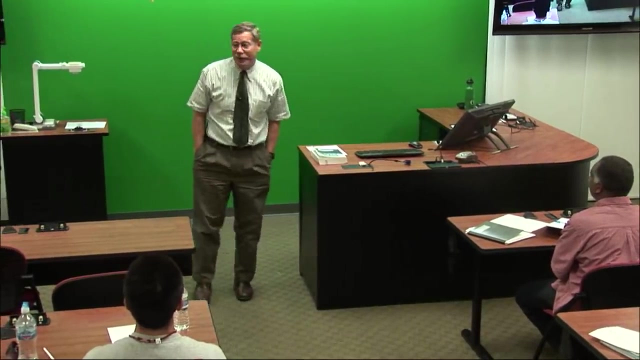 and see the answers you get, It will scare the hell out of you. Does anybody know what they're doing in these labs? Maybe a few. I would trust Rick Stevenson. There's one guy that does know his lab stuff, But there aren't very many guys like him around anymore. 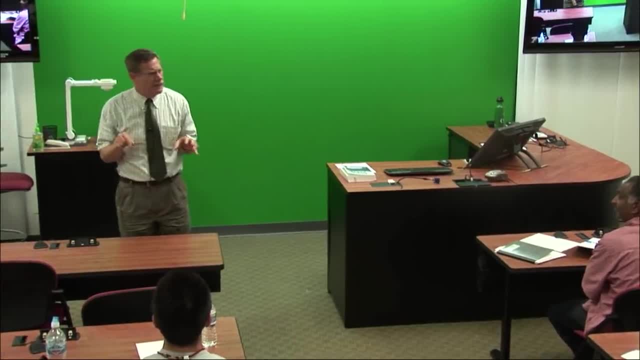 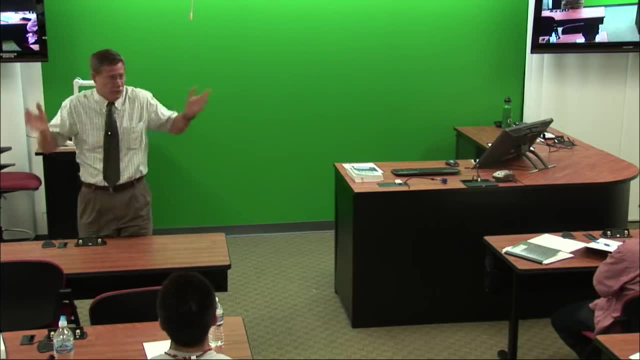 Most everybody have become computer jocks, And the NSF has this new program. It's an interactive soil mechanics laboratory, So you don't have to teach soil mechanics anymore. Who wants to do that? There's no research money in that. So we have this thing that they had a professor. 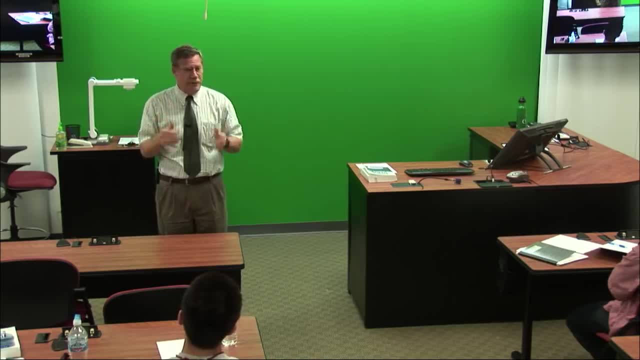 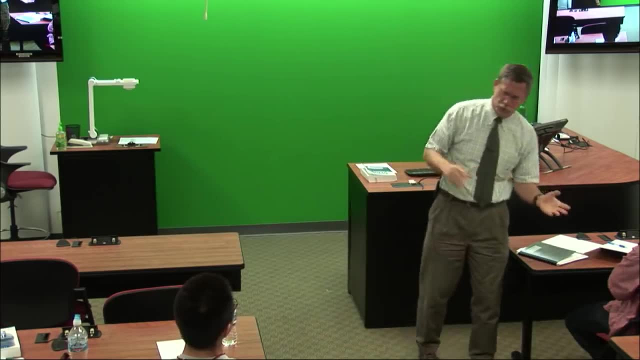 up in Idaho And I was one of the beta users. they sent it out to and said: Professor Rogers, since you had private practice, you're one of those kind of people. could you please comment on Professor so-and-so's program? Oh, oh. 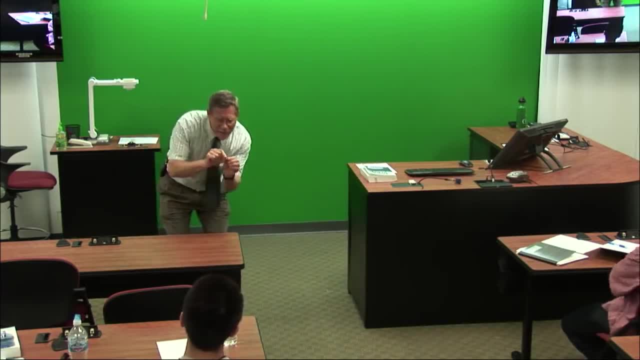 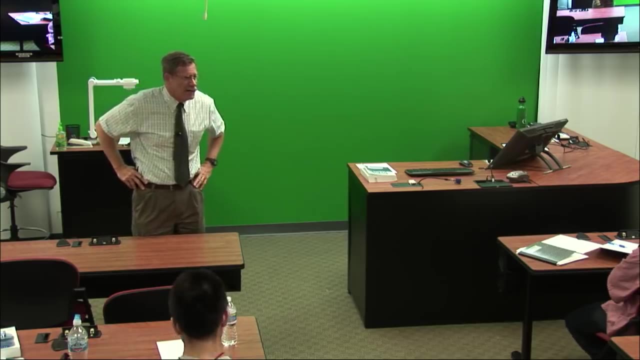 I never have seen triaxial tests that perfect, Just perfect. They were like Venus de Milo: Perfect, Everything, Just. oh, That's not real world at all. That's some PhD pinhead up in Idaho doing that. That's someone who hasn't run very many triaxial tests. 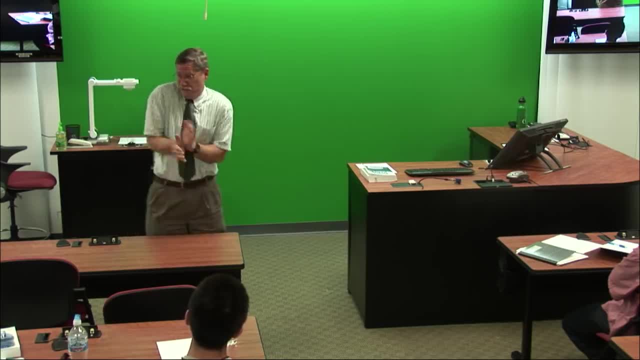 I never had them look that nice. You have to doctor them and do other things And there's air that gets caught in the lines. They ain't that easy to do. kids, Dynamic triaxial tests: Run. You don't want to do those. 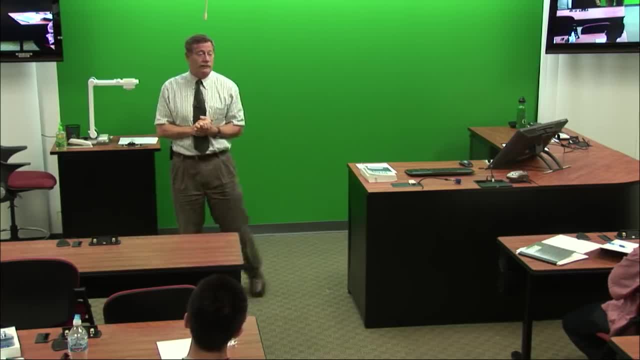 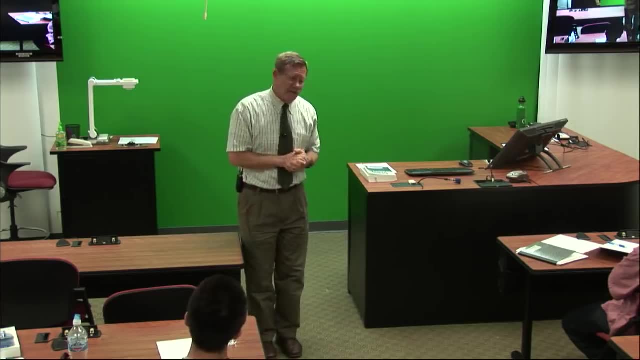 Those take you a year and a half Figure out how to do them correctly. There's so many things that can go wrong. Do we have those kind of people running soils labs? Not generally. You're lucky, You know- in soils labs. 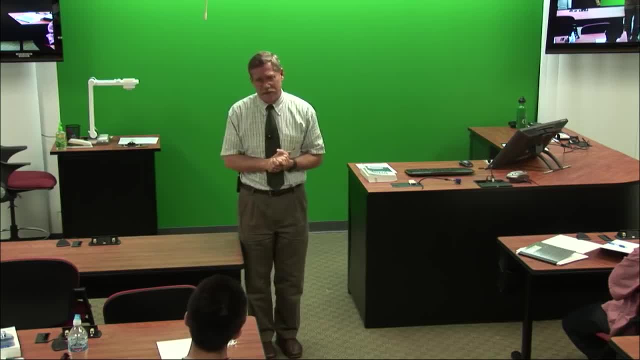 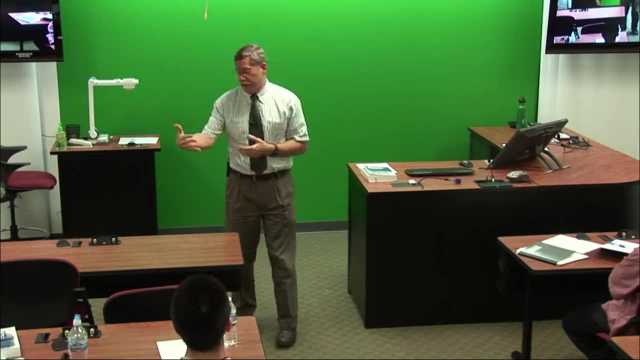 mostly people holding, you know, green cards and at the lower end of the pay scale, And you're not going to get that kind of control. That's why you have to have quality control. You need an old fart like Stevenson looking at the data going. 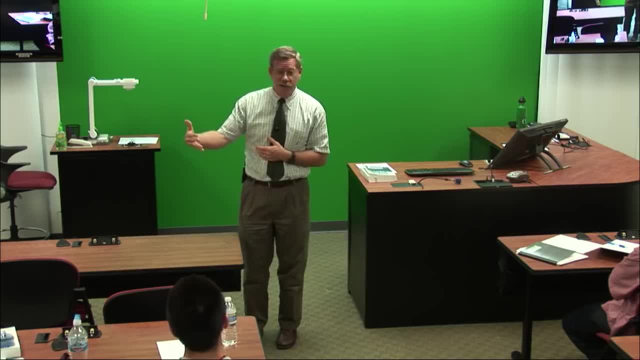 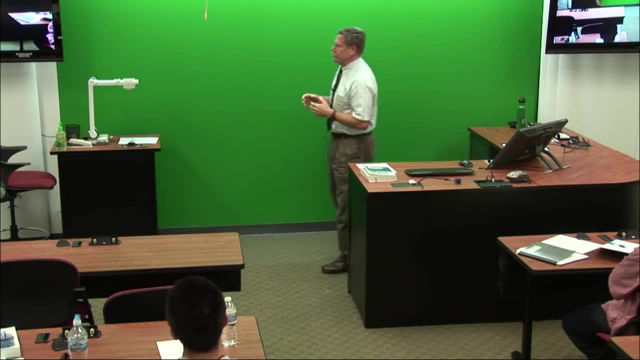 that don't look right, That's right. Doesn't look right, Doesn't look right. guess what? Probably isn't right. But I see more trouble with lab data. So why am I telling you this? Well, because I want you to become an astute observer of nature. 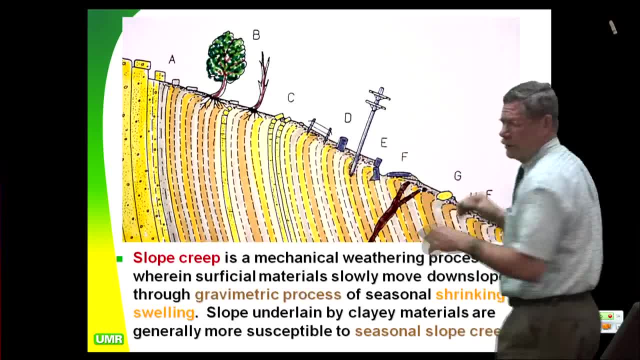 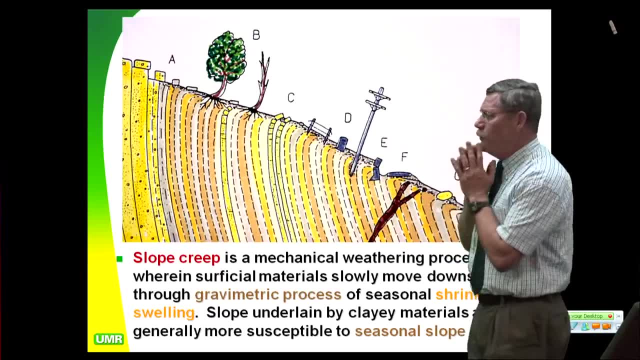 Nature and behavior are more important than lab data. You go out, You're driving down the highway and you notice the telephone pole is leaning. Bob, I wonder if it was built that way. Probably not. Probably was built this way originally And it's leaned over. 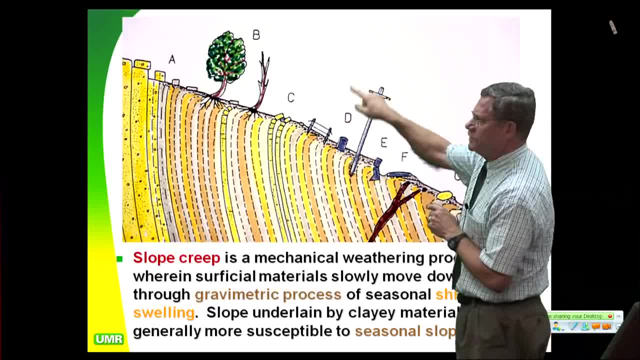 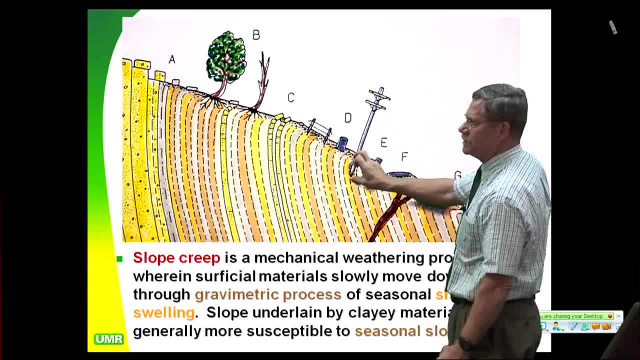 Oh, that's interesting. Now, this one you got to be real careful about, because the amount of tilt here is not an indication of the annual creep rate averaged out. It has to do with the bending moment and how deep this thing is And the fulcrum you have going there. 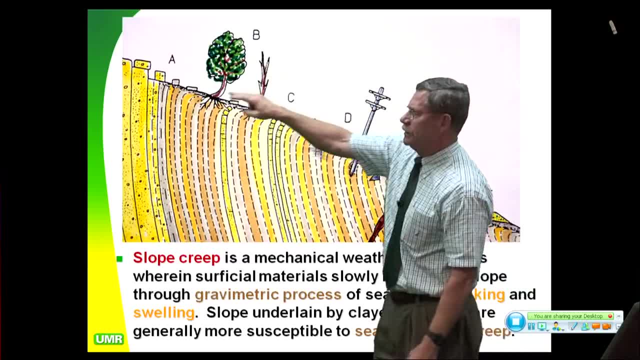 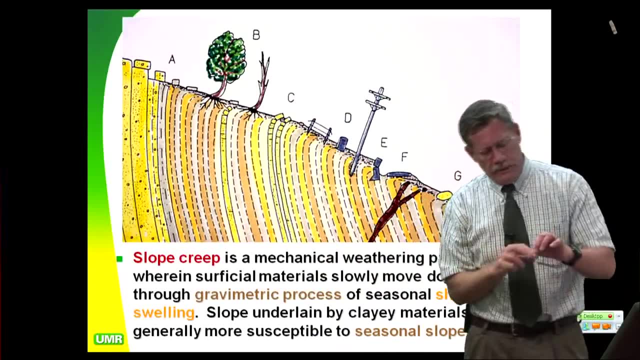 You'll see things like butt-bowed trees. Those are easy to back out. What do you mean? easy, Rogers? Well, they're easy. You can actually, you know, go get a Black & Decker drill. You can get the little coring thing. 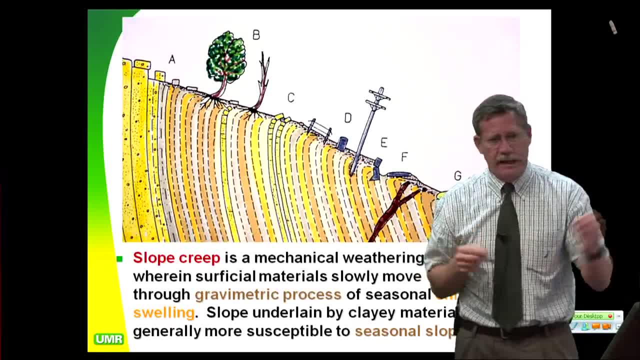 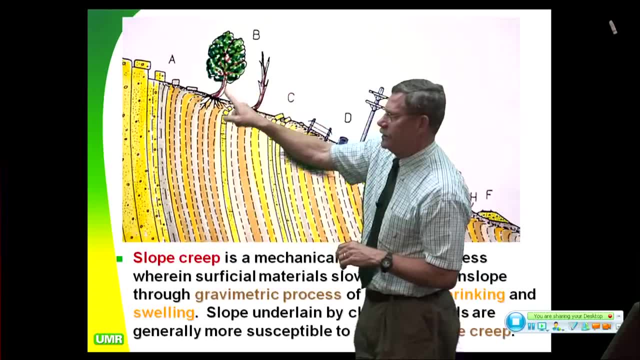 Drill a little tiny one-eighth inch diameter hole, Get the age of the tree, like that Doesn't take half an hour. And then, from the age of the tree and dropping a plumb line right down this major the offset, get some idea of the surficial creep. 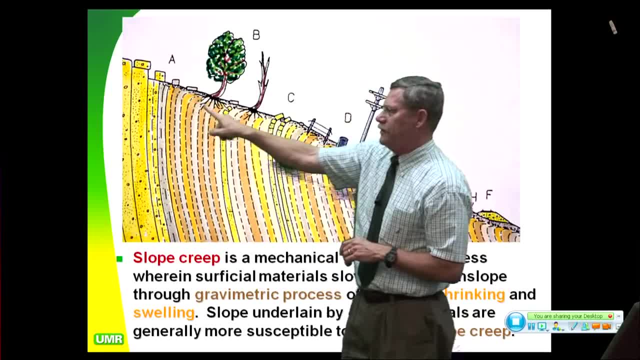 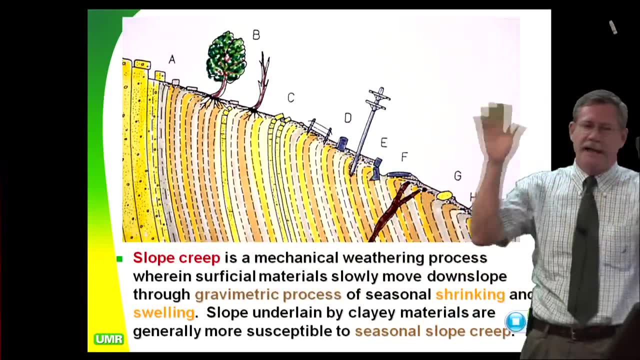 Now, here again, you have to apply the depth of the rooted zone. You got to know something about botany. I had a tree expert that I used on lots and lots of my consultations. I learned stuff from him. Every year we engaged him. 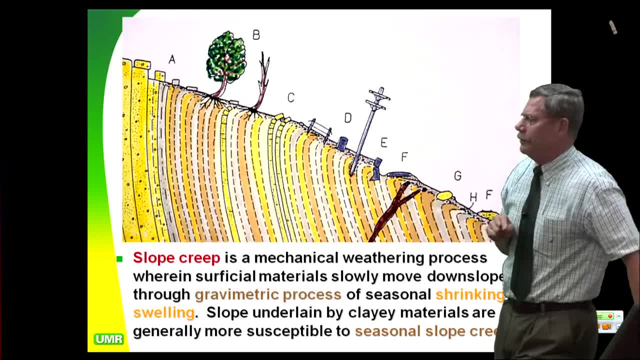 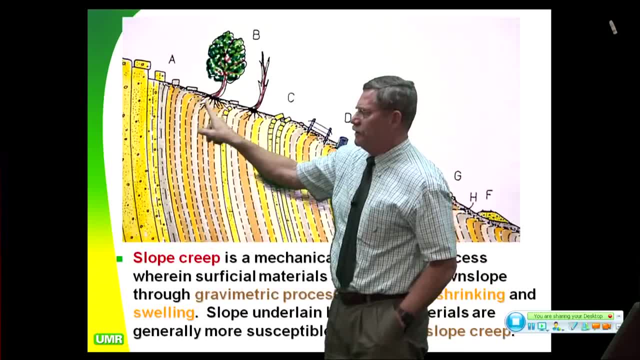 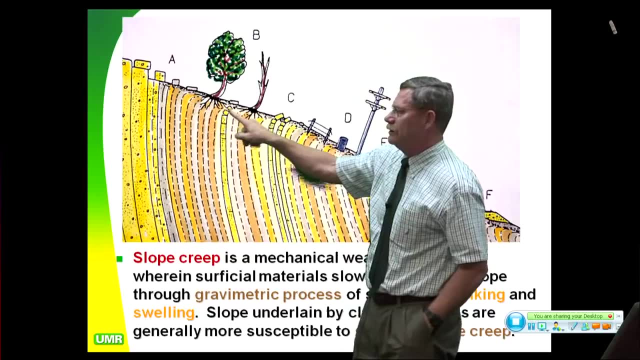 I learned new things. It was very valuable to spend the money, And so butt-bowed trees are an indication- Things like redwood trees. A redwood tree, you know. it will be 368 feet high And the root method is never greater than two meters down. 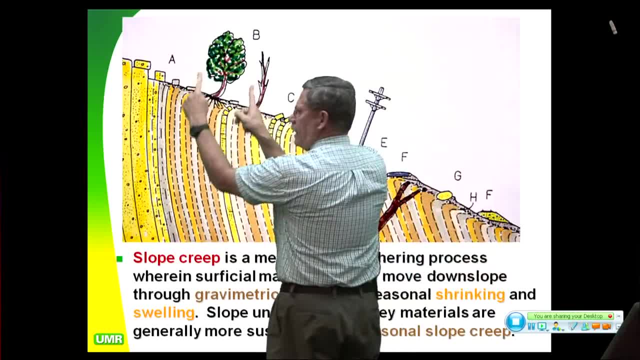 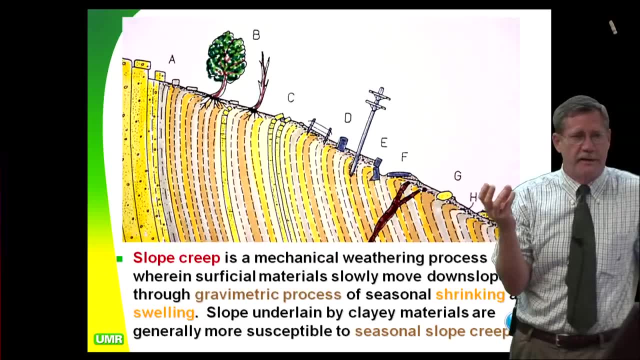 And it goes out, you know, like that, around the drip line of the tree, And a typical redwood tree will have 30,000 square feet of root cilia area. So it's out there sucking in 30,000 square feet. 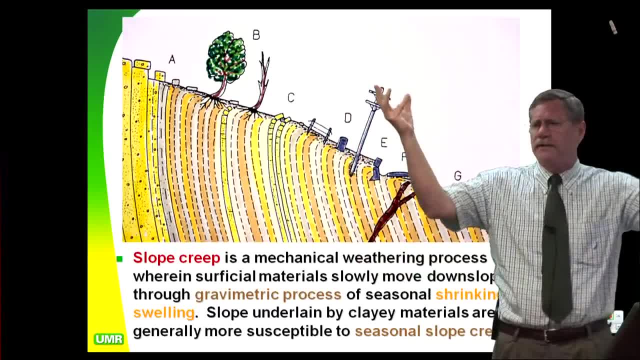 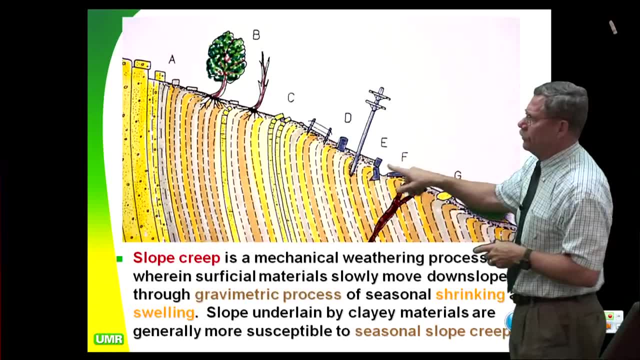 And it also absorbs water from the atmosphere, from coastal fog in the summertime. That's how they grow so big. So you want to be looking at all these different things. You want to be looking at old retaining walls. This is an old marble orchard. 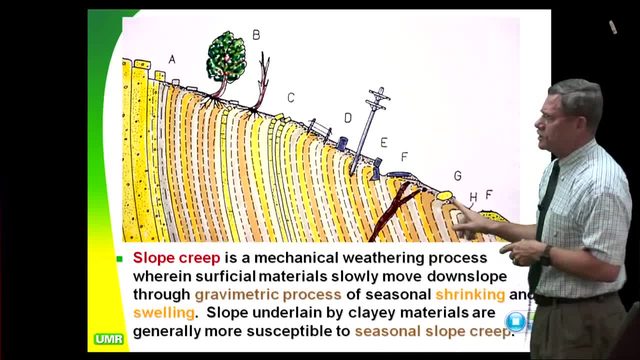 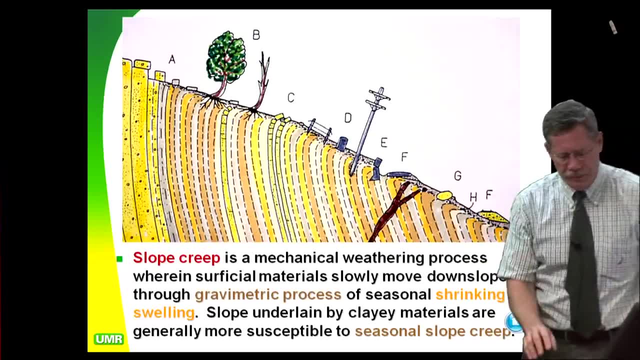 That's a headstone, and old fences, old roads, railroad, right-of-ways. You want to look at all these things and just say, hey, how are these doing? How much have they moved since they were originally built? That's a good place to take a little short. 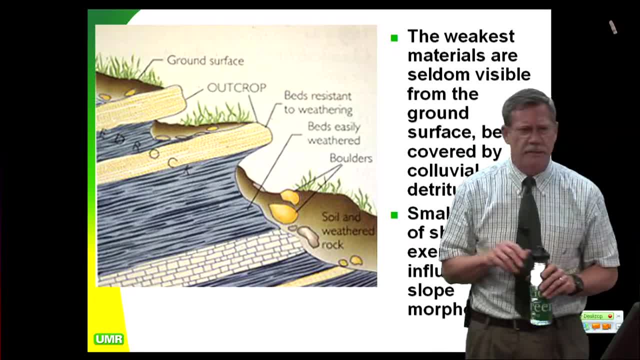 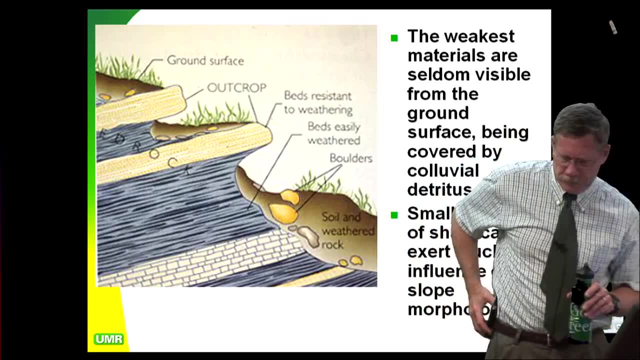 take a bathroom break. We got that's right 5 o'clock, So I'm going to take like a free four-minute break right now. If you want to go to the restroom, you can. We'll try and break it. 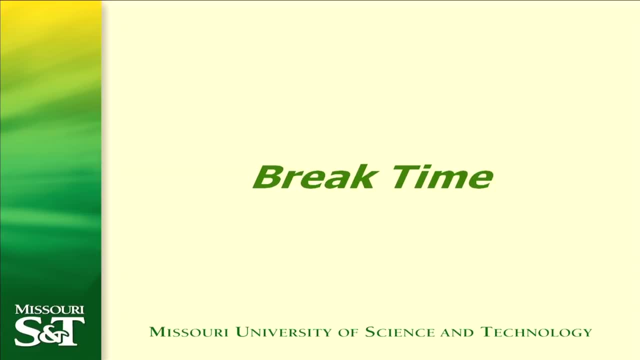 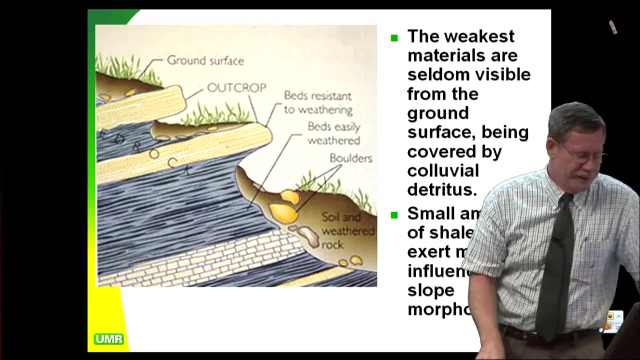 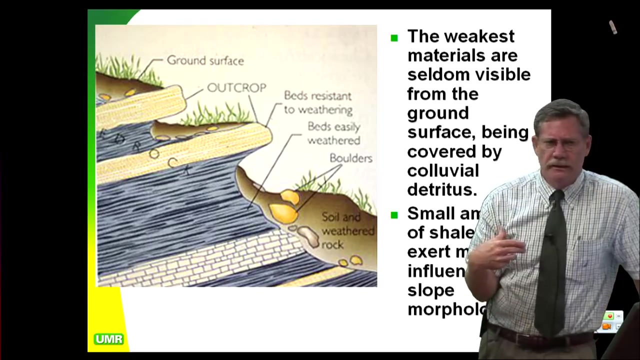 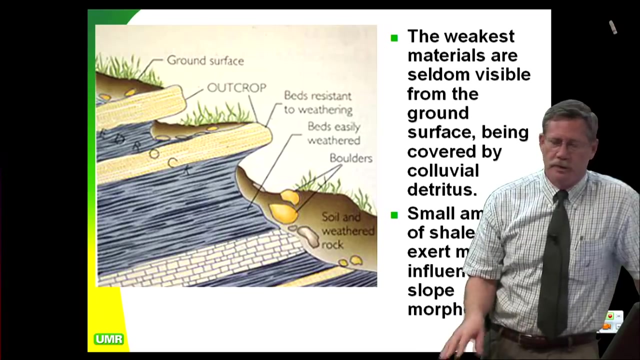 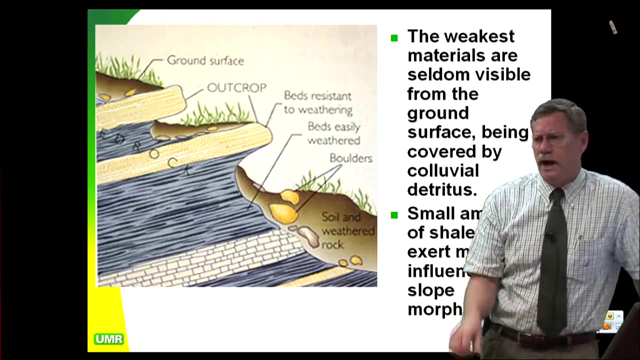 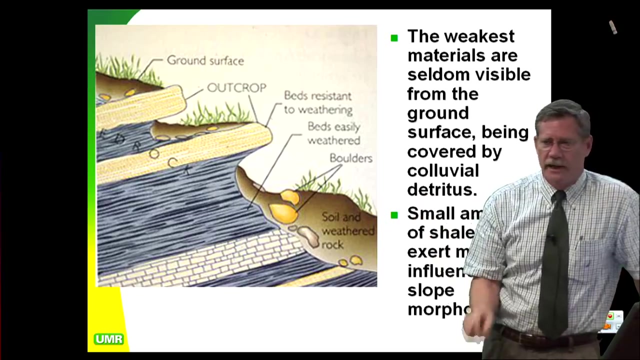 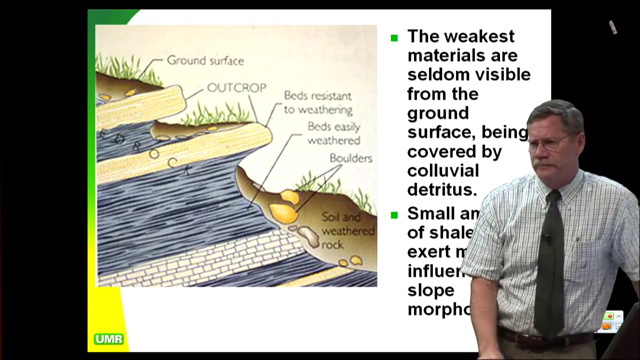 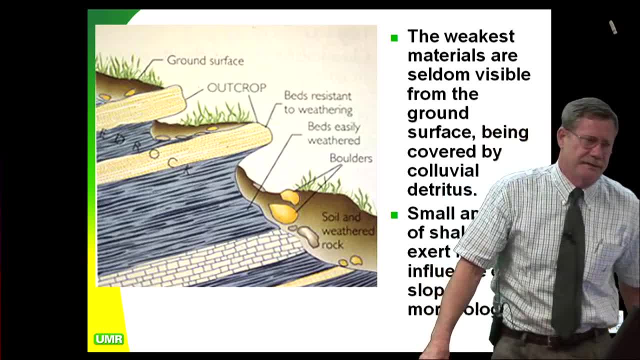 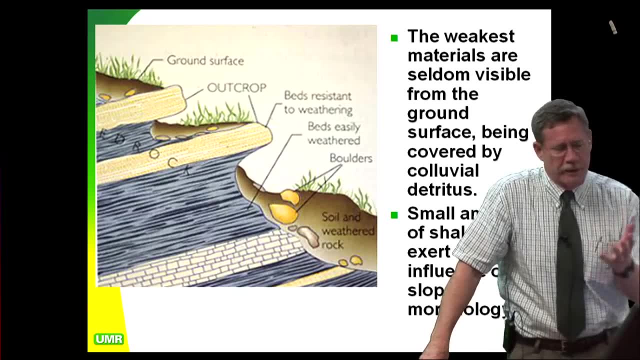 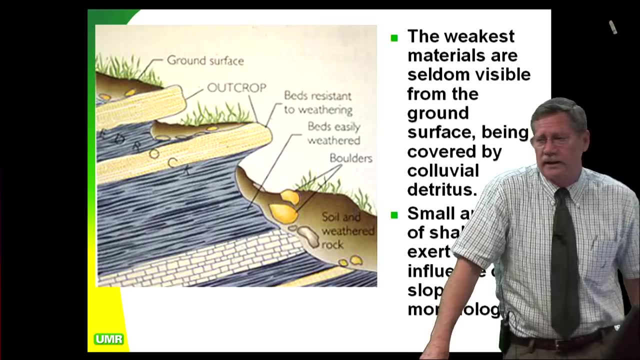 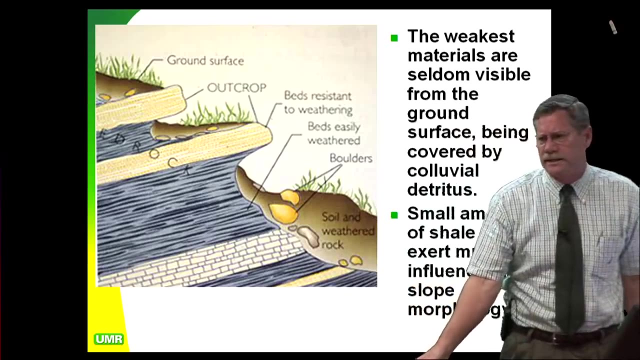 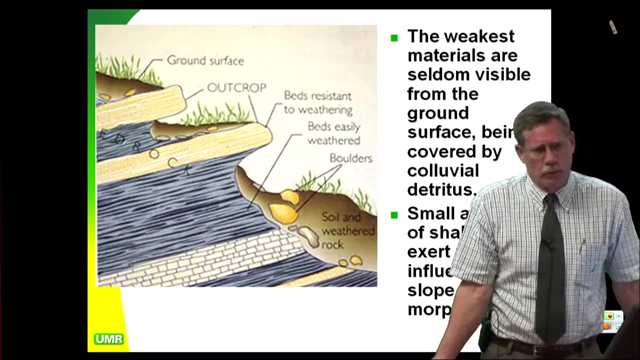 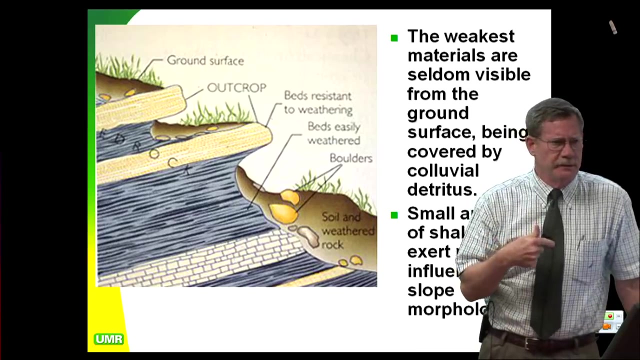 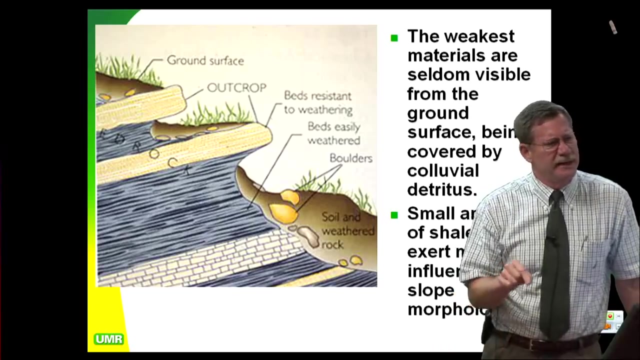 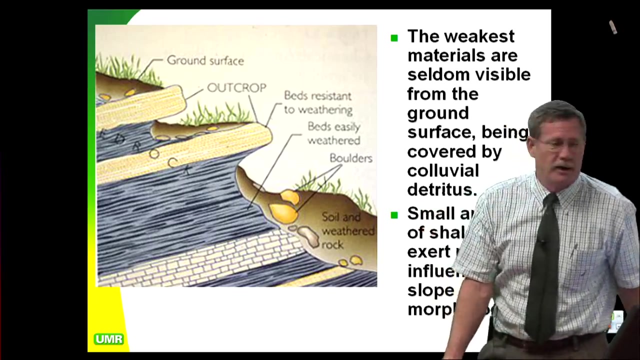 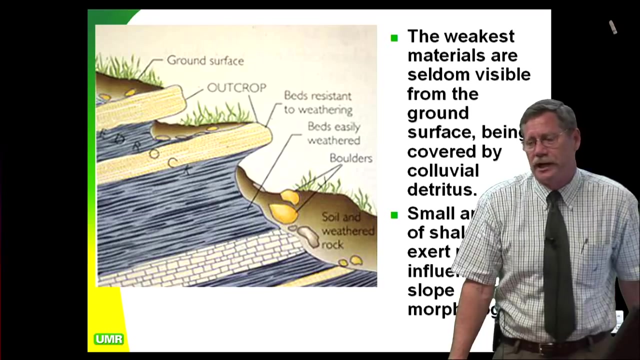 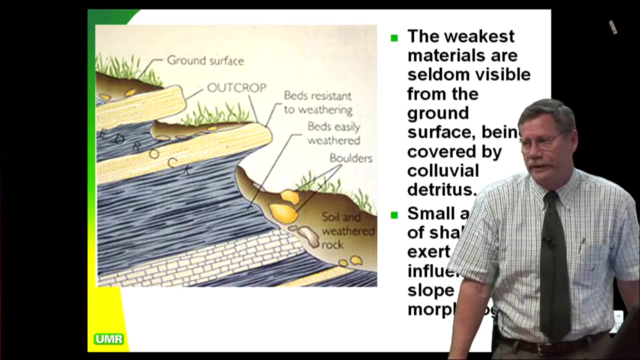 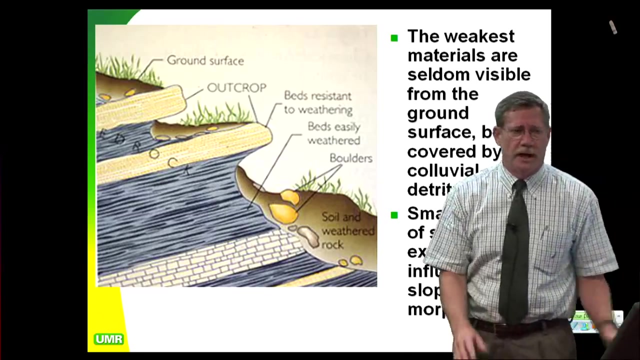 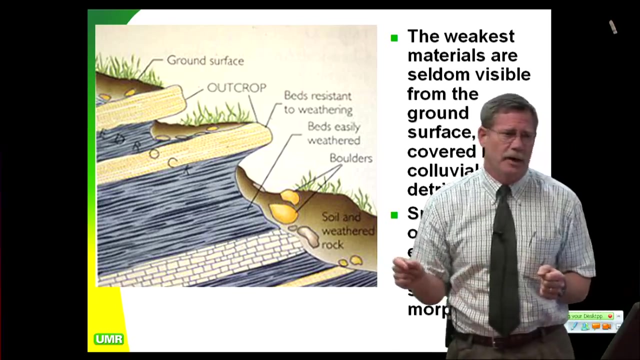 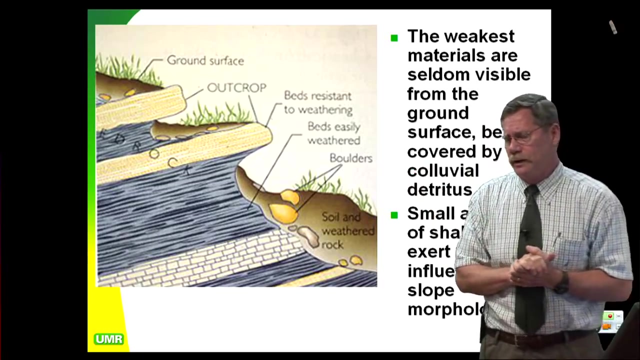 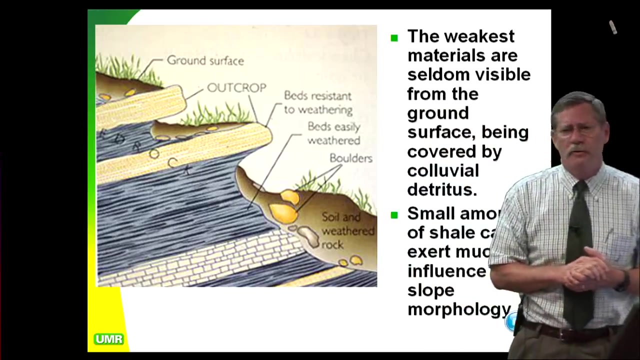 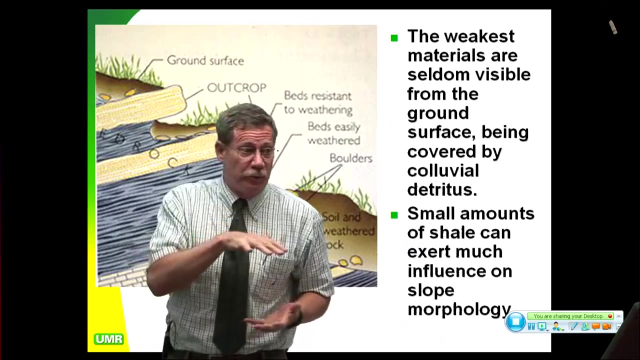 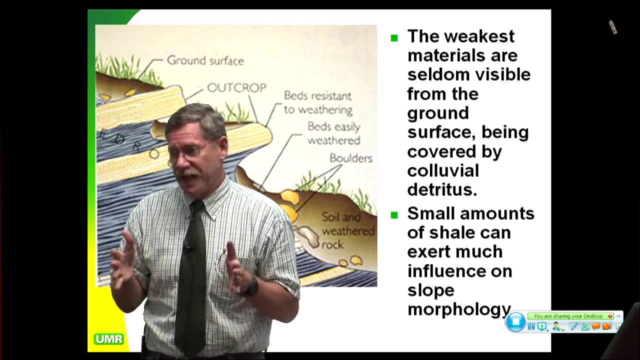 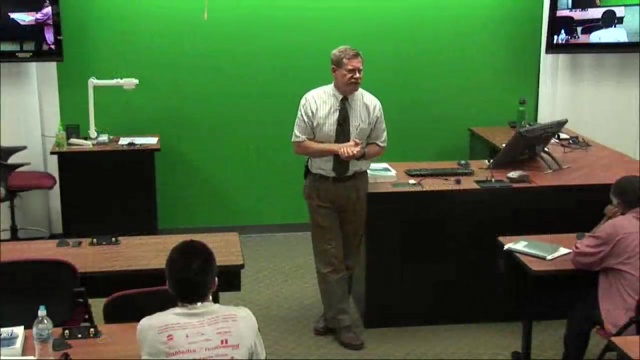 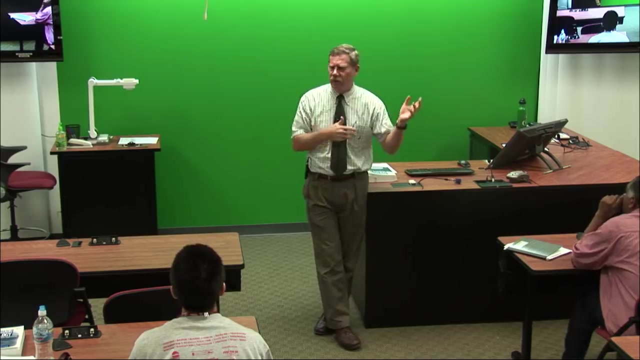 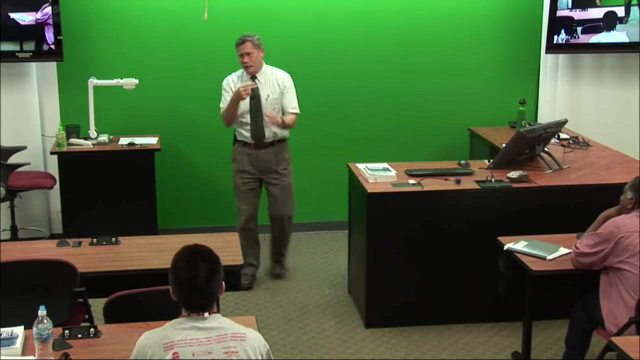 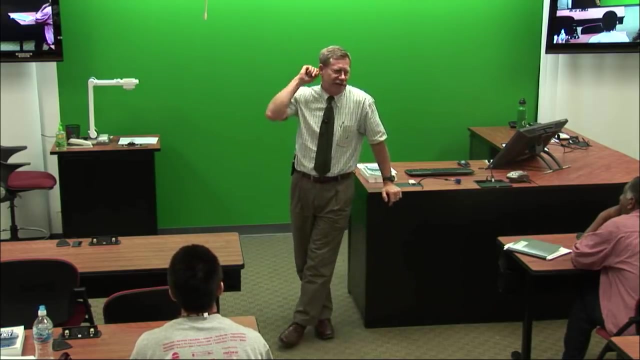 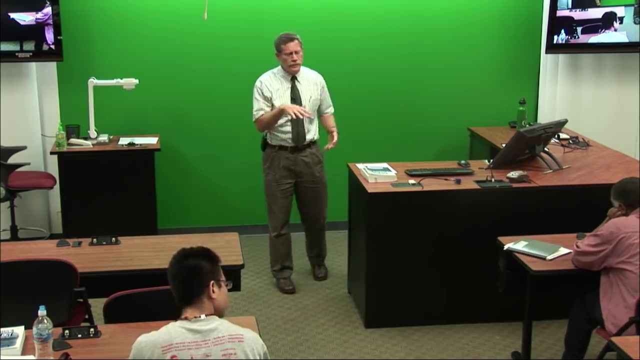 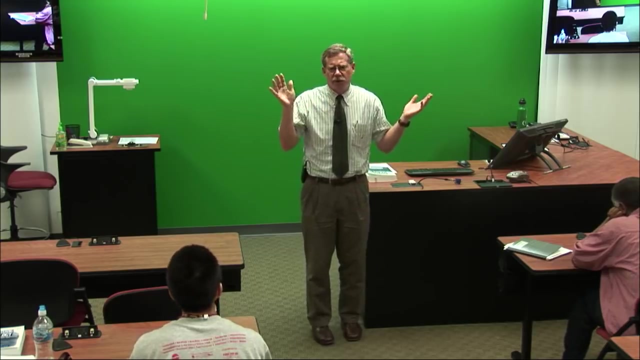 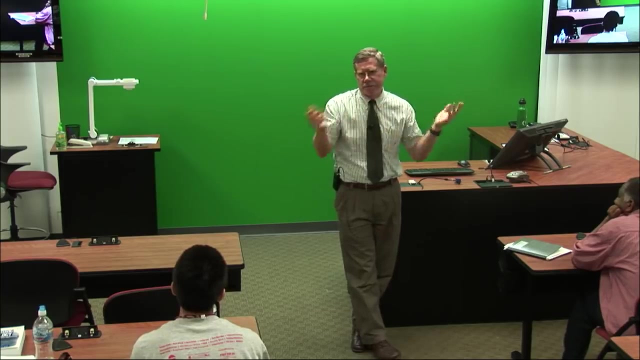 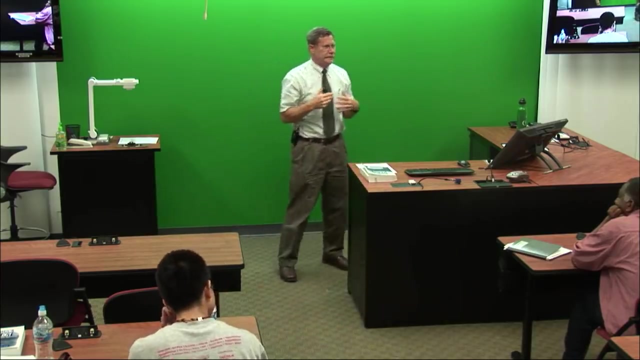 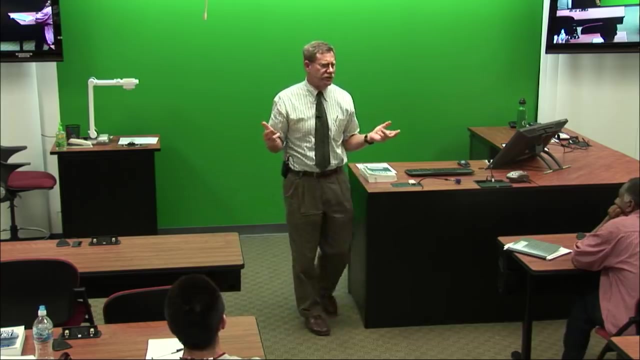 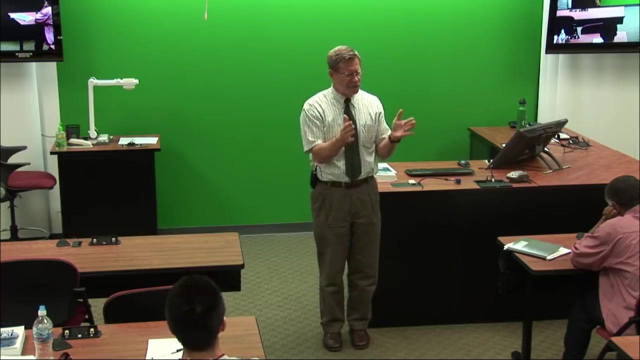 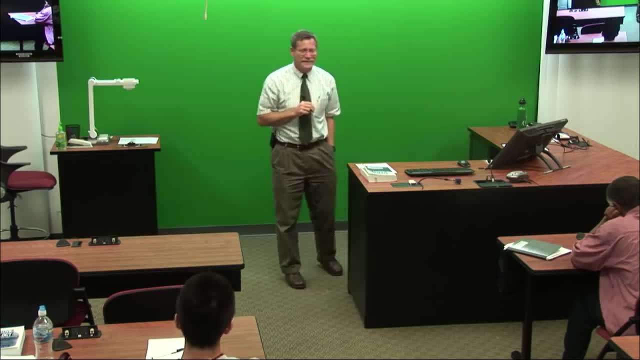 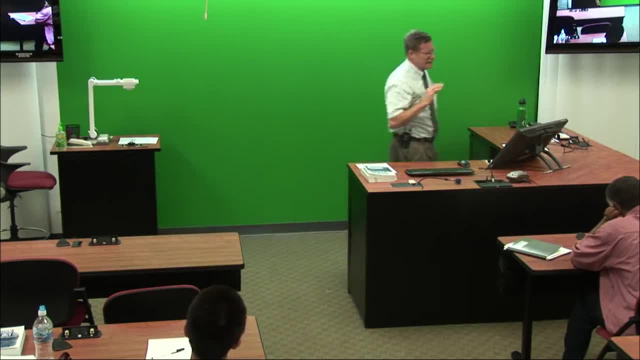 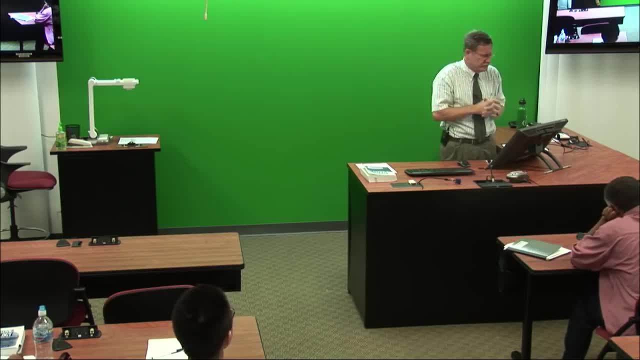 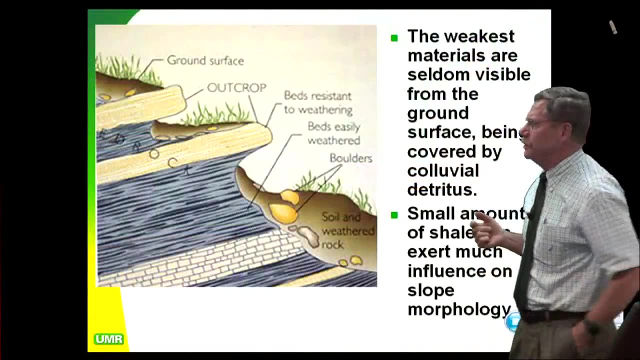 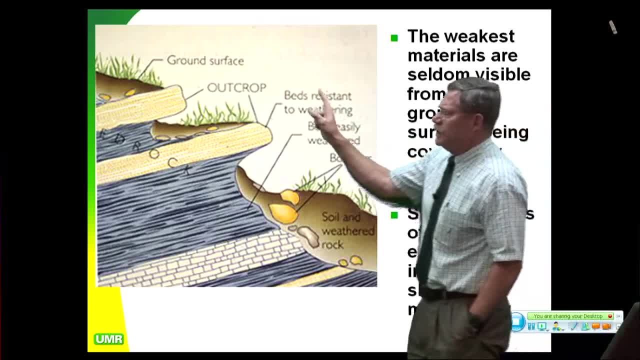 We'll be right back. You'll be right back. We'll be right back. You'll be right back. We'll be right back. We'll be right back. We'll be right back. Go ahead and grab this back. I hate the idea that this can't be doctored on the ground. 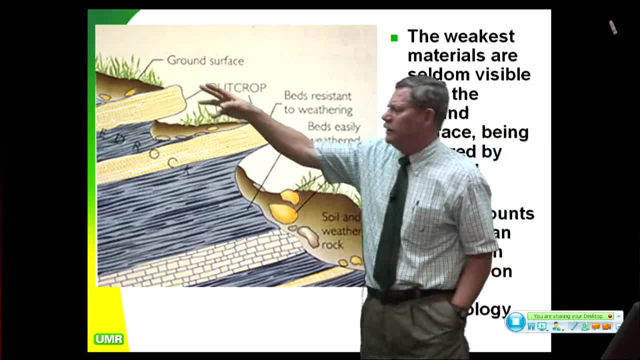 So I actually I know me a little bit better about this- How many people here have ever been through a situation, Or somebody who'd probably never been through a situation? We're going back down for a minute, So just wait a minute. 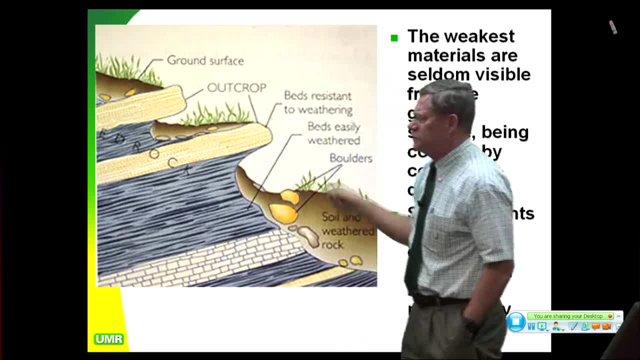 Why did you go through a situation like that? Where do you get all this MRP from? Anyway, kings and queens of a river, There's all those lakes and rivers and mud and stuff and water. The other come from a good day. 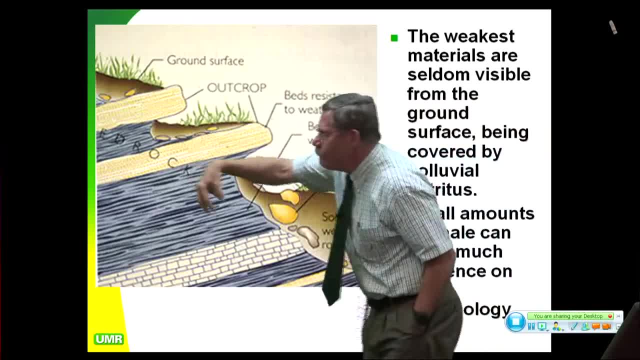 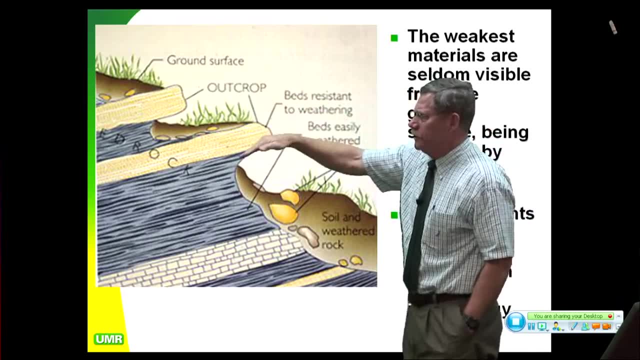 You get in there with a backhoe and go: hey, that's not sandstone, there's only a little bit of sandstone. That's the ledge rock that's creating the ridge, and there's all this stuff down here. What is this? 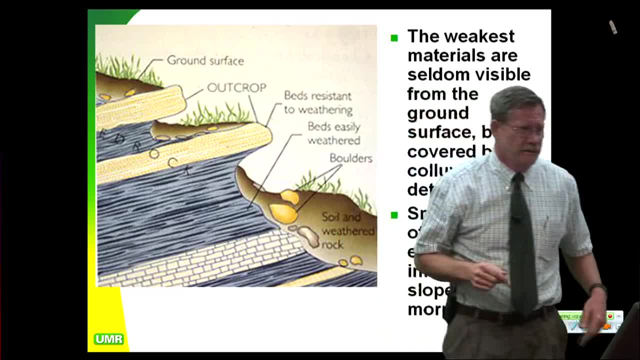 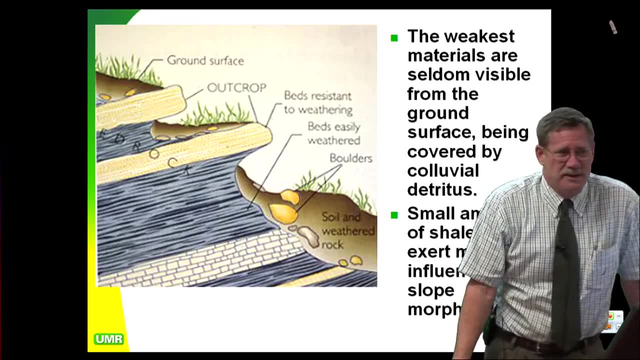 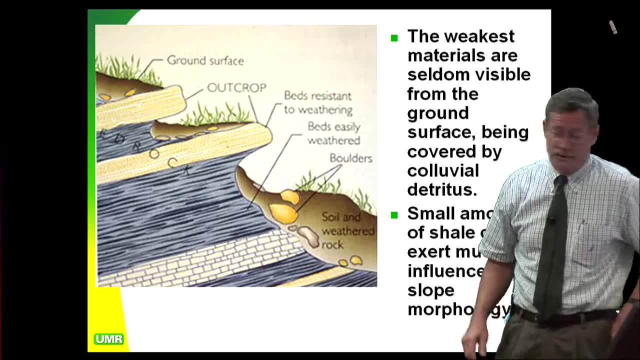 HIV, No shale. It's worse than HIV. shale Shale is bad doo-doo. All the world's geotechnical problems usually revolve around shales. That's why you need to take clay. mineralogy Shales have all kinds of characteristics. 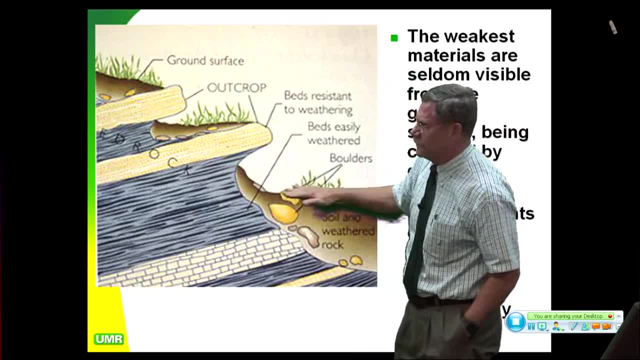 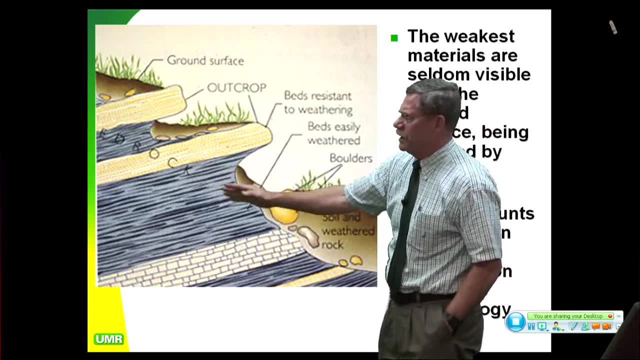 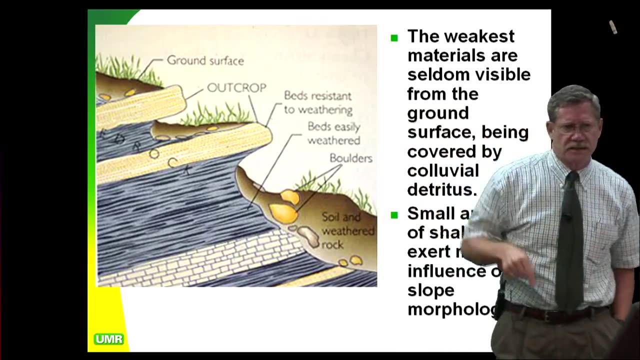 One of the worst is amount of weathering. If I have this protective cover on the shale right here, this colluvium, this slope wash right here, this protective covering will prevent this shale from continuing to ravel and swell outward, Because swell is a function of normal, effective stress. 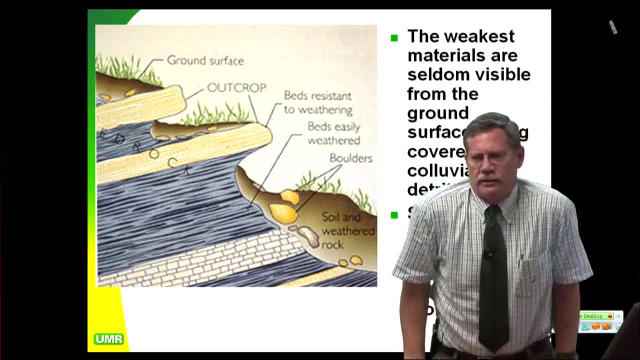 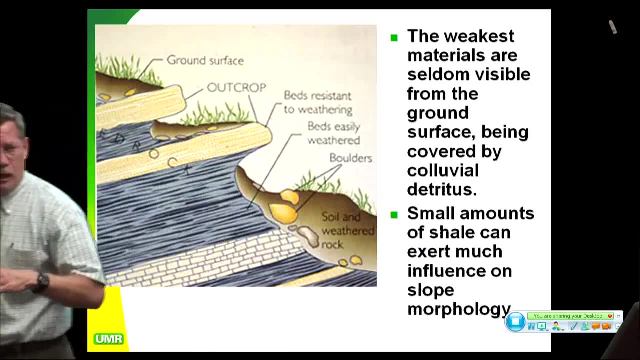 The more dead load I put on a swelling shale, the less trouble it gives me. That's why when I go to build an interstate, I put down four feet of rock. I don't put that there for drainage. I don't put that there to be the sub-base for the highway. 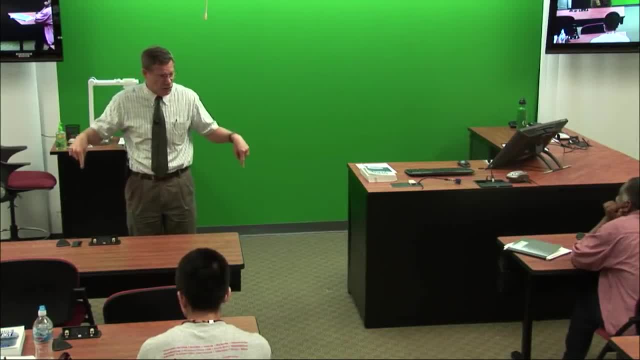 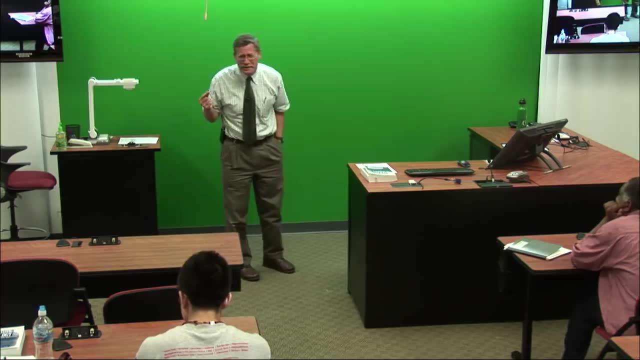 I put it there to be dead weight to hold the frickin' shale down. It's just dead weight to hold it down. A lot of geotechnical engineers don't understand that. believe it or not, They got through school somehow and didn't get that part. 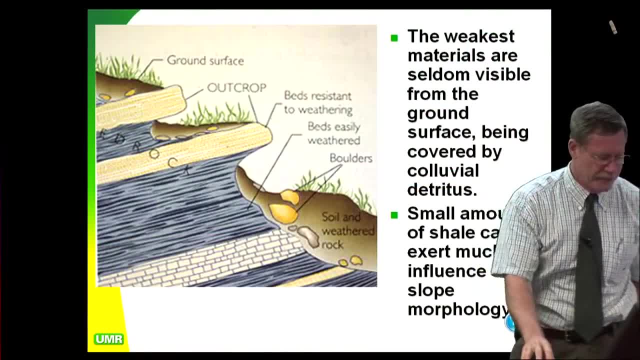 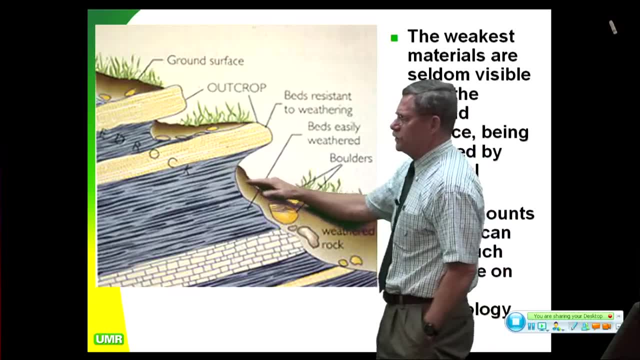 So it's not there for bearing, it's there to hold it down. So here you could be doing fine here, and then when you come in here and you clean this slope off, you take away this protective covering and you're going to start having trouble, right. 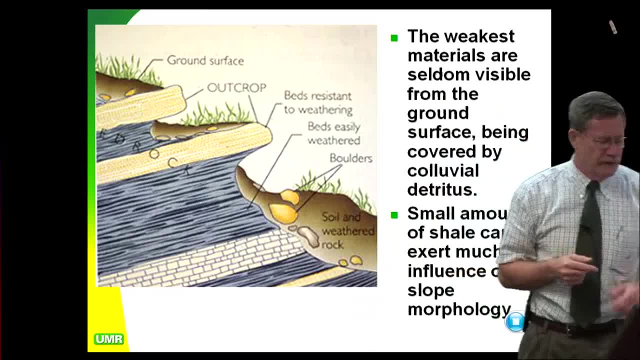 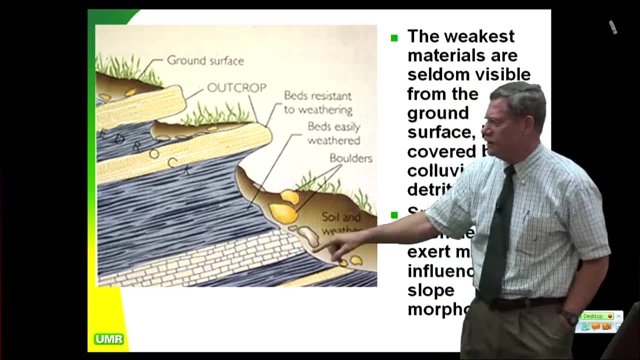 here. This is a real big problem. in places like Cincinnati They have lots of this kind of geology interbedded limestone shales and sand stringers. Sand stones are actually pretty thin, Limestones are pretty thick, But the shale controls everything. 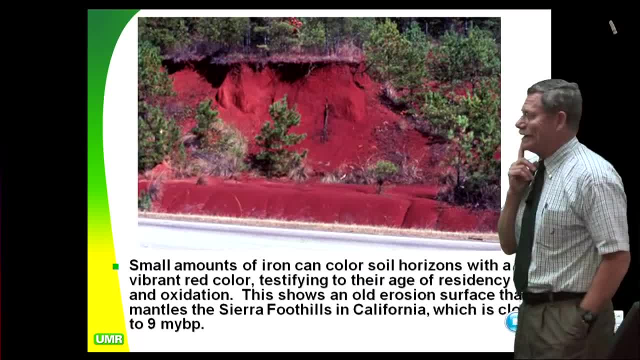 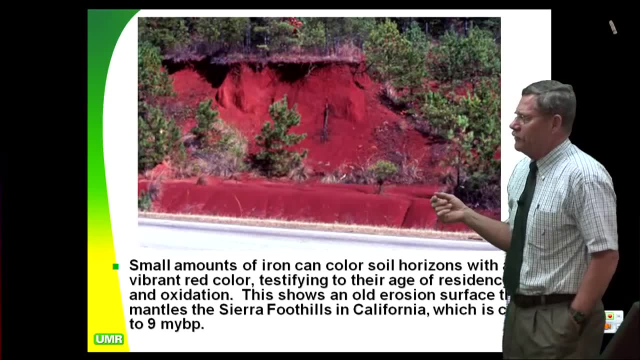 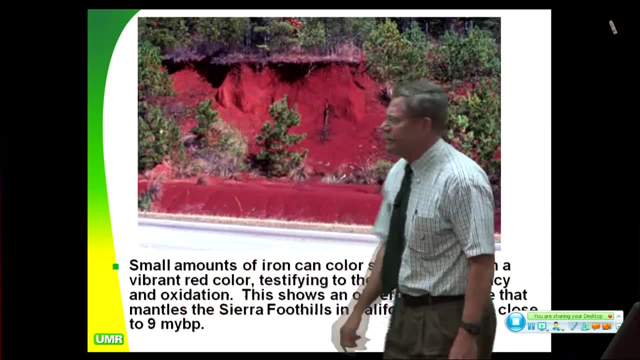 All right, small amounts of iron can color soil horizons. So here we are, in the Sierra foothills and we're looking at here is Merton Formation. It's about 9 million years old. That's what this NYBP Million Years Before Present. that's what that means, the geology. 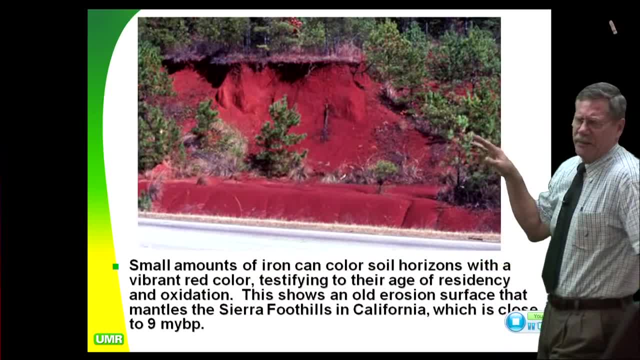 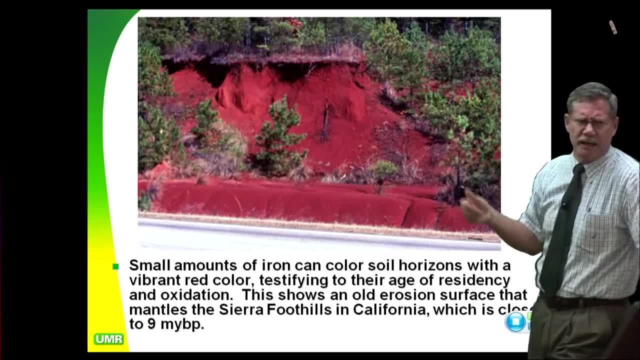 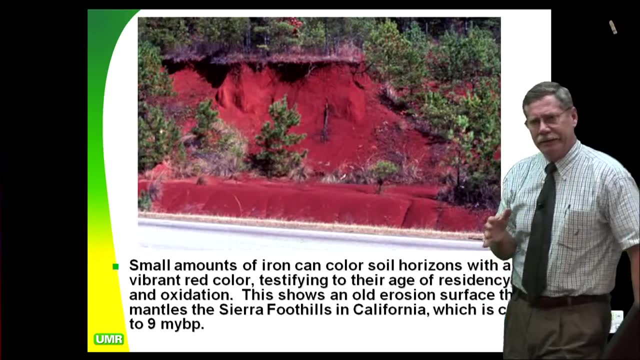 thing. Geologists sometimes just put that as MA. today MA means millions of years before present, K little a means thousands of years before present. So 11,000 or 11 ka 11,000 is the Pleistocene-Holocene transition, which came on about 11,000 years ago in temperate. 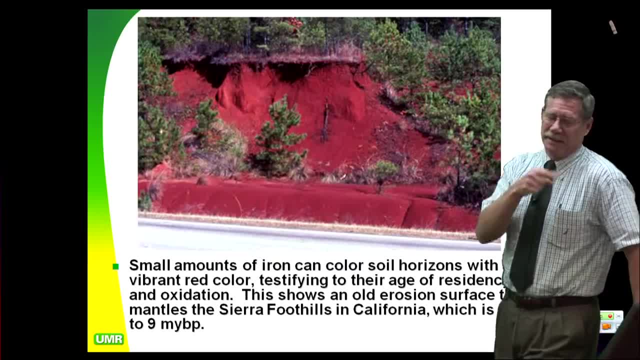 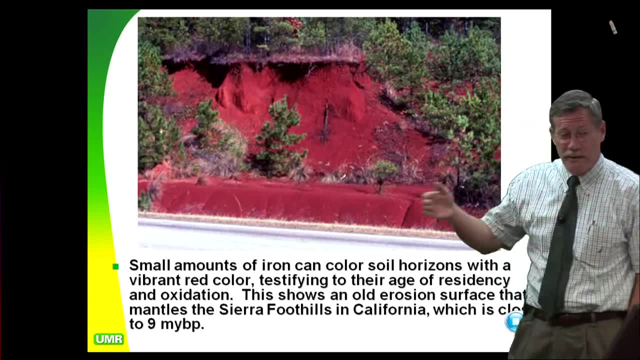 North America The Ice Age actually started ending 14,500 years ago, But in this part of the world it got here around 11,000 years ago. So it depends where you are really where the Pleistocene-Holocene transition is. 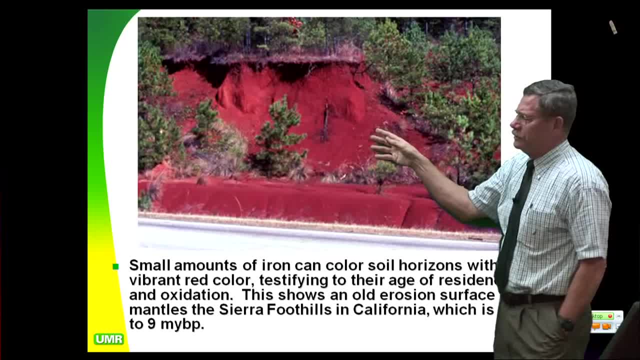 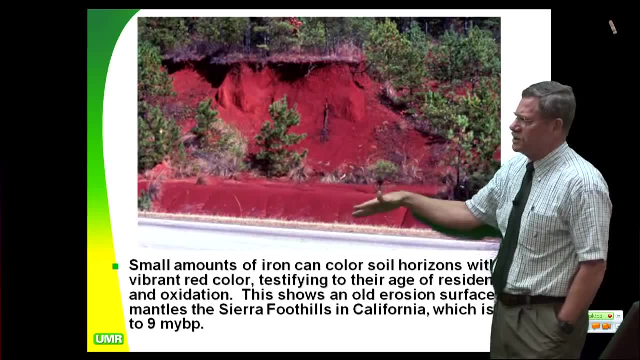 But here you see just a little. you have a sub-aerial weathering here with a sub-humid environment. It's getting drier and drier. over the last 11,000 years- This is 9 million years ago- this material 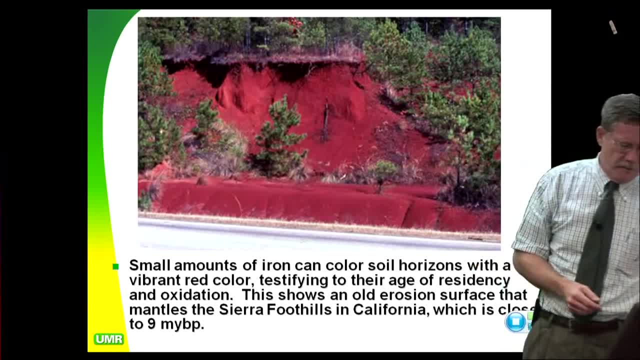 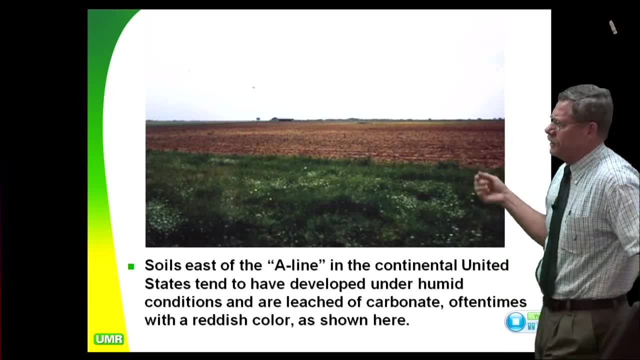 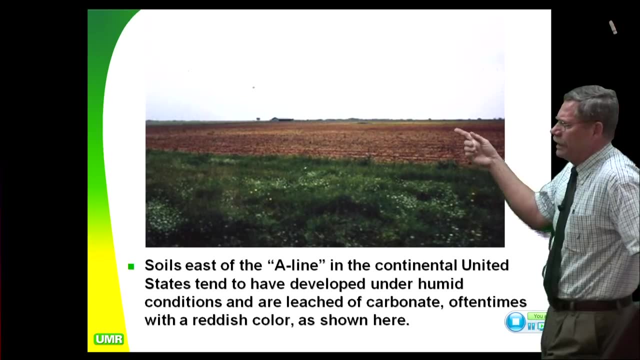 And so you color it very, very red from all the iron- Very little iron to actually color soil red. Here's a typical. this is at Johnson Lyndon Johnson's Ranch down in Johnson City west of Austin, about 90 miles or so, 80,, 60 miles. 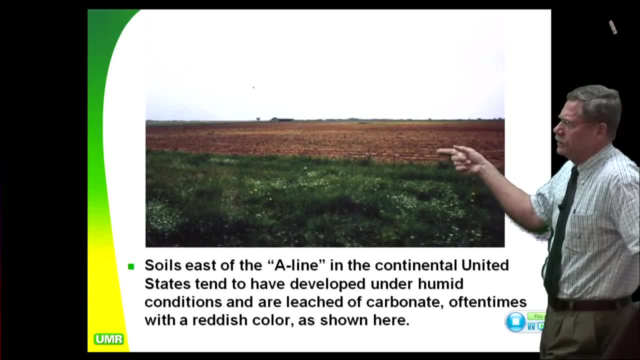 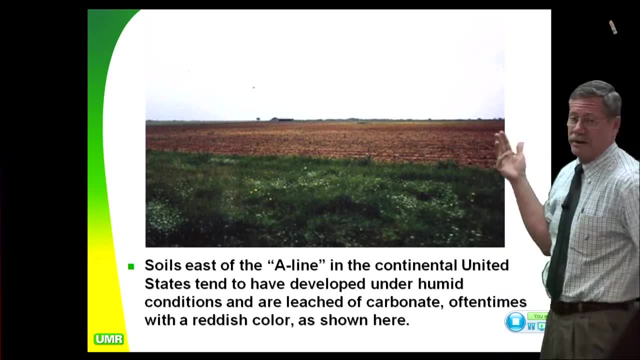 And here you see the red soils east of the A-line. So that's a typical. I'm just east of the A-line. I get out to Fredericksburg, about 20, 30 miles west of here, where Admiral Nimitz was. 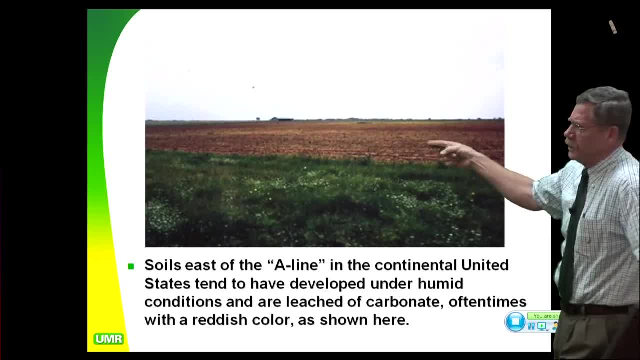 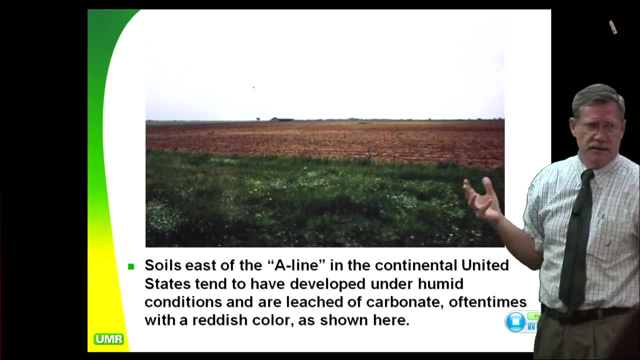 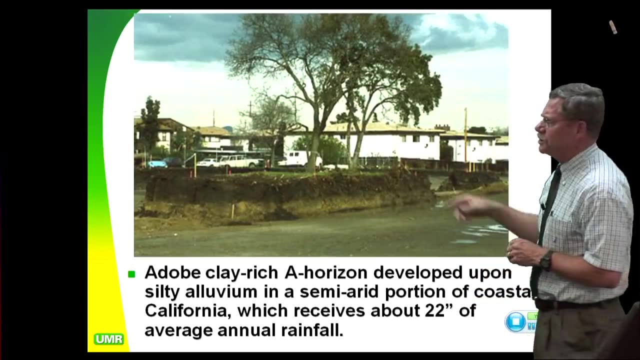 from and boom, I cross the A-line. I don't see red soils anymore. So the red soils go with humidity. They're in eastern Texas. Western Texas is carbonate-rich soils, with carbonate nodules more deserty environment. Here's an adobe-rich A horizon in Walnut Creek, California. 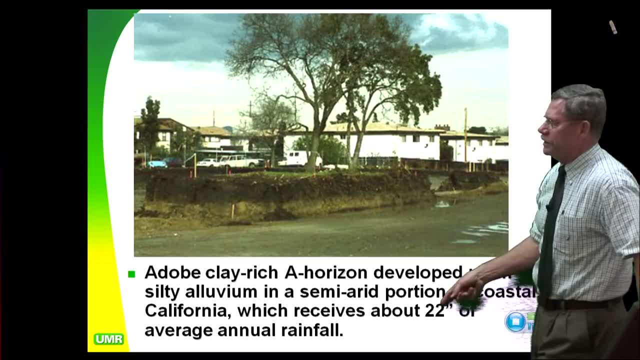 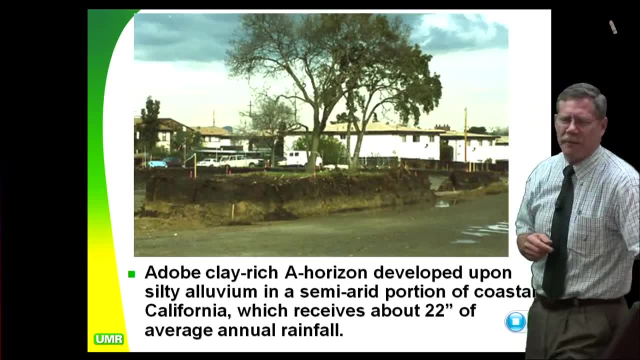 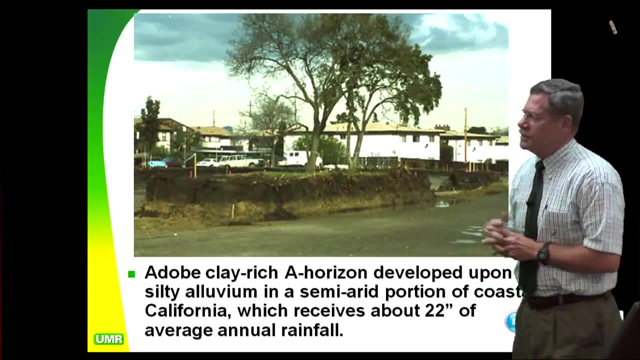 That's just east of Berkeley. This area gets about 22 inches of average rainfall And here you can see the soil horizons about 30 inches. That's pretty common, even around here in Rolla. Average A horizon thickness around here is about 30 inches. 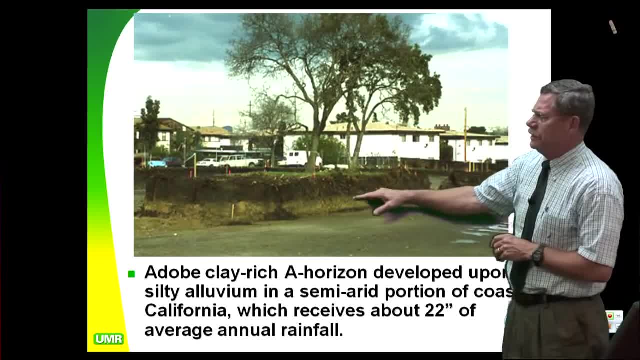 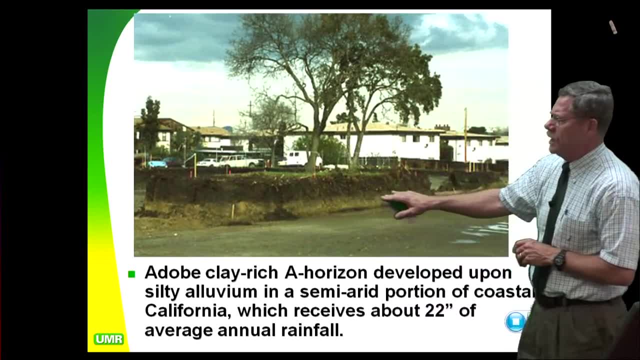 So 30 inches of highly plastic material. Below that we're in an argillic B horizon. This is actually the native alluvium right here. You see the native alluviums- Pretty nice stuff. The stuff above it has a lot more clay. 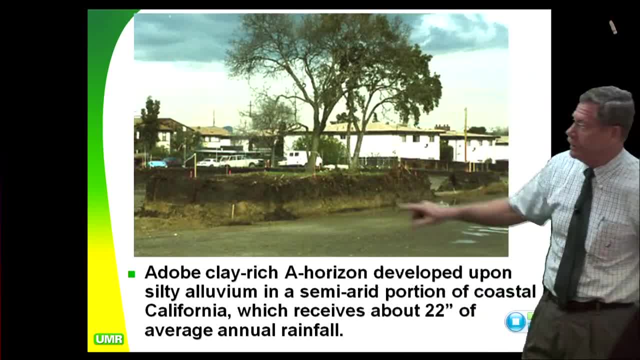 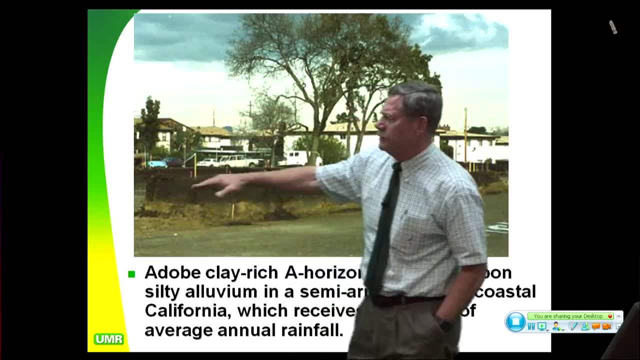 This is the native alluvium And a lot more reaction, And what you've got to watch out for in these areas is pockets. This drops down and you get a lot more of this bad stuff than you think you have. So what happens over here? this side of the building heaves a lot more than this side. 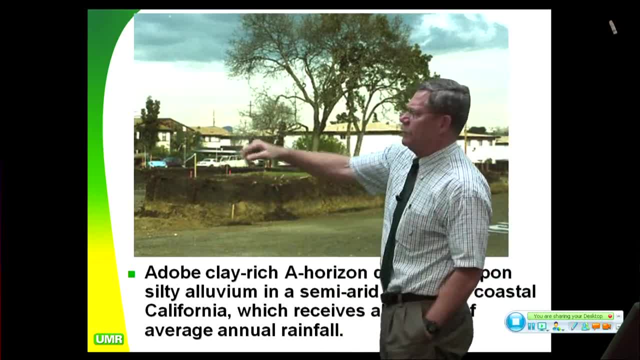 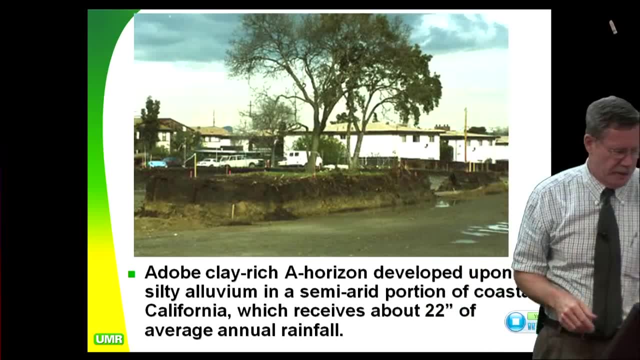 of the building over here And sometimes you heave a lot more. you break the pipes, You break the pipes, you add more water to the swelling clay and you're off to the liability. races Doesn't take long, All right. 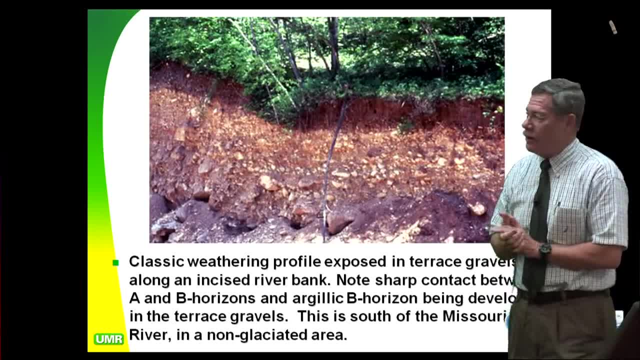 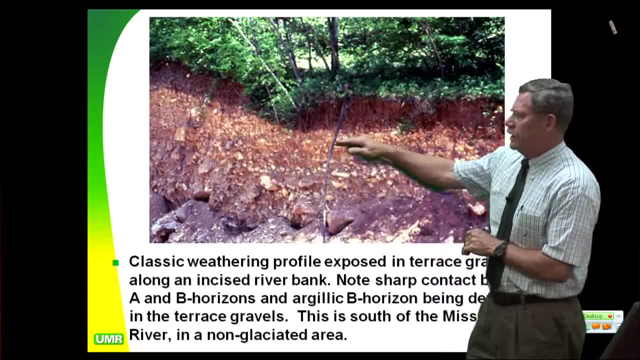 Here's actually a picture. This is actually right here in Missouri in the upper Merrimack River drainage over near Mansfield. This is by Scout Camp. I'm walking up the channel and I look over here and I've got a very, very well-developed 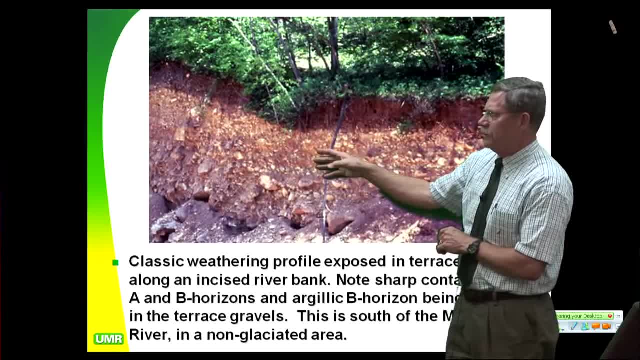 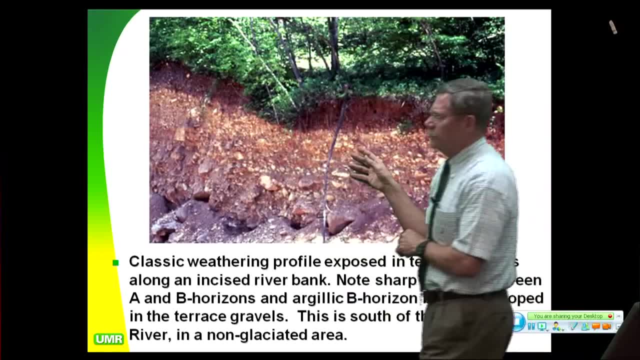 sharp contrast between my A horizon and my argillic B horizon. You know my argillic B horizon. you can actually see all this red, see that pinkish tinge. Those are the clays that are forming in river terrace gravels. 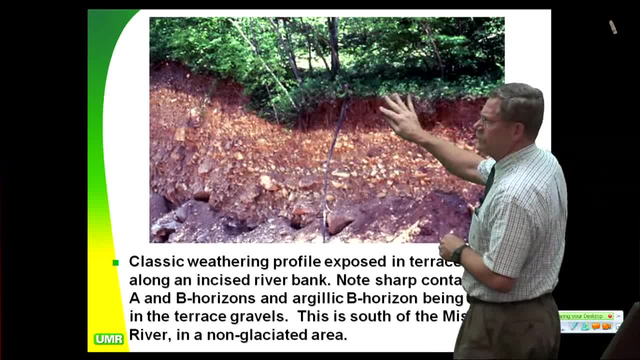 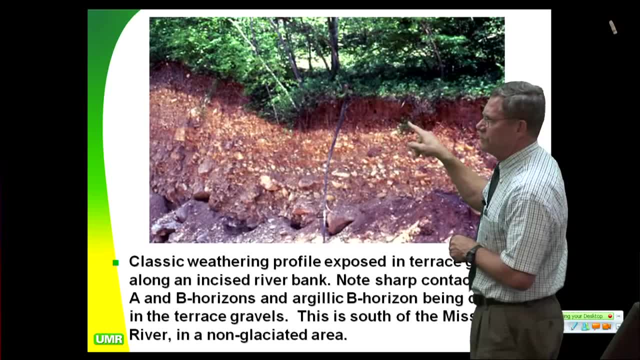 Terrace gravels And this stuff above them here is completely gone to clay. It's been there a long time. You can see things in there like gopher holes and burrows and stuff like that which helps get water and aeration in there. 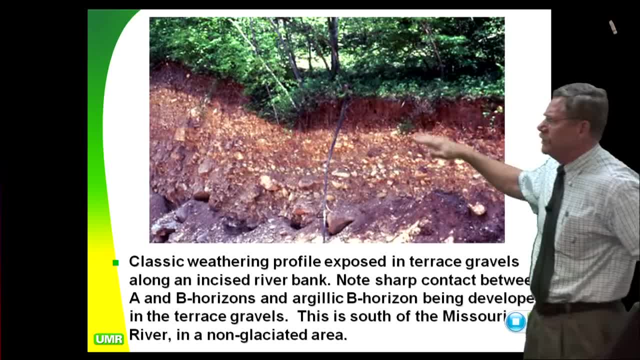 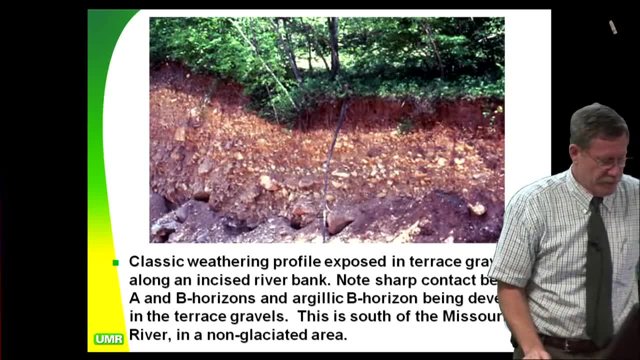 That's pretty typical of a non-glaciated area. If we were in a glaciated area, this would all be blown out of here. You don't see stuff like this north of the Ohio River or north of the Missouri River, except in the Wisconsin Dells, the area that got unglaciated. 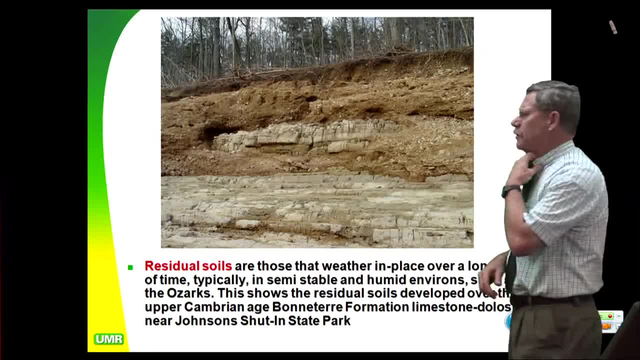 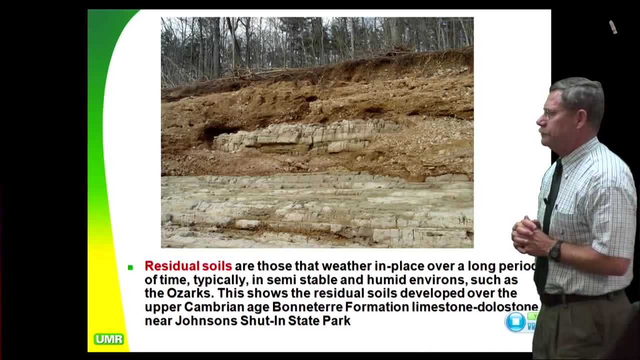 All right, Here we are in the Ozarks. This is over by the Tom Sock Dam failure, about 90 miles east-southeast of here, And we have here the Bontair Dolomite and you can see we have a very, very old colluvium. 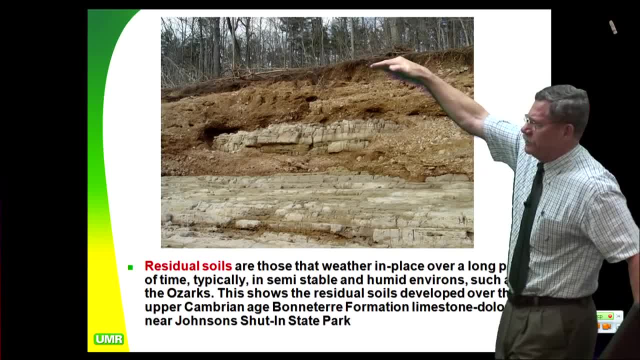 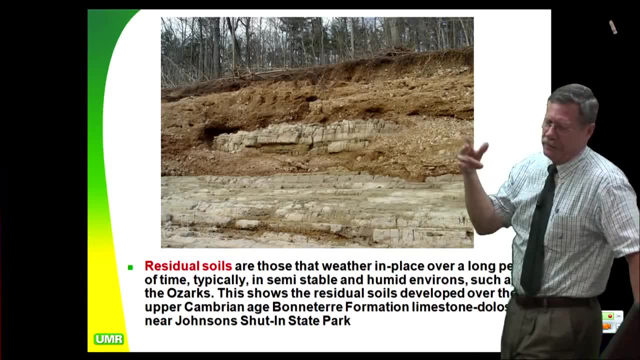 up here that has a very nice rooted A horizon. This colluvium's been there a long, long time, way longer than the Holocene. I don't know how old this is. It's been there a long, long time. 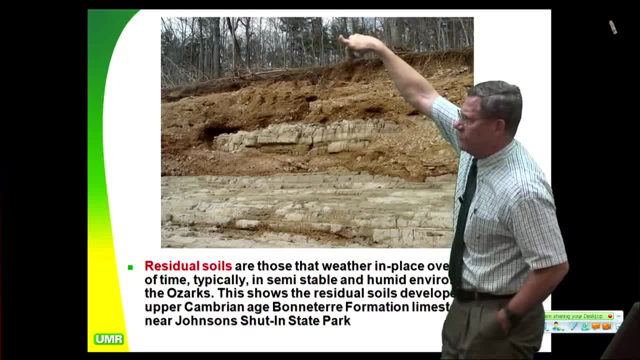 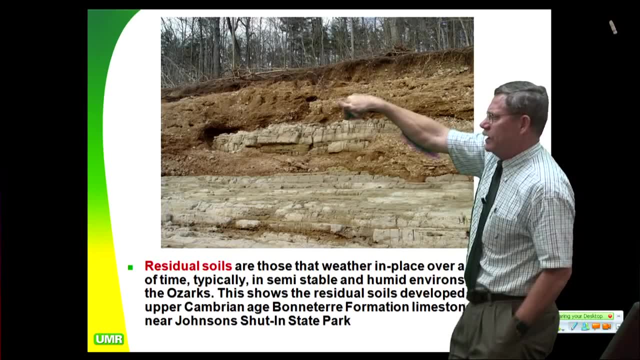 I don't know how old this is. It's really old. But now watch, If you do a boring ride here, come down bong. you hit bedrock Might as well. stop, Frank right, Go another six feet. 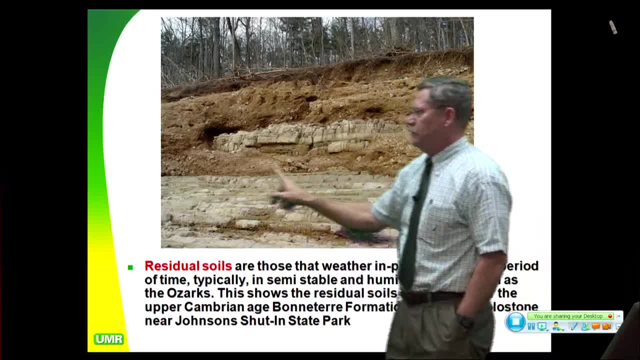 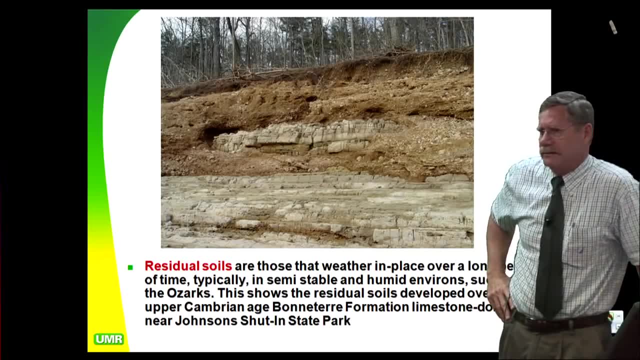 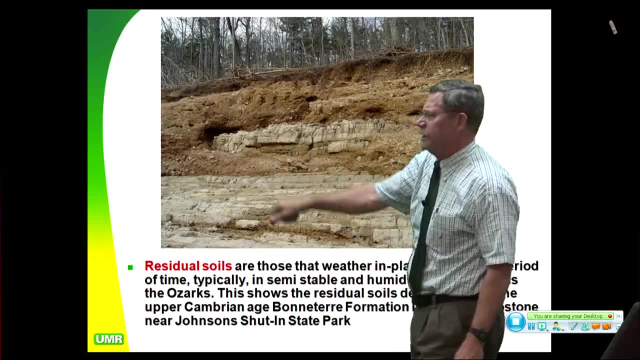 What's this? What's going on here? Old ancient Native American subway system. What is that? That's a filled cavern. That's a filled cavern, Got all filled up. See that All filled in. And so we keep going and then we get into more bedrock down here. 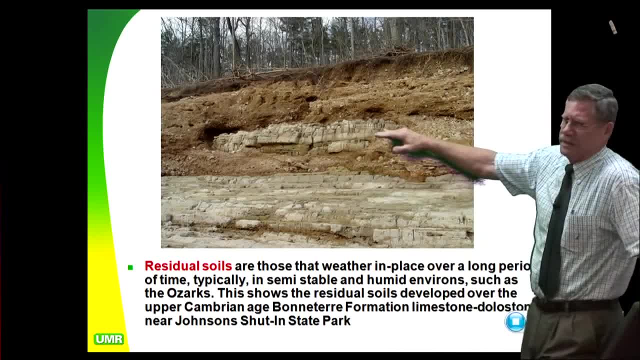 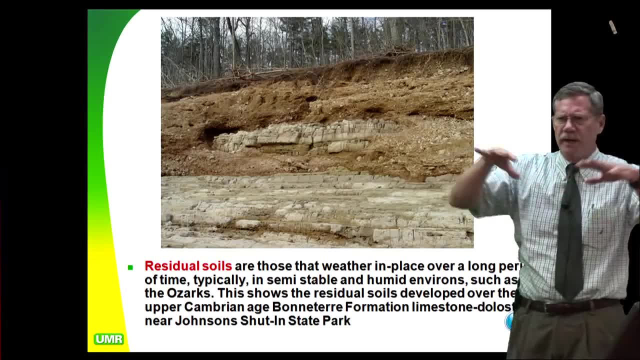 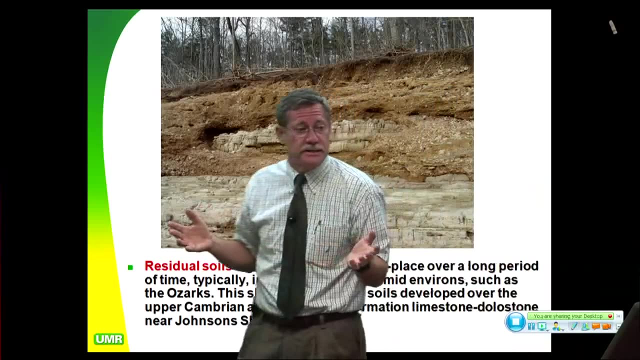 Now these things. unfortunately, that's about as simple a depiction as I can get for you. In reality, it's hideously more complicated, because caverns are the worst three-dimensional concavity structures on the planet. So when you're dealing in karst, which we are- 22% of the United States is on karst. 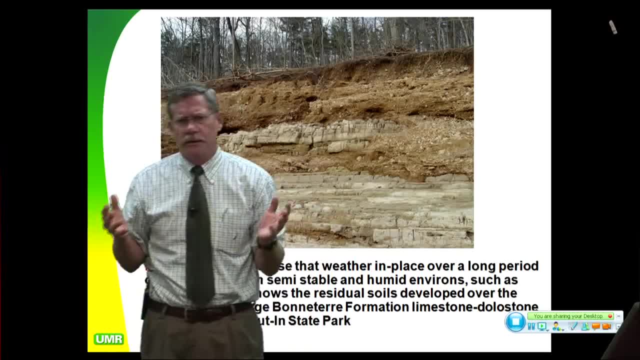 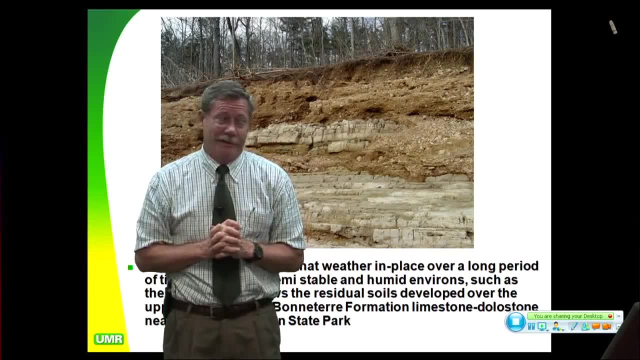 What does that mean? That's weathered carbonate rock. There's nothing more treacherous for foundations than building on karst. How many borings do you need? Oh, many more, As many as you can get When they were doing Disney World down there. to give you an idea, that's all karst. You know it's Florida, It's karst everywhere. How many borings did Dames and Moors Los Angeles office do down there? Each building had about 600 borings- 600? They Swiss cheesed it, yeah, because they had so many sinkholes. They had to know where the sinkholes were. They had to mitigate all the sinkholes, put in huge matte foundations. They were some of the most expensive foundations in the country back when that stuff was built Back in the 1970s. 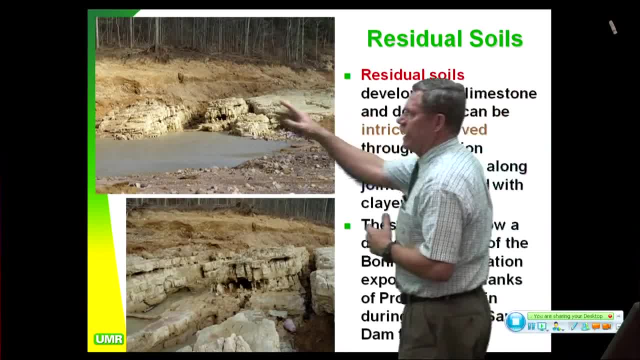 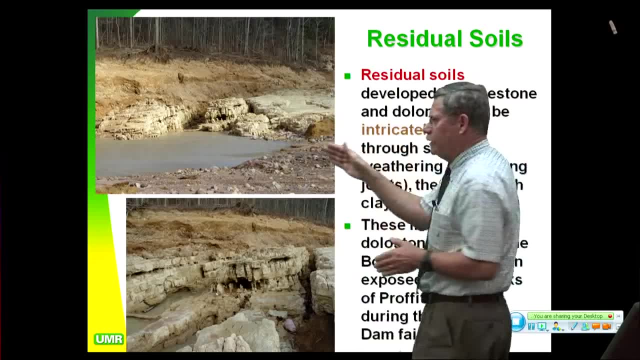 So here is the other problem. We're going to look in the other direction now And I was just showing you this stuff right up in here, exposed in the bank by the Tom Salk Dam flood. Now I'm going to turn and look and you can see these cavities sitting in here. 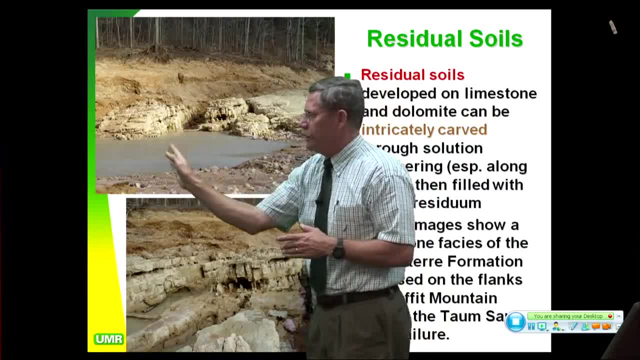 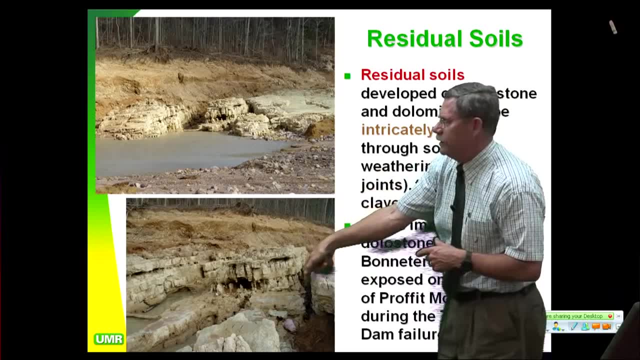 This is a joint line that's running along here. Here's a close-up of another joint line right in here and you can see if you drill the hole right down in there And through this thing you wouldn't get any rock, You'd just keep right on going because you're drilling right down the joint. 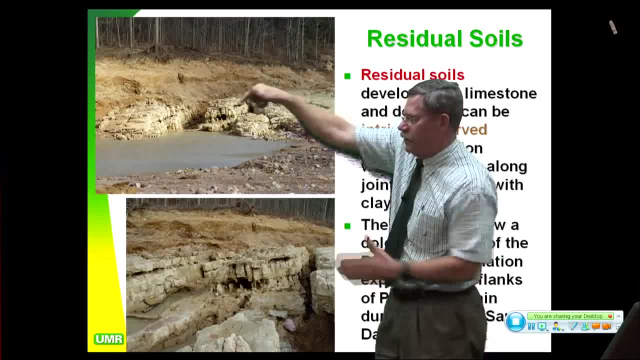 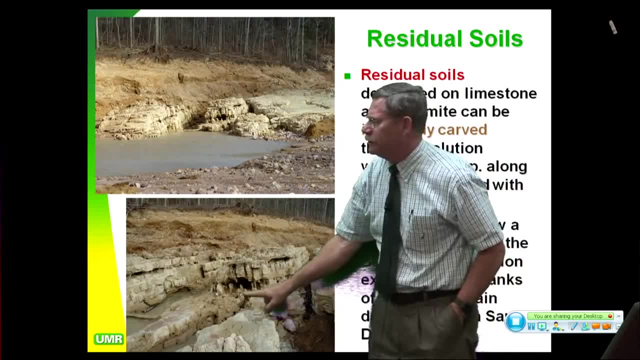 That'd be right same thing. right here You're drilling, right there, drilling right along these parallel joints. So in here you have some, actually some, demo cell structures. You actually have a bed in here that was more solutioned than the dolomite here. 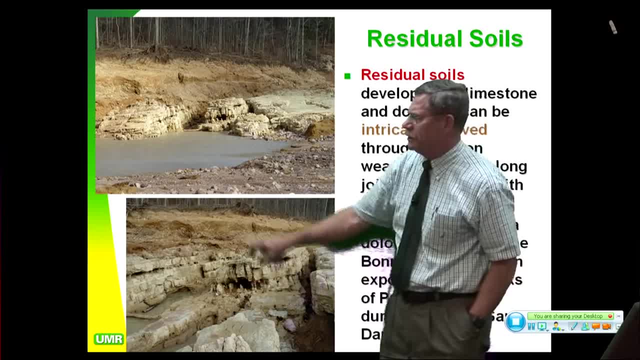 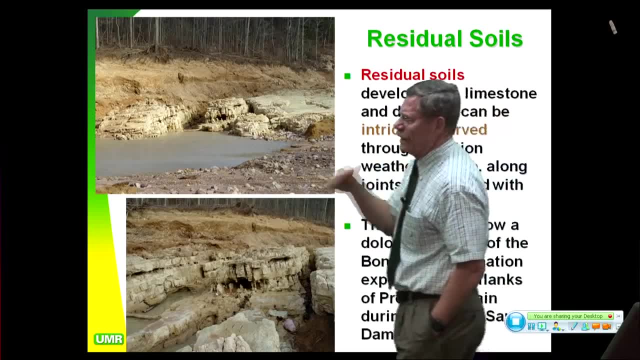 So this is a pure limestone. It's just gone And you can see here, if you were building a dam on this, which they try to build a lot of dams on things Like this, like Merrimack Dam, which is on my website if you want to read about it. 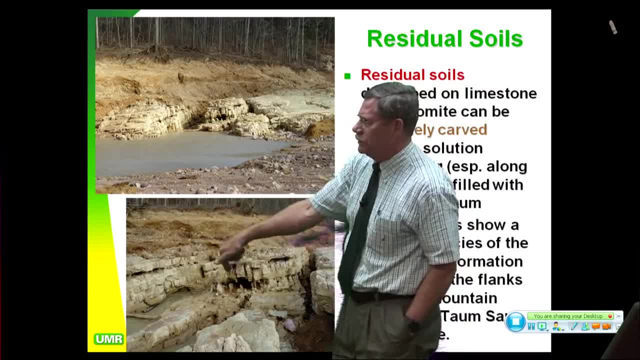 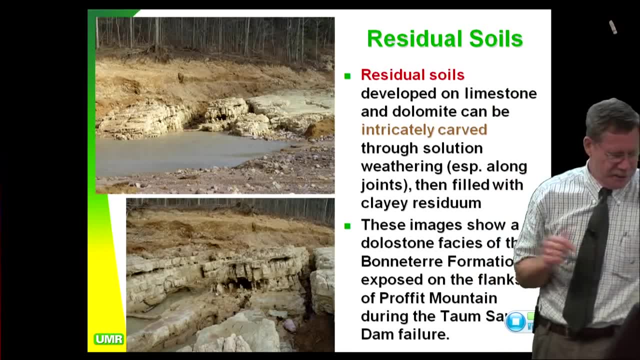 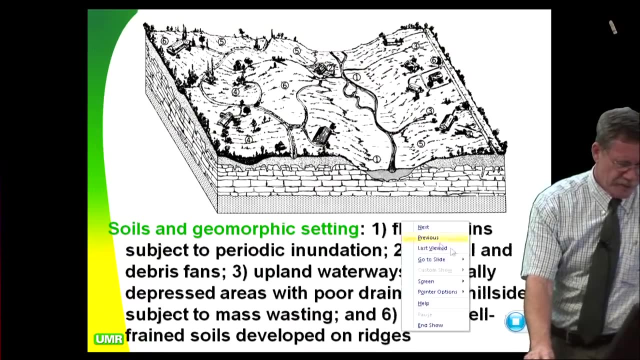 You get in here and you just start injecting grout and it's a grout contractor's pension plan. You never get done injecting grout in that kind of a foundation. It's just bad news. So let's go back one, excuse me. 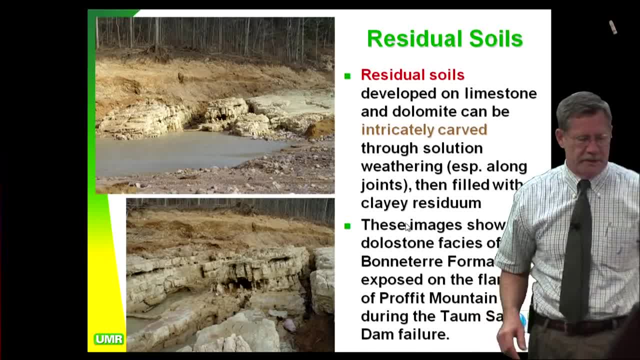 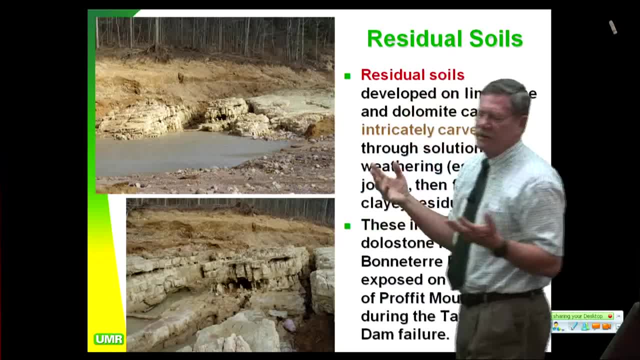 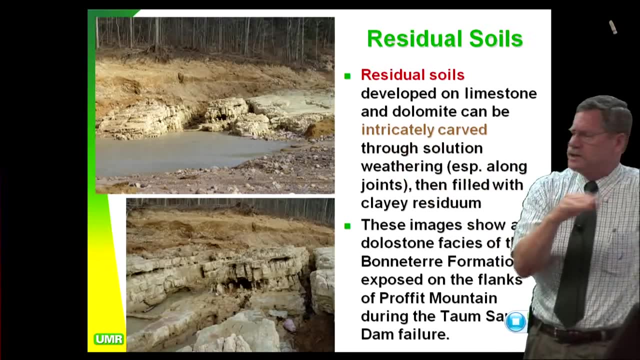 We call that residuum or residual soils. Residual soils have Weathered in place and they're very can be very, very complex And you really can't appreciate them until you gut out the site in three dimensions, like this, done by the flood. 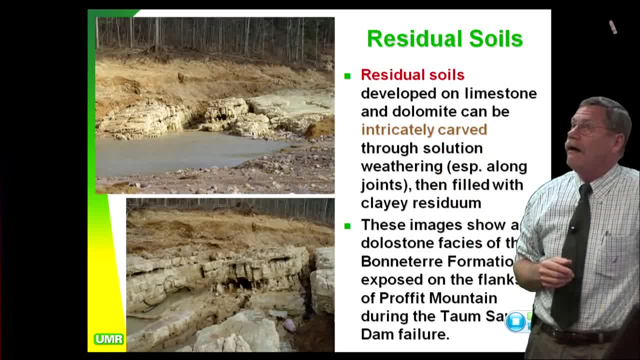 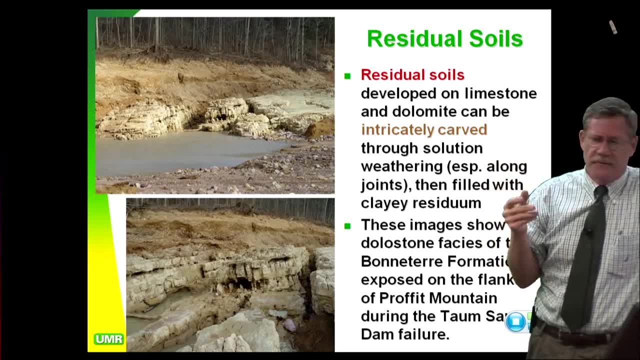 And you can look at all of it and you're going to go: uh, that's pretty complex, Yeah, very complex. So best thing to use in cars is geophysics. Geophysics is going to identify your anomalies. They're called those hot spots. 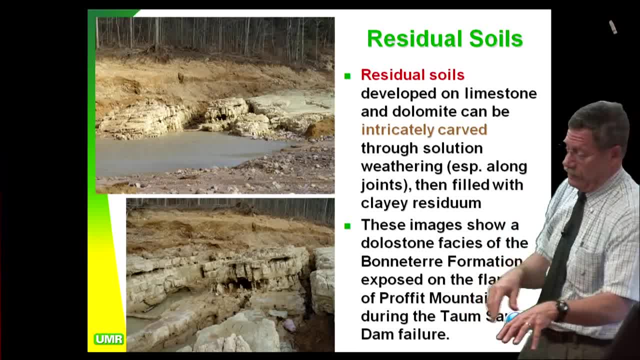 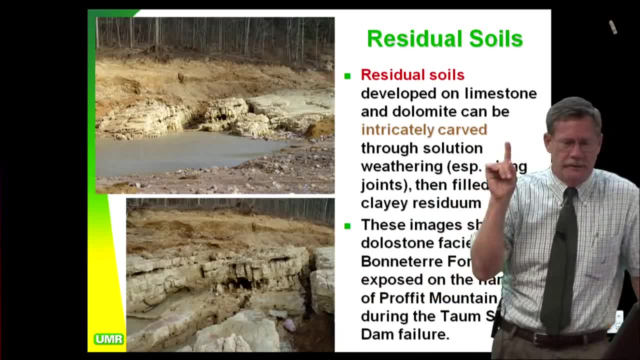 And so you go. well, I've got something going on here. I don't know exactly what. I've got something going on over here And some of those are old sinkholes, Those are old fissures. So geophysics by far is the way to go to start with if you're putzing around in cars. 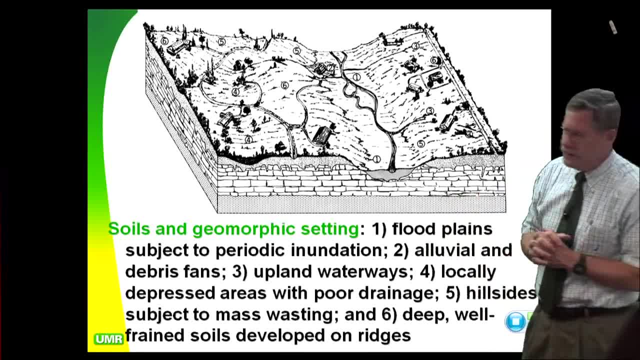 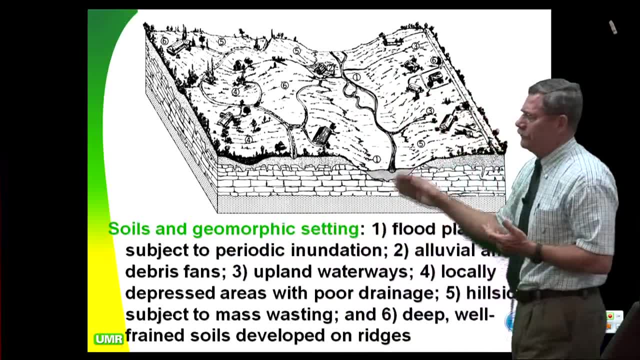 Okay, Big picture view looking down The geomorphic setting. Geomorphic setting is the lay of the land And you can see here we look at a geomorphic setting Down. here is the floodplain along the active region. This is the active river. 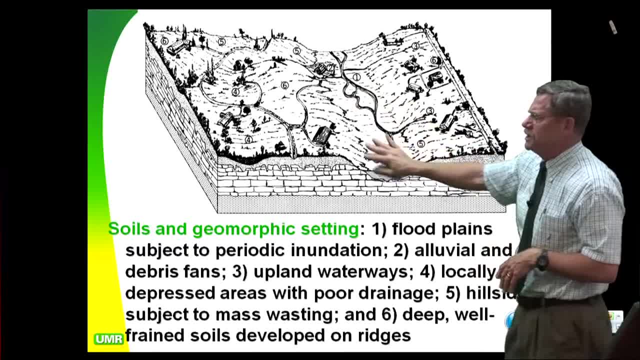 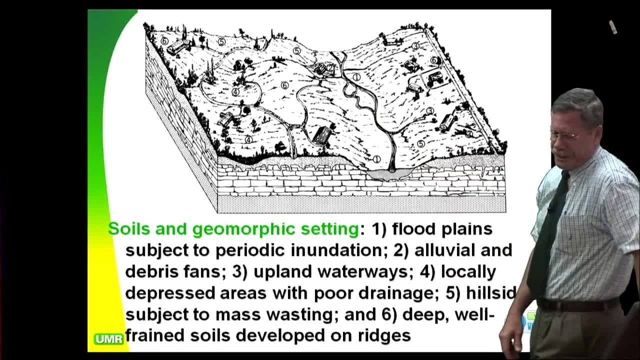 This is the bottom land. This is where everybody wants to buy in the old days. This is the expensive land because it has the rich nutrients in the soil And when they first got to places like Virginia and they got to something called the fall, 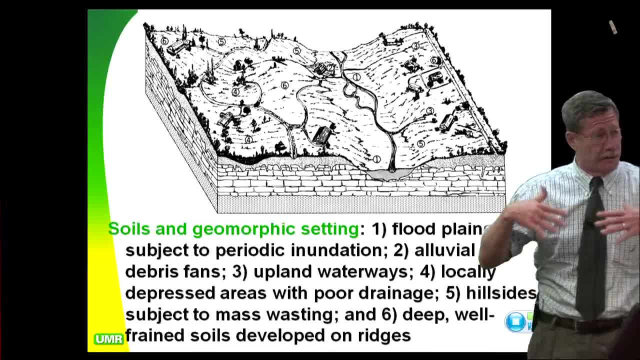 line, which is if you go to Washington DC. it's just below the fall line. There's the fall, the Great Falls of the Potomac, where this granite outcropped and the river drops about 12, 14 feet. 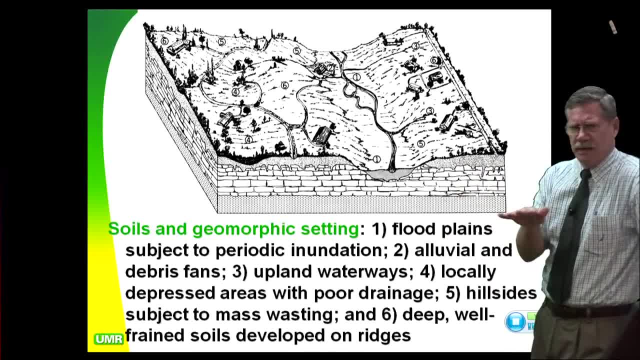 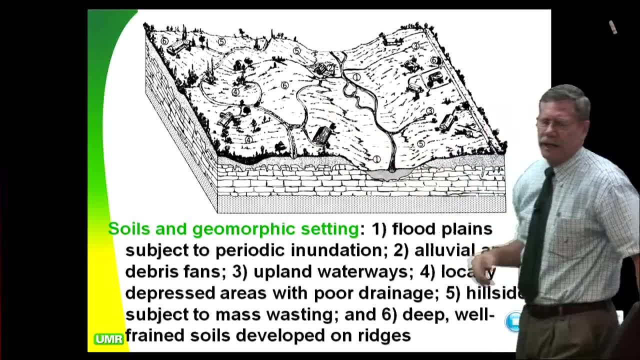 That fall line runs all the way along the east coast And downstream of it you have these very, very fissures. Okay, These are very fertile river valleys and when you get up above it you get elevated uplands And those lower valleys were very, very fertile soils but they planted tobacco. 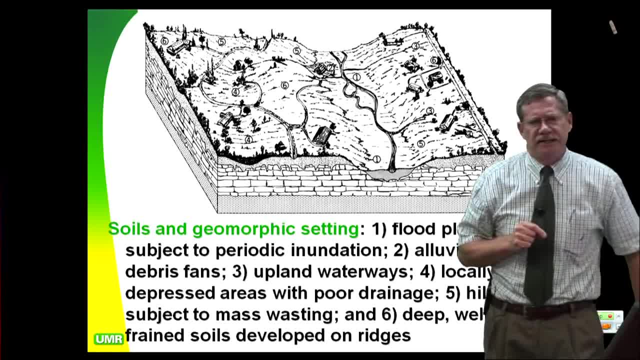 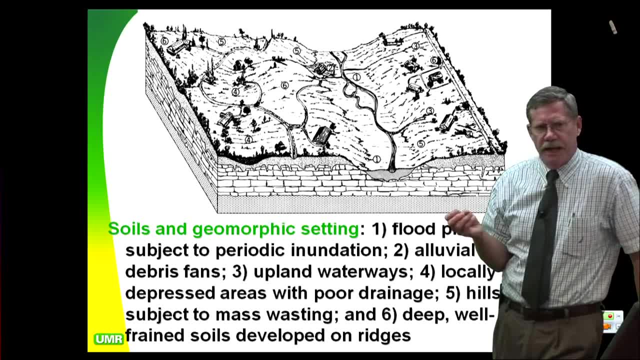 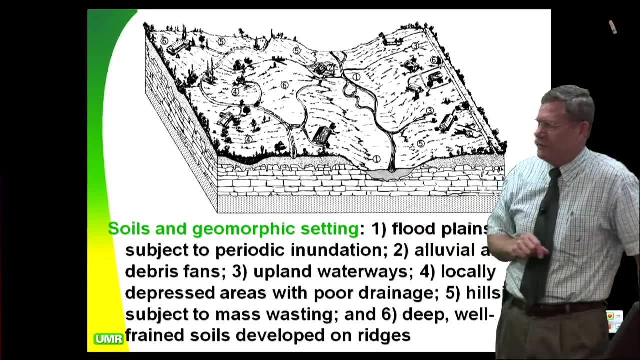 Tobacco was the cash crop back in the 16th and 17th 18th centuries, and they found that tobacco actually releases a very, very acidic enzyme, and so it leached the soil of all its nitrogen, the nitrates, very, very rapidly. So, after you know, every year you grew tobacco, the tobacco crop would get more stunted, more stunted And finally, seven years out, you were done. The land couldn't grow tobacco anymore. So what do you do? 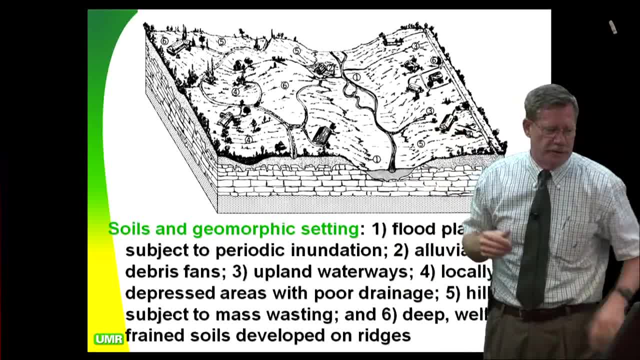 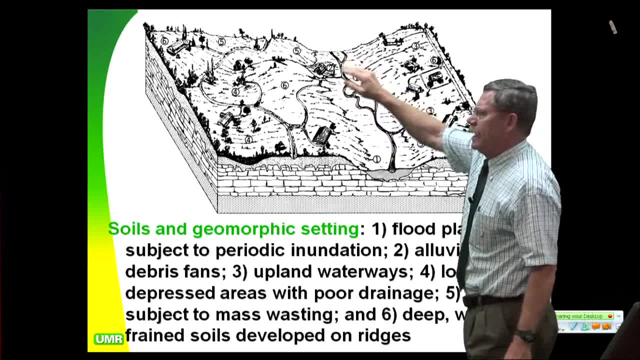 You move west and plow new land, grow more tobacco. So here, geologically, we have the most youthful soils going up this valley And as we get around the corner over here, we get other things. We get the ET. 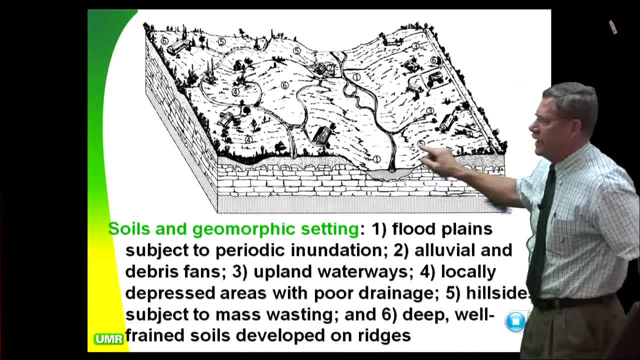 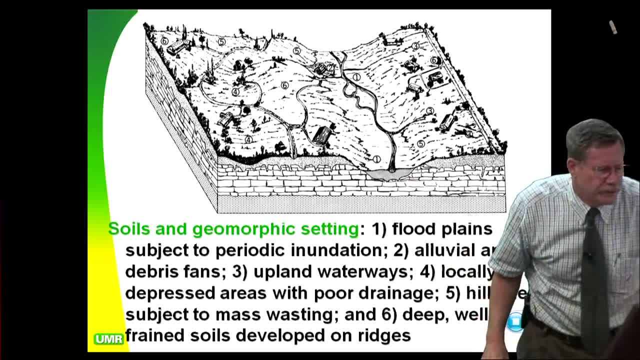 We get the ET, We get the ET things. So that's the alluvial. We have alluvial and debris fans. You can see- let me look on here- what they've called alluvial and debris fans. Okay, right here they're calling. 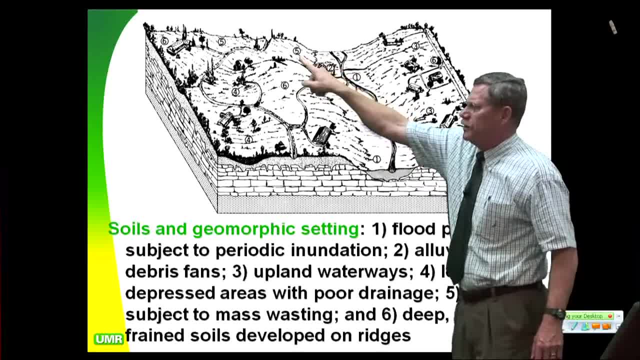 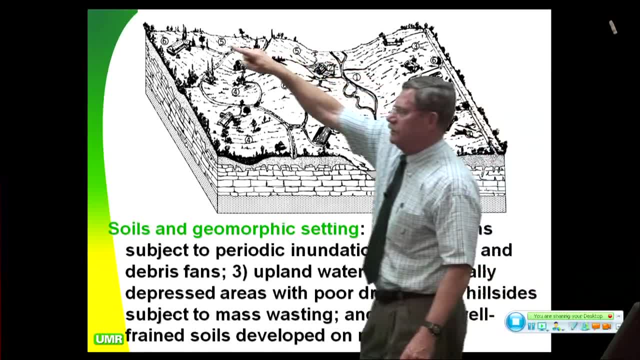 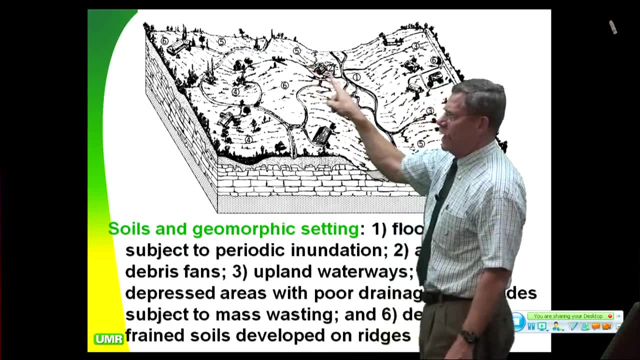 this little debris fan. You see these all over the place along the Mississippi and the Missouri rivers, Any of the major river valleys where you have tributaries feeding along, coming in right down here. you're going to get a youthful fan and you're going to 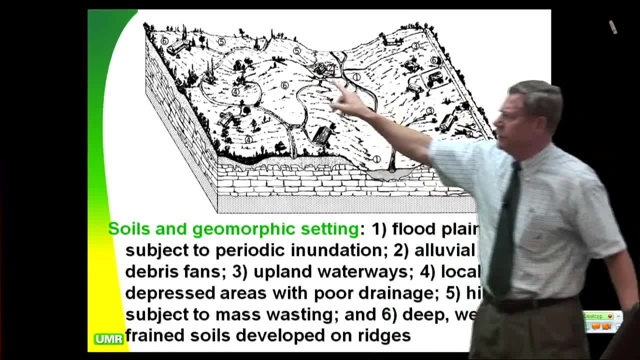 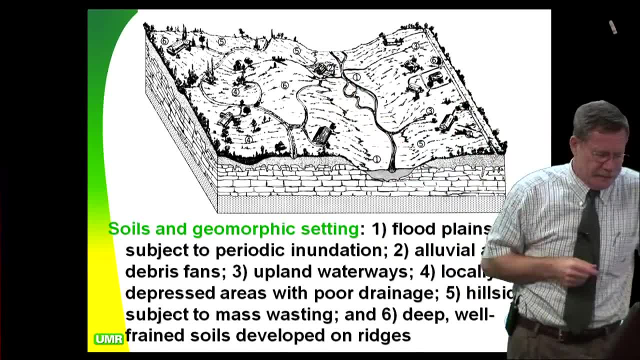 have to be real careful right in there, because that's a different soil condition from the materials right around it- Different soil conditions. So you've got to consider where you are. Terzaghi wrote about these things in his first book- His first book- that he 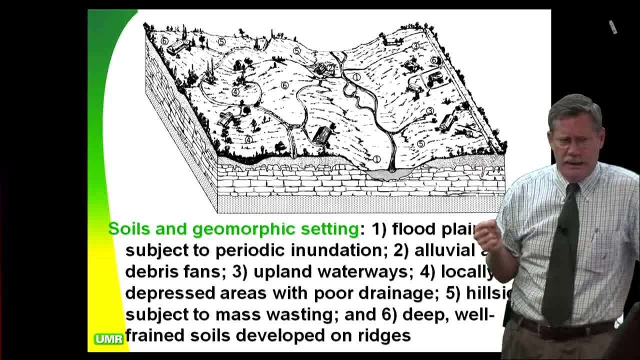 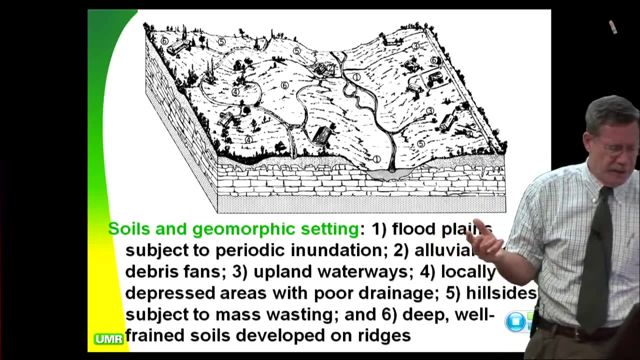 wrote or second book that he wrote. his first book was Erdbaum Mechanics in 1925, which is soil mechanics. His second book was Engineering Geology. Engineering Geology because he recognized the engineering geology. The geomorphology controlled everything at a site. You have to study that. So number 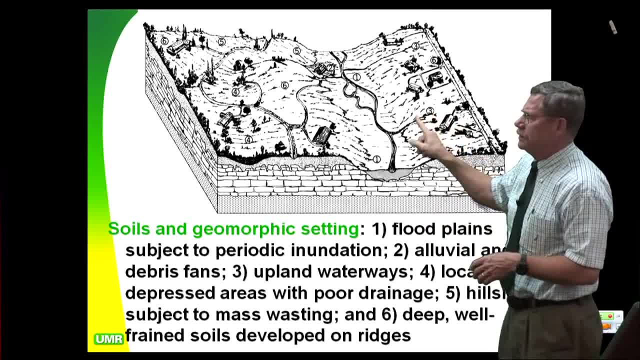 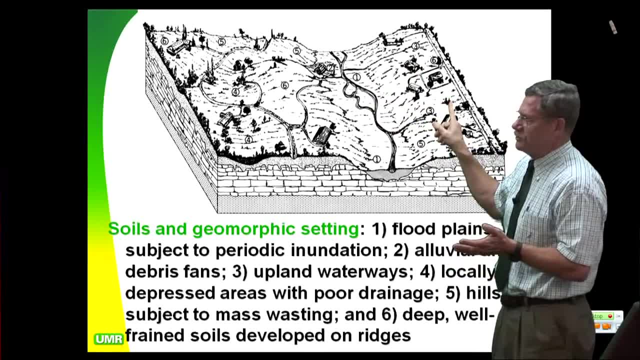 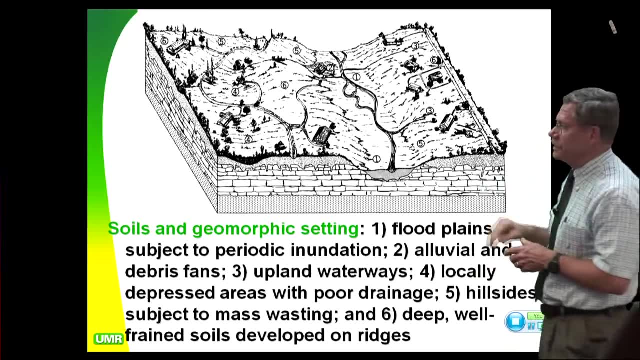 three is upland waterways. right here These are just these rivulets that come down off the uplands. Fairly short time to concentration, high runoff coefficient, depending on the antecedent moisture. Four is locally depressed areas. Now we have these all over northern St Louis area, northern St Louis. These are upland areas that have old sinkholes and highly developed karst profile And these are the kind of areas you've got to be real, real careful in when you're siting things and how you're draining things- One of the big problems we've had with highways we can. 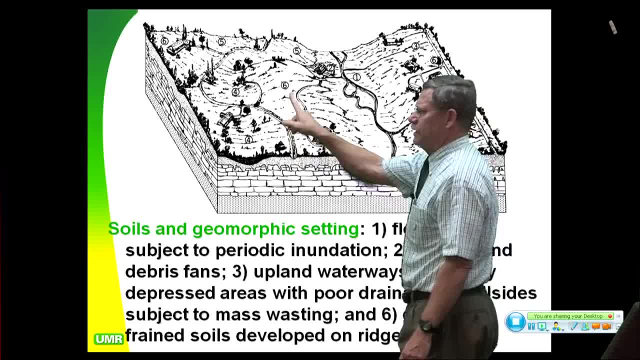 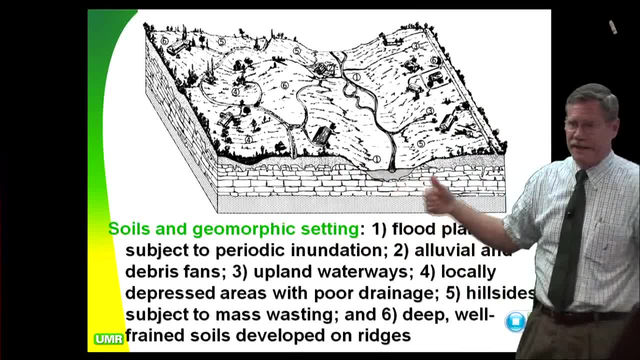 run the highways along the ridges. That's what we like to do in Missouri. Always run the highways along the ridges, because that's where the best foundations are And you don't have to worry about sinkholes and drainage. You're getting stuck so much. 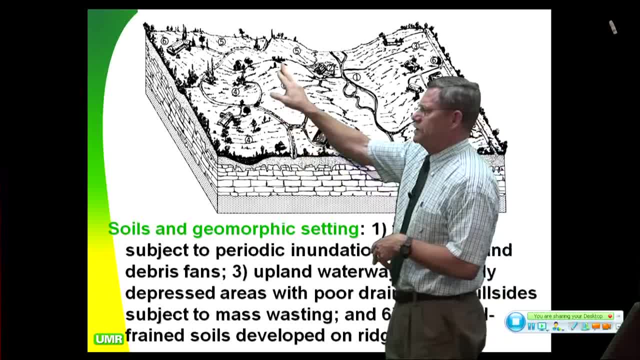 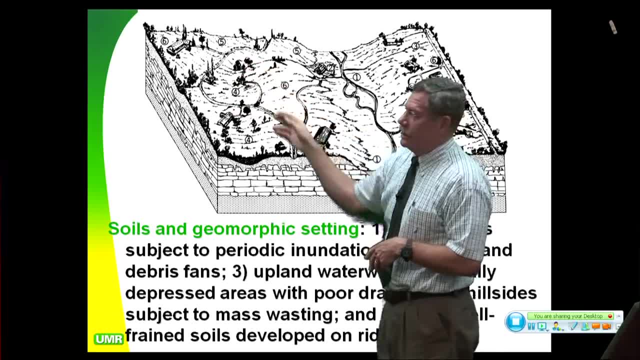 The problem with that is, if you run the highway along here and you have a lot of impervious surface every few hundred meters, you've got to do what Culvert or some kind of drain, So you have an unnatural concentration of flow going off over here somewhere. And what? 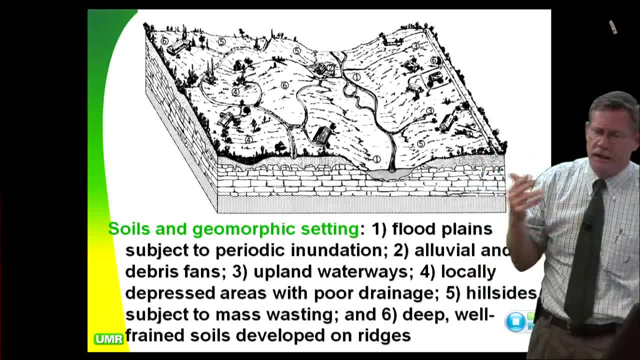 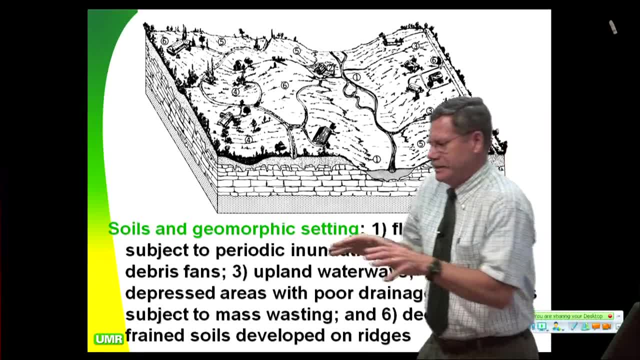 you find in. like Tennessee DOT, Missouri DOT, all of our triggered sinkholes are right next to the highways, Because we have all this water going over and suddenly we have four or five times as much water percolating into the highways, And that's what we're looking. 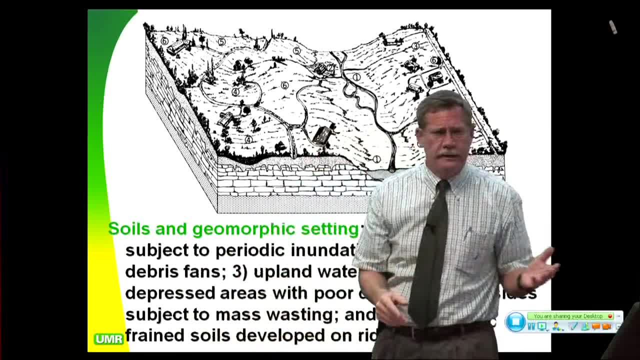 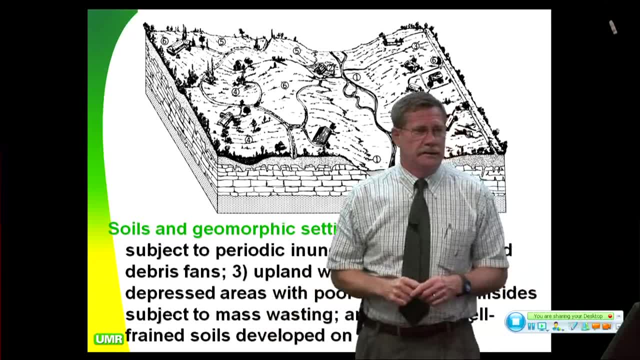 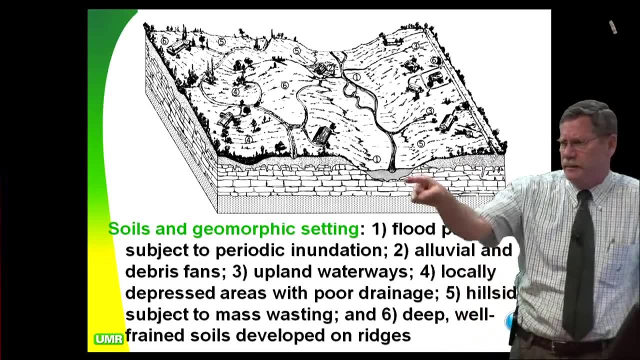 for. So the highway development is the trigger for that formation of that sinkhole. So the farmer who owns a sinkhole calls an attorney his son-in-law sometime, and they sue the Department of Transportation saying: but not for your public improvement, for that highway. 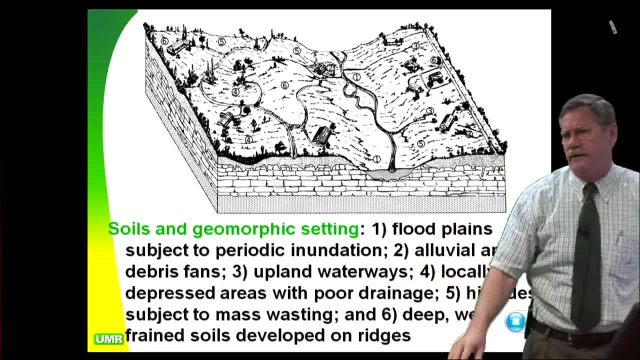 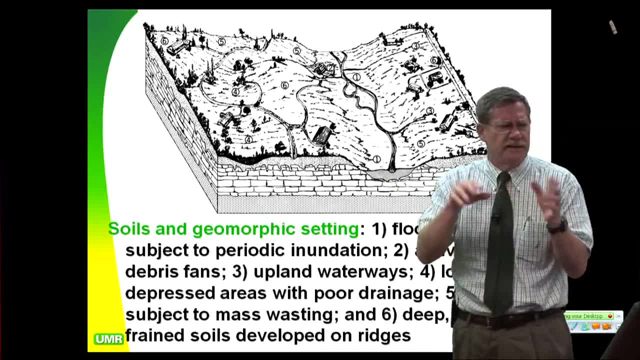 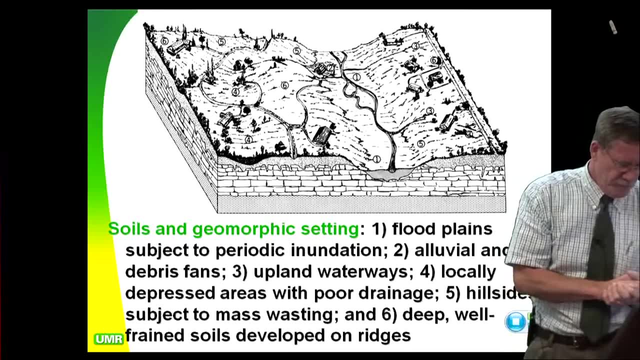 over there, I wouldn't have this big loss of pasture here, That's true. So they've tried to tighten up the laws on a lot of this stuff. Well, if you get sinkholes- too bad you know- Go somewhere else. 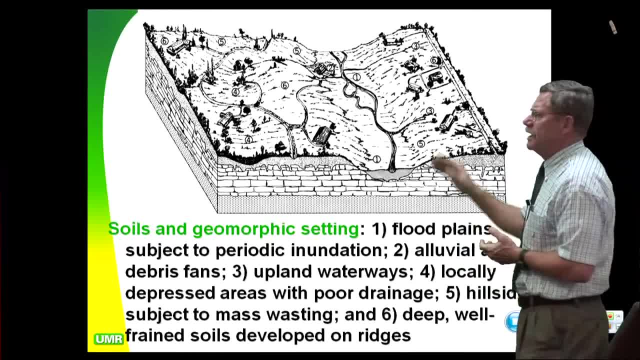 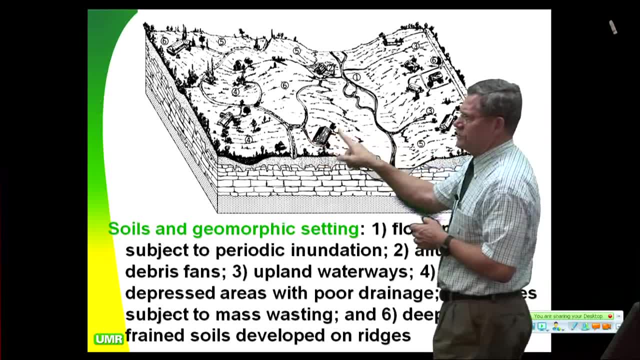 So hillsides subject to mass wasting. that means landslides, So any hillside can be subject to mass wasting, just depending where it is. A lot of times we put houses in places like this and then we put septic leach fields out here And we can actually flush ourselves. 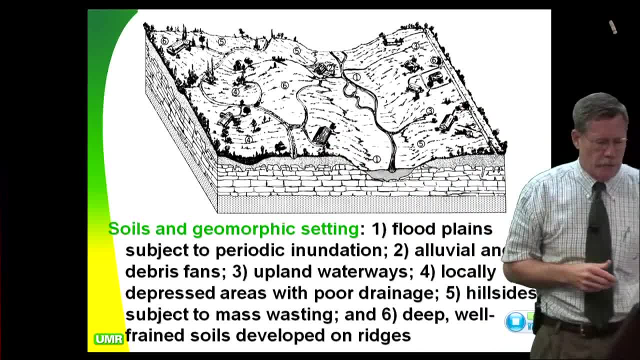 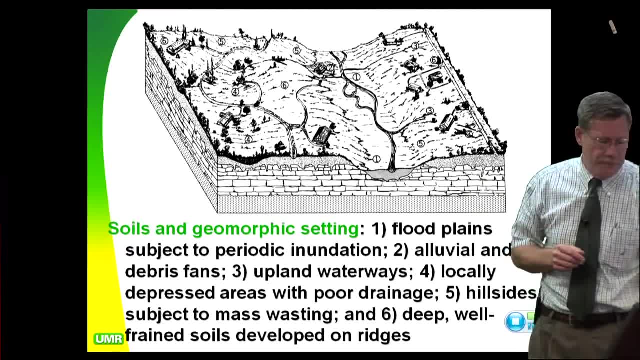 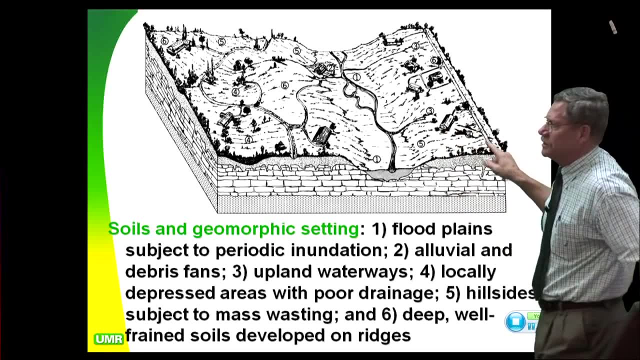 down the hill gradually by adding a lot more antecedent moisture So that when the storm comes it magnifies the impact of the storms, And then we have deep, well-drained soils That's not well-framed, but well-drained soils that develop on the ridges, And that's why 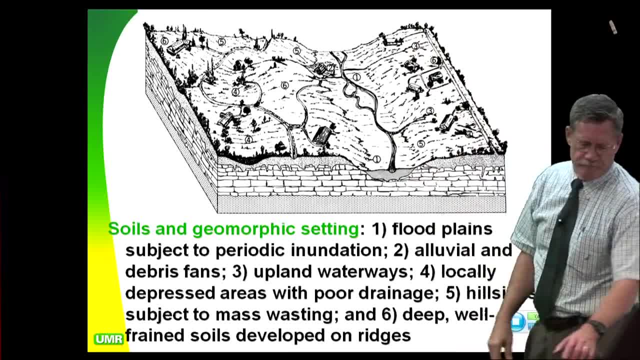 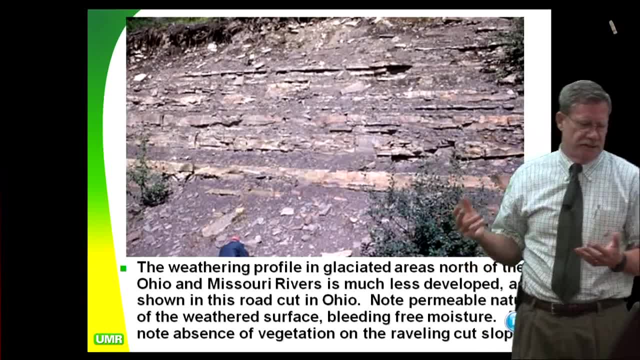 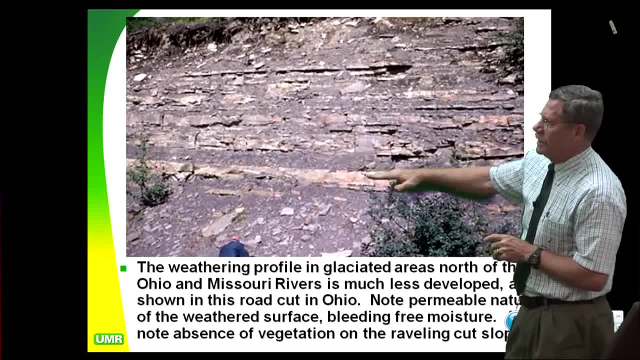 we see the highways going up the ridges And you see that around here. Here's a real typical weathering profile in glaciated areas north of the Ohio and Missouri rivers. This one's actually in Ohio- I picked here- And this is pretty typical We have. 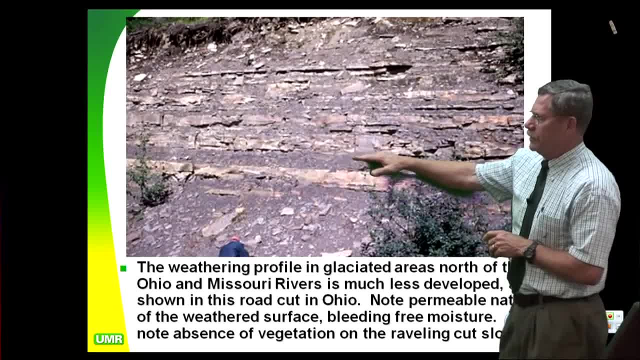 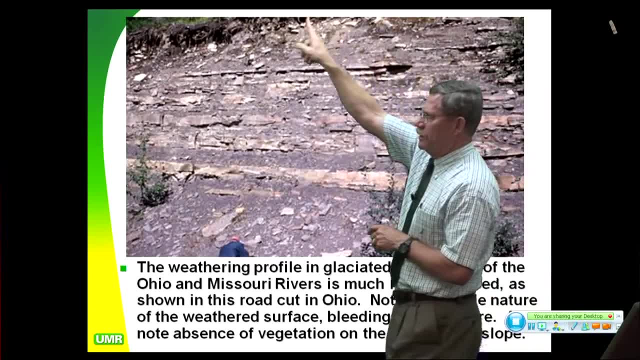 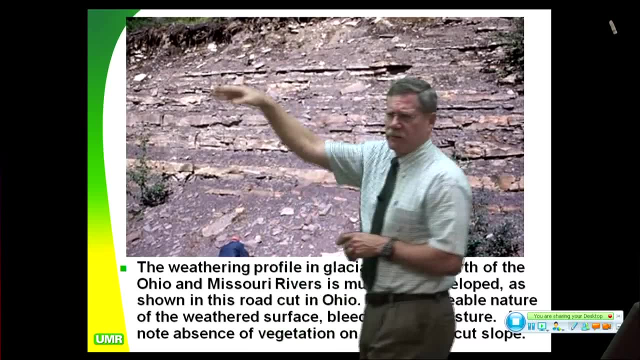 a sequence of lines. We have some stone beds intermingled with some shales, And you go up here to the top of the picture and you actually see there's some wet zone. right here We have a very immature, thin, immature soil horizon, because the soils that were there got carried off by the glaciers. 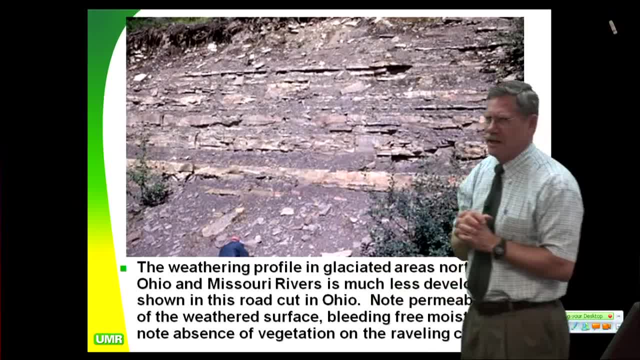 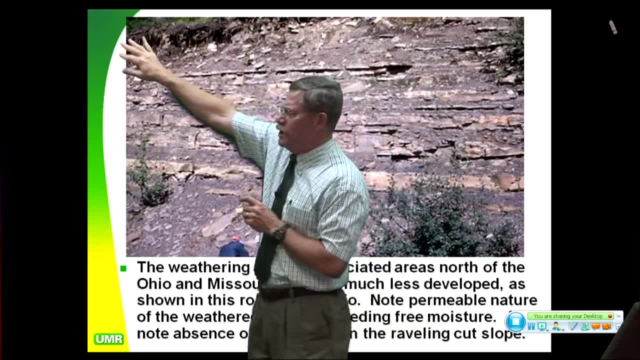 So the soils are gone. It's a completely different geology from down in Kentucky And so we also have a permeability boundary along here because of the soil creep rock zone. the hillside creep zone causes the materials to dilate. they have a higher. 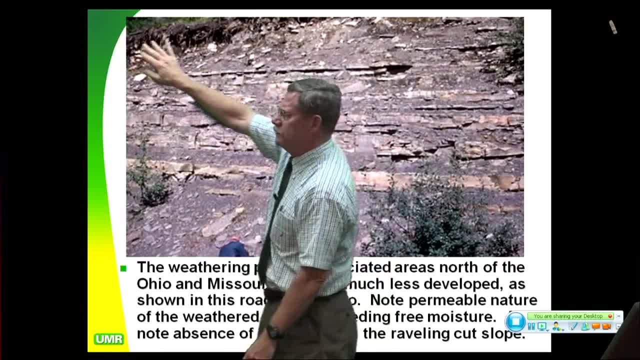 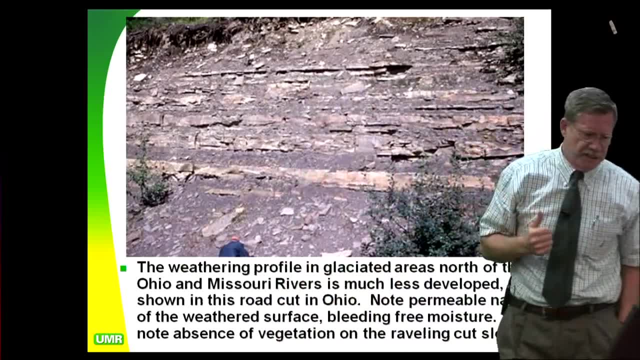 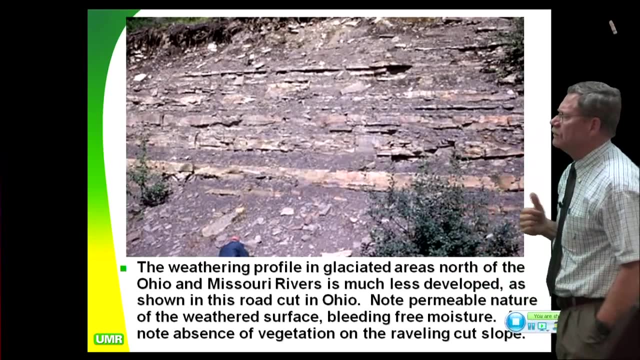 hydraulic conductivity. so you get a lot of moisture that weeps out of this area and you get a little under plucking going along right here. now, if you look at this cut, one of one of the first things you notice is absence of vegetation. I mean, we're in an area here that has, you know, gosh, 55 inches of rain. 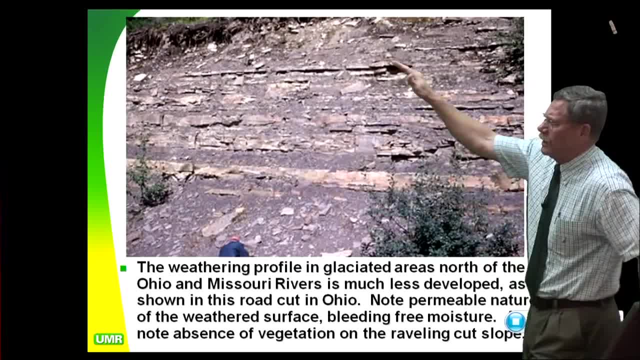 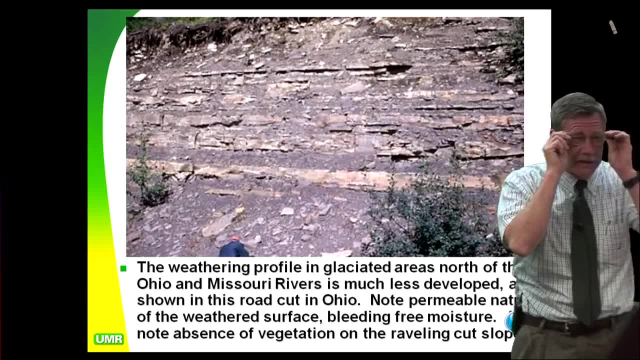 a year. I mean most of this. all you know summertime. why isn't stuff growing on this slope? that's one of the questions you want to ask. that's one of things I want to teach you to do. that's becoming an astute observer of nature. you want to. 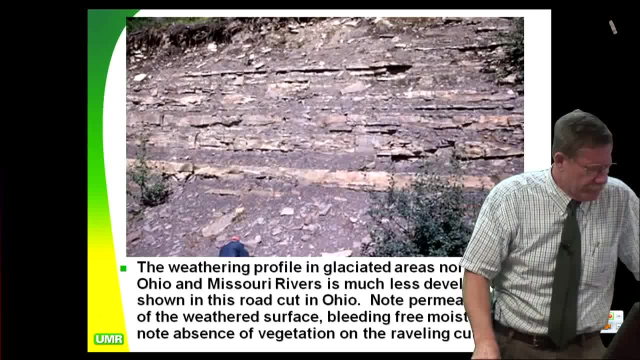 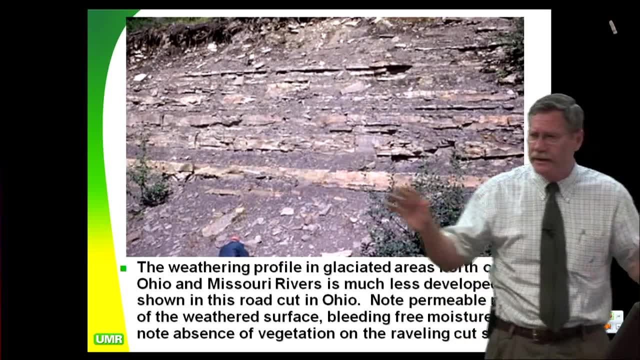 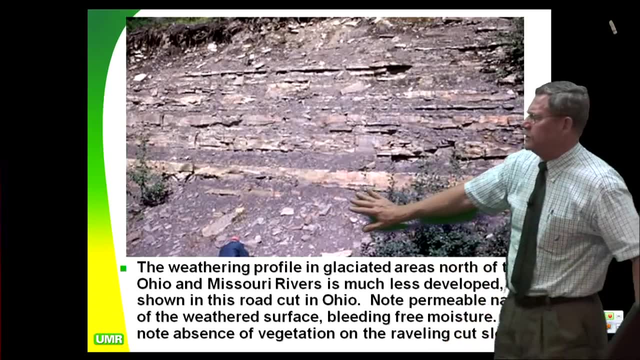 look at this slope and say, huh, nothing growing on this one. they took me out here to look at this one because they were having problems with it all along thing. now there were other slopes along here, similar geology. they weren't having these problems. I want you to notice something right away. number one: what? 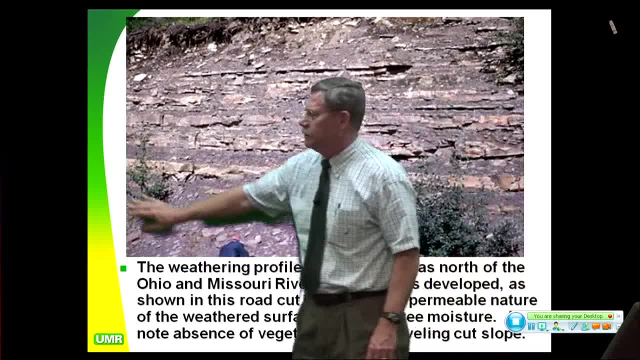 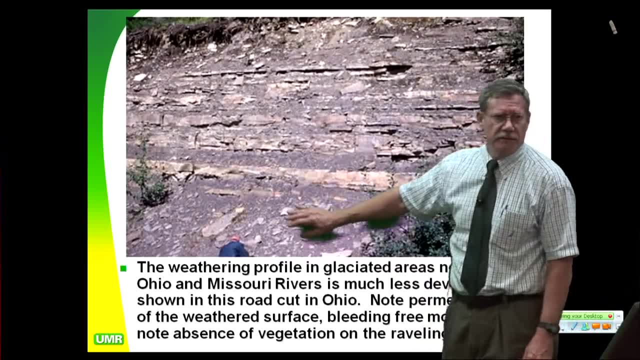 What's going on right here? What is this called Talus? that's a scree slope. that's a talus slope. Where's that stuff coming from? Is it young, recent? Yeah, that's yesterday. This is very recent, geologically speaking. 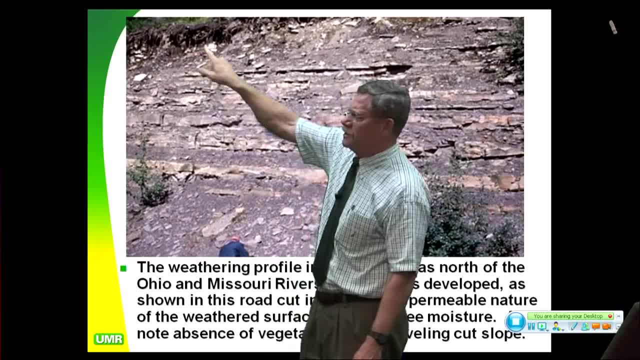 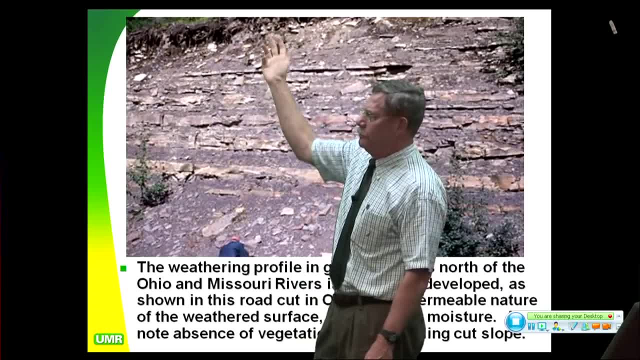 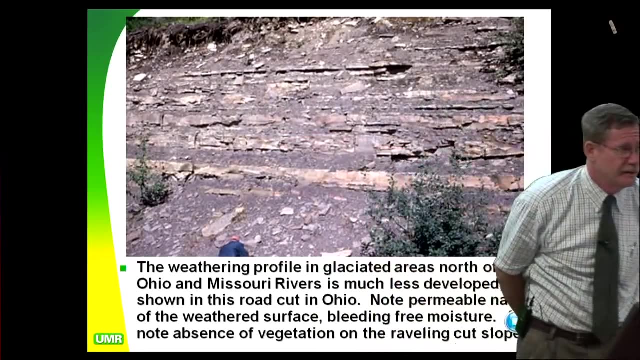 What's going on up here? That's where talus come from. Talus go down to here, So you have a zone that's very actively bloop, bloop, bloop. What's causing the blooping? Come on, what's causing it? The rainfall? Yeah, water, percolating water. It's not the rainfall, it's the percolating water where you have emergent seepage pressure. The emergent seepage pressure when you get a lot, when you get a lot of rain, like over a period of days. 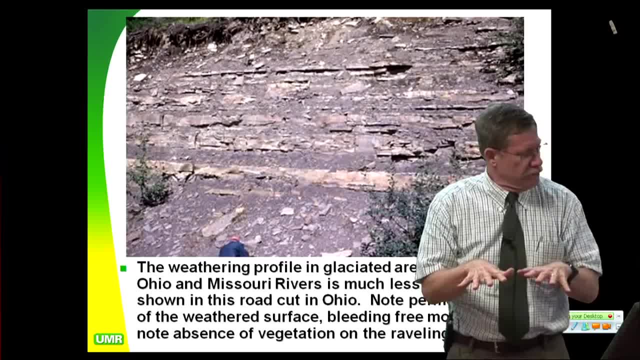 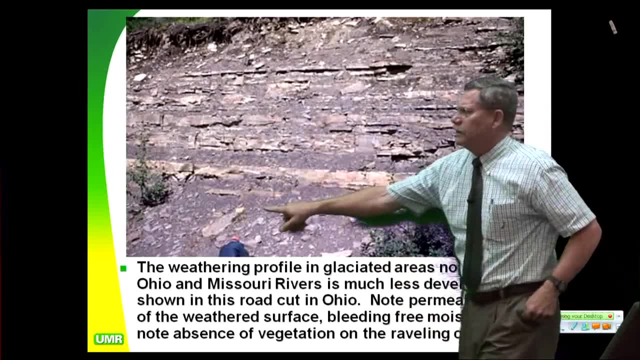 a lot of water seeping down. that is raising the pore pressure enough that you reduce the effect of stress and the blocks are falling off. So one block at a time. That's not all happening all at once, but it's just constantly going to be coming off there. 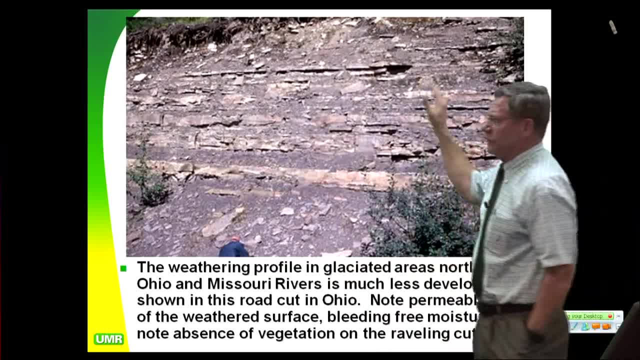 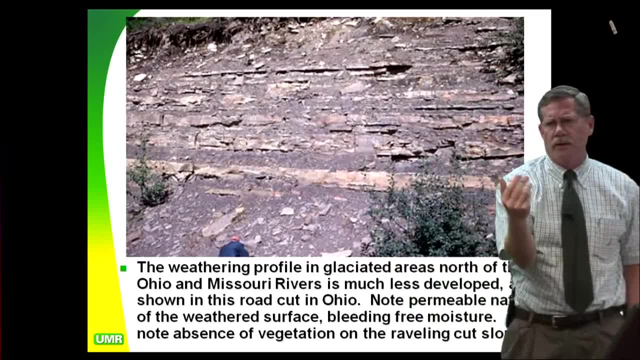 So if you wanted to arrest that problem, there's several things you could do. One: you could just shave this top of the slope back. Shave it back more like a natural slope, so that the water would come out gradually, not all at one place. 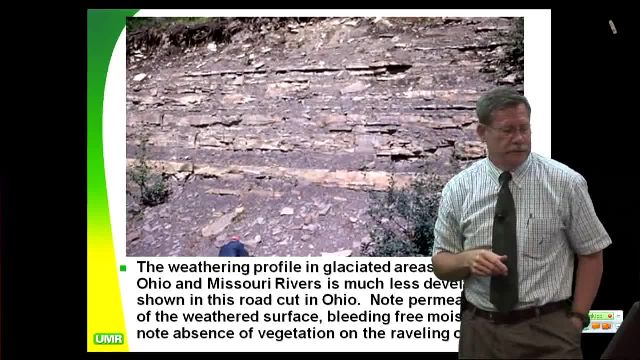 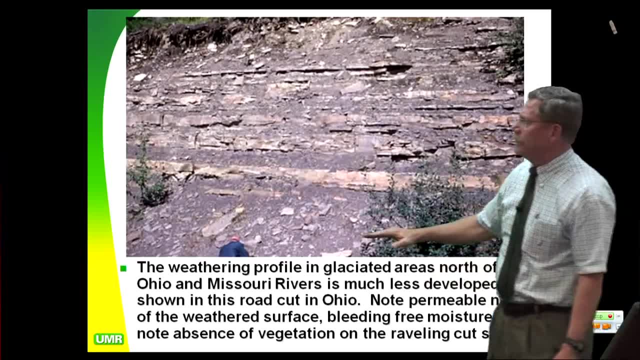 Or you could put a drain of some sort in up there. That'd be a little more iffy, a little more difficult to do. But a lot of times you're on highway, you're down here, and as soon as you get more than about 12 feet up, you're down. And as soon as you get more than about 12 feet up, you're down above the road. your options really start getting thin because it gets expensive. Anything you do to fix a highway, you want to do it on the highway and on the shoulders. if you can. As soon as you start going down the slope or up the slope, the cost is going to go out through the roof. When I get up on a slope, that's going to cost me four or five times as much per yard. 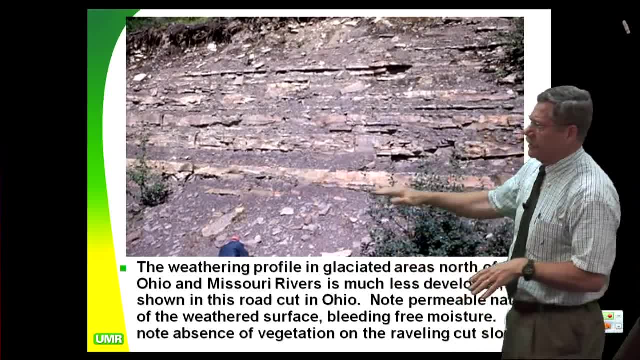 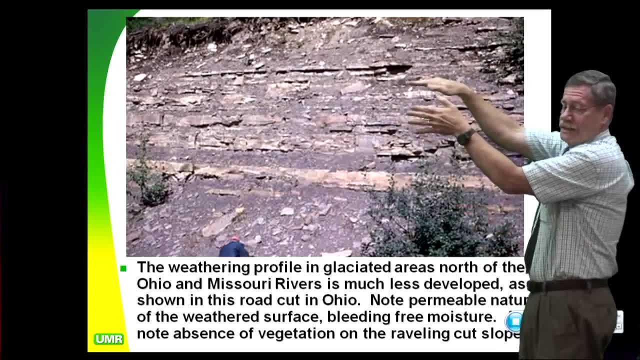 to putz around up there. So if I had to attack something like this, what I would do- I would actually build a rock ramp here and I would ramp up, get my equipment up 18 feet above the road and then work off that temporary platform, put my soil nails, my tie backs, whatever I want to put. 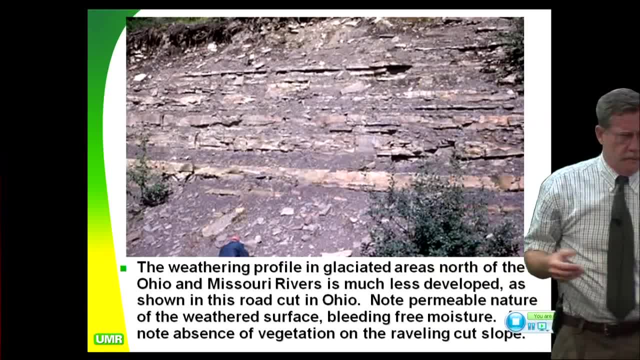 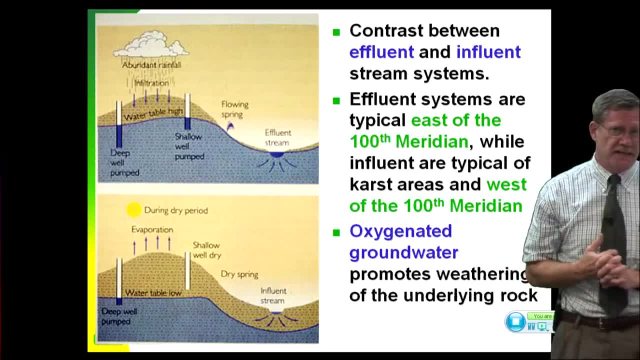 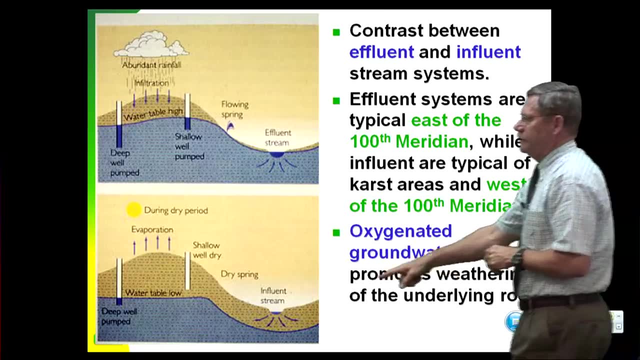 in, in, and then I'd take out that rock wall, make it out of gabions something that's nearly vertical Contrast between effluent and influent stream systems. In the Ozarks we have a lot of influent stream systems. 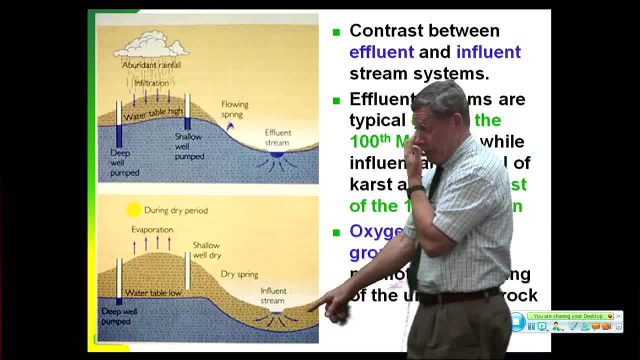 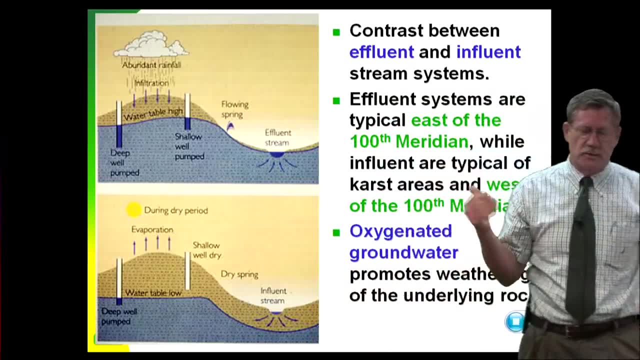 They're called losing streams. Dry Fork, which I live right along over here, is an influent stream. That means it loses its water pretty quickly. I mean I have water on both sides of my backyard. It's wonderful It's been raining. 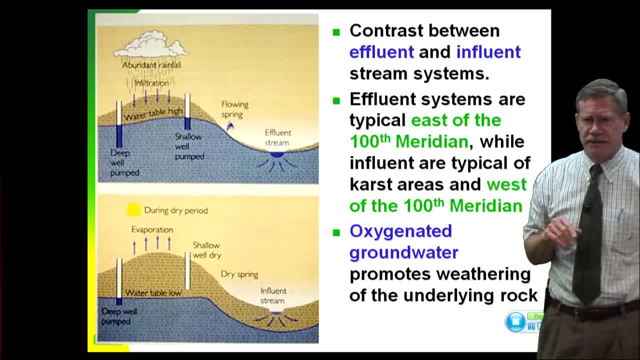 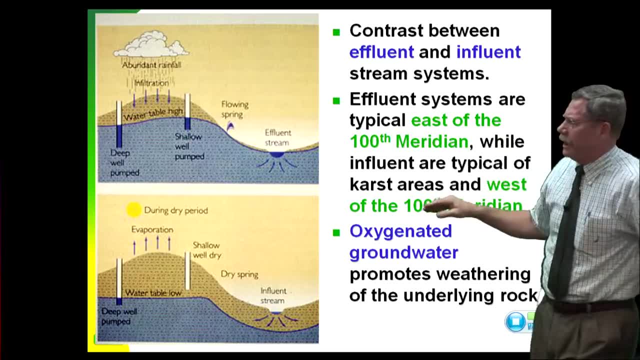 You hear all this gurgling and rapids going and everything. It's all over in two days And seven days later there's no water. About seven days at the tail, because I'm at the upper end of the watershed. So 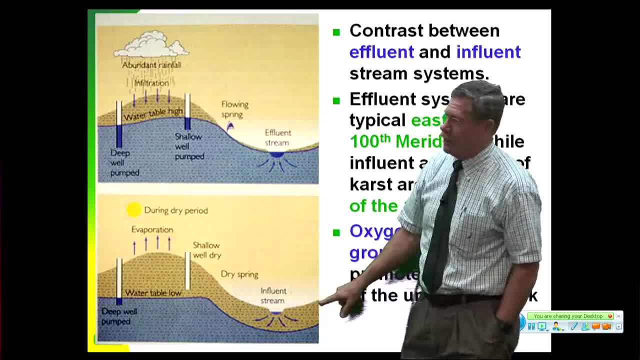 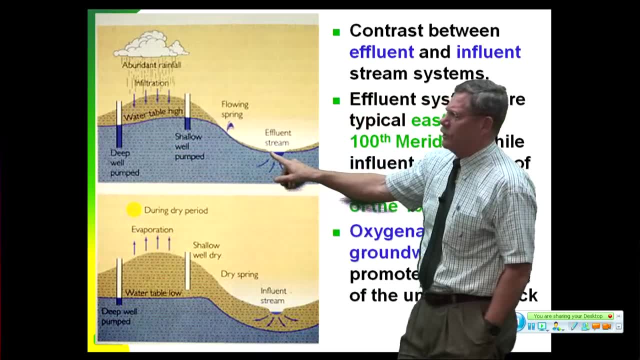 So losing streams, and they're pretty common when you're in karst areas. Karst areas have losing streams. When you're in a typical area with a typical kind of non-carbonate kind of stratigraphy, you're going to have typically an effluent stream. 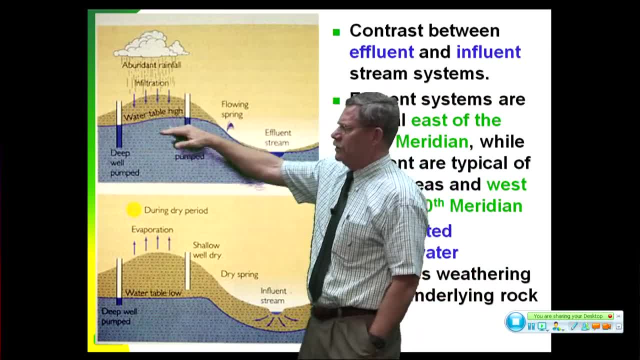 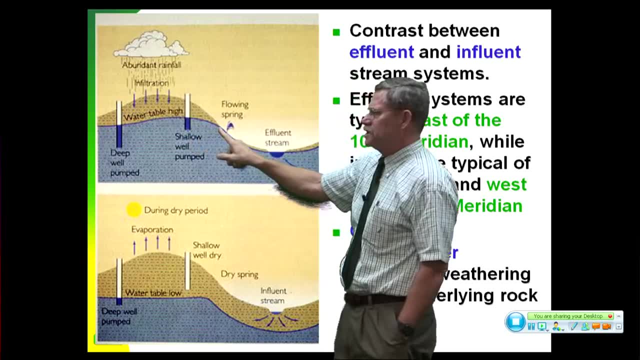 So you're going to actually have a water table up here. That water table fluctuates by decade and by year and season, And then you could have some springs once in a while- typically they're seasonal springs- And then you're actually going to have some feeding. 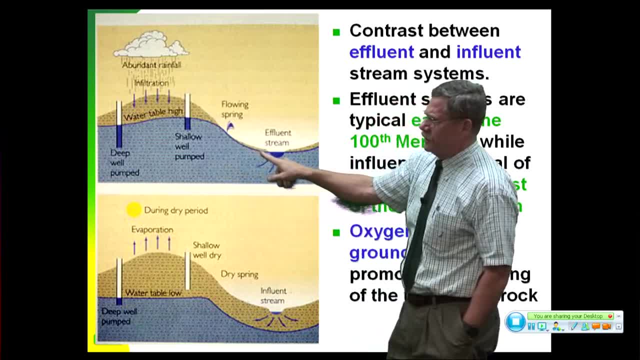 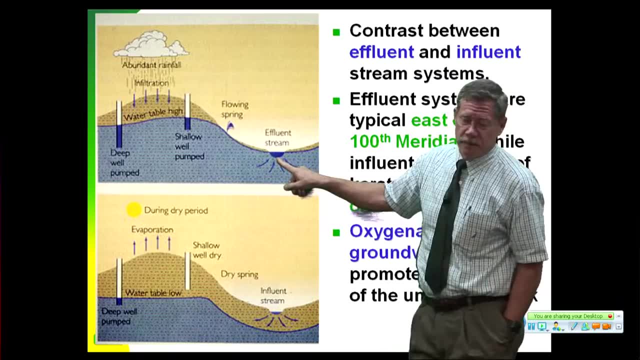 You're going to have this phreatic surface, the saturated zone that comes down and makes connection and is coincident with a perennial stream. Perennial stream Now, a lot of times you have a big stream like Shenandoah River. 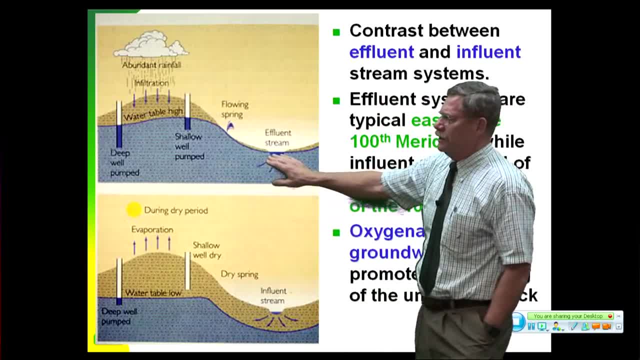 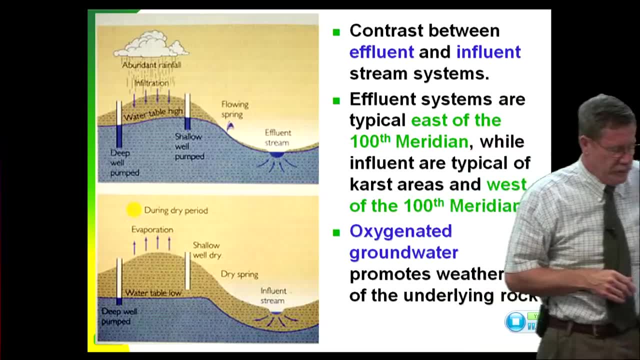 It gets about 10% of its inflow from percolation like this. That's a typical number. 10% That's back in Virginia places like that Around. here We have both systems, although we're dominated by this one. 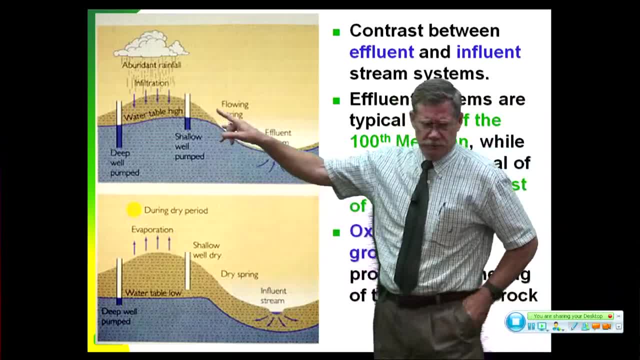 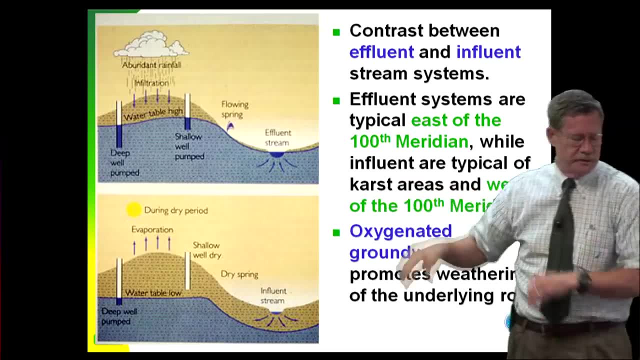 This one's really big time. when you get down to Kabul and that area, West Plains- You don't see any channels down there with water in it. Everything you see is big sinkholes all over the place. They're like big bomb craters. 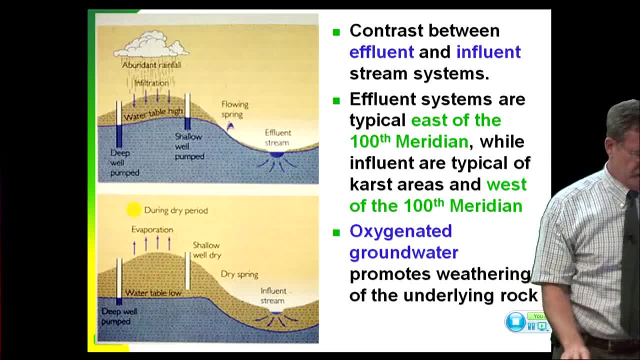 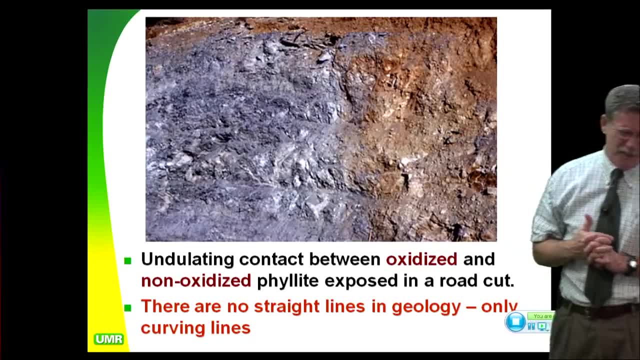 And so effluent systems. really typical east of the 100th meridian, Alright, Undulating contacts. That's probably the most important picture I'm going to show you, and it's not a very exciting picture. It kind of looks like a barf or something. 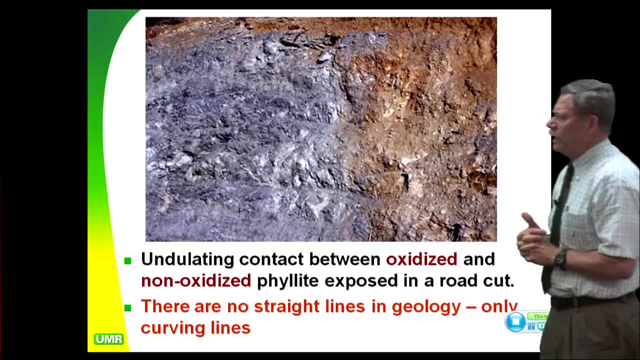 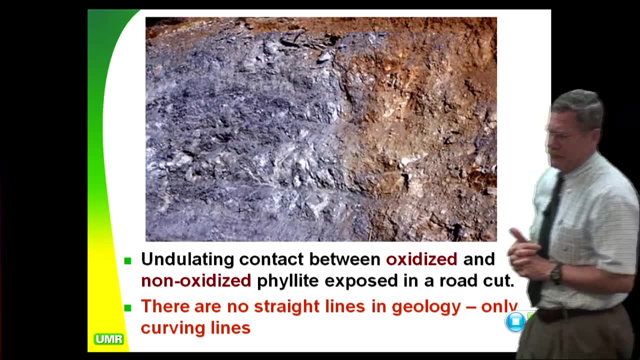 I don't know. It's pretty nondescript. What I'm looking at here is a quarry, a quarry face, and it's an old quarry. Now, one of the things I learned in California: you're going to go out and get people bids. 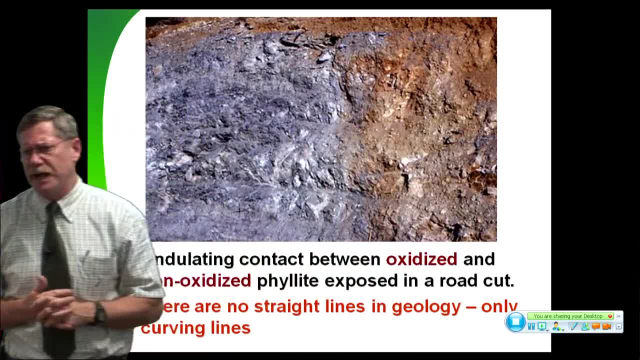 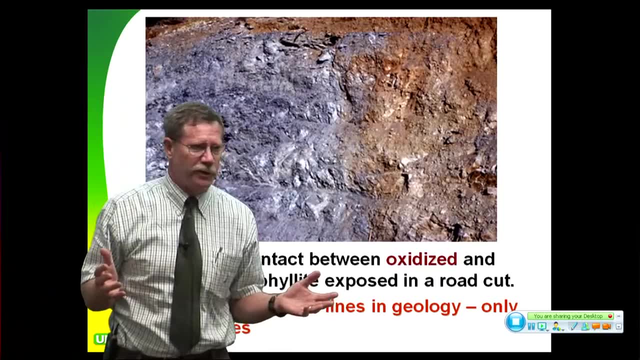 and plans, bids and spec in 72 hours. you better find out where all the old quarries are. Now in Phelps County we've got three active quarries and we've got 16 derelict quarries. You want to know where the 16 are because if you've got a derelict quarry just down, 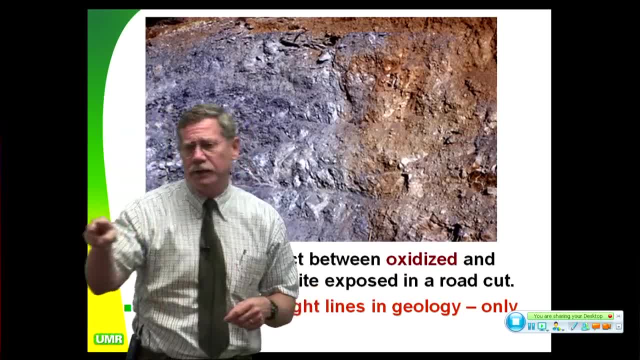 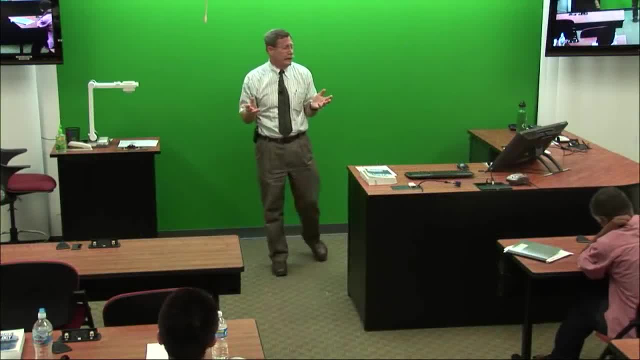 around the corner from some big problem. That means I can go put in a little small crusher- you know system- or I can just put in a skimmer, put in a screen, and I can actually go out there and for very little money get. 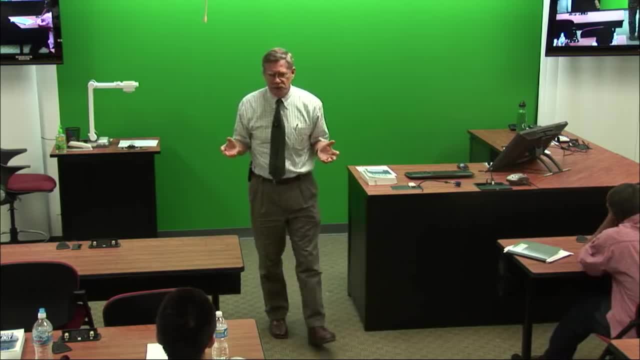 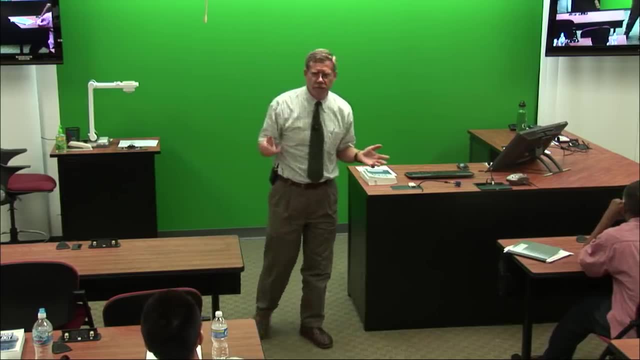 my rock, Because all the money in aggregate folks, is transport. You have a price per ton, 1.2 tons per cubic yard FOB. What does FOB mean? Come on Anybody from the working world, FOB is freight on board. 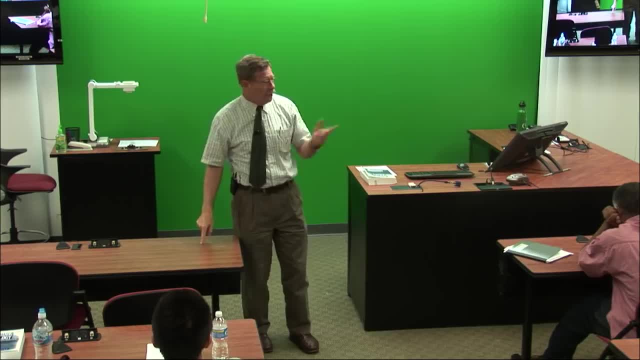 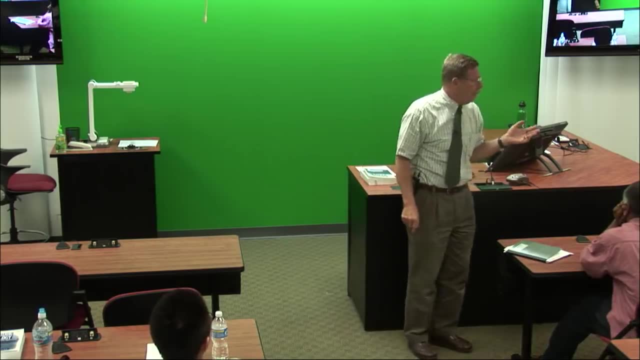 That's the price they charge you at the quarry. What does that mean? What do you pay for it over here at your house? 64,, 74,, 84,, 94.. Whoa, whoa, whoa, whoa, whoa, whoa. How much are they charging over here? 1.2 tons per cubic yard and they're charging it by the ton and they're going to charge you 6,, 7,, 8 dollars a ton. How come you're paying 68 dollars a ton over there? 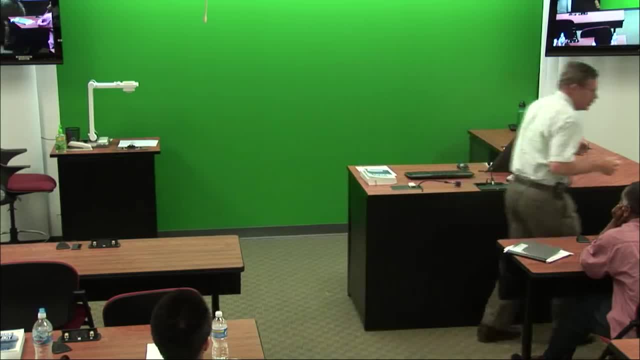 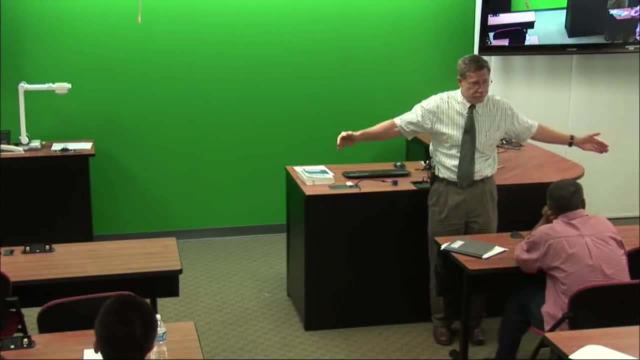 Because of transportation costs, diesel, Got to bring it over here and drop it, okay. So all the money is how far you got to go with it. So if I'm going to use rock gabions, for instance, I'm going to use gabions every time. if I'm 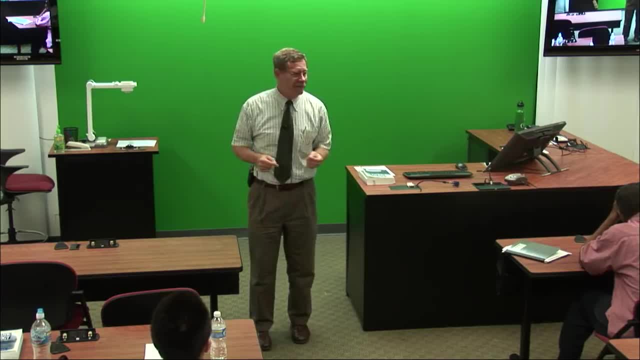 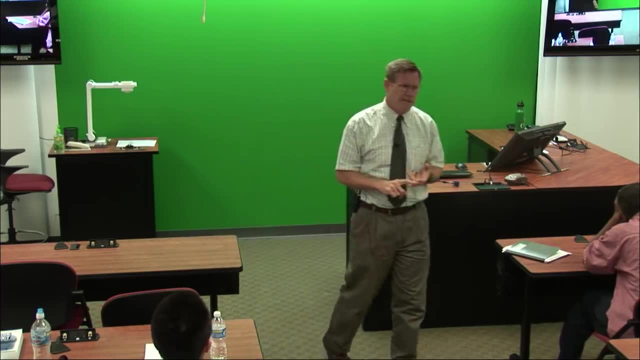 within three miles of a quarry, because it's going to be cheaper, because everything gets down to transportation costs- Concrete, steel, gravel, Gravel's cheap. So if you make a repair out of gravel or crushed rock, crushed two by three, you're going to 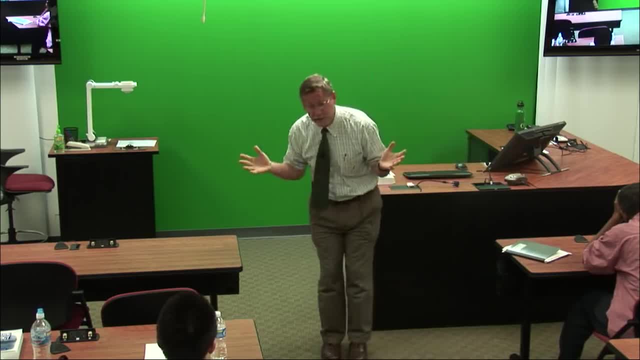 do it because you're going to get drainage and you don't have to worry about compaction. You can do it in the middle of the night, You can do it without you know raining It doesn't matter. So you want to know where all the money is. 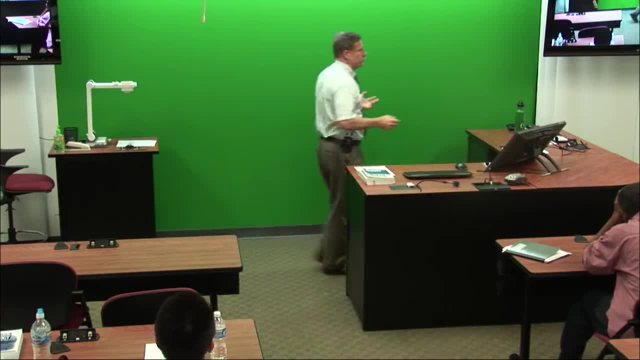 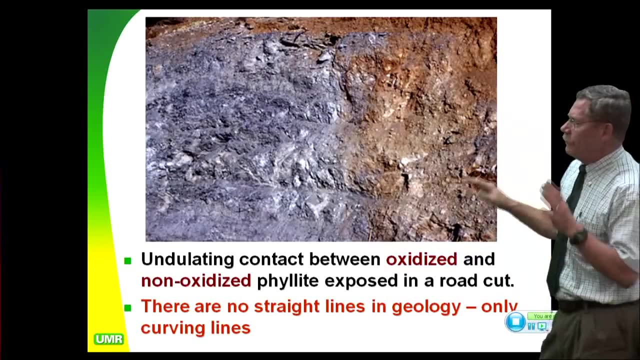 You want to know where all the quarries are. So I'm always out scamming all the quarries, looking at all the quarries. So we look at a quarry- Here's a typical quarry face- And I'm looking at a rock here, and this is all the same rock. 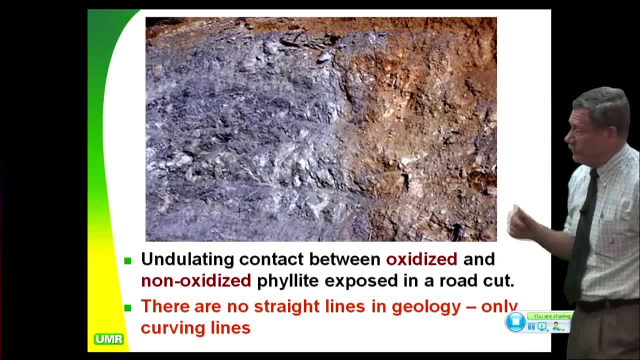 So I go get the geologist and I say, Mr Geologist, tell me what kind of rock I have. So he comes out here and he goes: you have a glycophane micaceous greenstone. Oh really, glycophane micaceous greenstone. 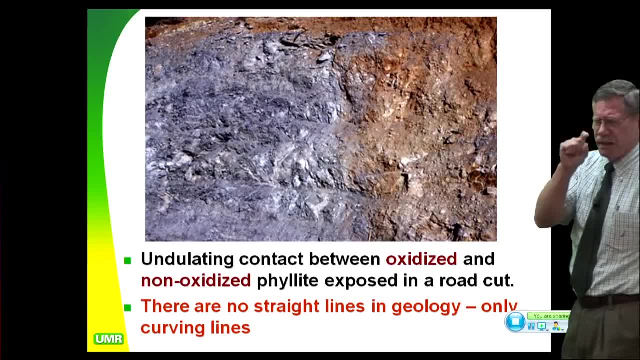 Okay, great, Got it. Okay. so he's going to give it to you in descending order of mineralogical content: Very, very useful for nothing in engineering, but you know, we know what the petrology is that way. 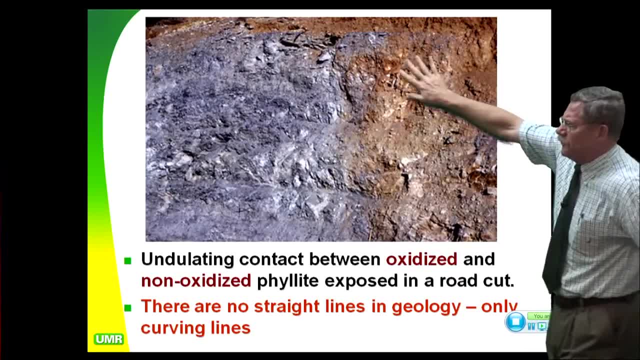 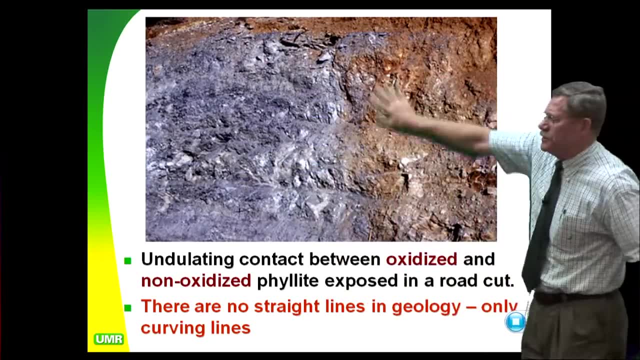 Okay, that's good. Okay, so why is this stuff red and this stuff is blue? And the geologist will tell you: This stuff is oxidized and weathered. This stuff is not. What does that mean to an engineer? That's an engineering term now. 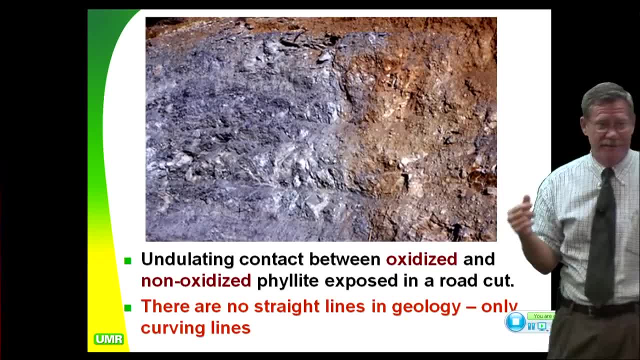 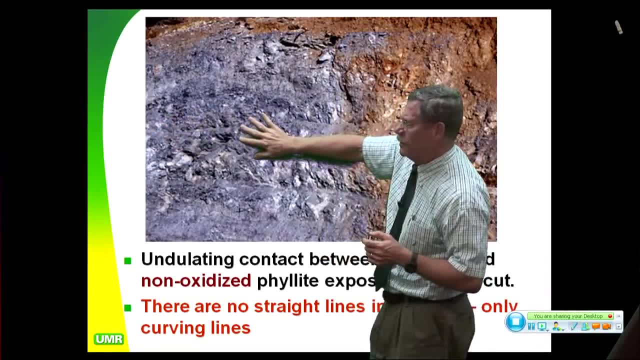 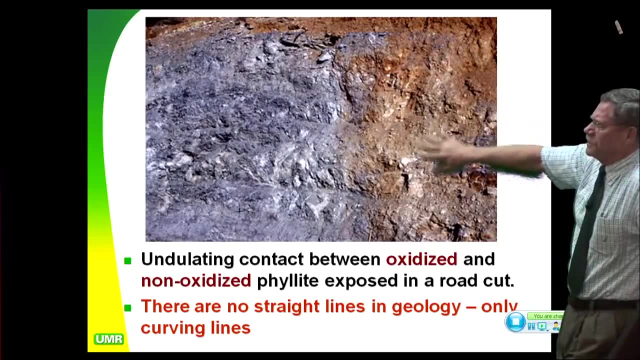 I'm going right brain, left brain, You like this? No, Okay, So oxygenated groundwater, non-oxygenated groundwater or no groundwater, More engineering stuff, Crappy material, lots of fines. can't use as engineered fill a lot of times because 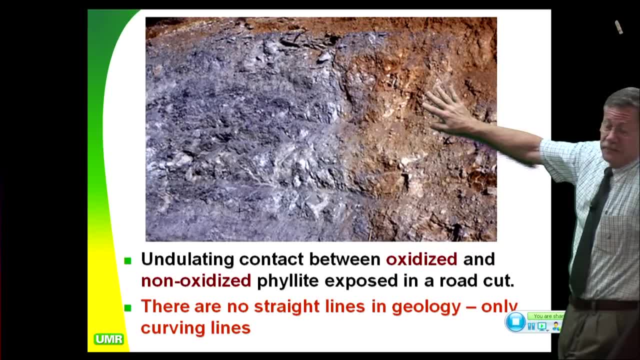 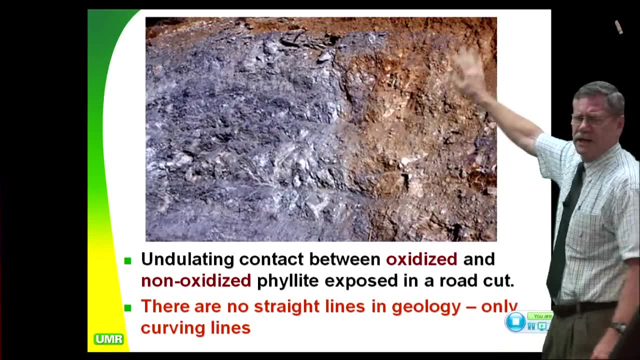 more than 30% pass in the 200.. That's the engineered fill spec in all the DOT books. This stuff you can use. So this becomes what we call in the mining industry. what do we call this stuff? What do we call this stuff? 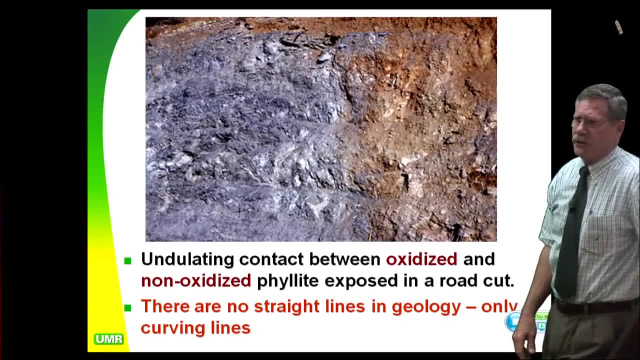 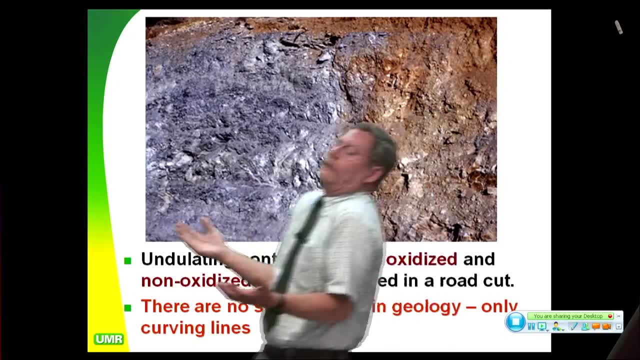 Burden Burden. It's like an old boyfriend, Burden Burden. I mean you've got to cut this stuff out of here and you've got to pay money to move it over here and get rid of it. It's waste. 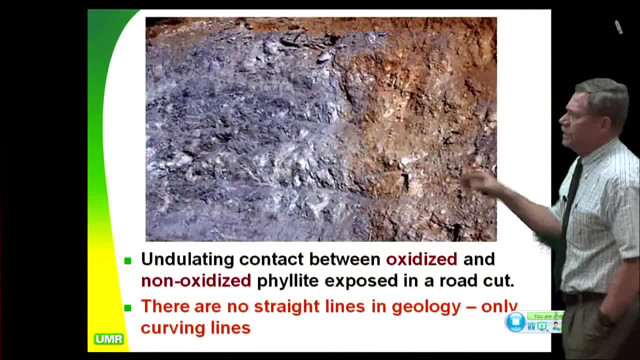 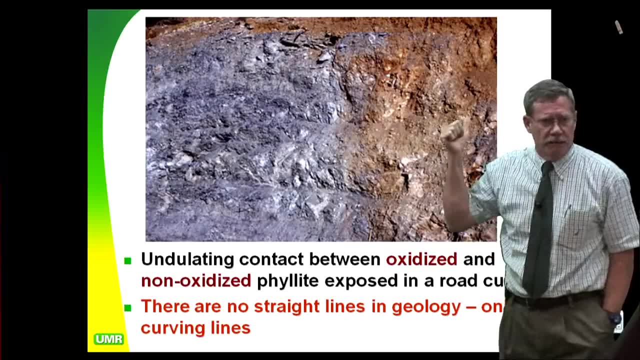 Now you can use waste dump material sometimes and stuff, but this is real typical of what you see in quarries. Go to some quarries, go to some road cuts and start looking. I want you to get the mark one eyeball. 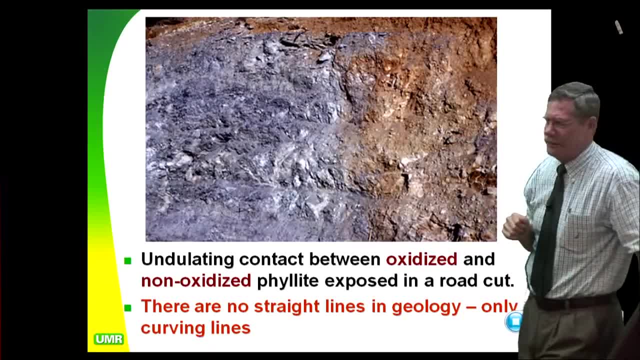 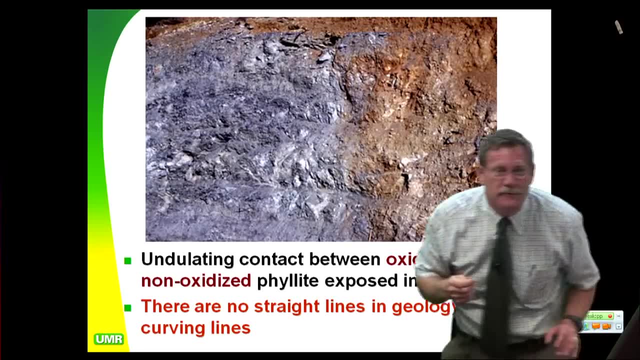 You're going to have an assignment. We've got to go out and make some observations. This is the kind of stuff I want you to observe. This is wild. Now, what would happen here? I send out the geotechnical engineer with a PhD from MS&T. 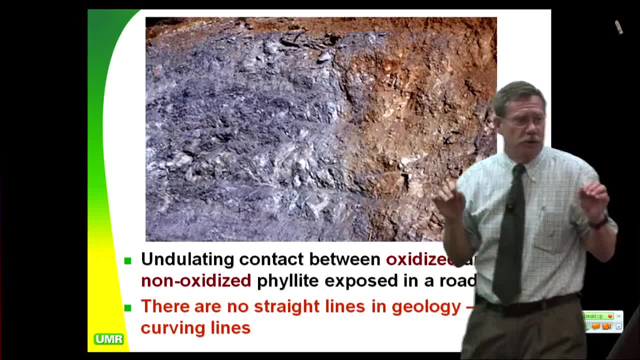 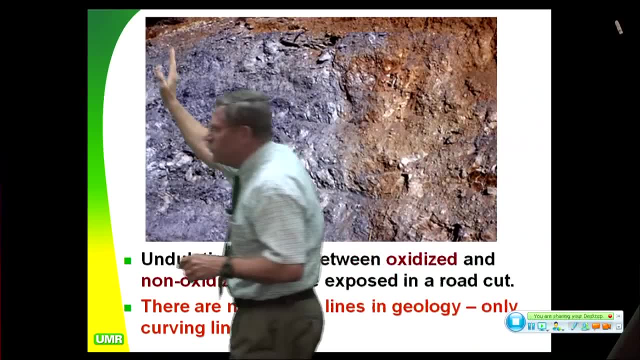 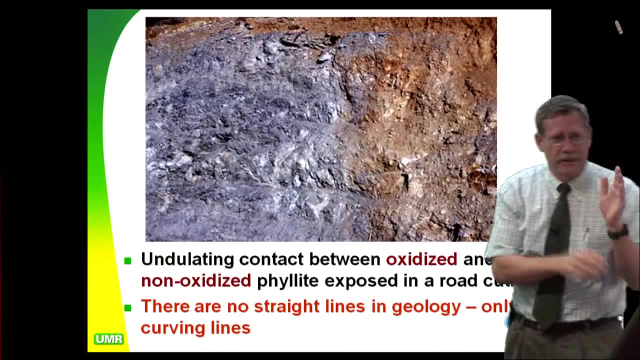 The name, the degree, the difference, And he drills a hole right here And he drills a hole right over here. What's a cross section? look like Two completely different materials with a line between them going. don't know what's going on. 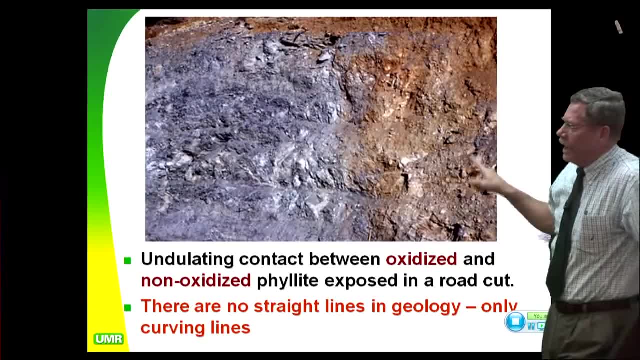 So it's a cross section drawn from this arrow. It depends if you use this drill or another drill or just use the hole and zoom it up What I want- So the drolet I want to deal with that Go down. It depends what the hole is. 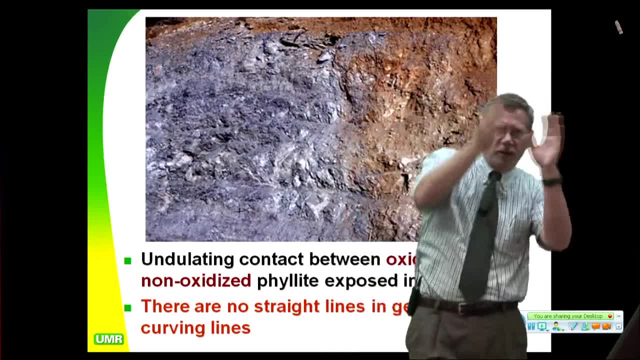 You're going to say, oh, that might be a bridge, Let's go go up to the成. A bridge is going to be a bridge. Shall we go next? Are we going to go vertical? Yeah Yeah, Welcome to the real world. 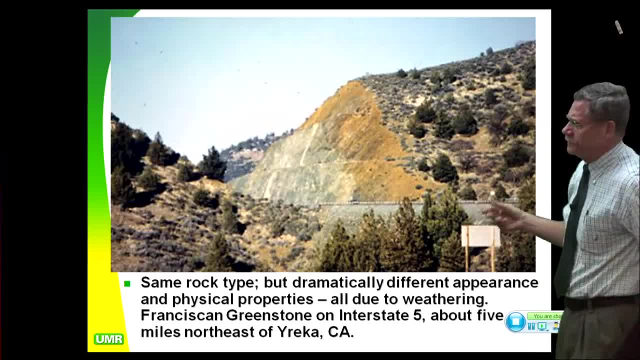 That's the real world. Highly undulating, contact. Highly undulating, Which is a big college term for moves all over the place. okay, All right. Here's another view: Interstate 5, coming down to the Klamath River Crossing, north of about five miles north. 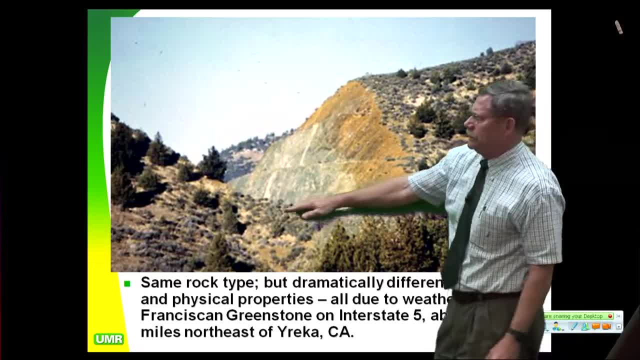 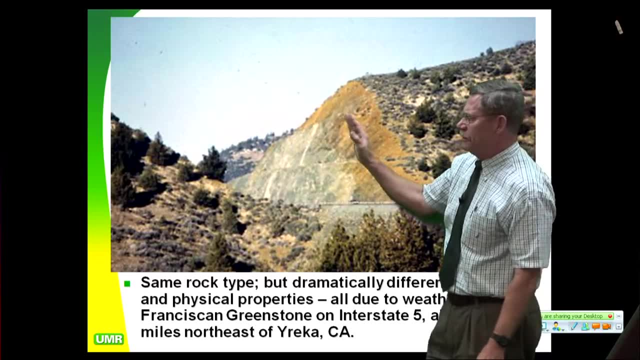 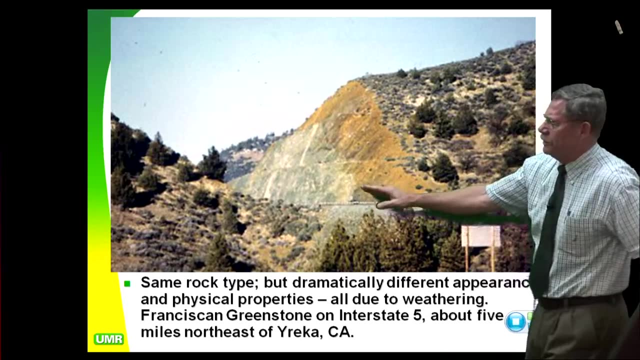 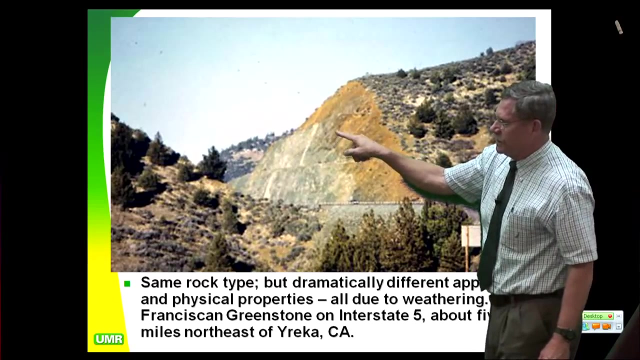 north of Wairika and we're seeing a green stone here cut about 200 feet high for a four-lane interstate highway. This material is the exact same material as this material. This is just the weathered zone. Now, that weathered zone is about 50, 60 feet thick. Now look at this. 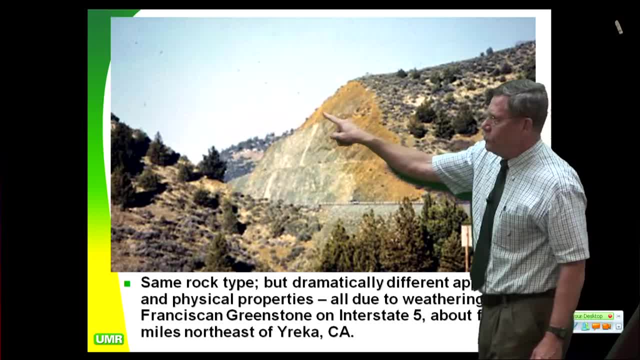 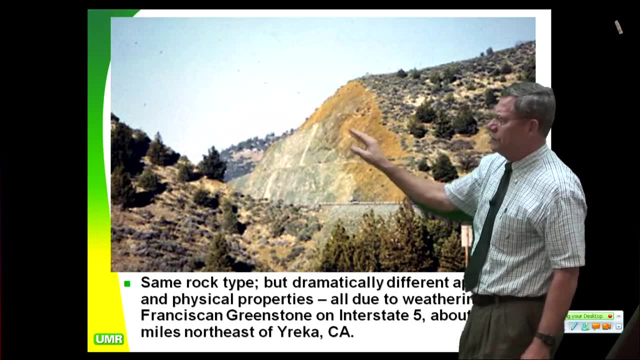 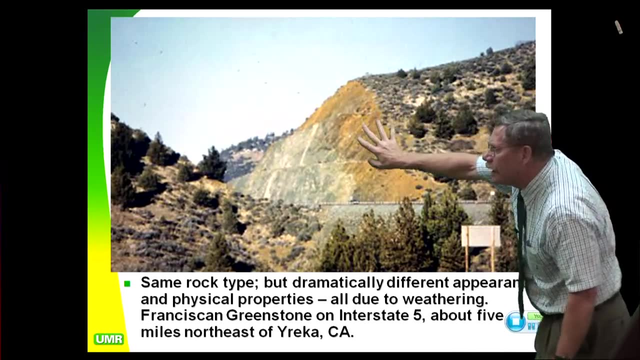 That's the contact Watch. You got to have some material here that's really resisted weathering right in the middle of that zone. But what's happening here is water is raining on this slope and percolating through and coming down through this stuff and you're having oxidation. You're. 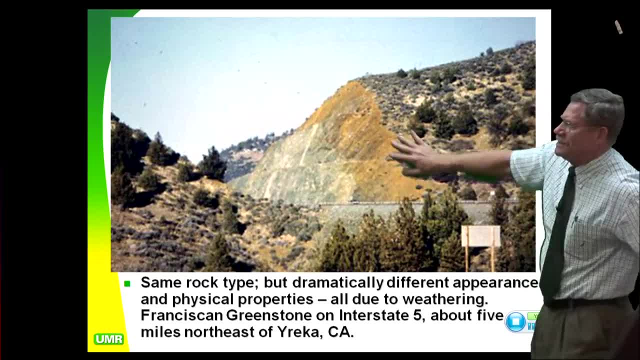 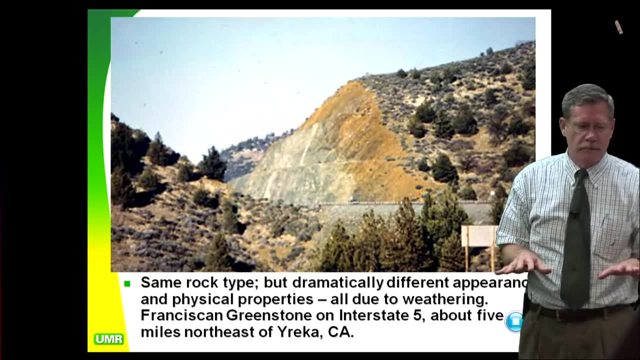 having cation exchange. This material is different material. It has a much higher permeability and it has a lower permeability. You're going to have more strength and you're going to have a lot more fines in it. You're going. 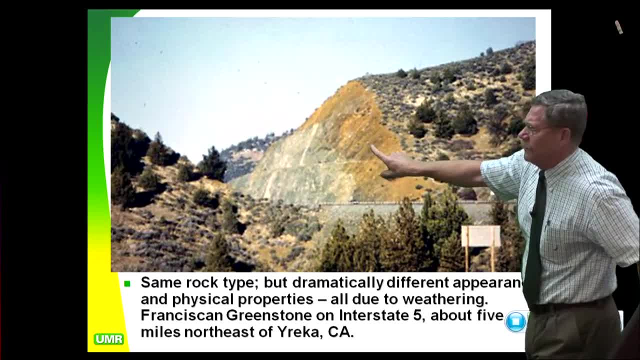 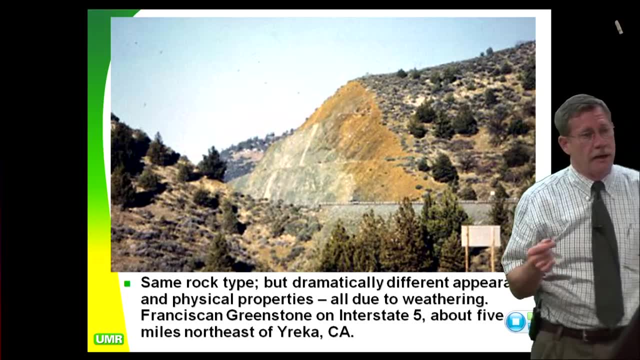 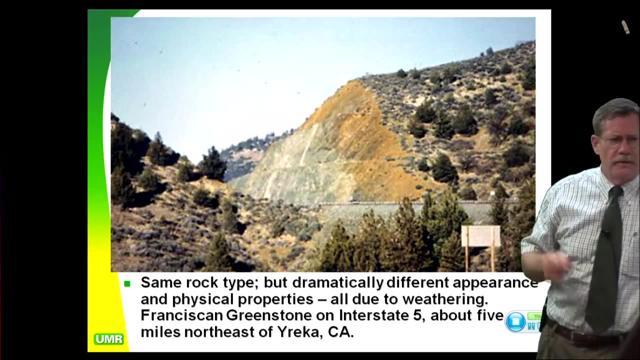 to have a much easier time excavating this green stone- weathered green stone- than you are excavating this green stone, And that's the kind of stuff we try to put in all our bids and spec packages. Well, how do you delineate between these things, Dr Rogers? Shearway velocity usually. 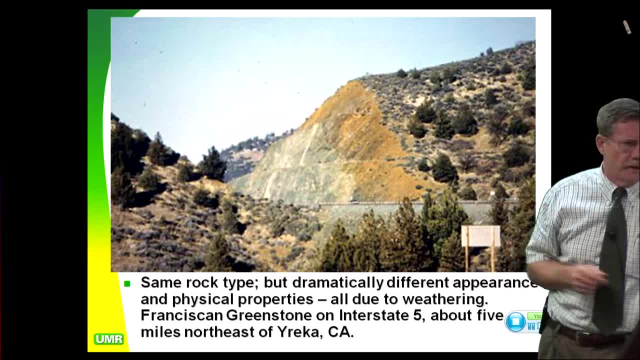 Use shearway velocity for excavatability. We cover that in the 441 class. So we go get all the old catapults. We go get all the old catapults. We go get all the old catapults. They all have crown-pillar tractor handbooks. Going back to handbook number 1, I think 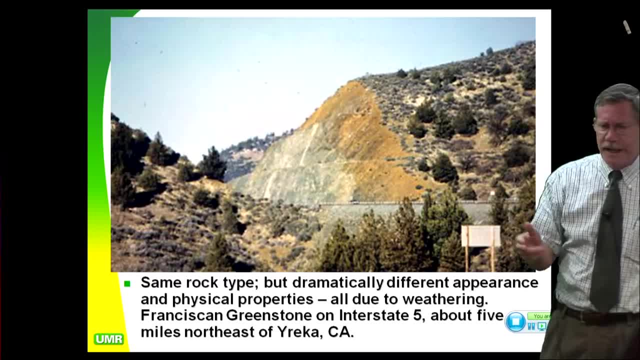 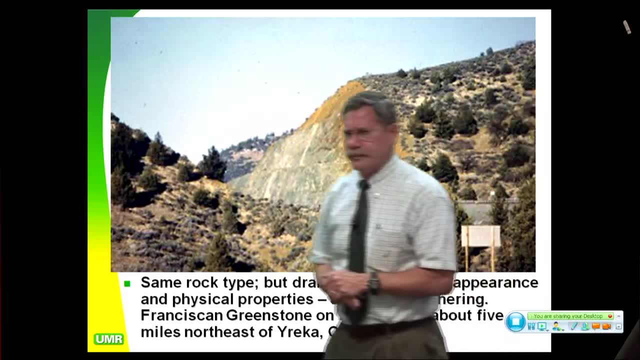 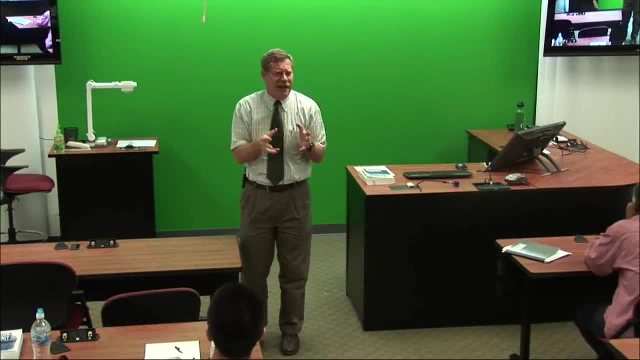 we're on 47, now 44,, 45 in there They have the shearway velocity versus ripability for different kinds of equipment. Of course CAT always wants you to buy the biggest, most expensive equipment, so you can't use this year or last year's CAT handbook if you've got a D8. You've 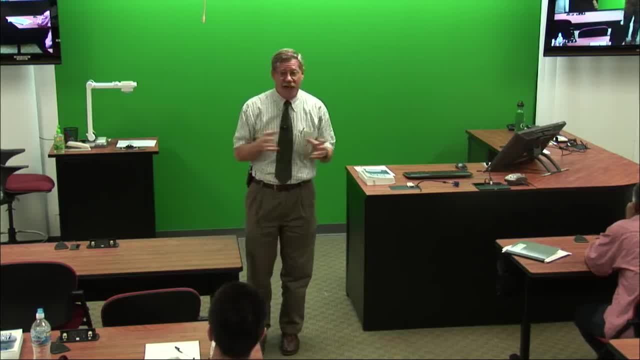 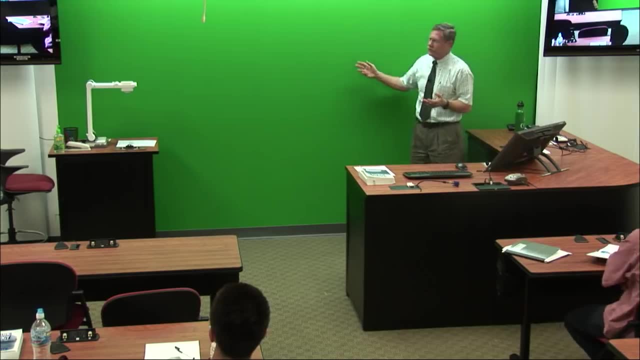 got to get back to 1977 and use a D8-H. You have to have the old book to see if you can rip it or but the rip ability is really important in a situation like this. so the rip ability of this material and that material you're going to get paid four. 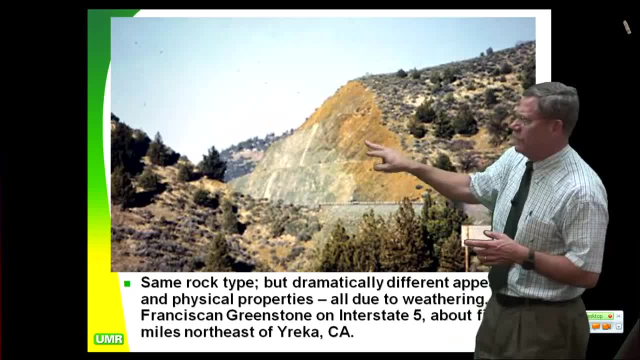 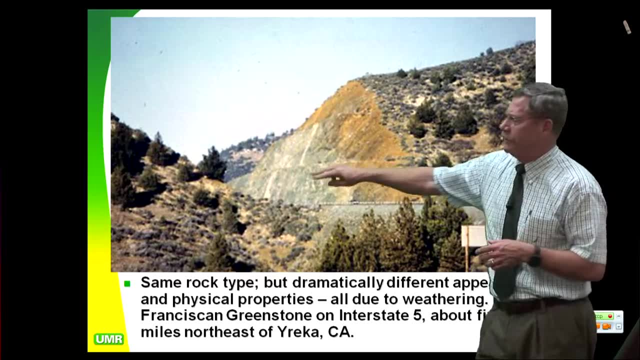 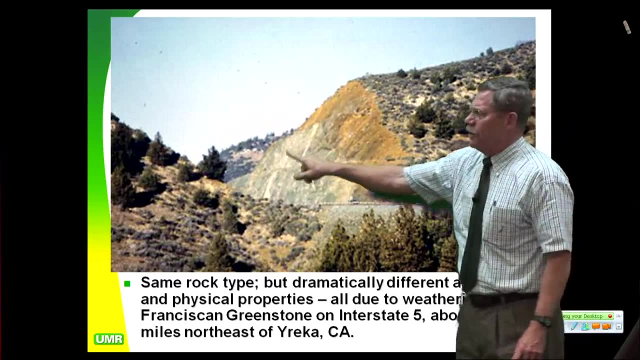 or five times as much to remove this material as you are. that material and this material is going to be an order of magnitude higher permeability or two orders of magnitude than that material, because that material, the joints and this stuff are all cemented by calcite. so that's why it's not getting weathered. 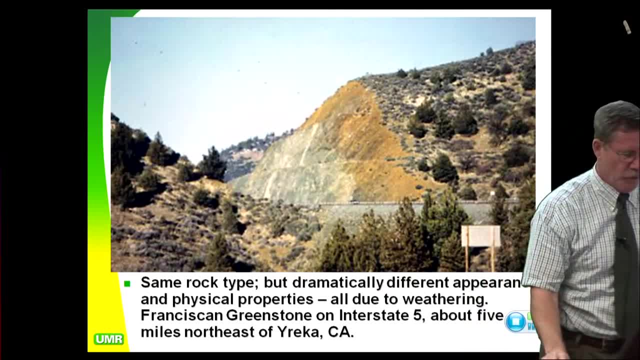 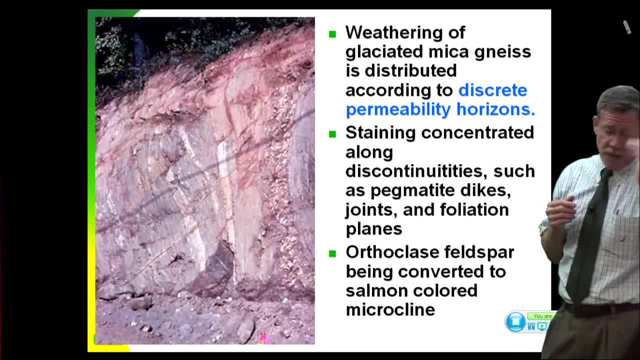 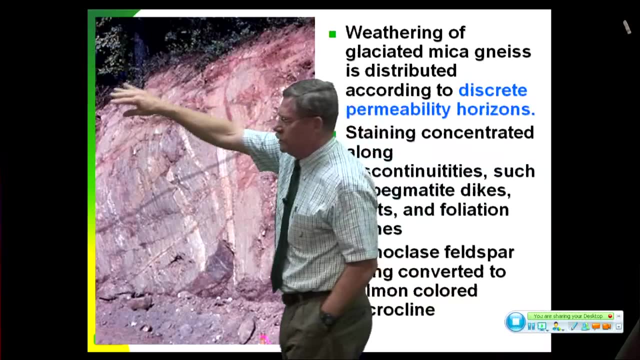 cemented by calcite, it's in the rain shadow, doesn't get enough water. okay, here's another case. this is actually over in, or I'm in the snowy mountains of Australia and this particular picture and I have, I'm in Granite's here and you can see how things get booted up up here by the creep zone up on top and then 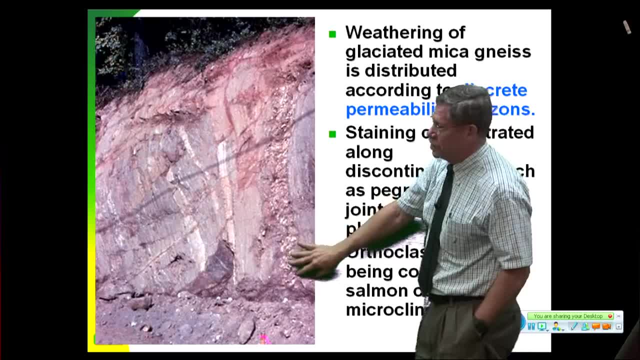 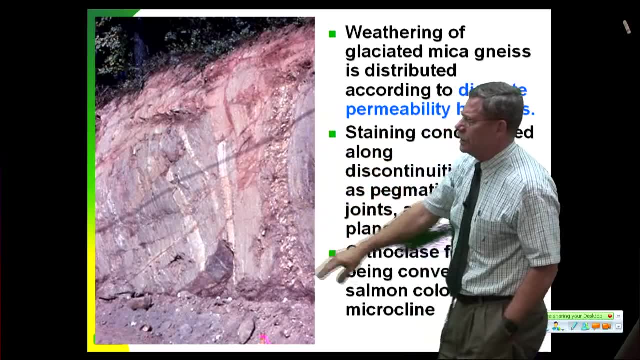 this is a pegma type dike in the granite, much different from the granite dike. you can see how things get occurred up up here by the creep zone up on top. and then this is a pegma type dike in the granite, much more porous, and so I have more of the feldspar staining in here. The orthoclase is being converted. 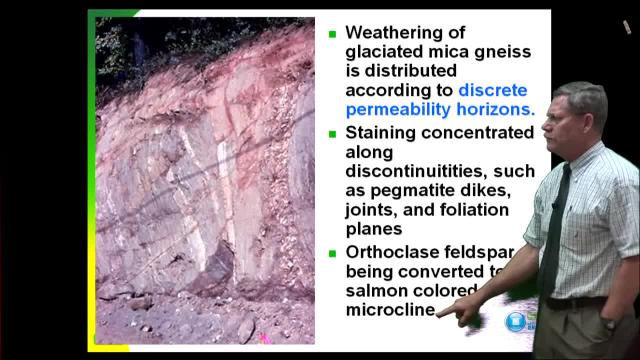 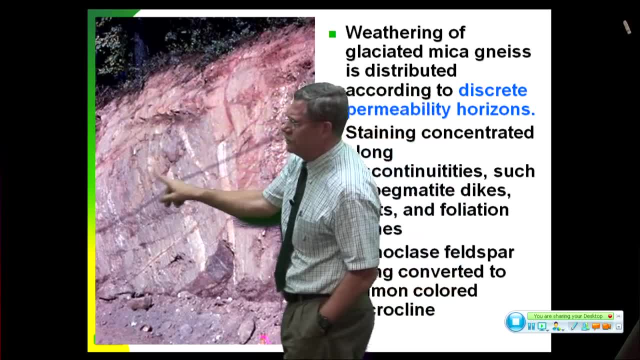 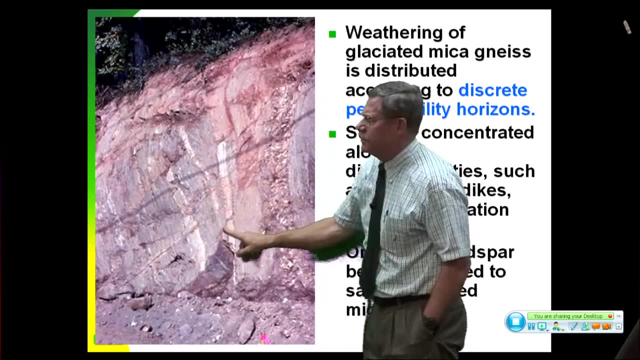 to the salmon-colored microcline feldspar, and you can see here a very definite zone right in here where it's more weathered. and then you have these little stringers here and there, especially along joints where you have more water. Water travels through the joints and so you're going to get a. 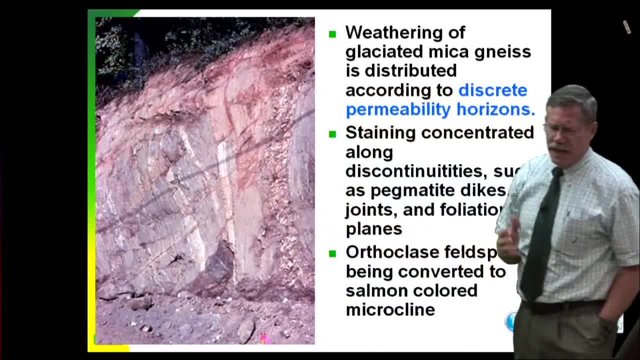 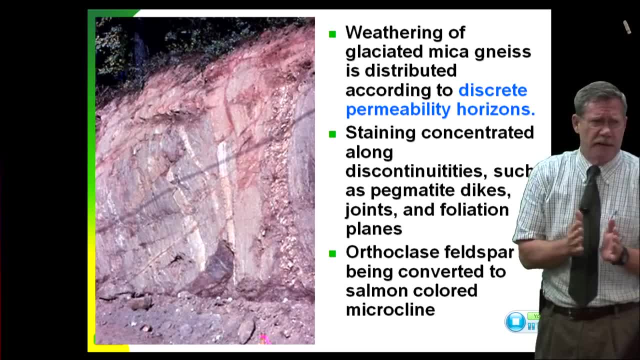 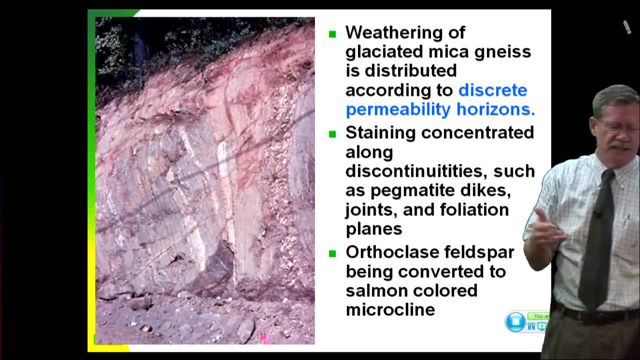 little more weathering along there, a little less strength. Now you can have healing of joints, especially by iron that makes them stronger. That's like injecting superglue, but that's the minority. Most of the time the process of fluids running through there actually weakens it. 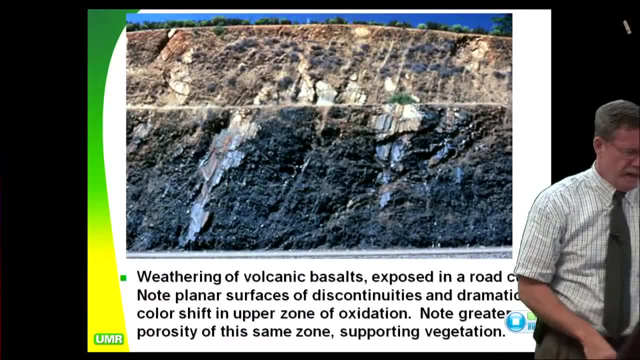 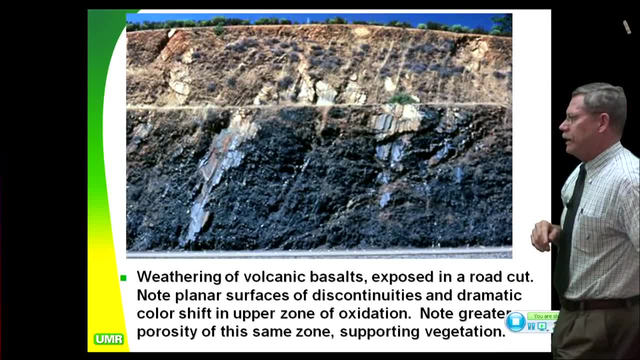 instead of strengthening it, but not always. Okay, here we are in Hawaii and this is a fairly recent highway cut for DeWilson- DeWilson Tunnel- done back in the late 50s, early 60s, and if you look at this same cut today, you 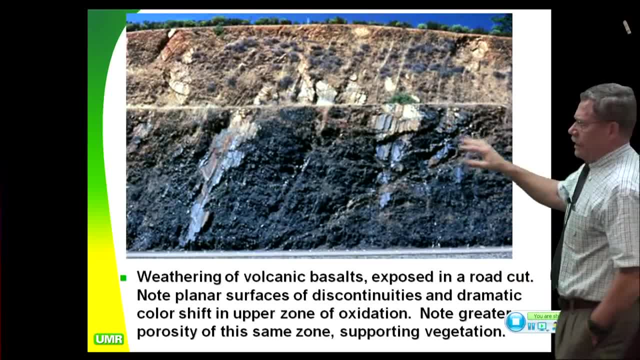 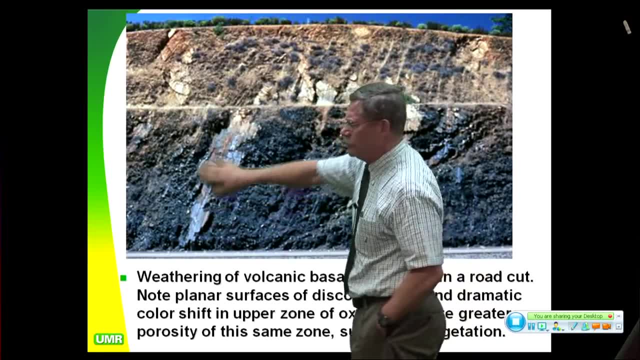 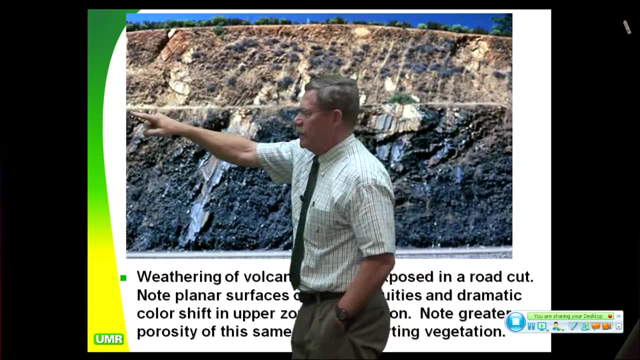 can't see anything. It's just covered with jungle. but this is looking at the Koolau Volcanics and they got some of these big joint surfaces here. Here's a big joint surface. You can see where they had a planar failure here. but as we go up towards the original hillside we can see we have an. 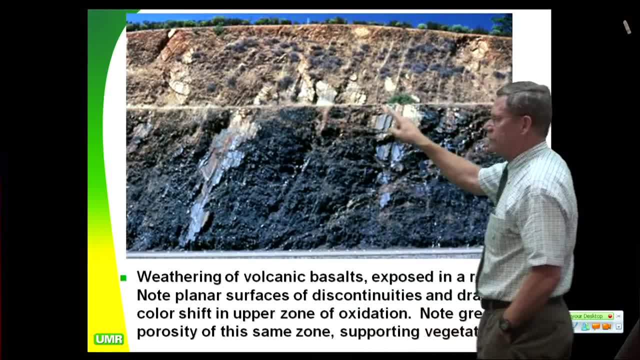 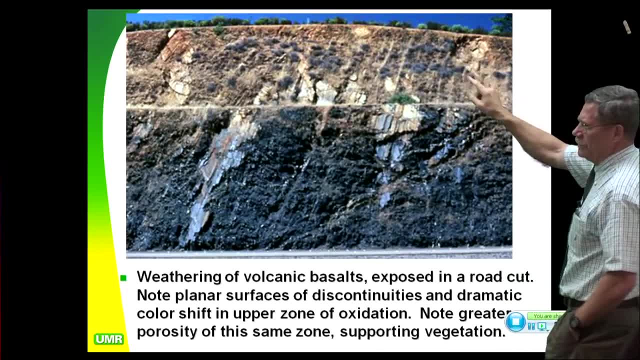 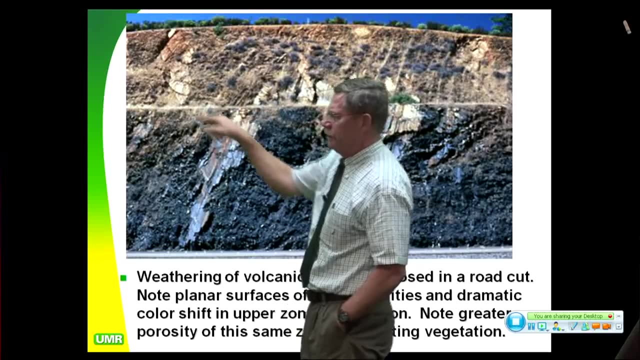 undulating series here. Now, the reason why we have this is because of the weathering And this material up here you can see these little shallow pop outs that have been occurring right here. This material is much more weathered- there's another one where they have a pop out, come out eroding here- than the material down here. 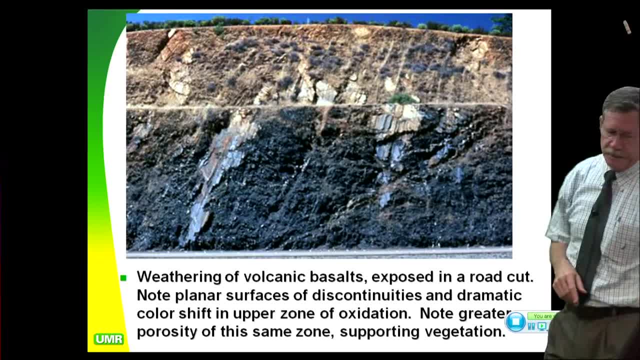 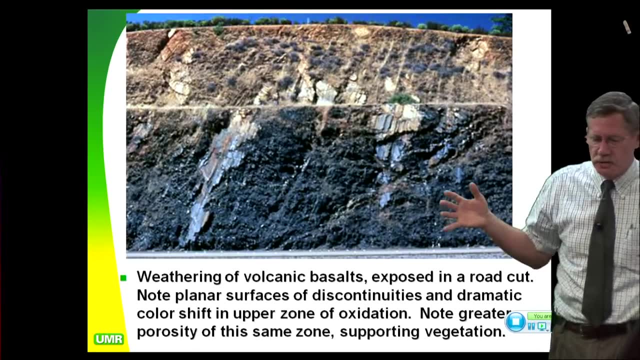 So it's all the same material, It's all the same Koolau, Volcanics, but the porosity impacts the weathering. Now, volcanic rocks are extremely porous. They are just like the volcanic rocks. They are extremely porous. They are just filled with joints, Ubiquitous jointing, because they shrink so much as they cool, and they cool very, very rapidly. So you get lots and lots of joints. You don't want to build dams on volcanic rocks. Just don't go there. It's like building dams on cars. You can do it, but your brother-in-law better be the grout contractor. 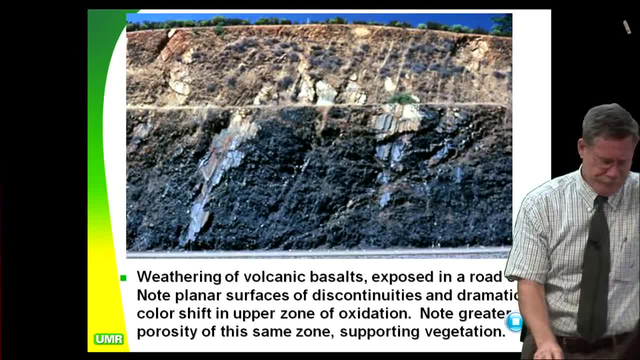 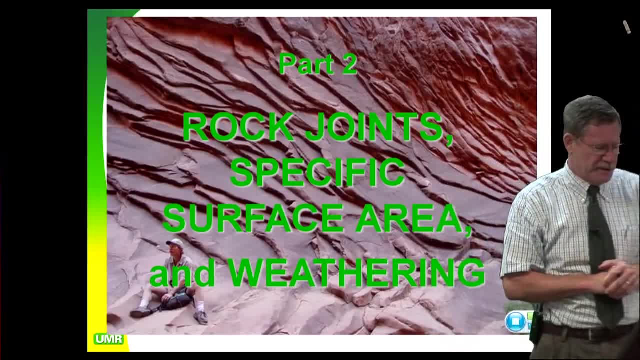 and you're getting a kickback from them because you're going to do a lot of grouting. All right, 544 pm And we're going to start on rock joints. Rock joints: specific surface area and weathering. 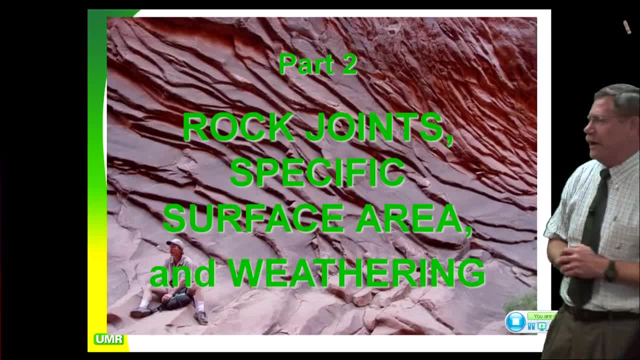 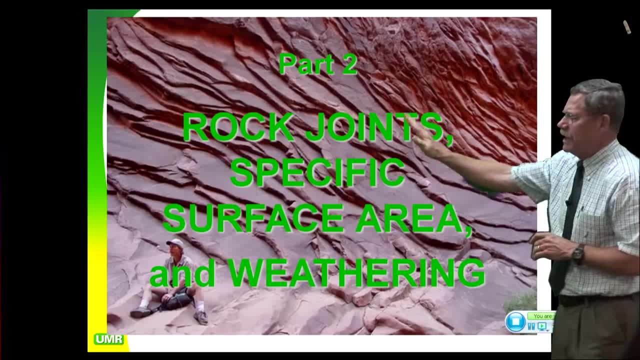 Here I am in a place called North Canyon That's a tributary in Marble Canyon, Upper Grand Canyon. I'm in the Esplanade Sandstone. It's a Pennsylvanian age, Remember, it's a quartz aranite. 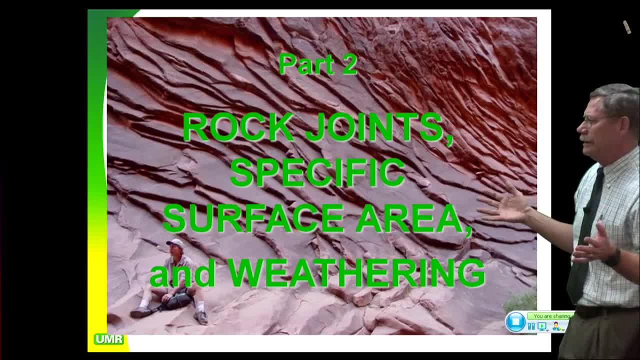 Look at how prolifically jointed this rock is. I want to tell you something: That's the strongest sandstone. It's the strongest rock in the world. It's the strongest rock in the world. It's the strongest rock in the world. 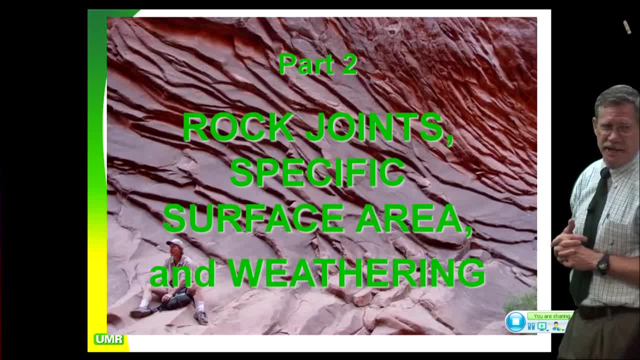 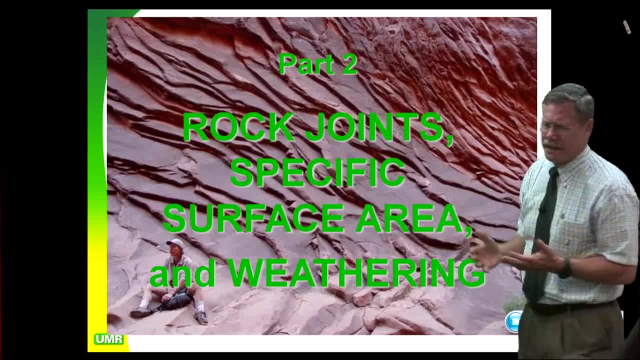 It's the strongest rock in the Grand Canyon. What The strongest sandstone has the most cracks in it? Yep, Yep, it does, because it's got very low strain threshold. It's not mushy, So this stuff has been excavated by a natural channel and it's exfoliating. 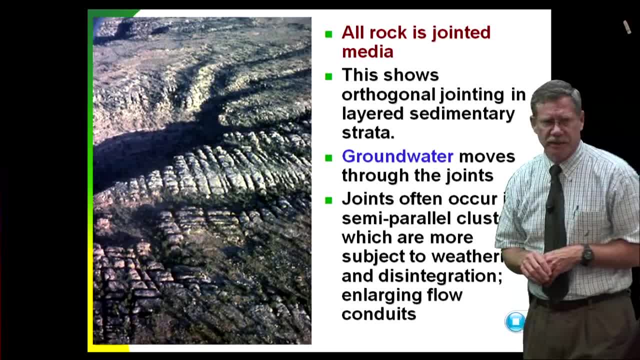 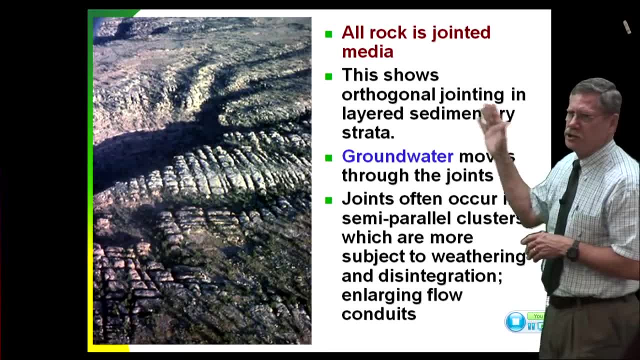 And no, you don't just get exfoliation in granitic rocks. That's another fairy tale that we get in some of the physical geology books. All rock is jointed media. This shows the orthogonal joining in a layered sedimentary strata. 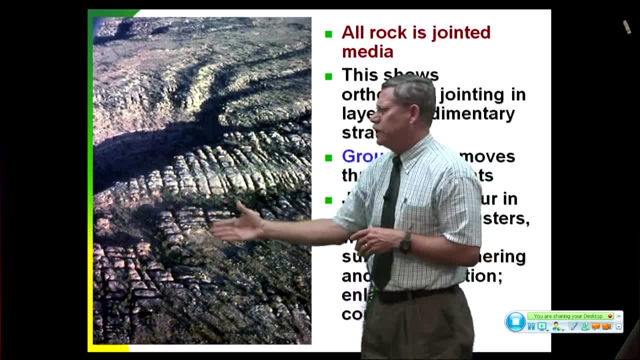 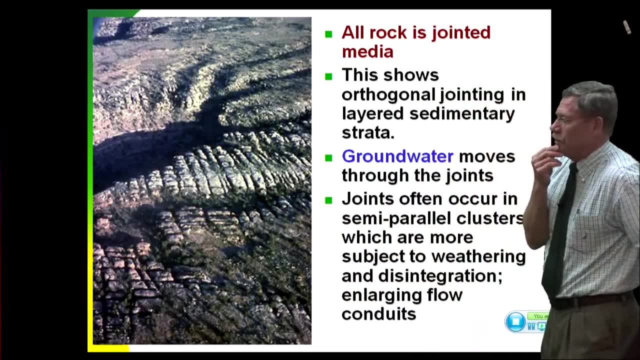 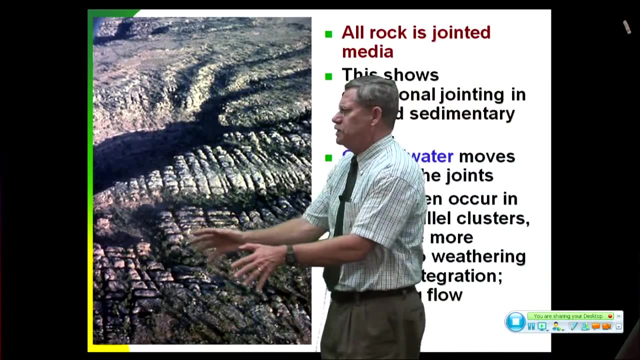 And groundwater travels down these preferential paths, So groundwater in this case. I'm flying over the Green River Canyon near Green River, Utah, And what's going on here is groundwater has flowed down these regional systematic joints and it's solutioned out. 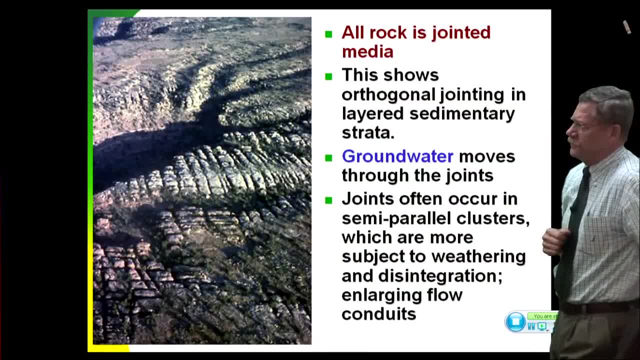 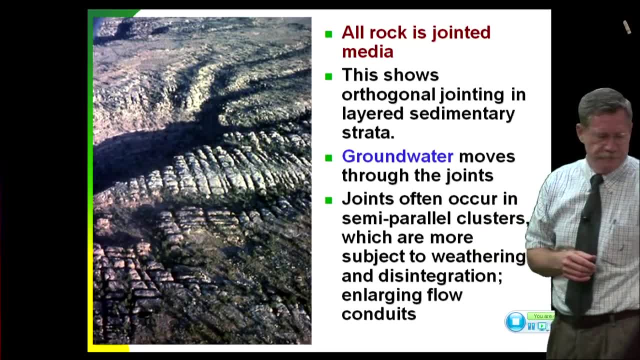 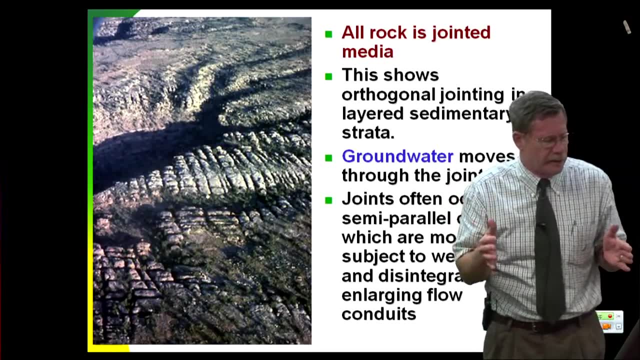 These corridors, these preferential flow corridors, So you have weathering and disintegration and it's enlarging those flow conduits that are sitting there And you can see any of these things in remote sensing data. You get remote sensing data in a semi-arid area. It's very easy to see the near vertical joint suites. 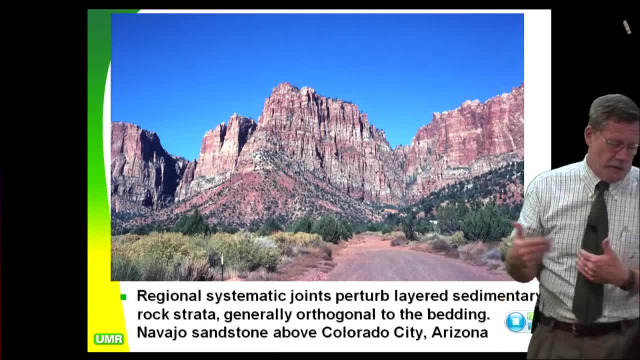 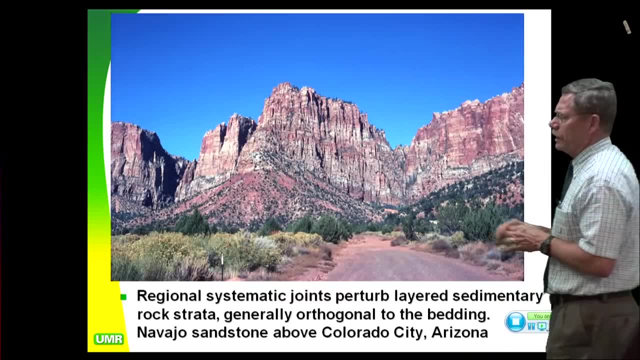 They're not hard to pick out. Now, here we are on the ground, and so we got another view. here We're on the ground, We're near Colorado, We're near Colorado City, Arizona, along Short Creek, And we're actually looking at the Navajo Sandstone. 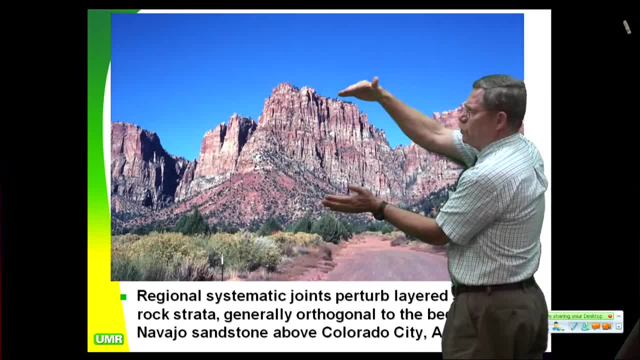 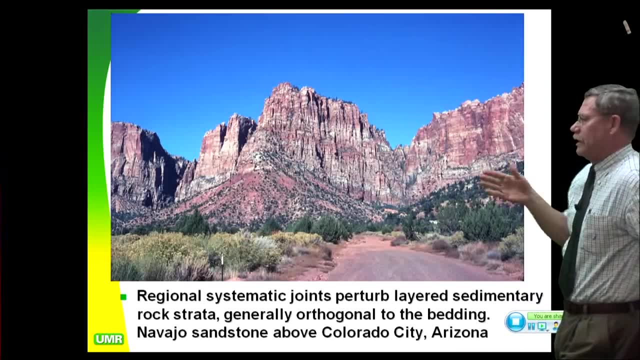 That's a Jurassic unit. It's about 2,300 feet thick. in this part of Arizona, Utah, We're right near the Arizona-Utah state line right here. Utah is just to the right here out of the picture. So what we're looking at here these are joint faces. 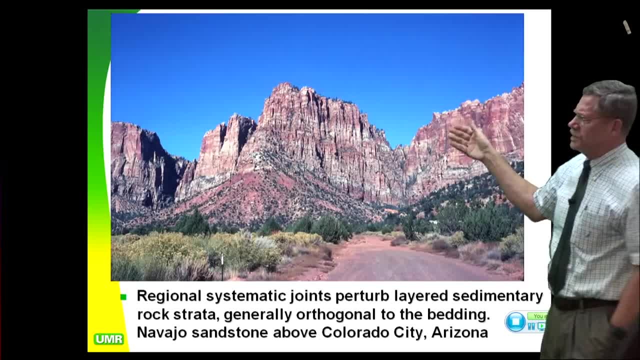 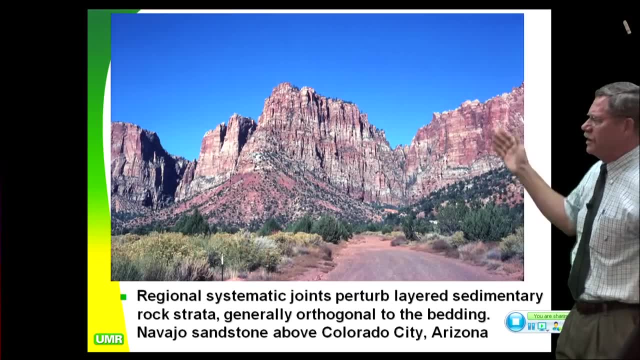 This is a sheer joint face. Most of the time when you go to a place like this, This is just south of Zion National Park. When you go to places like Zion or Yosemite, Rocky Mountain National Park, Glacier National Park, what you're usually seeing are joint faces. 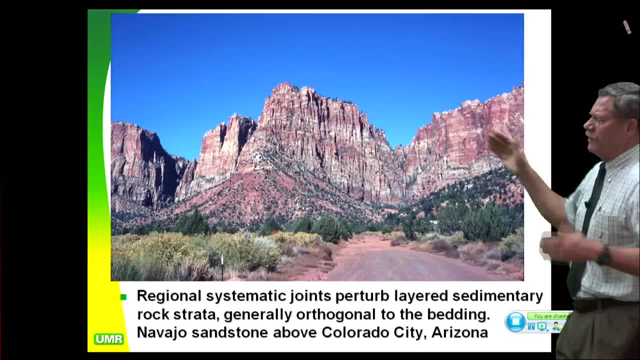 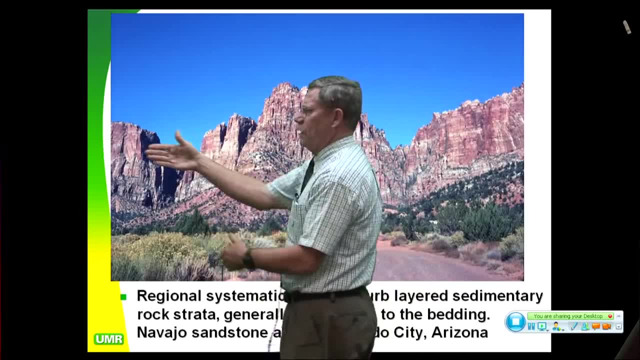 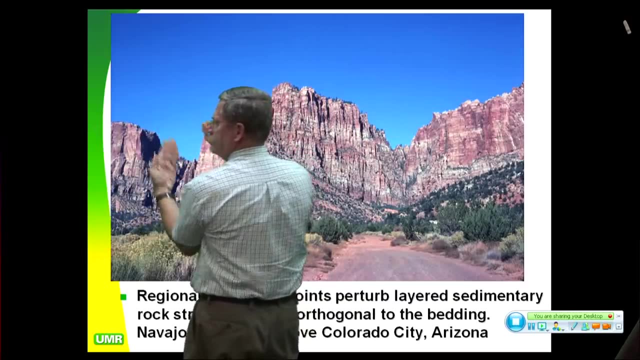 These are huge, regional, systematic joints So they have very regular geometry. Right here you see one joint going down big, huge face And right over here is the joint. that's almost 90 degrees of that, believe it or not, going this way. 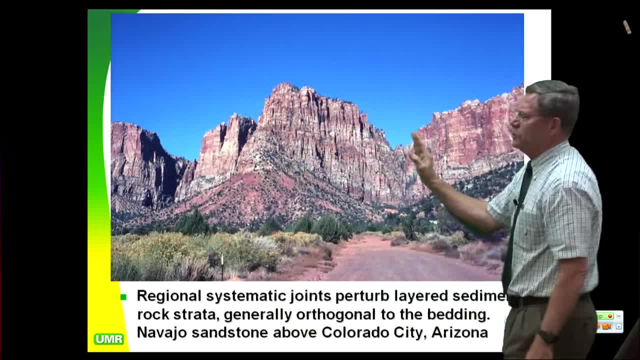 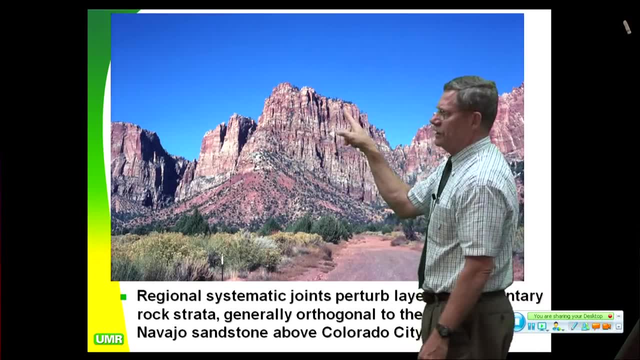 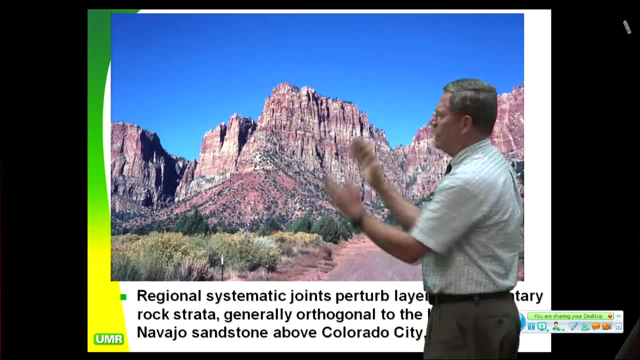 This one's going that way. What I'm seeing here is a very unusual in that this is a face that's transverse to both joint sets. So what I'm seeing here is thousands and thousands of 2,000 foot high joints, And they're actually crisscrossing one another like this across. 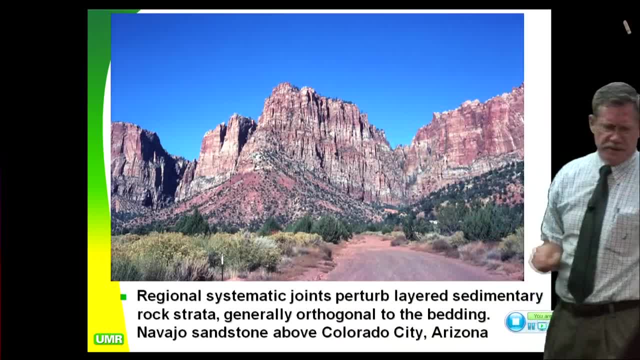 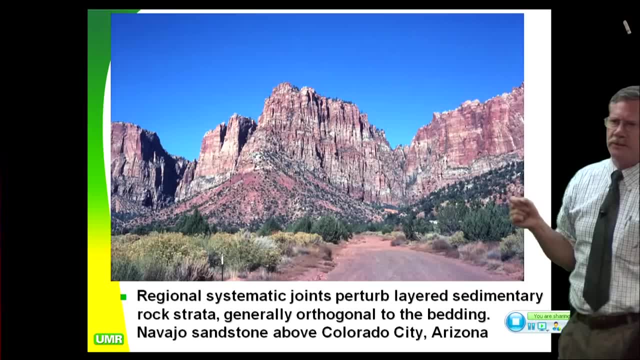 And so what you see here, I want to get through to you, is all massive rock is jointed And fluid flow goes through the joints. When I first started serving as a consultant to EPA years ago, I didn't want to have anything to do with the geo-environmental industry. 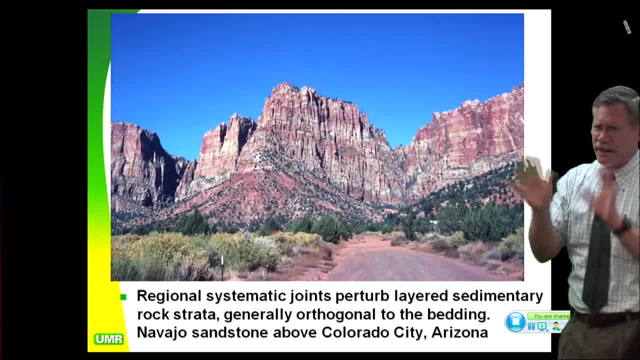 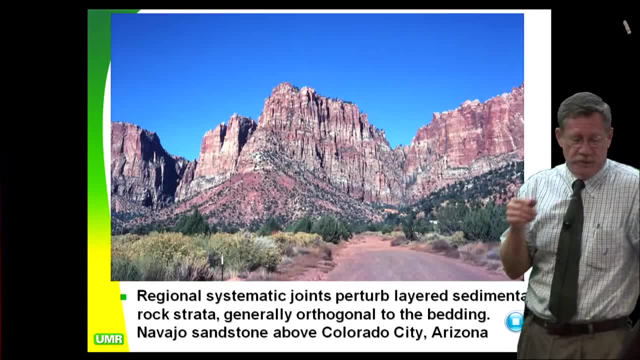 It just isn't sexy to me. It's not like doing the combat engineering I do on sliding highways into the Pacific Ocean and stuff. But I got roped into it through a friend who was doing Lawrence Livermore National Lab And they were having all these problems. 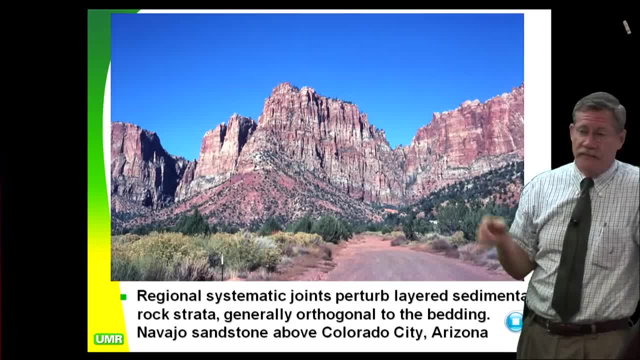 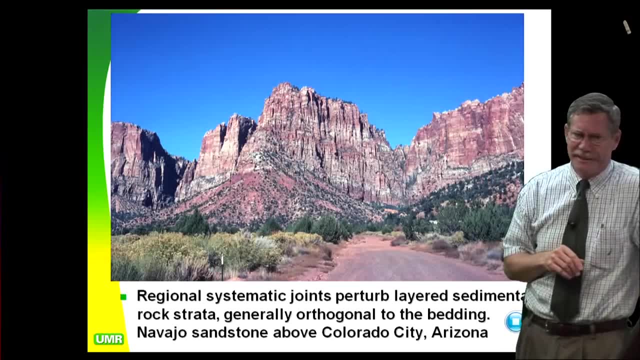 And so I started becoming a technical referee on these very difficult lawsuit cases that the EPA had on landfills, especially places like Texas. And you had these guys. you know they were soil mechanics, people with no background in geology or rock mechanics. 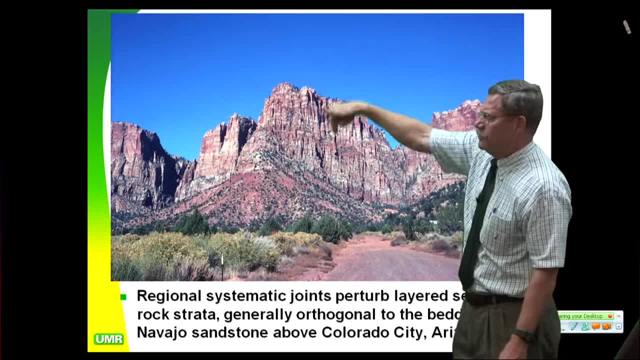 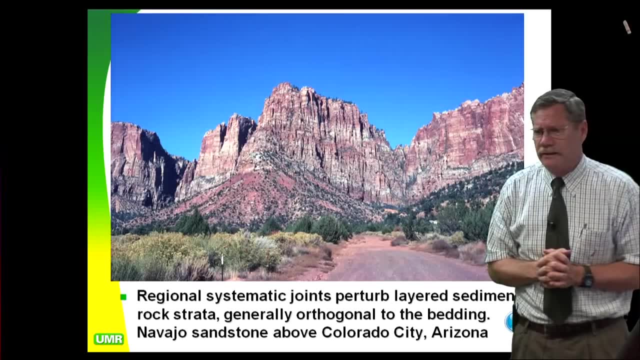 And they're going out into sites like this and drilling vertical holes and then saying there's no leachate leaking out because they didn't encounter any leachate in their vertical hole. Now, kids, here's a joint surface. Here's a joint surface. 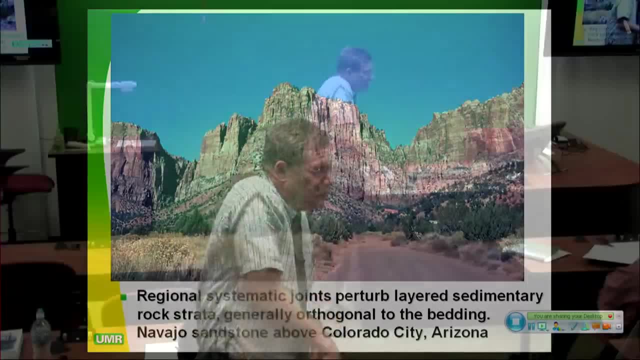 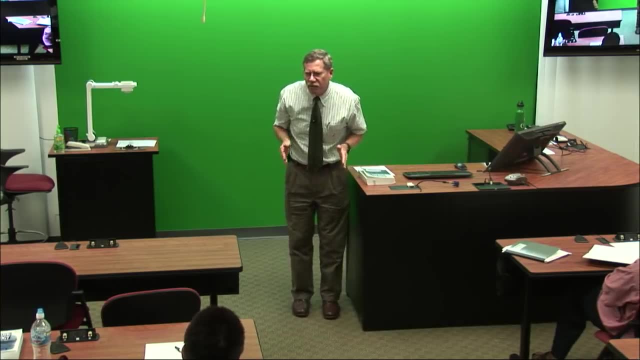 All the fluids go along the joints. If you drill a hole right here, you're never going to see them. Vertical holes in vertically jointed rock is the work of a moron. Shouldn't even have a PE license. That's stupid. That's wasting your client's money. 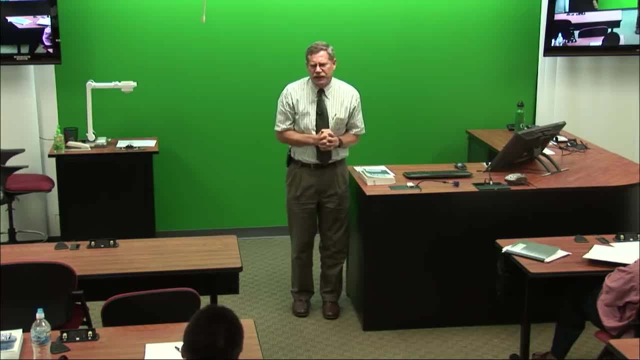 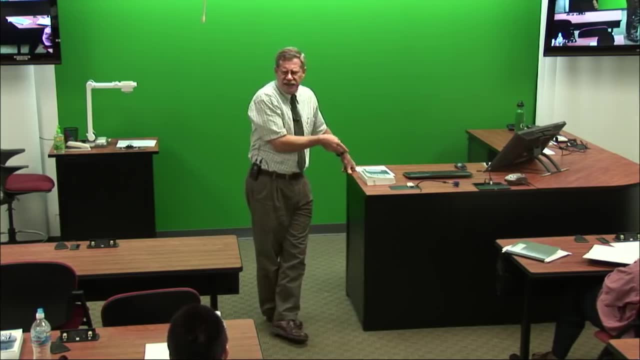 Horrendously wasting. I wrote some stuff like that. That's why I had to move to Missouri And people wanted to kill me. I'm not kidding. What do you do in a case like this? You have to do angled holes. 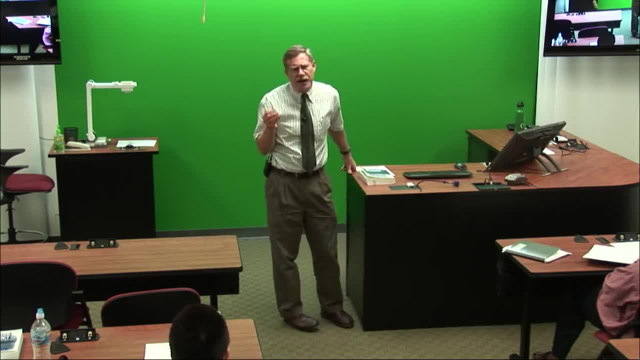 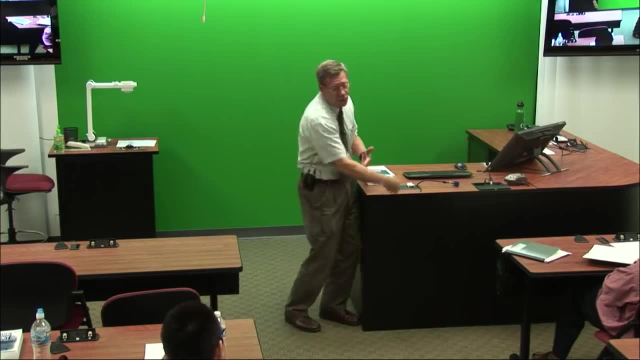 You're going to mess around with trying to find dense, non-aqueous phase liquids who are sliding down the joint surface. You've got to do angled holes so that you pierce all the joints, Or you pierce some of them at least. 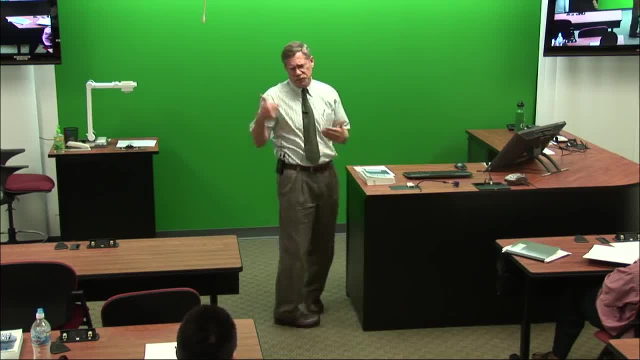 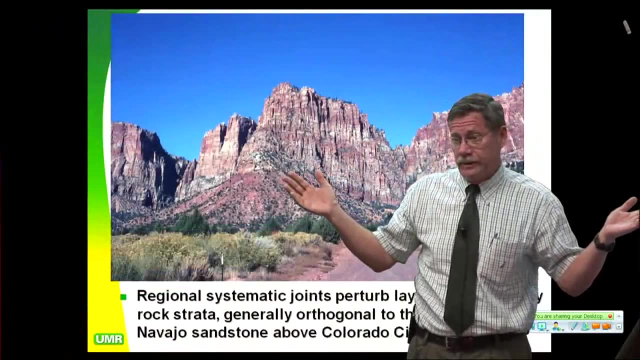 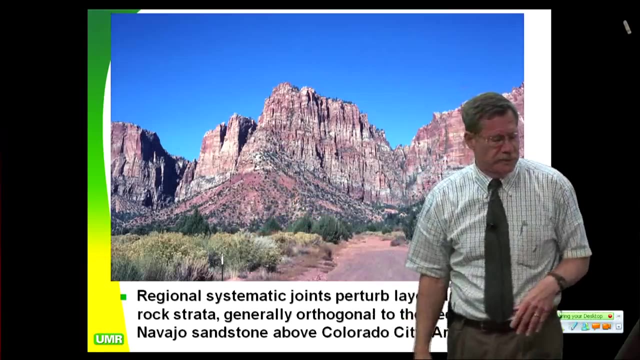 Do an angled hole, 15 degrees, go through and then do your sampling. Now, as soon as we made these applicants do that, everything changed. It's pretty sad. You had an industry there that was just expanding so rapidly. they weren't bringing along the right kind of expertise. 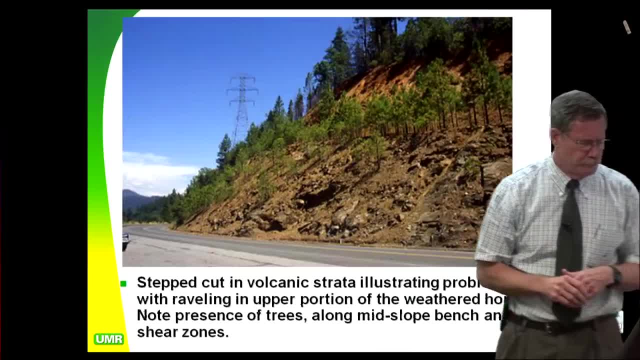 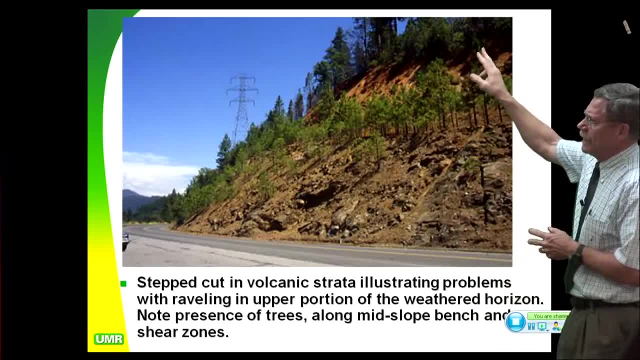 That's why you have to have third party peer professional review. Here's a step cut in volcanic strata that illustrates some of the problems in raveling that are real, typical on highway cuts, Or any kind of cut for that matter. 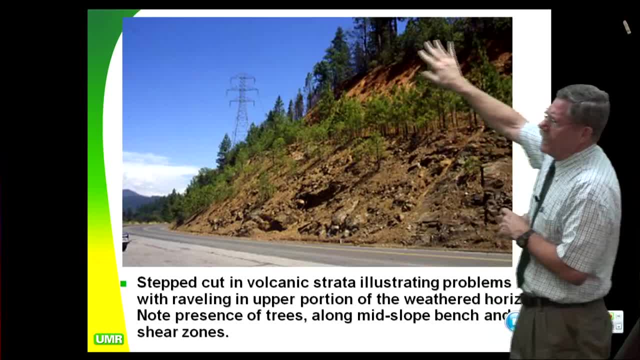 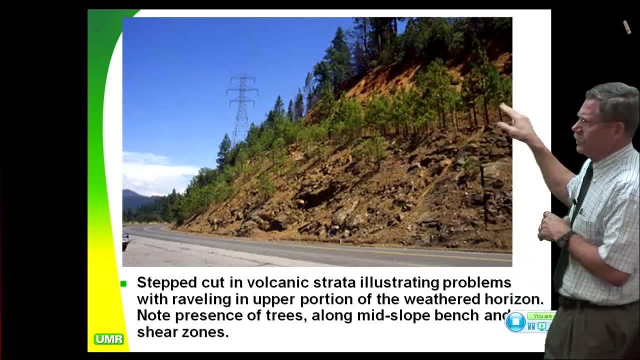 Most of the weathering is going to be in the upper part of the cut. This is where all the action is going to be. This is where everything goes wrong. Most materials come down and they either clog up your bench up here, your drainage bench, or they come sailing down and make it all the way down to the highway. 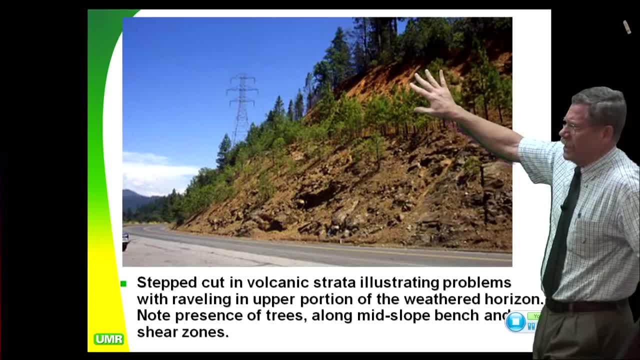 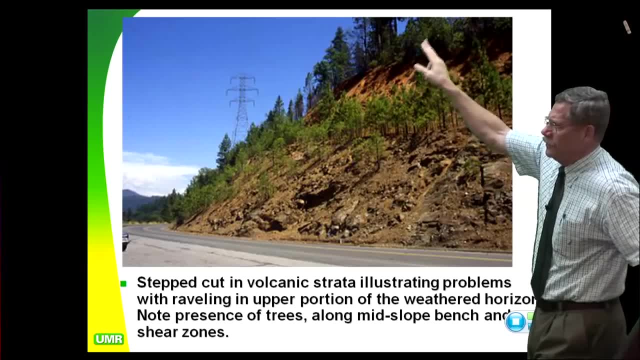 It's the kind of stuff that drives us nuts Because it's very hard ahead of time with a typical geotechnical investigation, very hard to come in here and predict how much raveling trouble you're going to get off this thing. 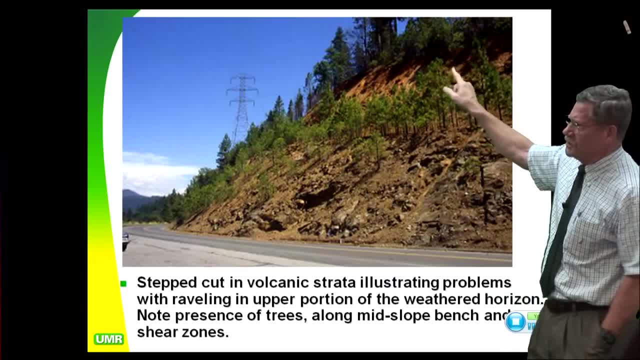 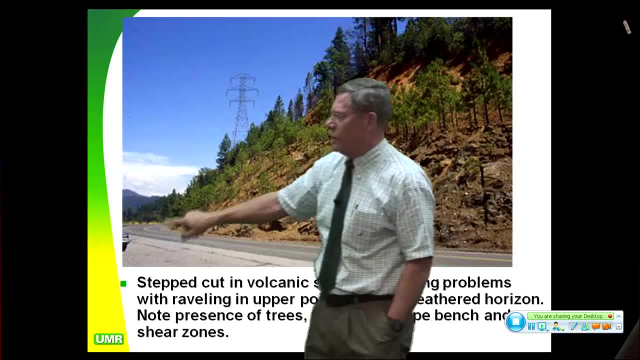 You've got to realize you get one rock up here that loosens up and comes bouncing down here and through conservation of momentum, it can come bonk, kabonk, kabonk right onto the highway. somebody hits it and they become a quadriplegic. 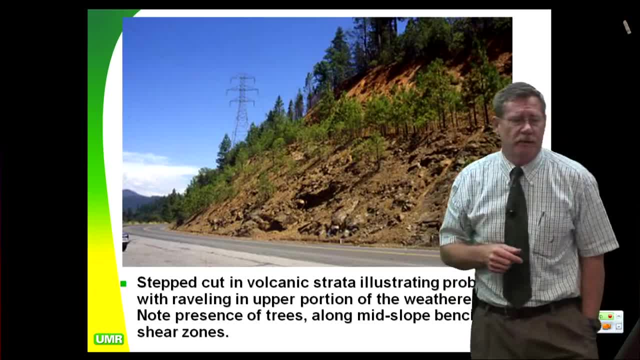 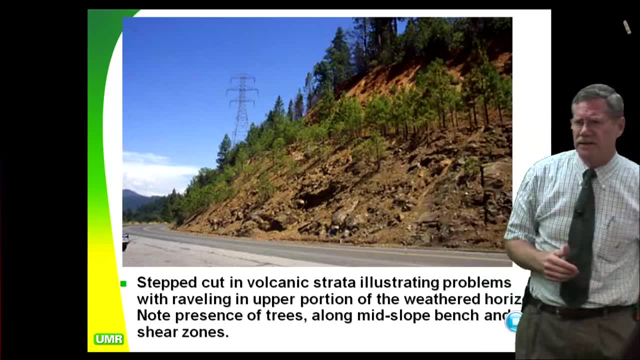 You're out $20 million paying for their medical bills. Now we've saved some money on the slope here by not shaving this back. We saved, you know, $30,000.. We just lost $10 million in the first accident. 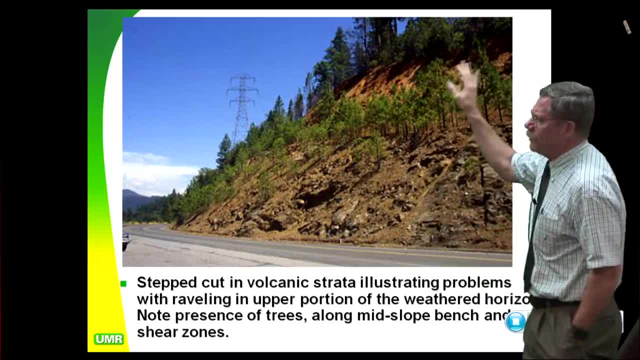 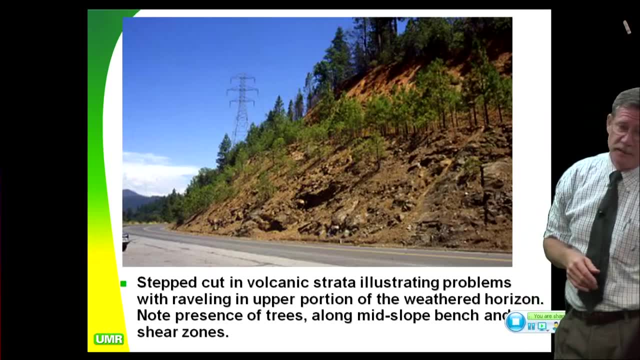 So you've got to look at what's cost effective Now. back when they were doing this kind of work in the 60s, they were assuming these cuts had a life of 20 years. That's ridiculous. I mean you're looking today: 75 years- pretty much a minimum. 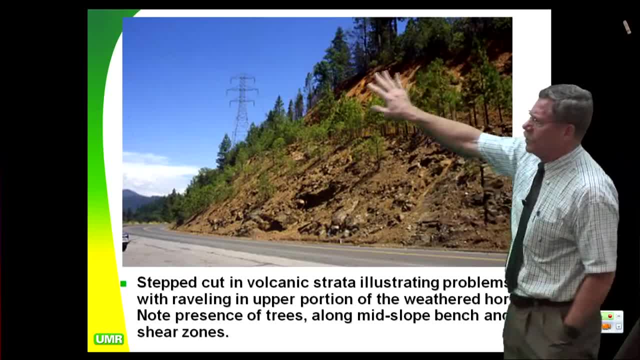 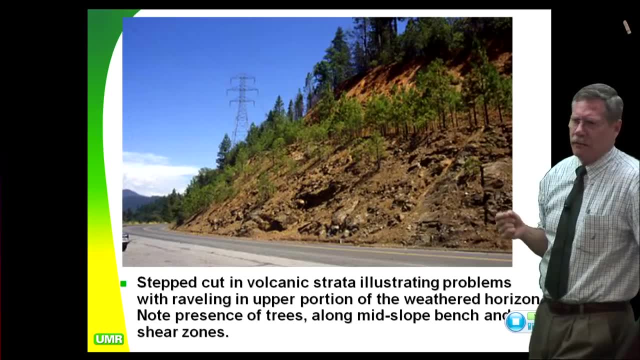 But we still don't have good numbers on erosion rates and weathering and aging effects. That's the one huge area of geotechnical engineering we're not doing real good on. We can't go out drill holes in a couple days. take the samples to the lab. 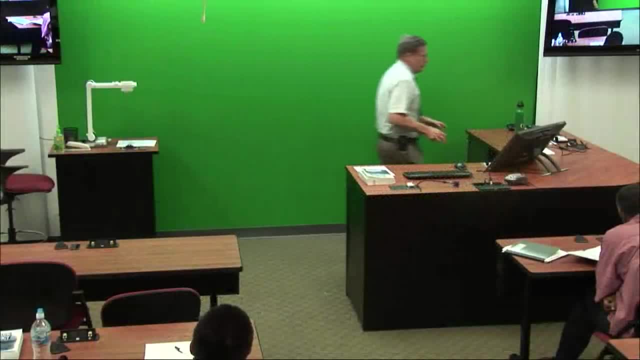 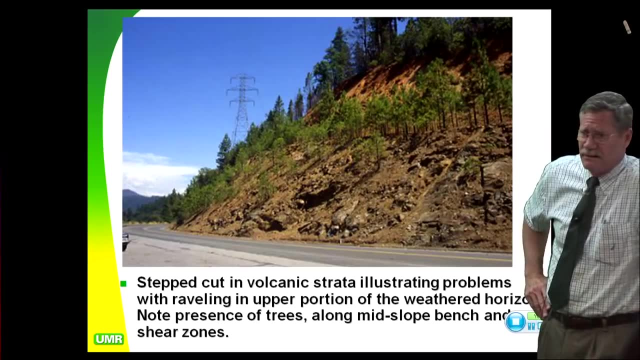 run a bunch of tests in the lab and get the report out all in less than three weeks and tell you how the site's going to behave over the next. you know, 37 years, 67 years, You know you can't do that. 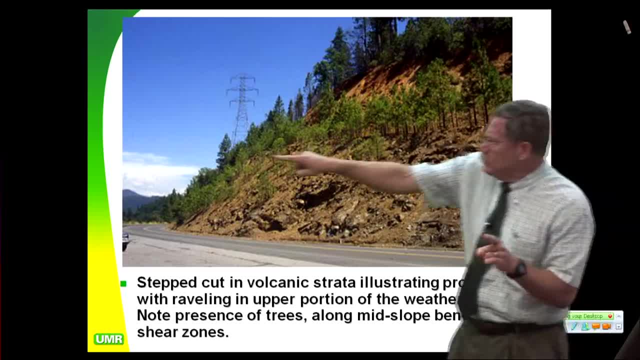 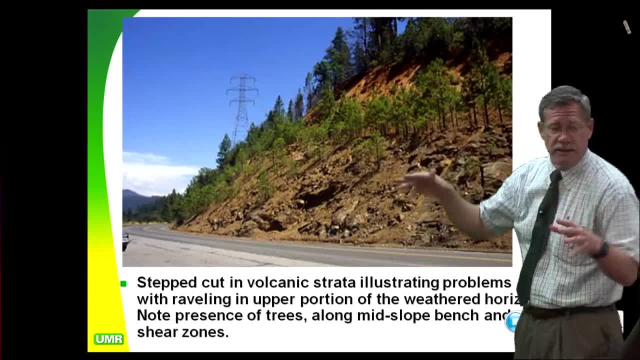 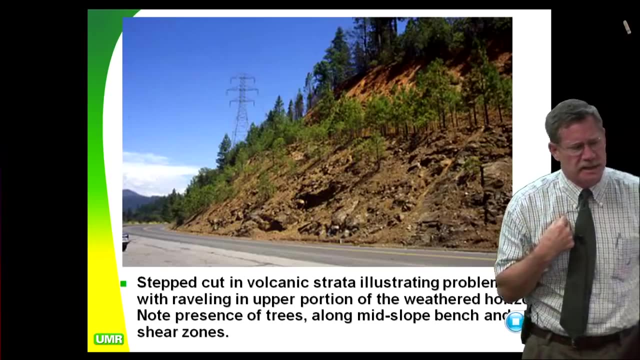 The only way you can tell that is to get your butt out here and look at the slopes in similar geology, similar hydrology situation to your project site and see how they've done Everything that I've learned about my business. that is really important. 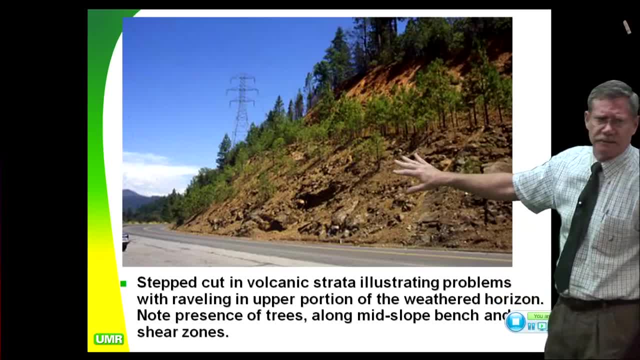 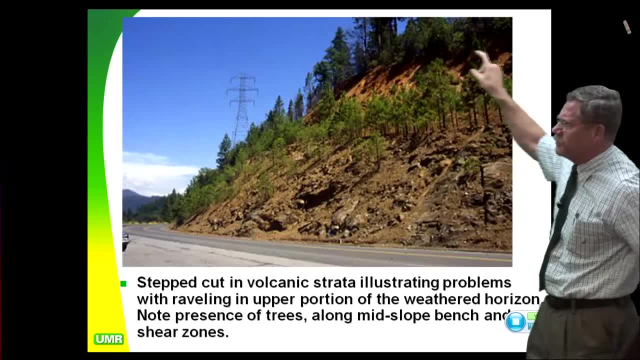 has come from direct observation and experience. It didn't come from the classroom. It came from going out and looking at slopes like this one, going up here and making some measurements and going- this is colluvium up here, by the way. 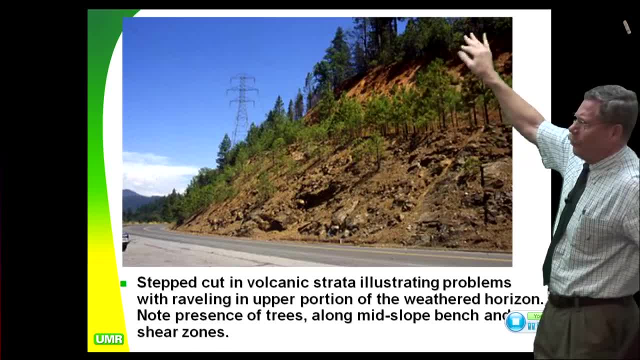 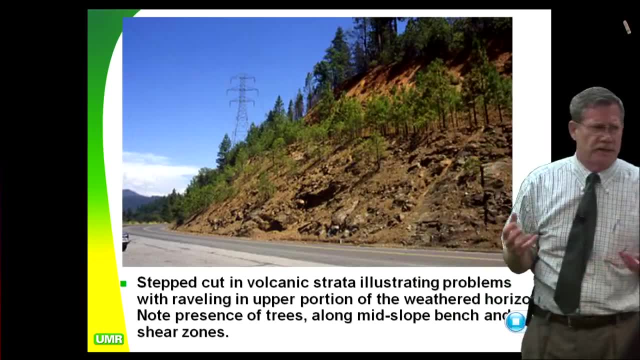 This is soil And they left it in at a one-to-one cut slope. Soil doesn't stay on a one-to-one cut slope unless you can keep the moisture in it. keep some negative pore pressure going, keep it there And what happens is when the water spills over this thing. 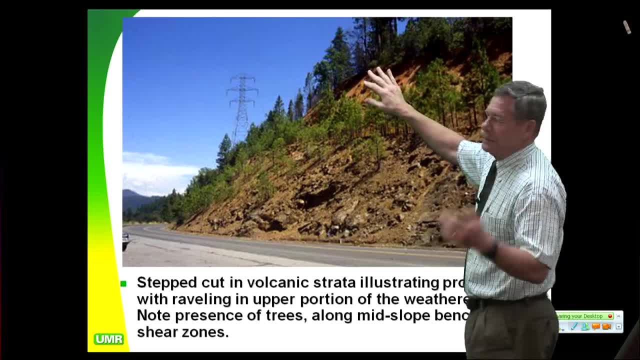 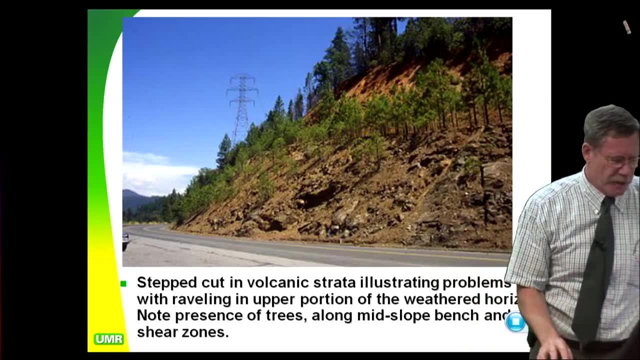 and it gets saturated. every once in a while for a couple days this just comes apart. It just starts flaking out, coming down on them. So it's a big problem. Notice here: they did a tree planting program to try and they thought that if we put some trees in here, 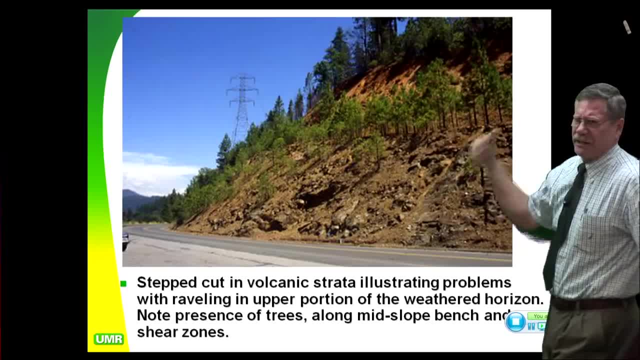 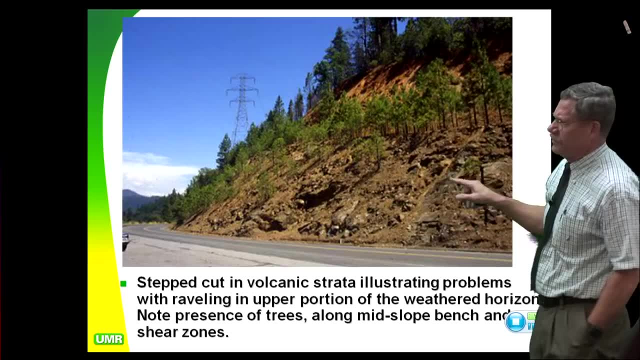 then when the rocks come down, that will absorb some of the energy of these rocks coming down. But the trees you know pretty hard to plant trees on a slope like this and have them survive. It's basically like you know. they get cooked like Thanksgiving turkeys. 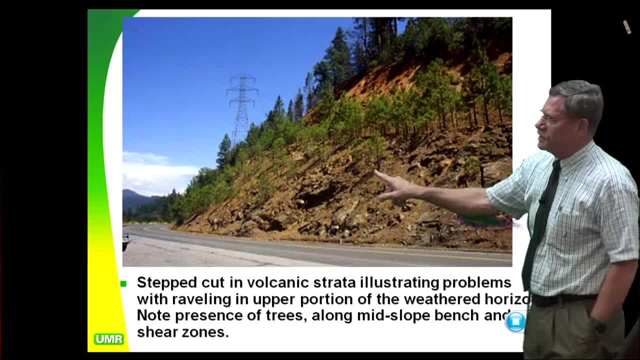 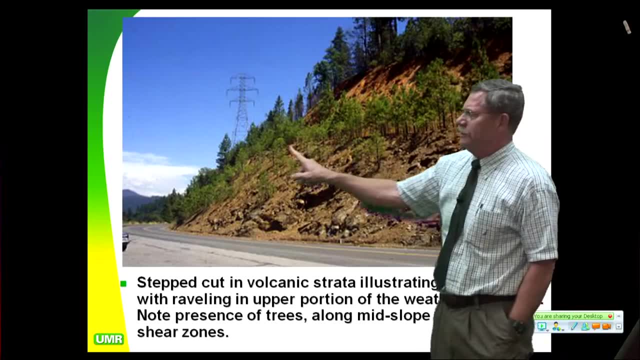 This thing's so hot You have to plant them on joints, The ones that are right on a joint. the ones that are right on a joint will get enough water to survive, but that's about it. Well, most of these trees are on the mid-slope drainage terrace. 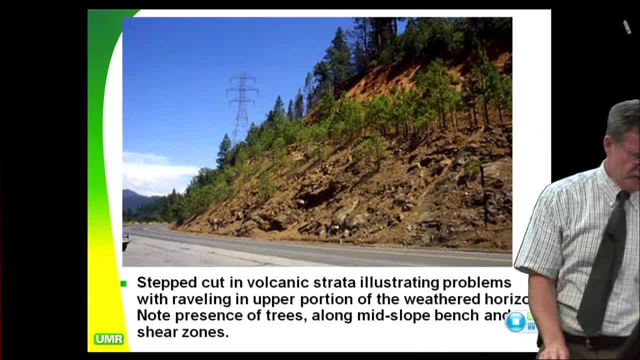 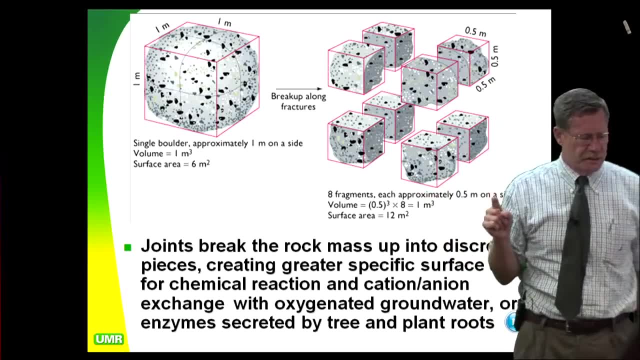 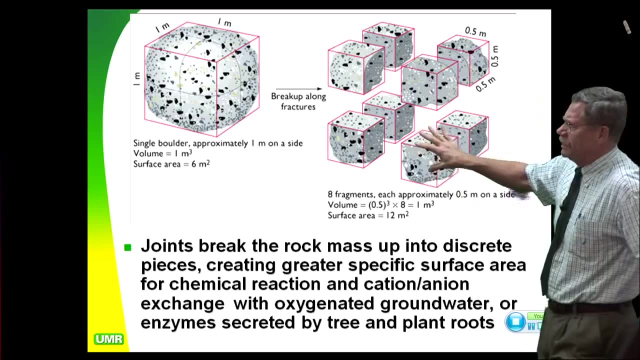 that actually survive. They had a very high die-off on this one. Okay, One of the most important slides I'm going to show you is right here. Joints break the rock mass into discrete pieces and they create a much higher specific surface area. 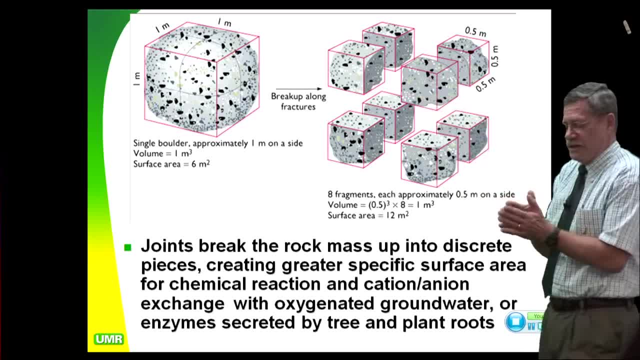 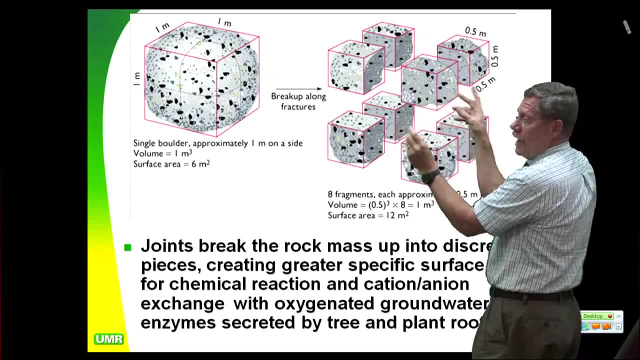 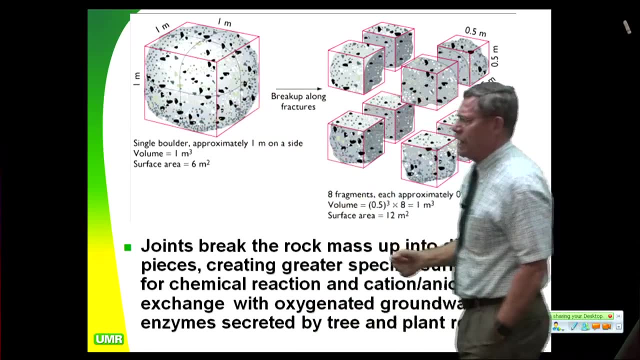 The more fractured my rock is, the closer the fracture spacing is. the thinner the beds, the more rapidly it's going to weather and ravel and have chemical ion exchange. Big blocks take a lot longer period of time to react because they have less specific surface area. 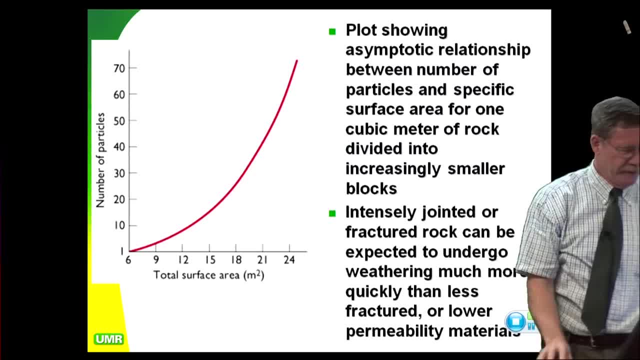 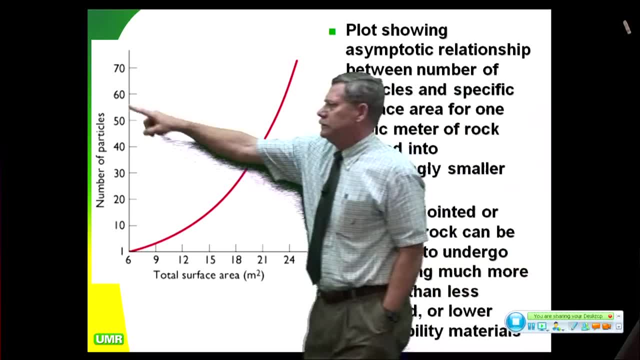 Okay, So you don't have to be a rocket scientist to understand that one. Here is a typical plot showing the asymptotic relationship between the number of particles- see over here on the y-axis and the total surface area, And you can see here. this thing's just taken off. Big surface area means much more chemical reaction for chemical weathering And it also means much smaller pieces for wedging, like ice wedging in mechanical weathering, So it gets you both ways. So units that are more thinly bedded, like shales. 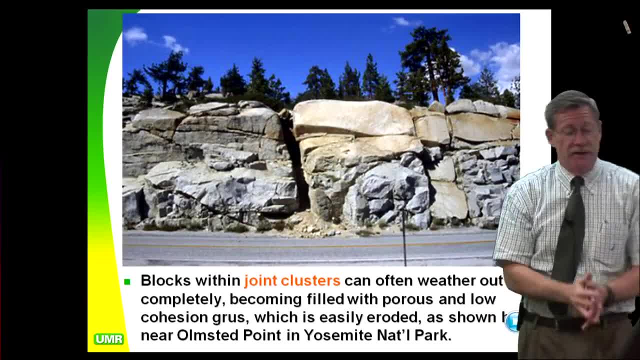 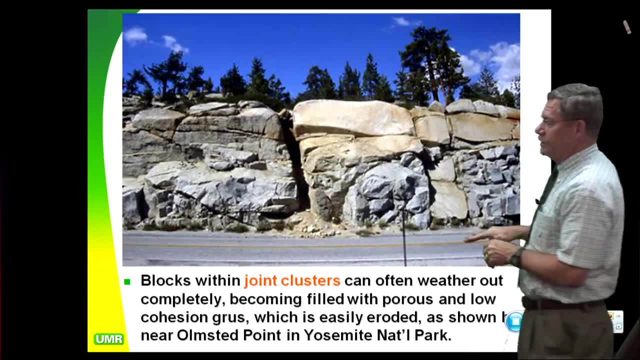 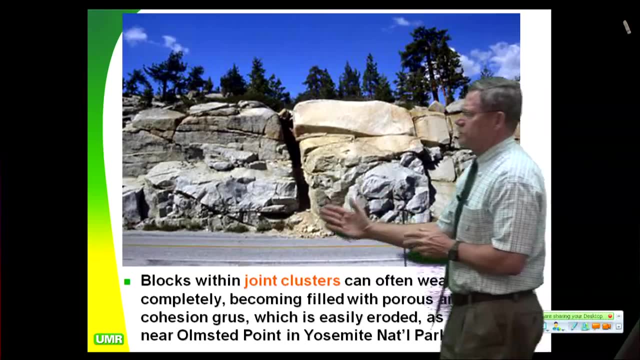 are always the problem. Now here's a case where we're near Olmsted Point, Yosemite. We got a WPA highway here- Actually it's a Civilian Conservation Corps highway- And we have some joint clusters. Here's a joint cluster. 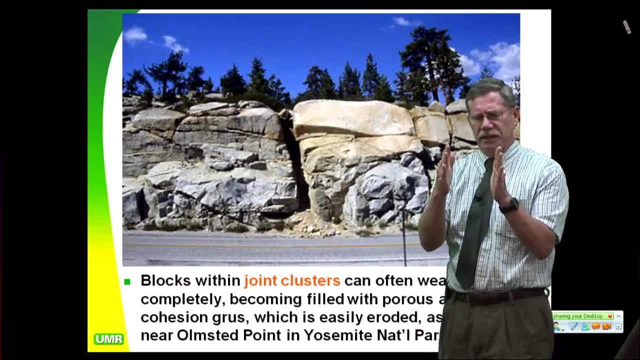 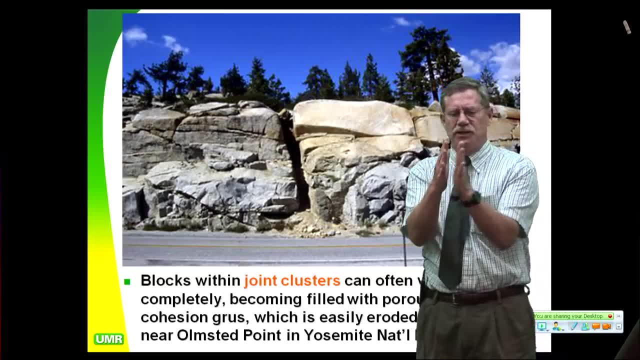 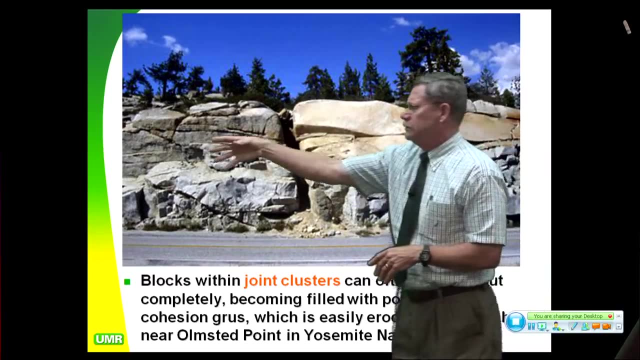 And a joint cluster is where you have a whole series of joints right next to each other, And so you have very high specific surface area in these blocks, maybe an inch thick between the joints, So you get a lot more moisture running through here as compared to here or here. 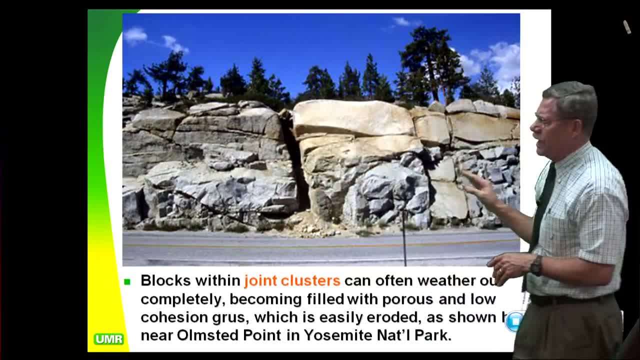 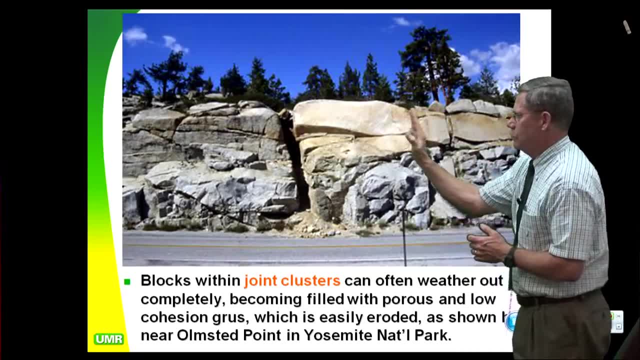 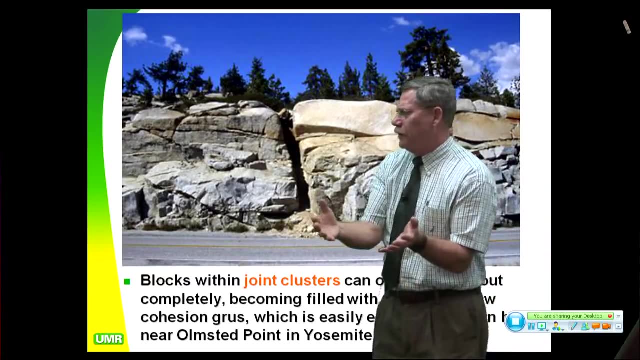 And so what happens here is after they cut this cut for the highway, which is about 22 feet high- and you got another joint suite here and right there- And after they cut the highway, they of course plow it for a while. 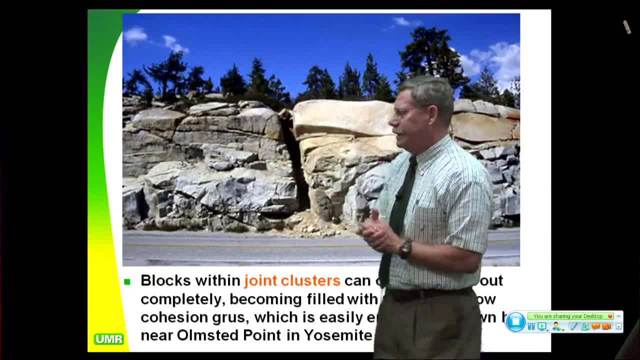 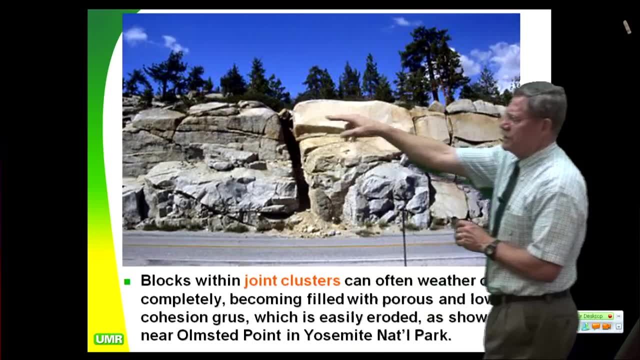 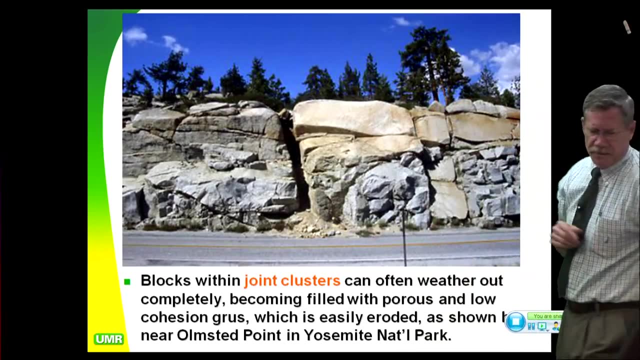 before they close it all down And then they throw the snow up, And that thrown snow up here creates insulation And what happens is they get pore pressure buildup in here and the thing blew out on them and actually caused some problems with the traffic. 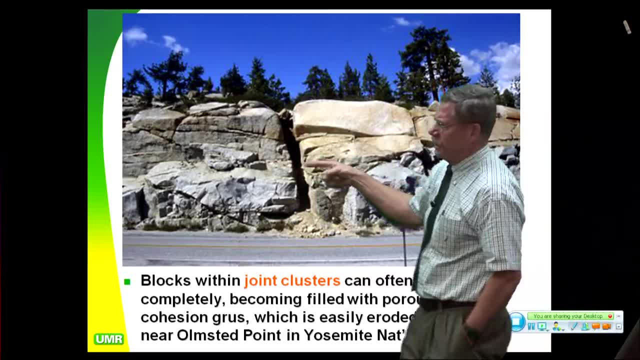 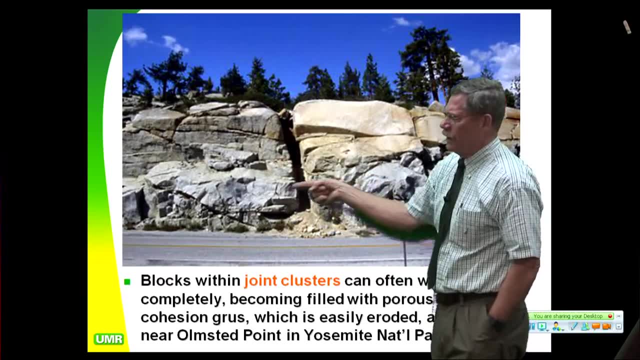 And we actually, when they were doing the Helms pumped hydro projects- Pacific Gas and Electric, 1977, 78 timeframe- they were doing a tunnel and went through one of these things and they drained an entire mountain And it was so catastrophic. 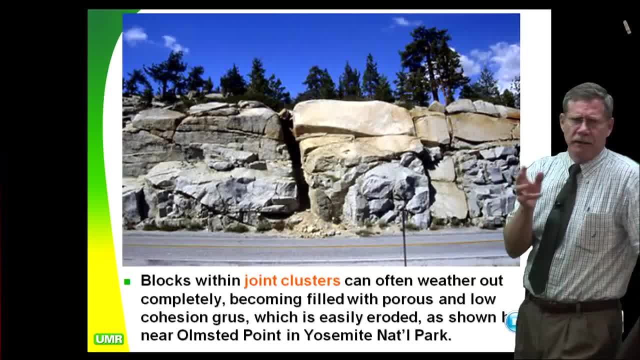 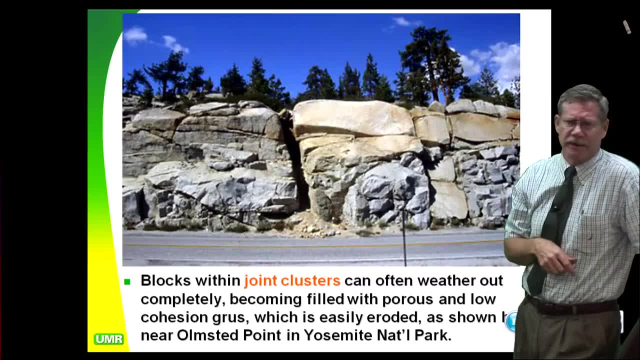 the amount of water that came in from the cluster that everybody in the tunnel tried to get out, and they killed a couple of guys through accidents, one of which was a classmate of mine from Berkeley with a master's degree, His first job out of college. 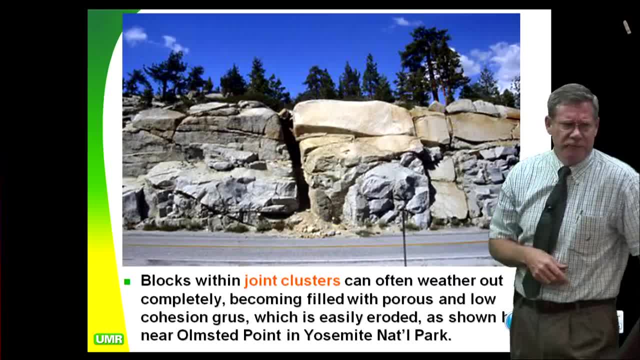 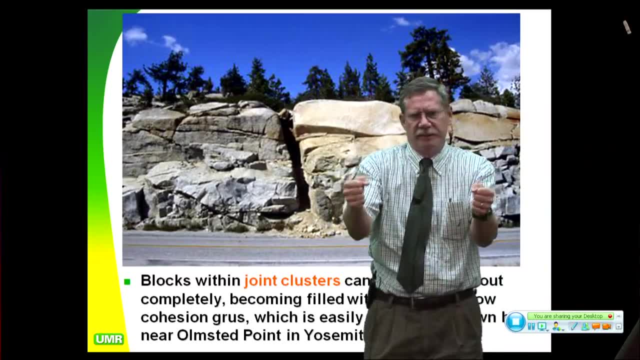 He was there one year, 11 months actually. He got smashed when one of the guys operating one of the miners, the underground mucking machine, did a wide turn like this and smashed him and then drove out to save himself. Didn't think about saving anybody else. 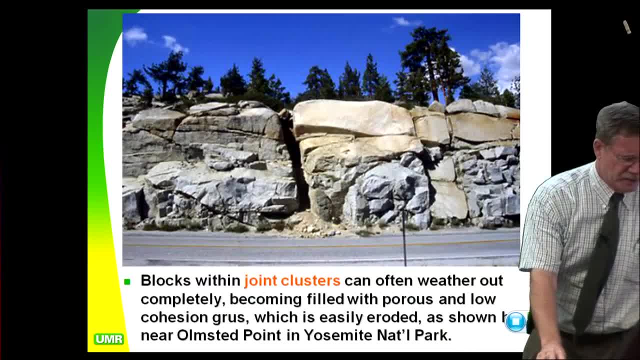 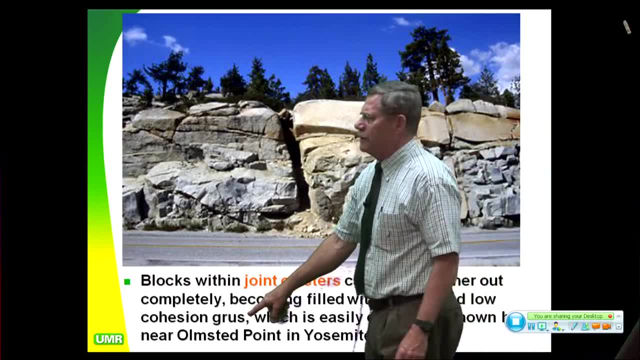 And he just killed my friend. So joint clusters are always going to be filled with porous, low cohesion grass, And that can be pronounced any different way like lus Lus, los lurs grass, grus guntk. 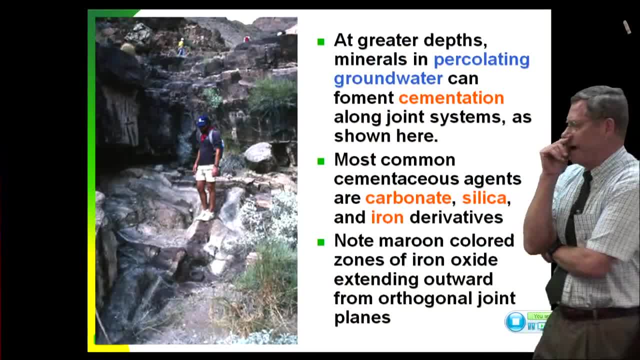 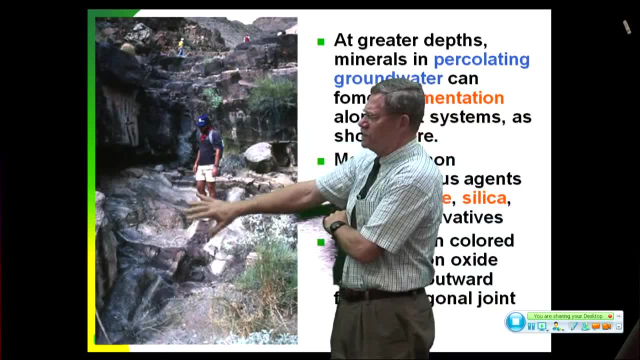 It has all kinds of different pronunciations. Here we are in Grand Canyon and we're actually walking around here- and this is a pre-Cambrian Zoroaster granite- and we're actually walking right on the joints, where the joints have been mineralized with iron. 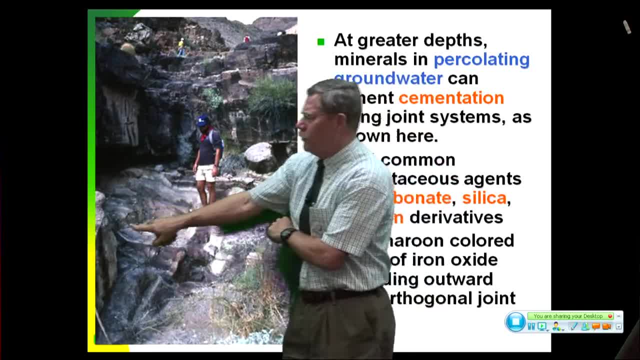 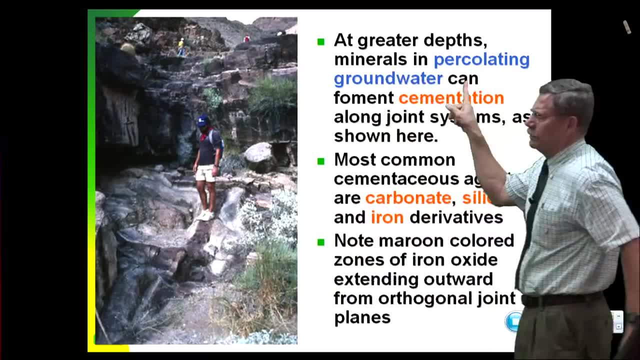 So this is more resistant and the core rock, the core stone, is actually the pools here. It's been eroded away, So percolating groundwater can also cause cementation along joint systems And this is a big issue in the basement rocks. 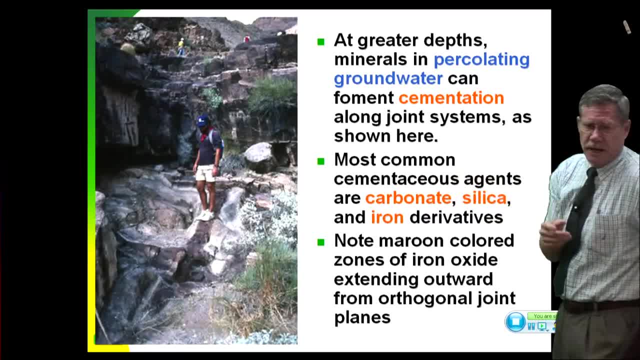 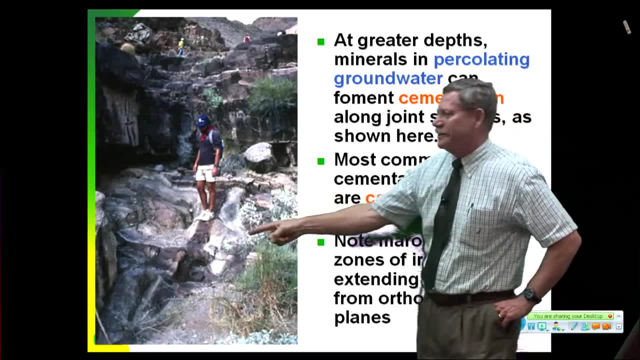 here in middle America, You get down in some of the basement rocks like we've had, we've encountered in the Washington metro and places like that, and woo, you come along and hit it. You come along and hit an iron stone in here and it stops you. 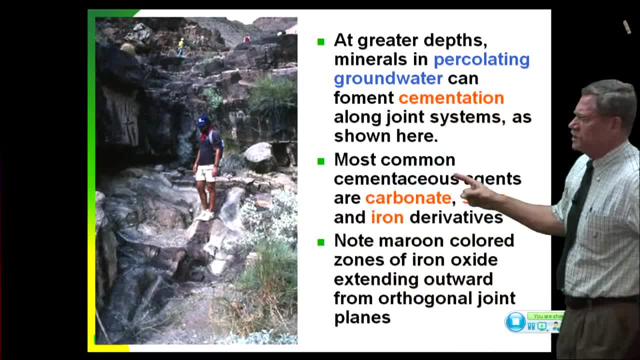 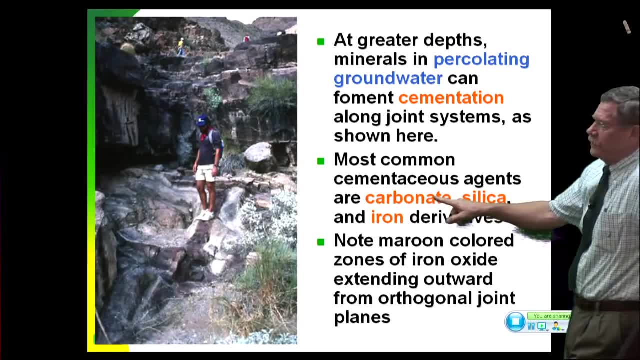 This is like hitting steel. It's really something. So most common cementation agents are carbonate, silica and iron. Carbonate's very, very soft Hardness of three: Silica is seven, Iron 7.5 typically. 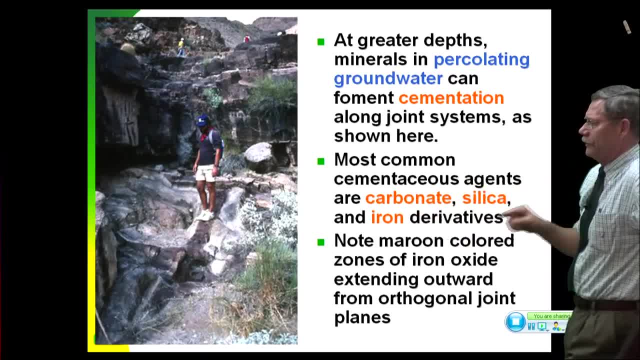 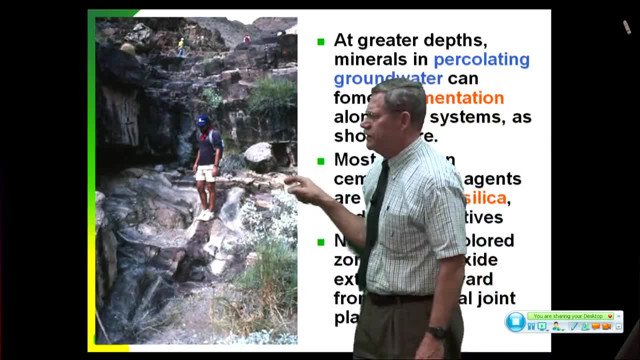 Iron's bad news, Really hard to cut through And note. the maroon color is the iron oxide And it's going both directions. So you see the maroon's actually going along here, going in that direction, as well as the joint. 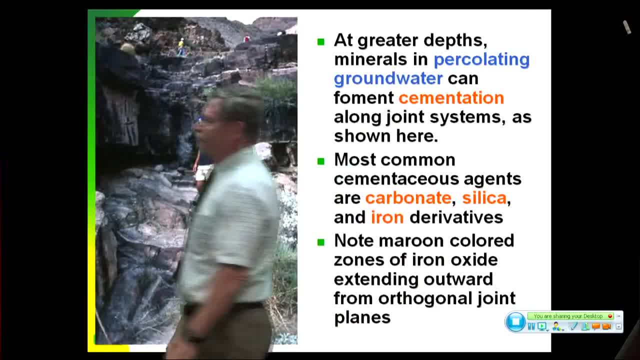 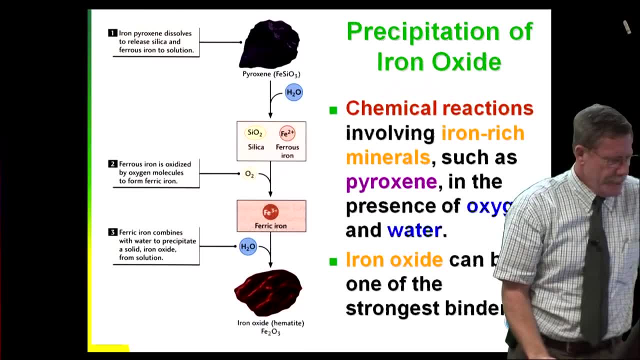 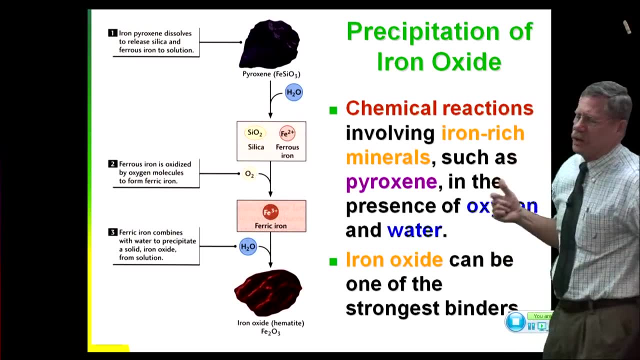 going in this direction here. So those are orthogonal, regional systematic joints. All right, The precipitation of iron oxide we should always be aware of, because this is much more common when you get to subtropical and tropical subhumid climates. Chemical reaction involves iron-rich minerals. 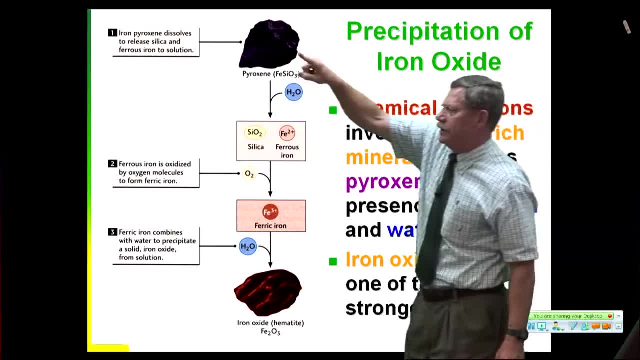 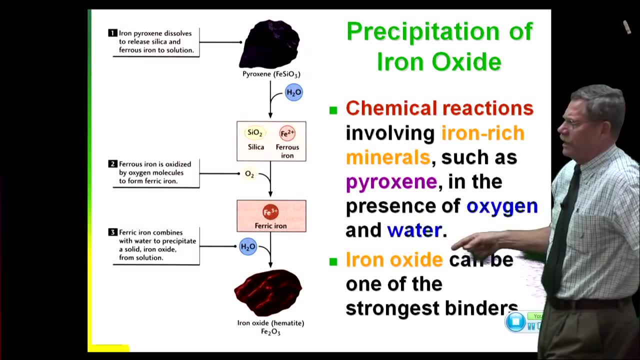 Usually the pyroxene coming out of the things like granites, granitic rocks, And you have pyroxene in the presence of oxygen and water. You're going to get iron oxide And that iron oxide is an extremely strong binder. It's hematite. 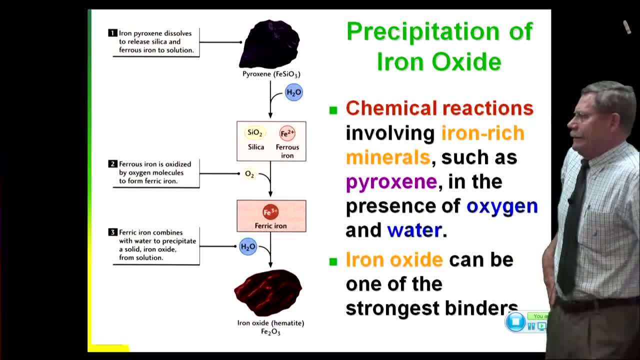 It's Fe2O3.. And hematite can really give you fits on construction. It can be used in construction projects for a lot of reasons, And also, if you get it in the concrete aggregate, you're going to get rusting problems too. 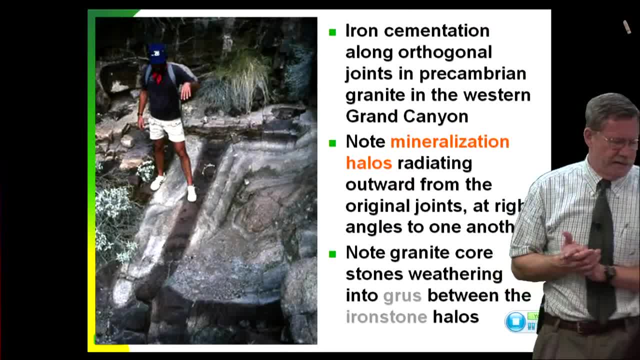 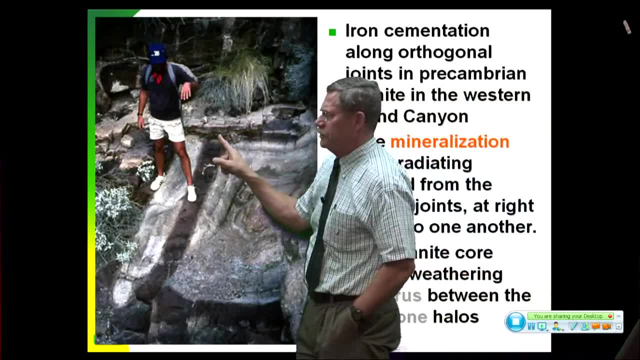 So it's bad news for that. Here's another picture of that case in Grand Canyon. This buddy of mine is standing on, it Marks it, And you can see these mineralization halos. What I'm showing here is we have an iron-rich halo in the middle. 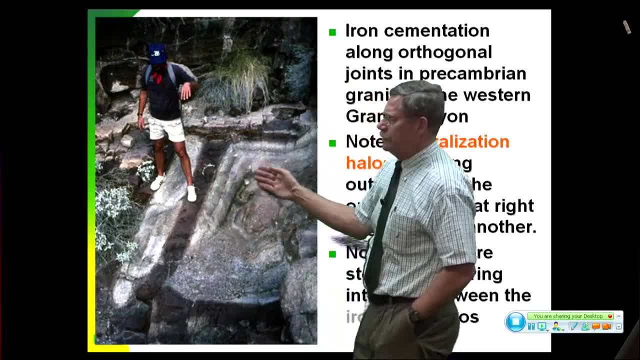 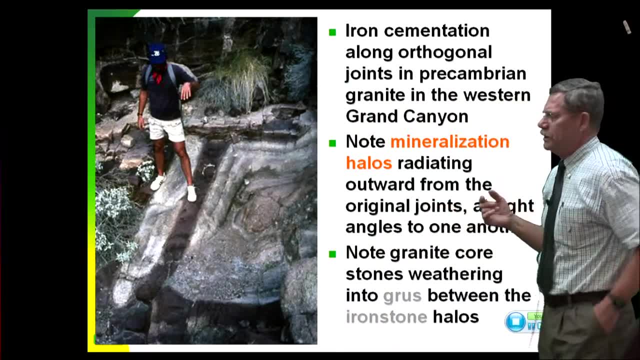 But as you come out, you have other materials that have cemented, that have percolated through these joints together And that's a function of the solubility coefficients of those different kinds of salts. So if you look around, Death Valley, California, 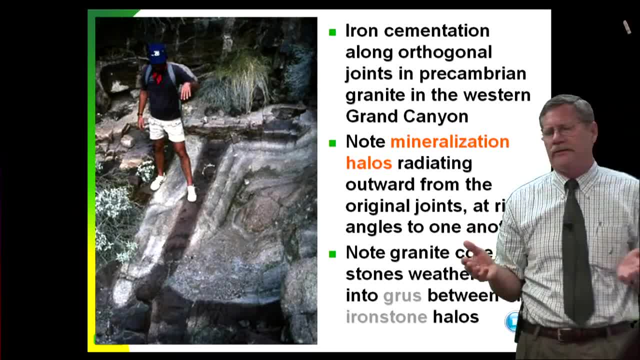 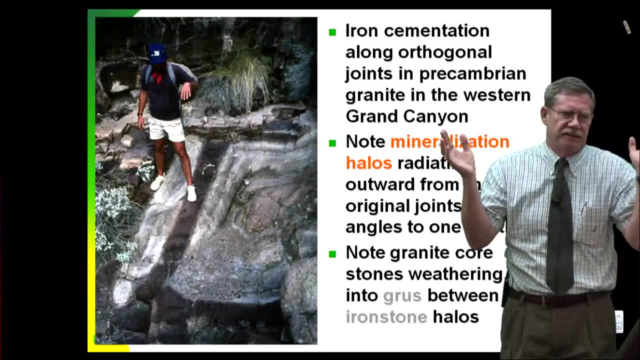 that's the low point. at Badwater It's 283 feet below sea level. Well, they had a lake in there. It was 700, almost 700 feet deep all through the Pleistocene. up till about 7,000 years ago it dried up. 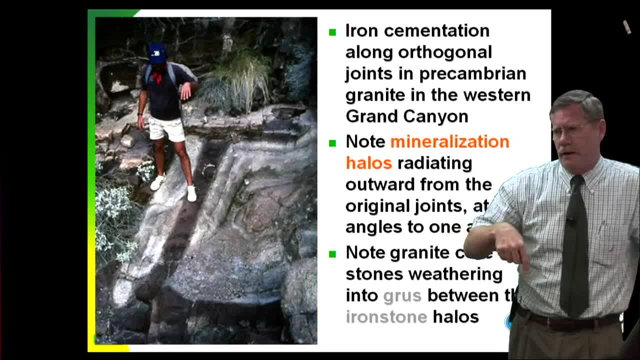 And I went out there When I worked for US Borax. we drilled a hole at Badwater and we hit 1,000 feet of lacustrine sediments, 2,000 feet of salt, 1,000 feet of lacustrine sediments. 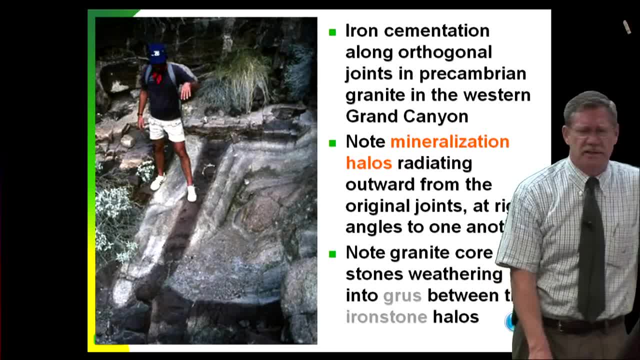 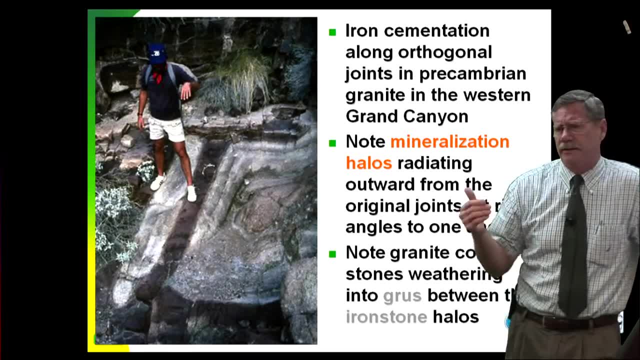 green clay, silt, and then 2,000 more feet of salt and we stopped. We're down two miles Just salt, salt, salt, salt salt. Same kind of geologic structure as the Dead Sea between Jordan and Israel. 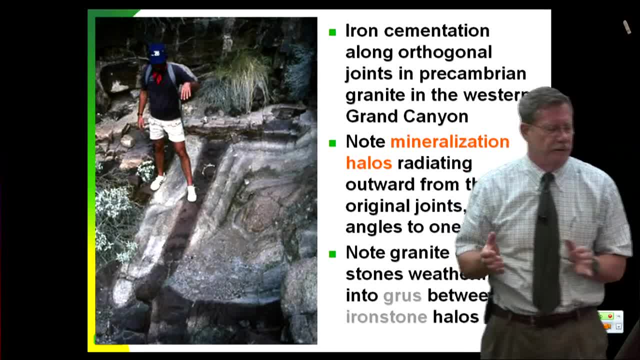 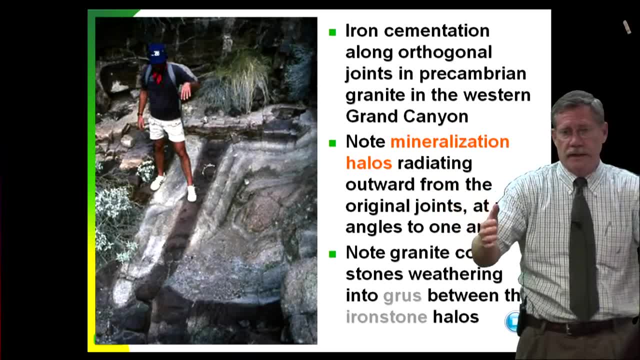 which is much deeper: It's 1,800 feet below sea level. So what's going on there is you have halos of salts As that lake shrunk. in the case of the Dead Sea, it was called Lake Lisan. 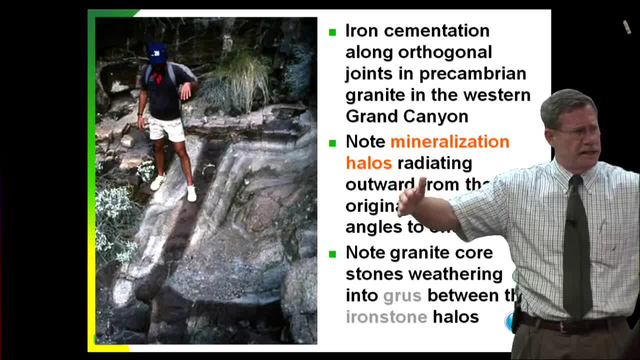 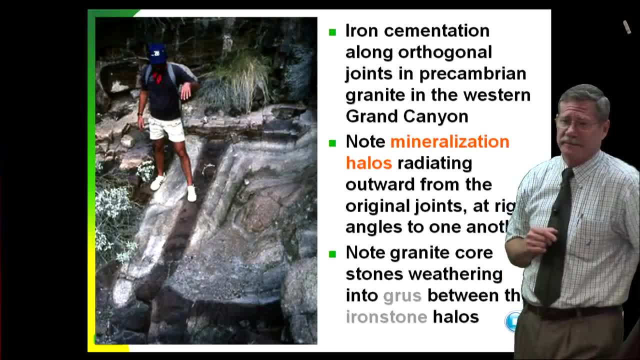 Glacial Lake, Lisan, As it shrinks. you get the carbonates first, and then you get the halites, and the last thing to come out is the potash, the potassium salts. And so they mine those salts in the Dead Sea big time. 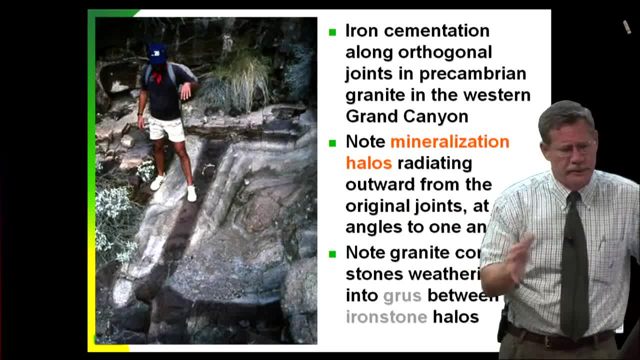 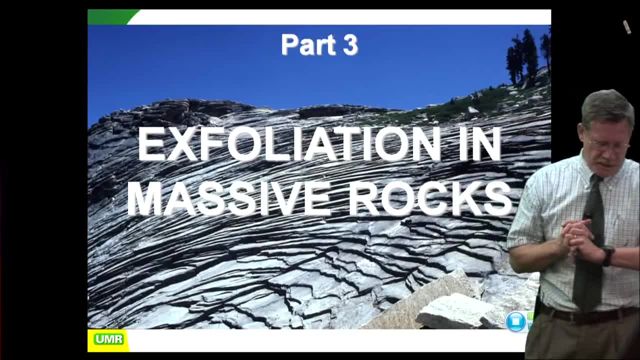 The whole southern base of the Dead Sea has all been diked off years ago. They extract potash out of it- Exfoliation in massive rocks. Do you want to take a short break now, or just have me stop at 6.20 instead of 6.30?? 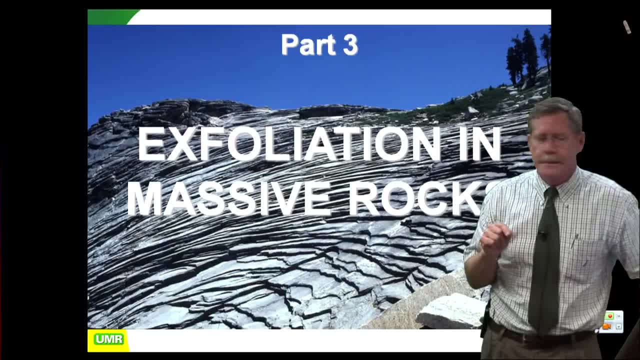 6.30.. What, So we can stop later? I'm talking now. I wonder what else they. You want to stop earlier By going on right now. Does anybody want to have a bathroom break? Okay, What I'm going to do then. 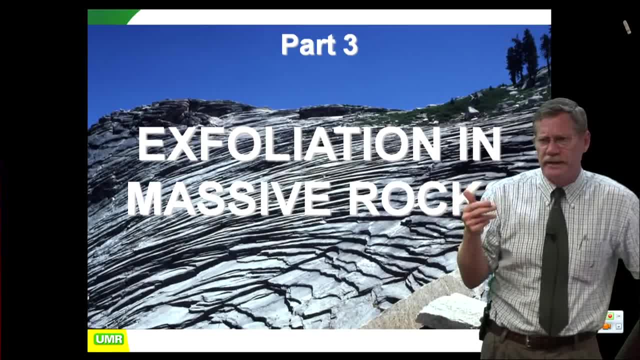 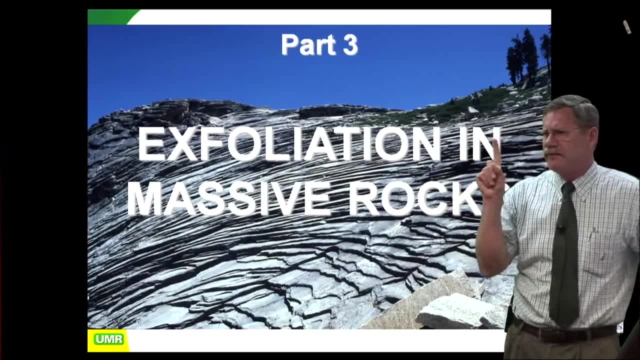 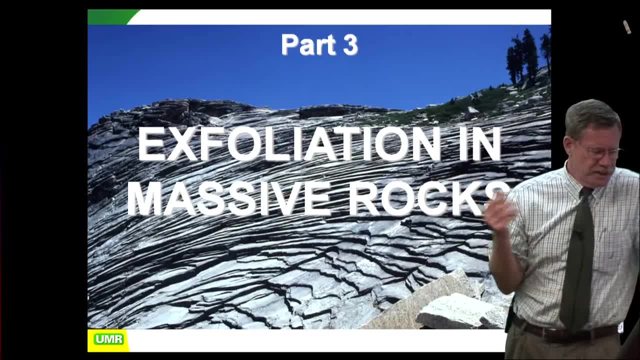 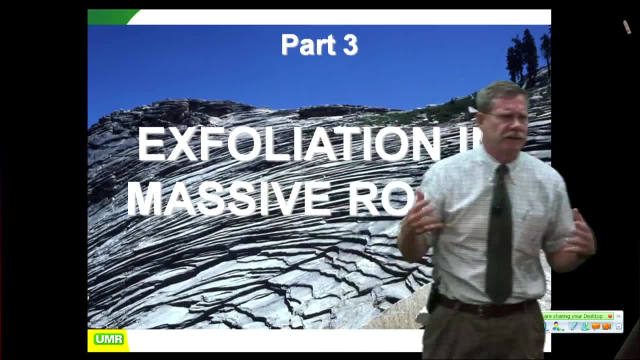 Okay, Okay, Okay, Okay. I'm just going to take this Actually three more minutes because it's dinner time. Exfoliation in massive rocks. Here's how I got interested in geology. I was always interested in civil engineering because I grew up. 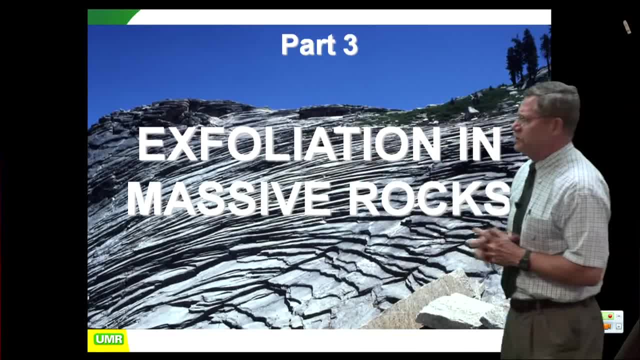 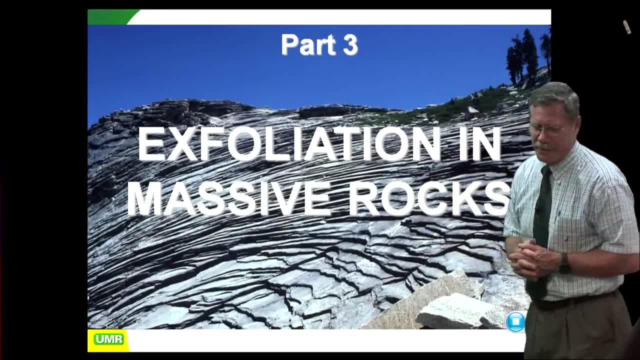 in a general engineering construction, family, earth moving, And so what I was really interested in was rock climbing in the Sierras. I went to Royal Robins Rock Climbing School here at Yosemite National Park when I was 17 years old. 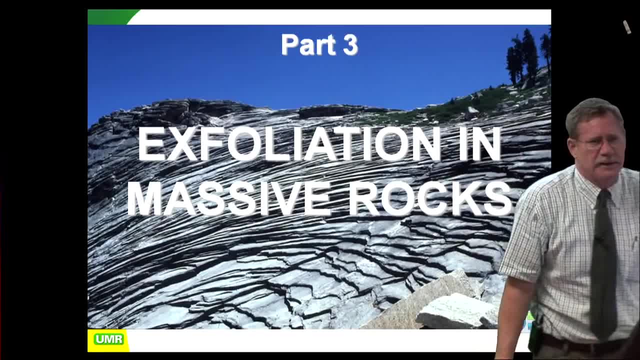 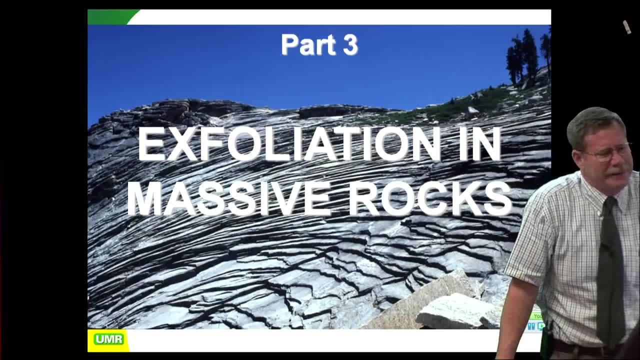 I spent my entire life savings. My father was furious, So was my mother. My dad wasn't art prof. You know he loved, you know of art and fine things in life. My mother was a librarian. He goes, I pissed away all. 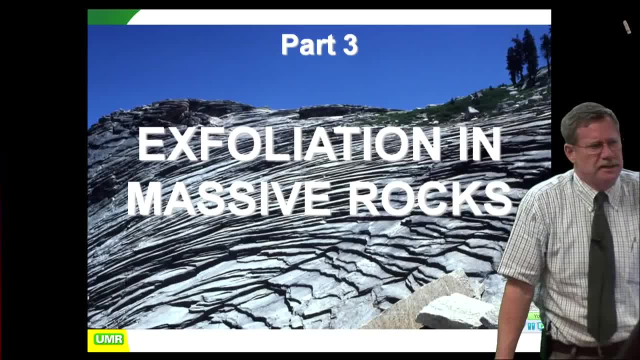 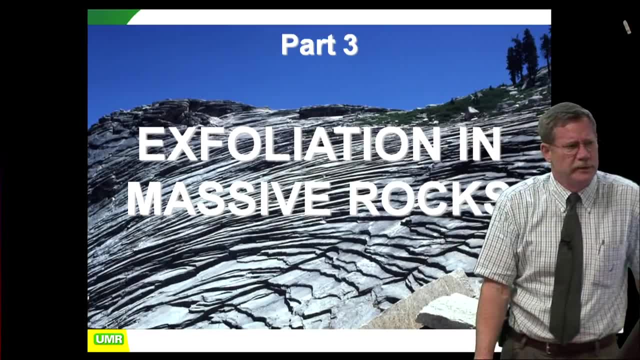 of my college savings. Well, I figured I want to fly jets in the military. I'll just have the military pay for my college. That's what I did. I went off to school. I never took a loan in 10 years of college. I always worked. I was always hustling, In fact, when 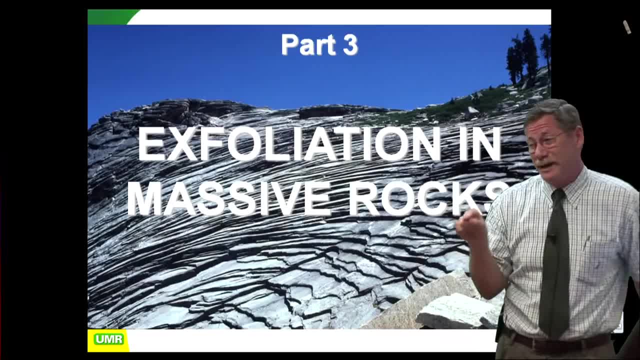 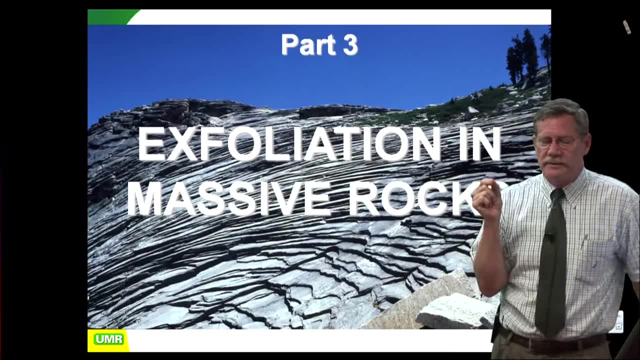 I was at Berkeley. I had a great business. I actually made more money with this than I did as an engineer for three years with a PhD and PE. My credit is to my dad. My dad said: you want to make money, you've got to do something people need, but you don't have. 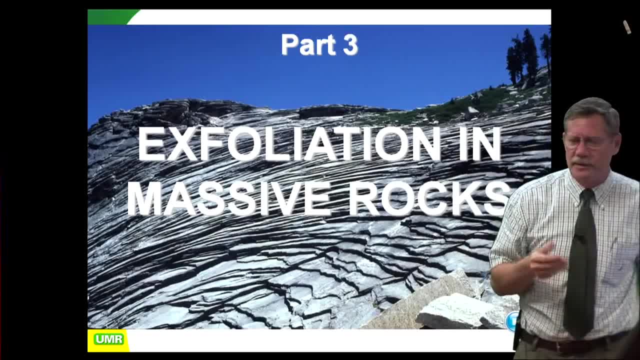 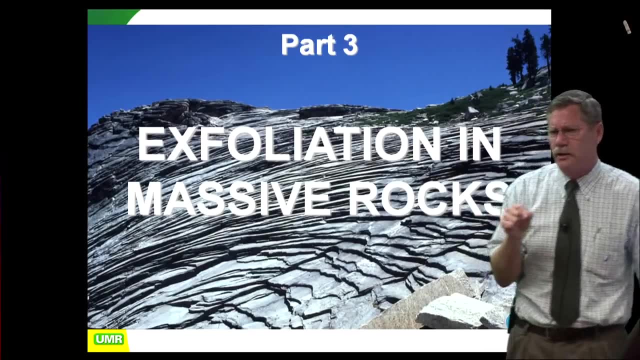 a bunch of competition in it. What do they need? in the Berkeley Hills They had poison oak all over the place. Nobody wants to pick weeds or kill poison oak. Americans don't want to do anything dirty, hot, sweaty. I took those on. I had a poison oak removal. 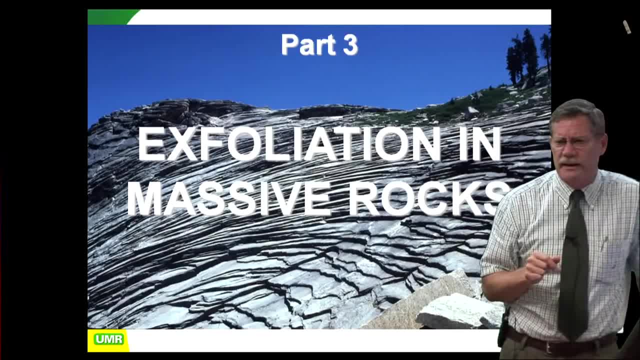 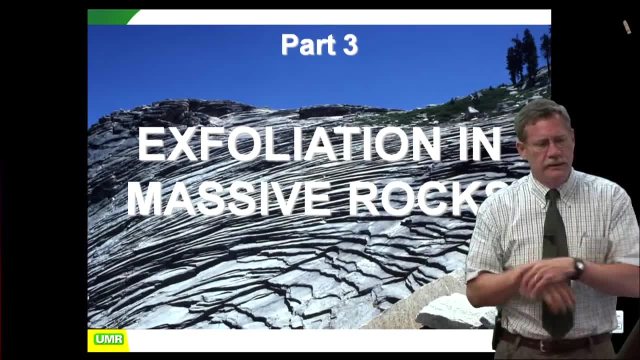 service. I was the only guy in the phone book that had it. I made $60,000 a year while I was in grad school. It was a pretty good deal going out there. You just tech new up, get out there real early, be done by 11, come back the next day. tech new down again. It's. 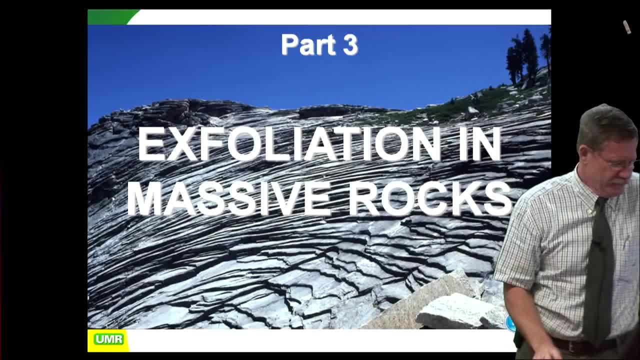 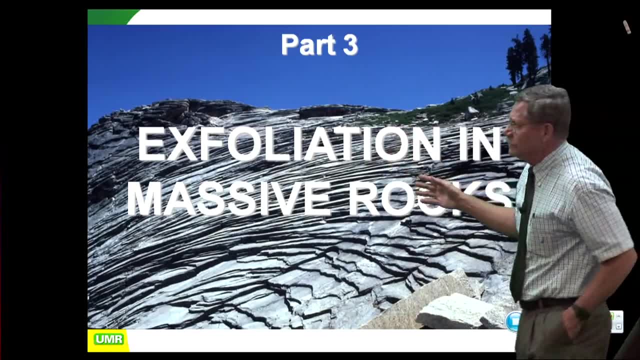 not that hard to do. I wonder if anybody's ever relit that up again. Anyway, it was good money. I wasted my money to go to rock climbing school, but this is the kind of stuff that I saw. This is Little Shut Eye Pass in the Sierra Nevada. This is the strongest rock. 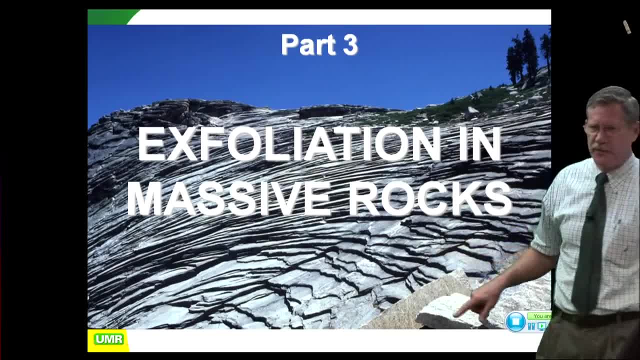 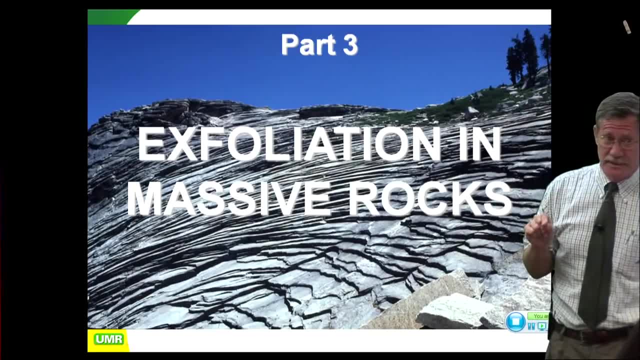 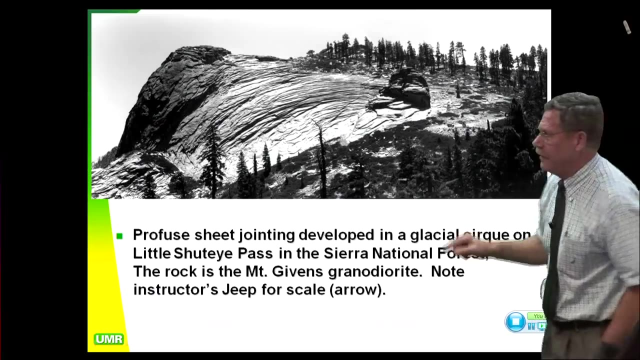 in the Sierra Nevada. We tested it at Berkeley. It was like 34,000 to 37,000 PSI, compressive strength, 10 times stiffer than structural concrete. Notice what strong rocks do. Strong rocks are Brittle, Brittle. Thank you, Brittle. So here we are backing away. And, by the way, if you've got, 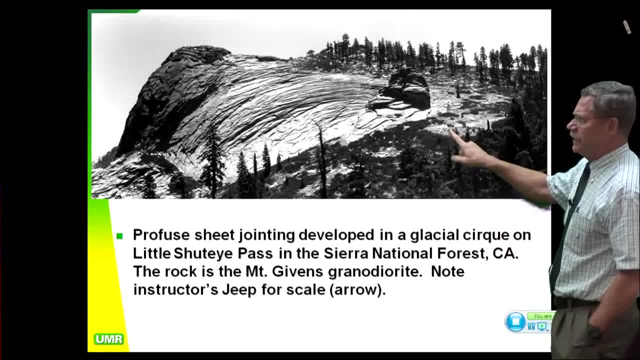 really good eyes. that's my Jeep right there, my Jeep CJ5.. Not the same one I drive now. I drive a 43.. That's a 65. That was my first one Bought when I was 18.. But here we are, The Jeep's parked there for scale. 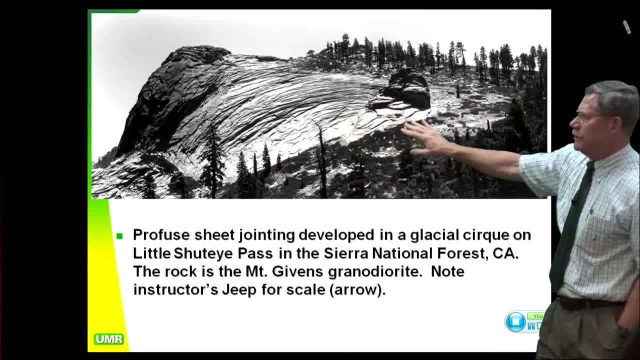 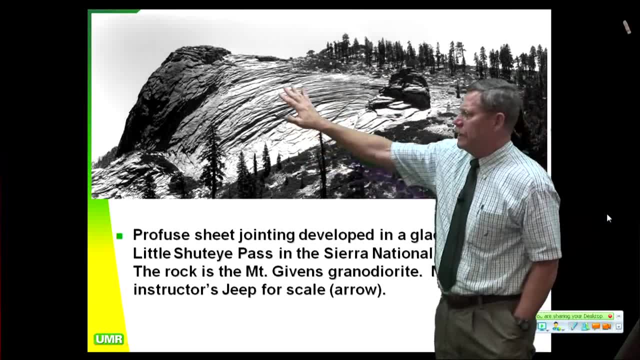 And then you're looking at this glacial cirque here in the Mount Givens, Granite, Diorite. This is a big glacial cirque feature, about 500 feet high, And this thing is just permeated by countless sheet joints. 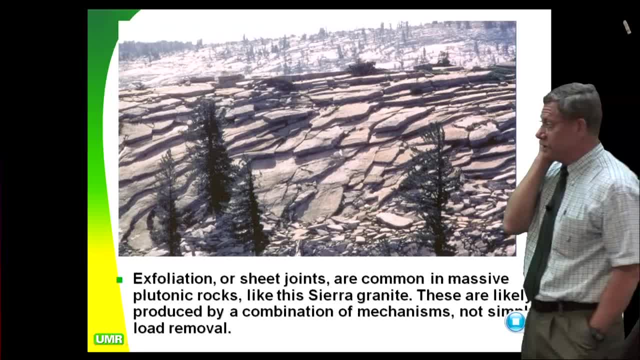 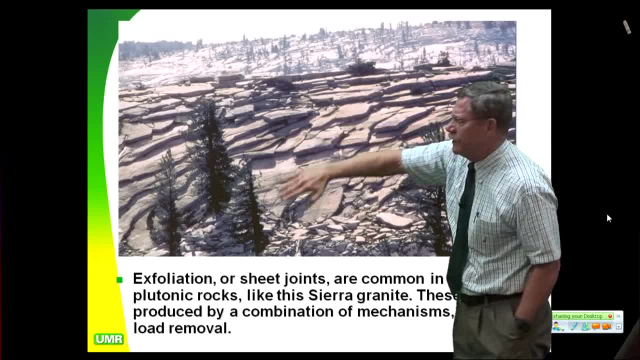 And when you get up close to sheet joints, this is what they look like. This is up in the, actually in the Tenaya drainage in Yosemite. This is big, huge sheets and then they are semi-parallel to the ground surface. 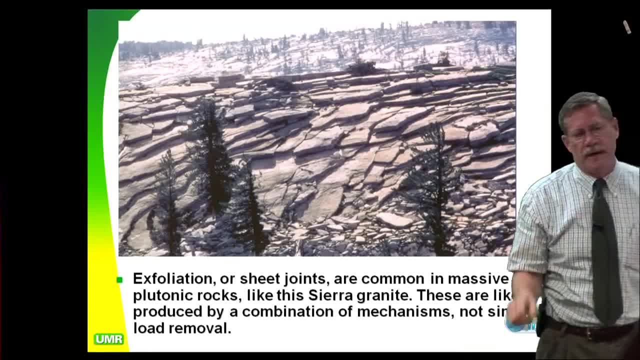 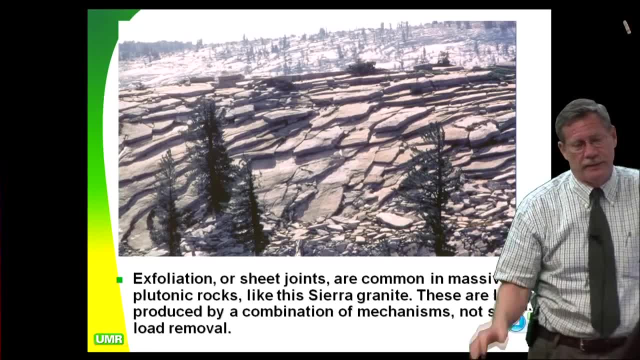 Now these are what drive us nuts with dams. These are tied to probably 50% of the dam failures I've worked on all over the world are sheet joints. They didn't take them seriously. I had one in Brazil just a couple years ago. 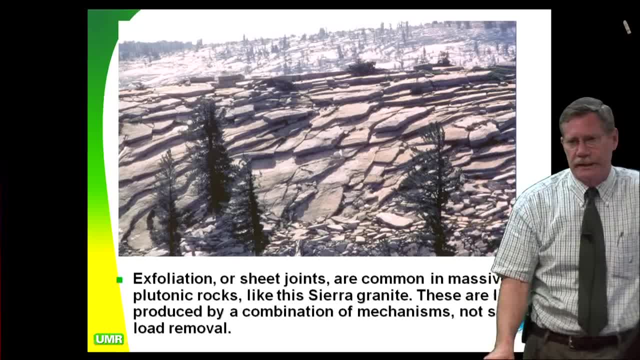 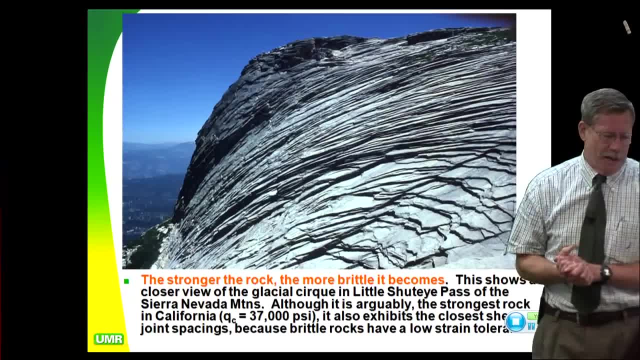 Brand new roller-compacted concrete dam failed on its first filling because they didn't grout the right abutment, the sheet joints. Here's what they look like up close. So you see, here this is a closer view of the glacial cirque in the Little Shuteye Pass. 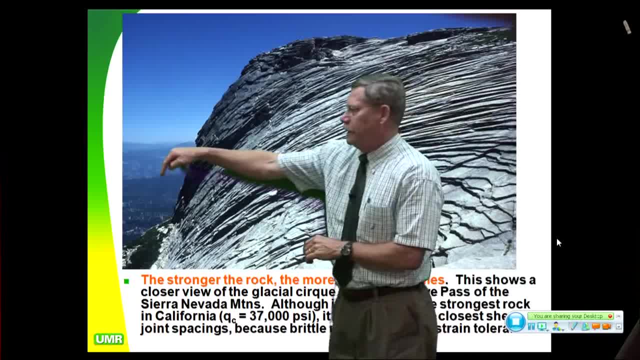 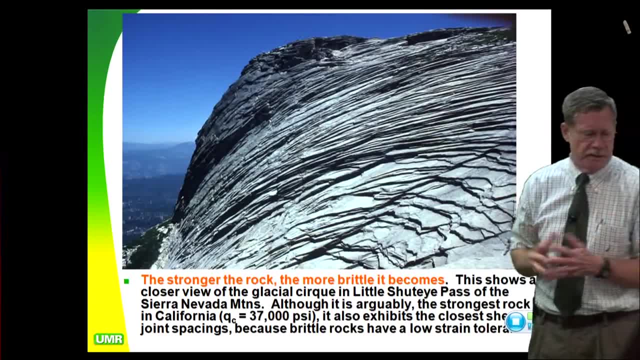 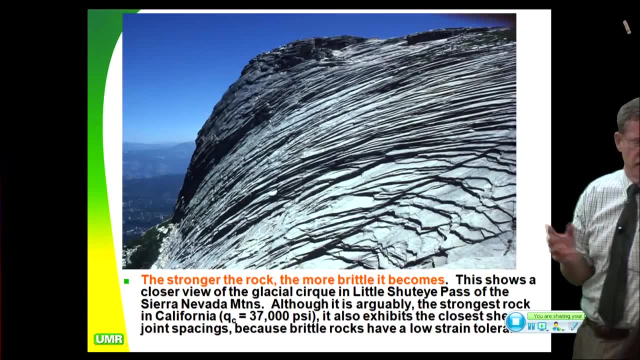 And there's a dam, big dam, right down here in the upper San Joaquin River called Mammoth Pool, where they battled enormous problems with sheet joints And that was one of Terzaghi's last consultations they did. He wrote a very famous paper on it called Dam Foundation on Sheeted Granite. 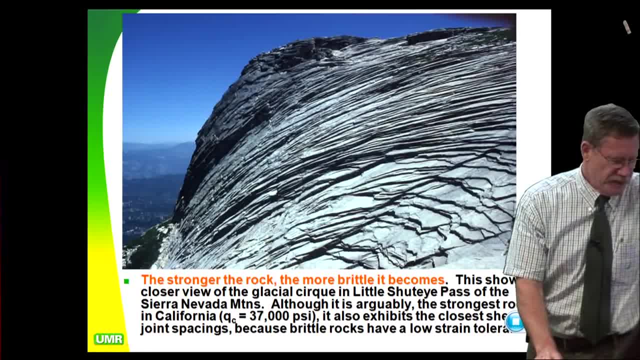 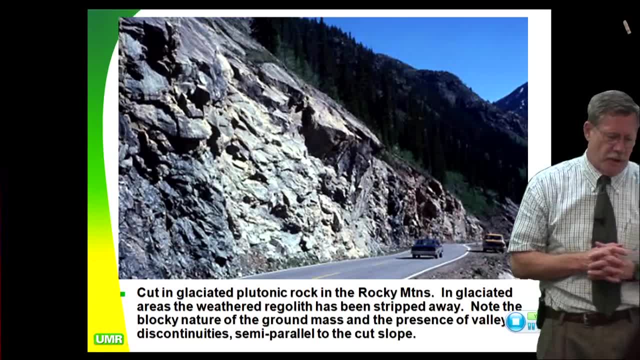 which appeared in Geotext, And this is a great example of a technique in 1962.. But these materials have a low strain tolerance. They're very strong but low strain tolerance. So here we're going to move. we move to the Rocky Mountains. Independence Pass in the Rocky Mountains. 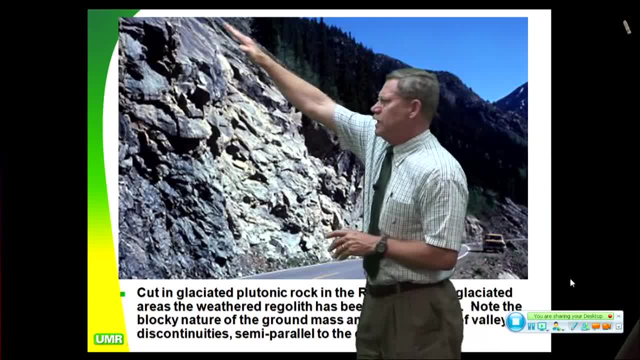 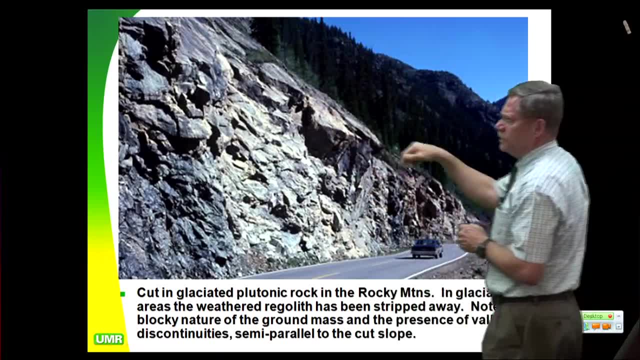 This is a glaciated area. See a very planar surface here. It's been glaciated. All the soils are gone. see no soils. We've been glaciated. All the soils have been moved away by the glacier. So man comes in here, does line drilling. 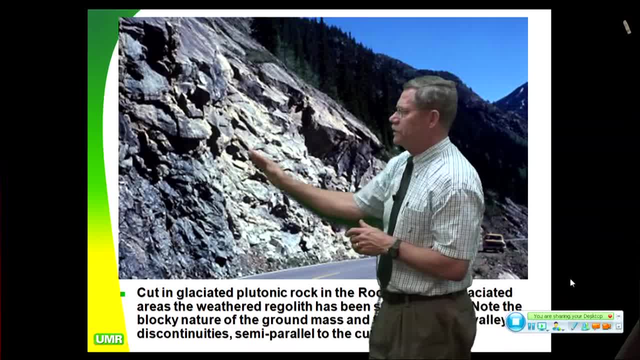 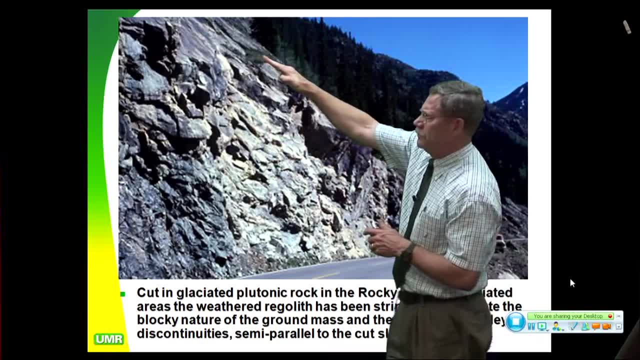 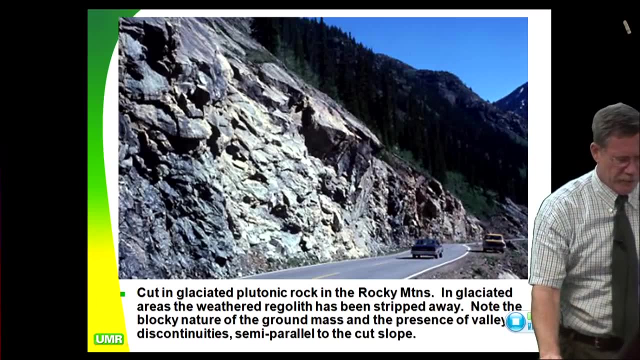 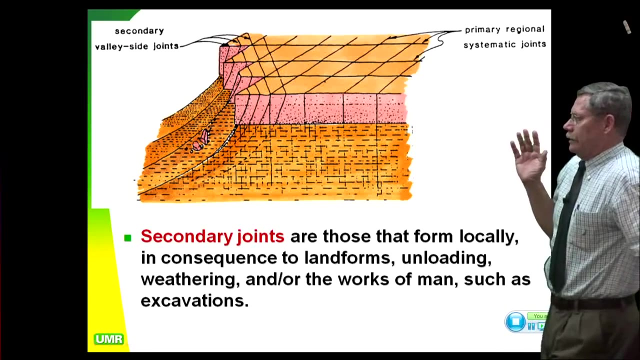 what happens here? well, you get wedge failures. these wedge failures are along valley side joints that form semi parallel to the ground surface. so this is a real big problem in massive rocks anywhere you go around the world. here's a drawing I did. it's from my PhD thesis- where we're actually looking at Zion. 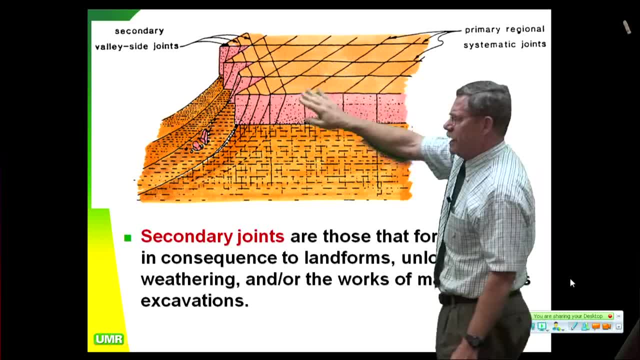 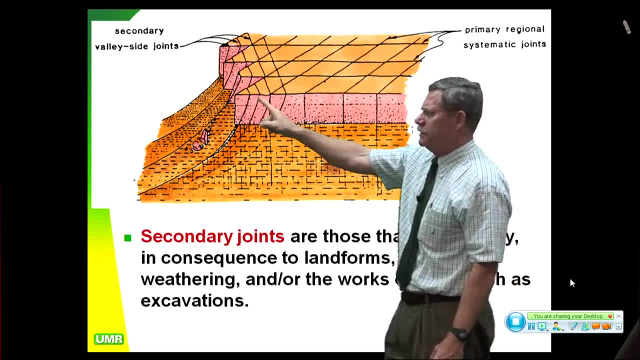 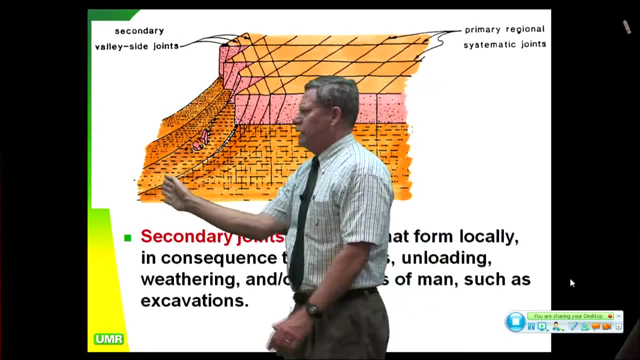 National Park and we're looking at here is the regional systematic joints cutting through the Navajo sandstone, on top the Moen of shale and sandstone, and you get these diagonal valley side joints that are parallel to the trend of this canyon right here. so we got this Canyon running up like this, these things. 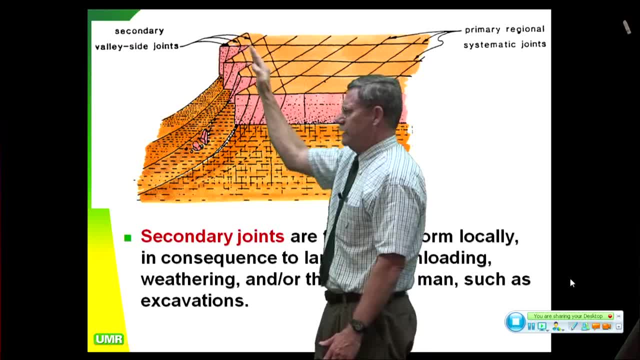 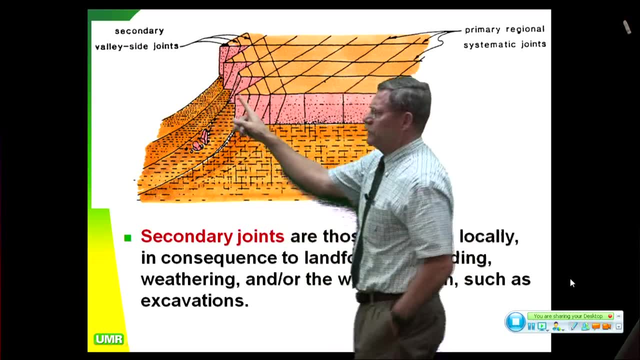 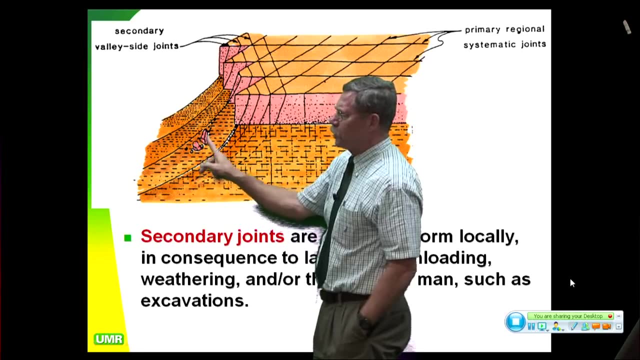 all right, gotta do this right. these things are parallel to that. so when you're walking along out here as a geologist, you don't see these things. they're back behind the face. what you have to look for are big hunks like this. a drop rock and you go. what's this big, huge pump of rocks doing here? 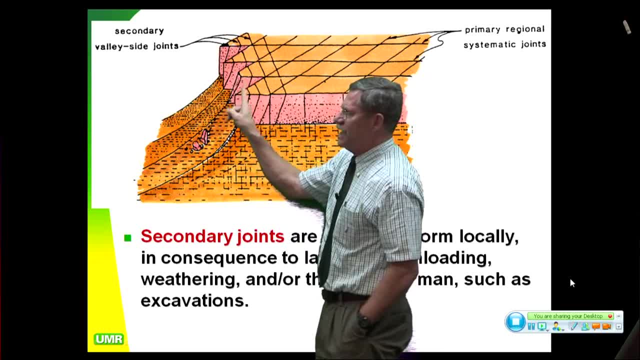 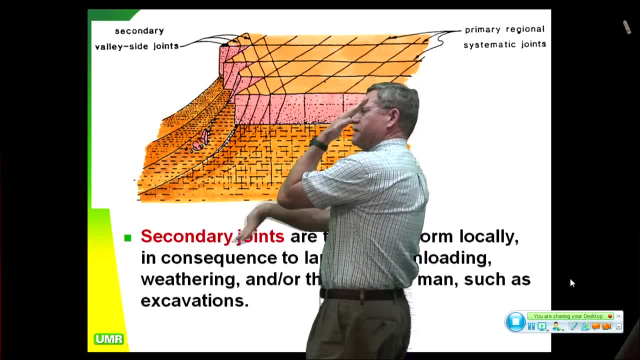 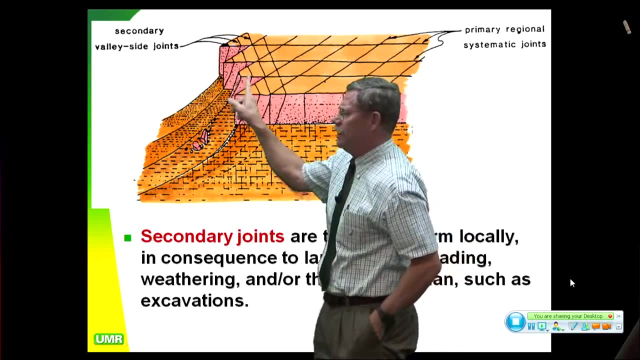 well, you look up, there's the face it came off of, and that face is inclined like 60 degrees. it's just perfect for a rock slide: 60 degrees, 45 minus P over 2. that's why. so there is your clue. now, how do you go track these things? you go in these little re-entries. 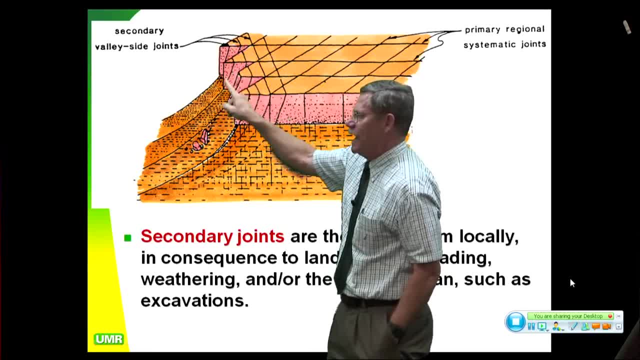 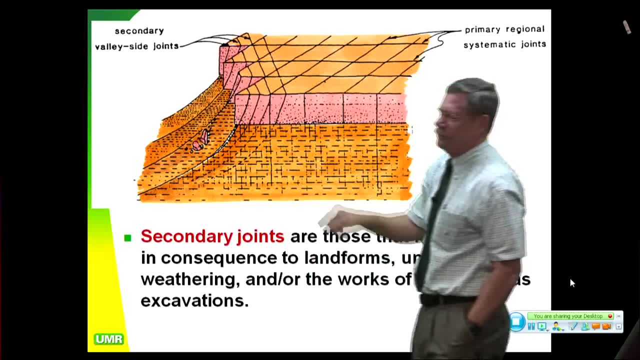 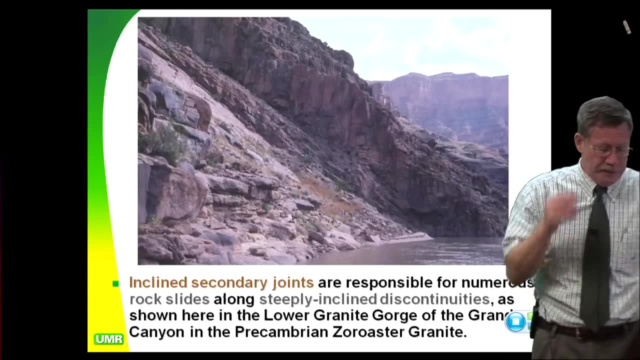 you go in these little side canyons and you get in the side canyon aha, there you see them, see that and you start seeing these features. now these are really problematic to deal with for highways and pipelines and dams. here's one in the Grand Canyon, upper part of Lake Mead. I've been a consultant on a Hoover Dam. 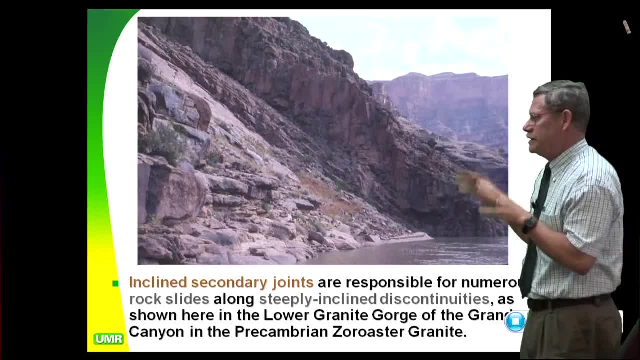 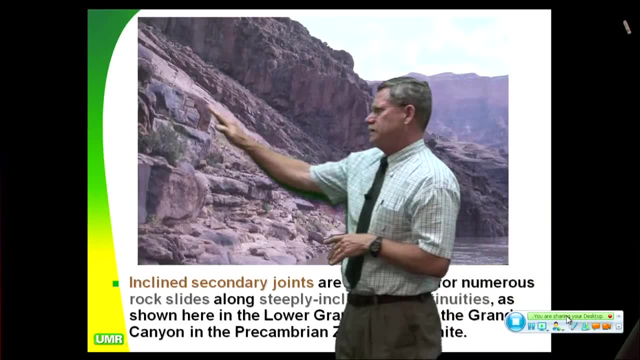 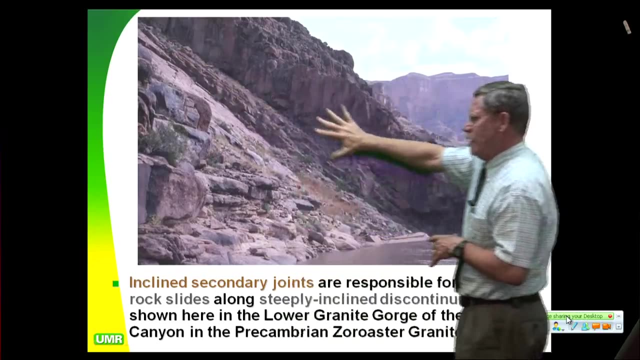 for over 30 years now, because I did part of my PhD thesis out there. and this is a Zoroaster granite, these are valley side joints, just a whole bunch of them. boom, boom, boom, boom, boom, boom, boom and the whole mountain here slid down, big block slide, coming down on about a 40 degree. 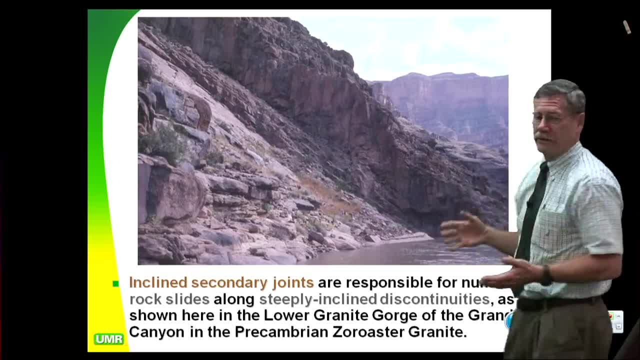 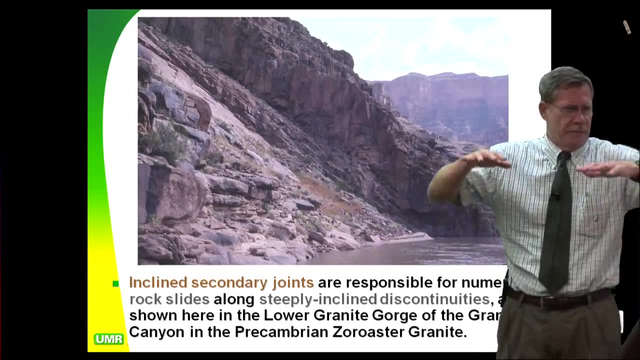 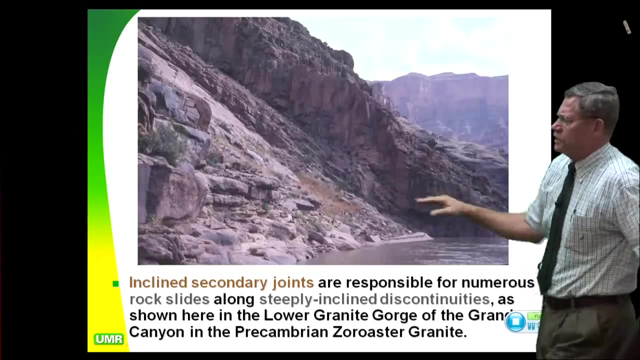 slope and went into the river and blocked the river, had a big landslide dam and that doesn't last very long geologically. the river builds up the behind it, a bunch of silt builds up behind it and the river just blows the thing out of there. so the dams, debris is all gone, but the scar where this thing. 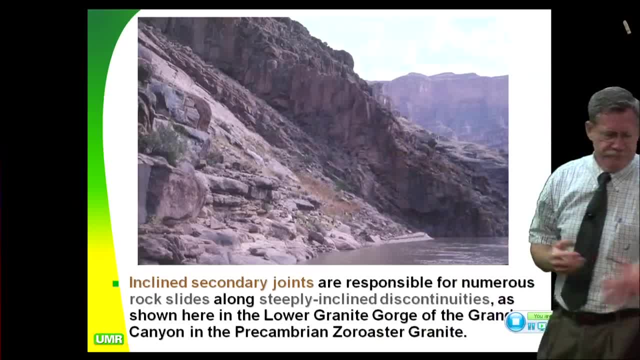 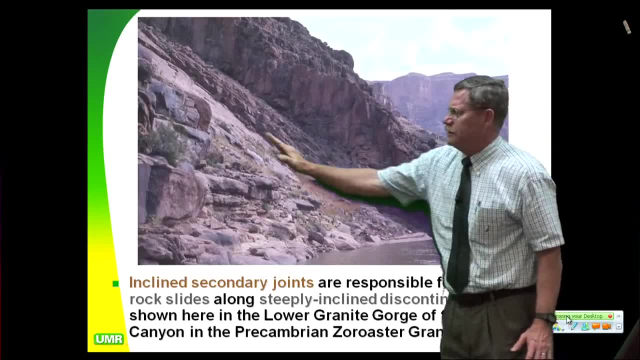 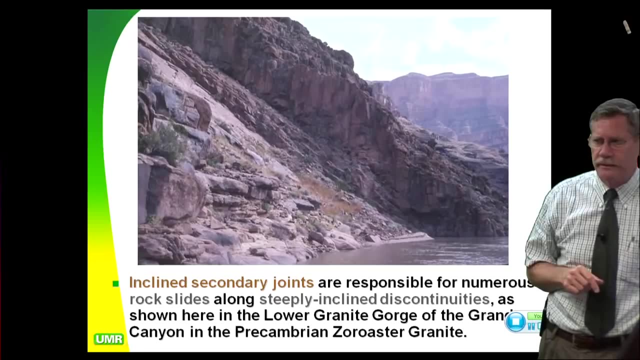 came out from and recently, you know very geologically very recent- is there to see. so in this kind of a case you can actually go up here and see the valley side joints very, very well exposed. but every dam site I've ever worked on in the world has had valley side joints, every single one. 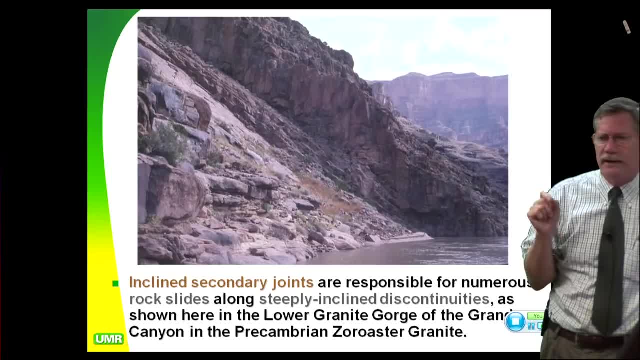 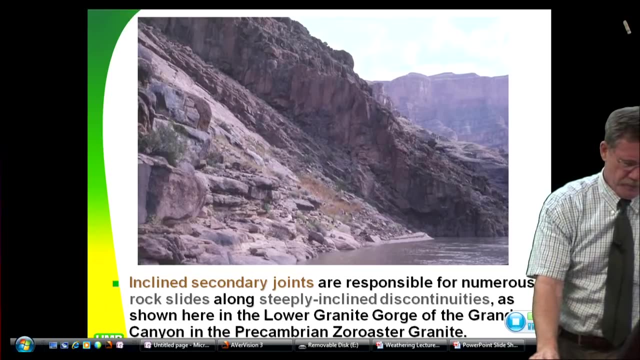 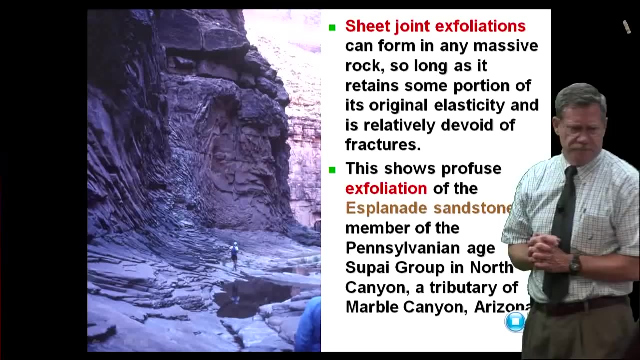 one of the first sites I worked on was Reza Shah Kabir on the Karun River in the Zagros Mountains in Iran, and they had just all sorts of problems with the foundation on that. when they got in there and started digging things out, it looked like Tom Sock over here. oops, we're done. okay, no sheet joints sheet. 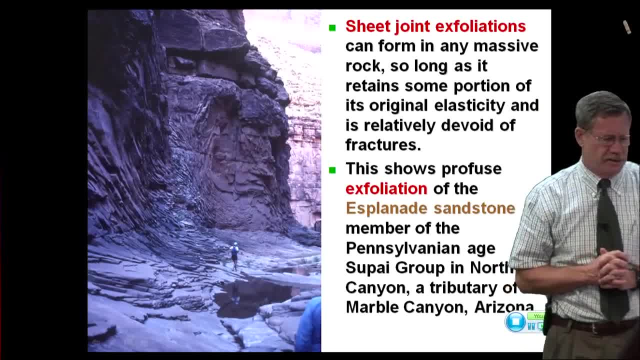 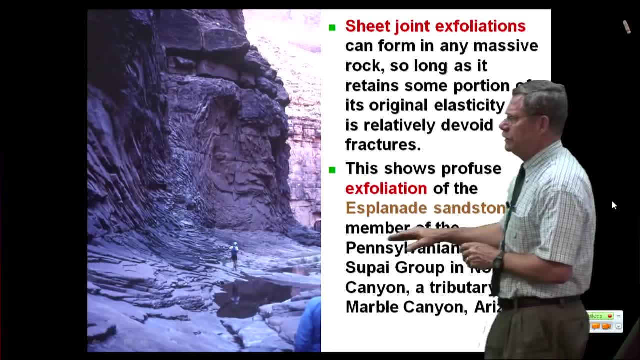 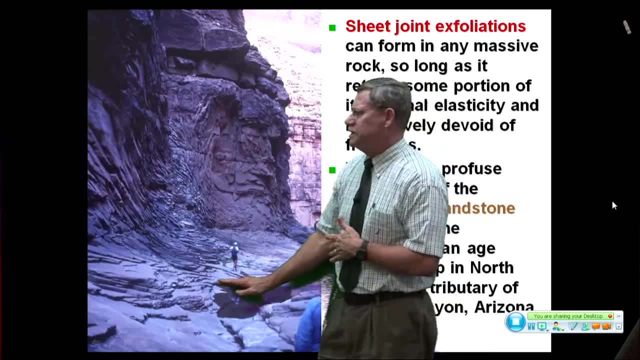 joint exfoliation can form in any massive rock, so long as it retains some portion of its original elasticity and is relatively devoid of fractures- what you see it in here. my wife actually took this picture. this is a in one of these tributaries in Marble Canyon and you can actually see these fractures. 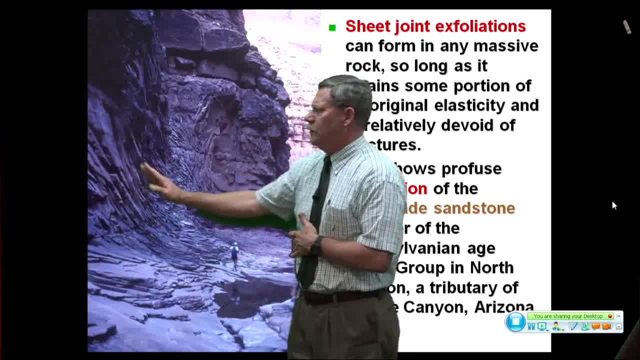 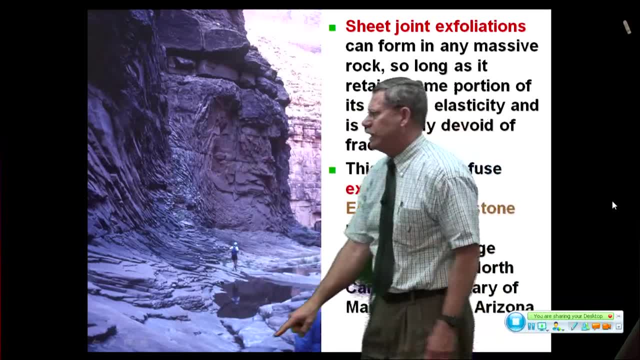 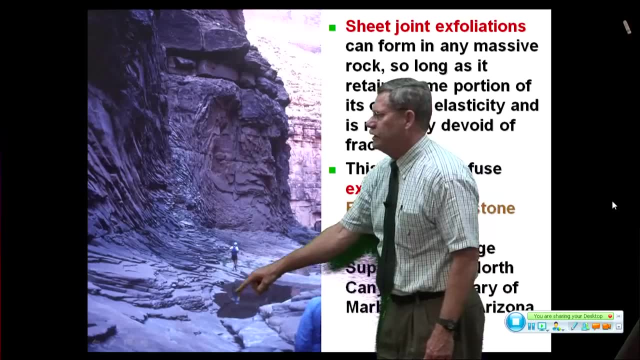 curving up there. they're forming in response to the excavation of this side canyon, and then we're actually looking down the canyon and you can actually the canyon is joint controlled by this master joint set, and this one right here, this is a pool of water, right here it's going down. 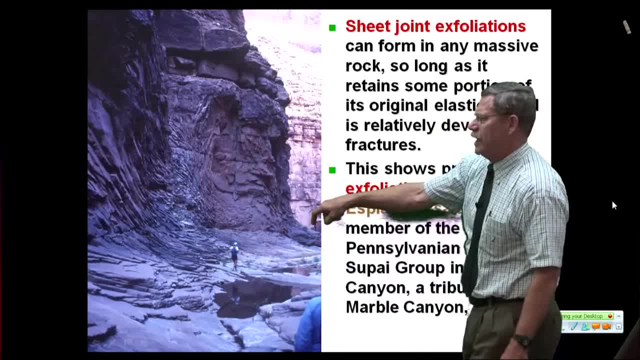 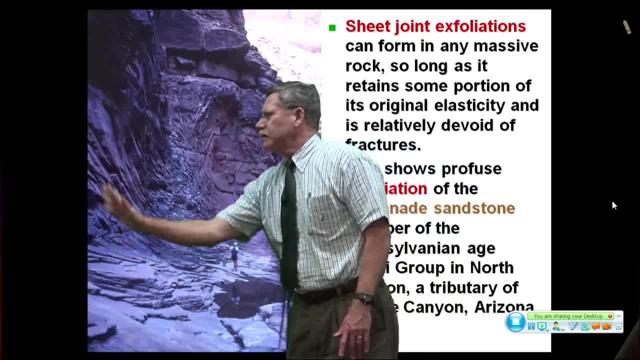 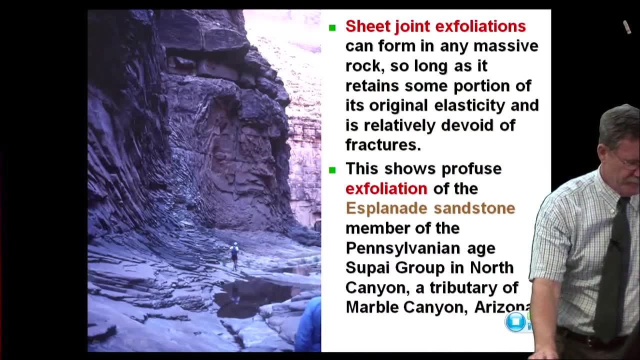 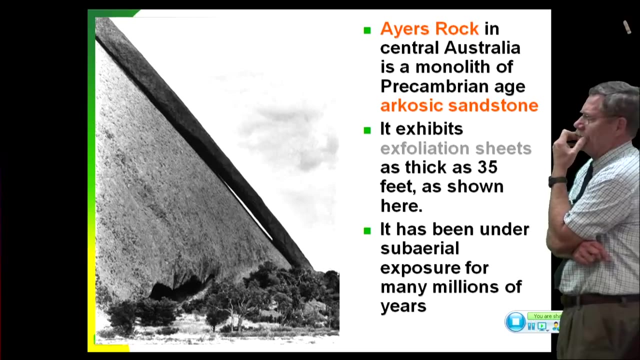 stream and the Colorado River is down there about three or four hundred feet lower in the picture. so you have these, these series of joints that are curving around like a big U. they're u-shaped and that's in the Esplanade. sandstone member. here's the largest one I've ever seen. this is Ayers Rock. 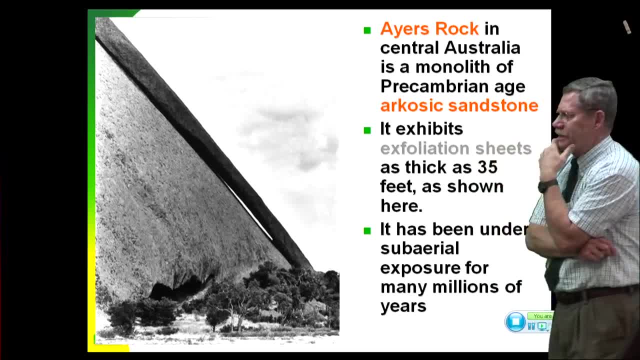 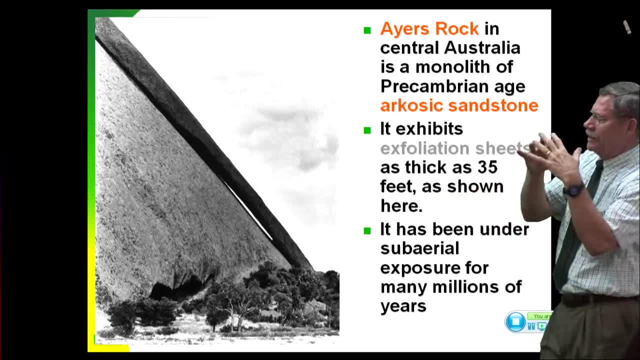 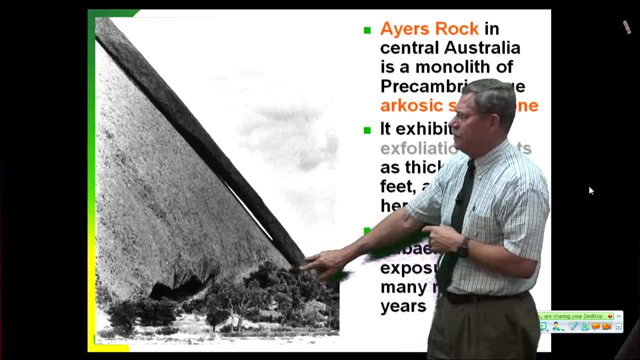 it's in central Australia. it's a archosic sandstone of Precambrian age. it's about nine miles long, about a half mile wide, I think. it's about 600 feet high. and what's going on here? this is a. this is an X full exfoliated slab. it's about 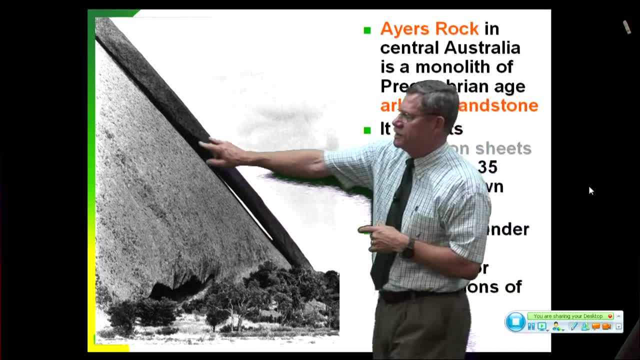 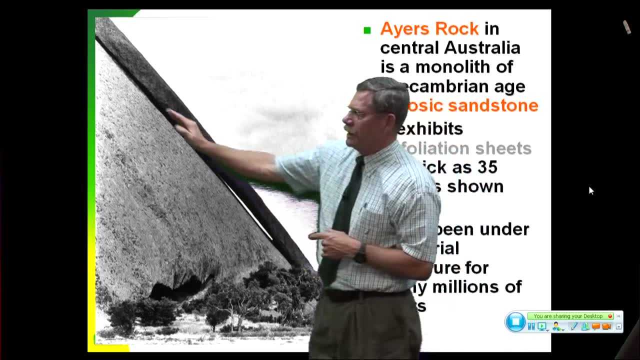 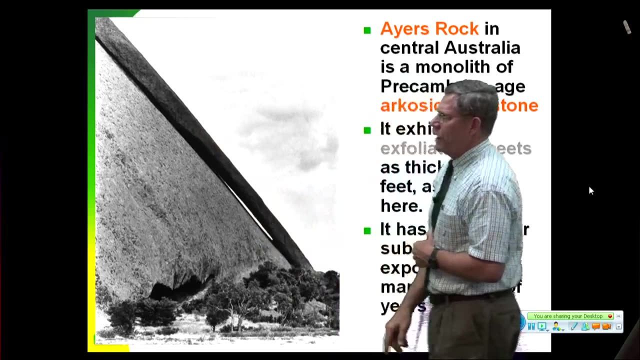 35 feet thick. that's a three and a half story building. this is an enormous feature and you can actually see daylight right through this thing, because this is buckling, this is Euler buckling. this is actually bowed outward and you get this gap in here and these little alcoves down. 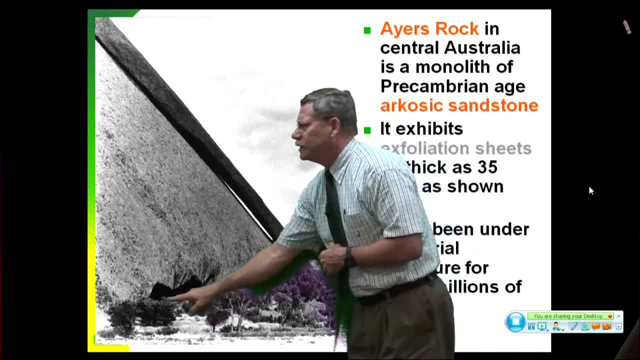 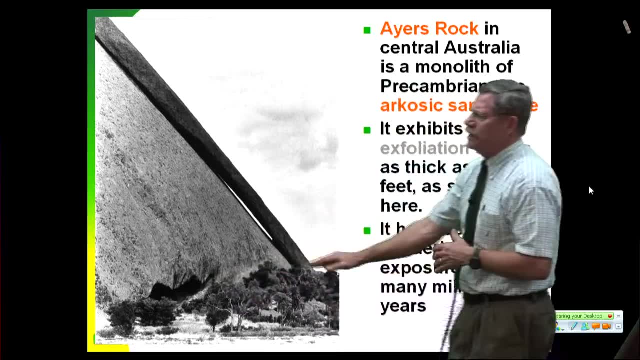 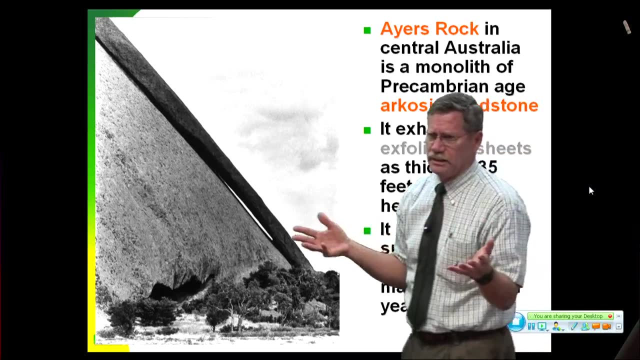 here are where they've had chemical weathering of the Arkos, because the old erosion surface used to be right up in here. these used to be buried and when you're slightly buried you have condensation of moisture just under the ground surface. this is the same way we got the damage on the Sphinx over in. 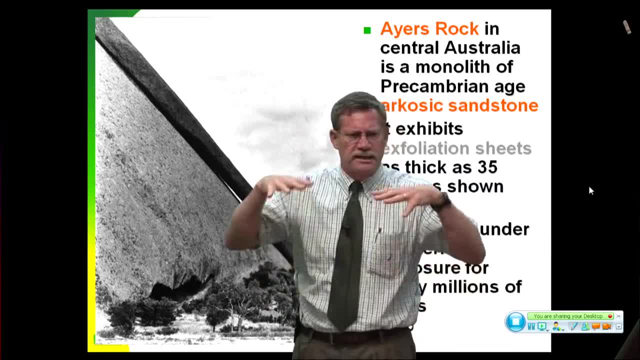 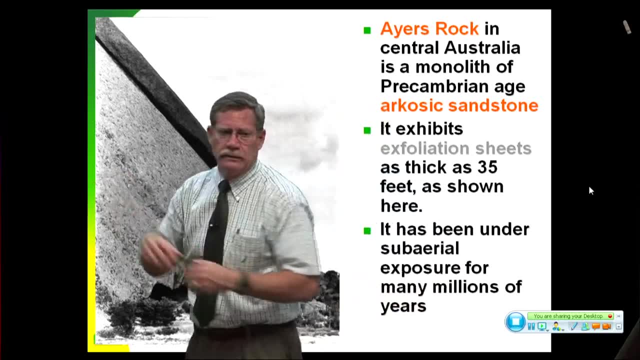 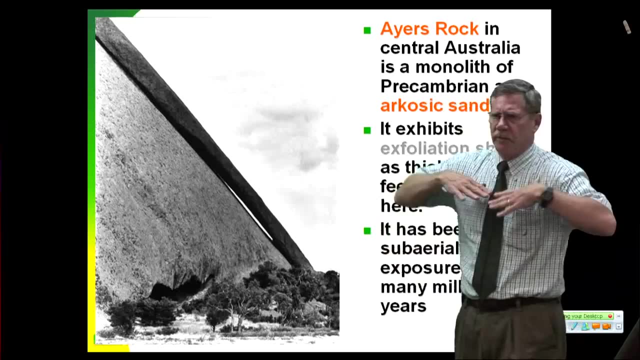 Egypt. the Sphinx was buried, two-thirds buried. you get condensation of moisture in the sand. that moisture then attacks the carbonate in the sandstone- Nubian sandstone- and you get pits- the pits out. so when they excavated the Sphinx, out all the part that had been buried prior. 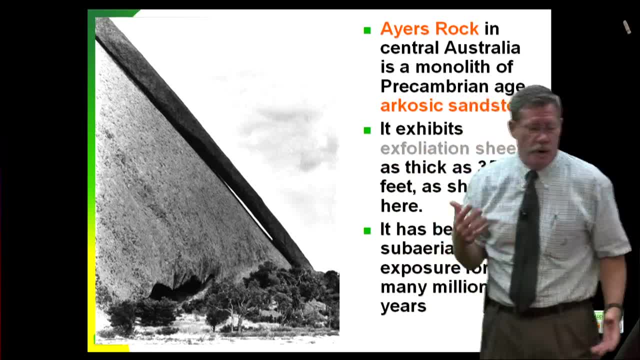 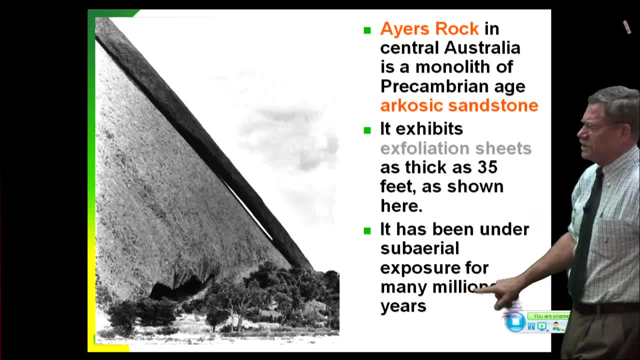 to the excavation is all pitted out and weathered- chemically weathered. so this one's been under sub-aerial exposure exposure for millions of years. Western Australia has a a ground weathering surface that dates back to the Cretaceous, so past the KT boundary. 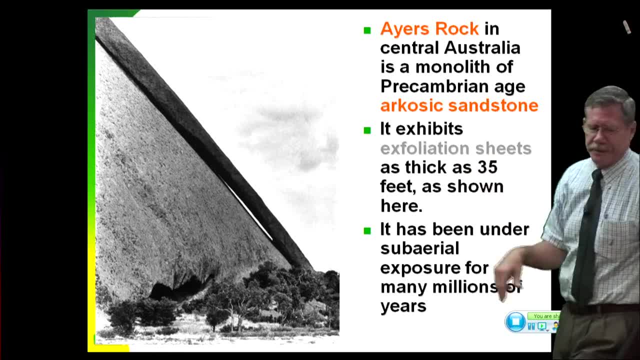 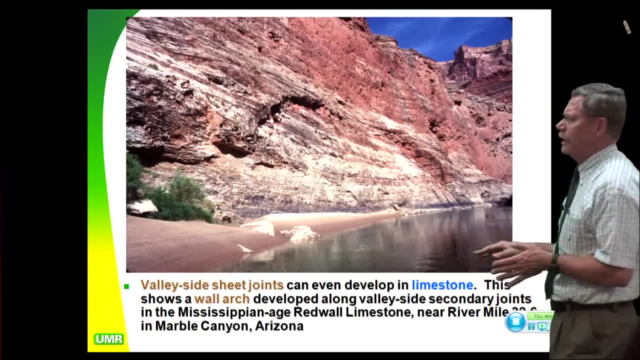 that's the oldest weathering surface on the planet is Australia, so that's why we had some of the biggest slabs there. now here's one where I'm actually floating down the Colorado River, my first trip in 78 rolling along. that was one of my life. 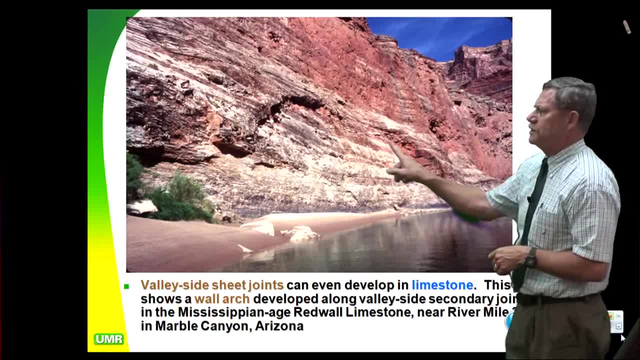 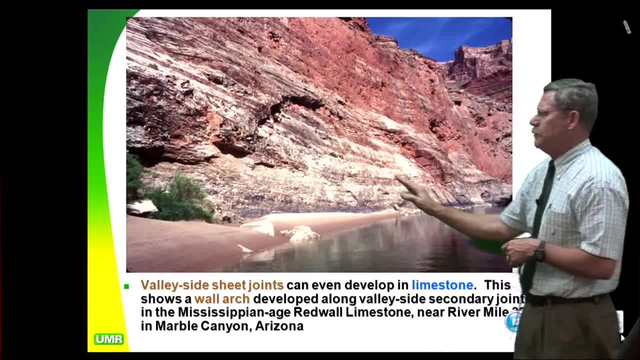 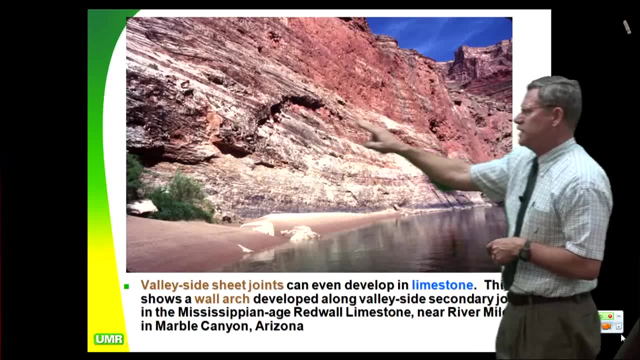 goals and I'm looking up here and I actually seeing a big wall arch coming around and curving around. this is a valley side, joint again and sub-parallel: coming up right like this, going right like that and on up and we have this wall slab that's pulled out in tension, so you get this circle effect. 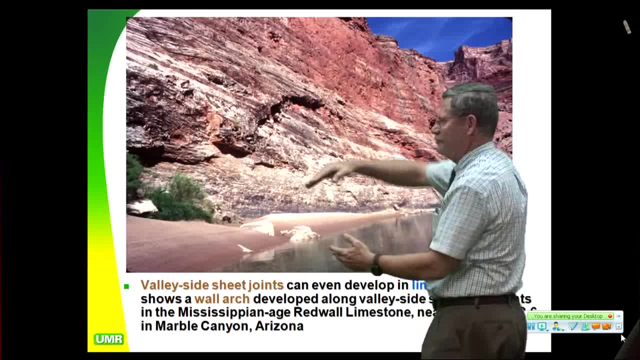 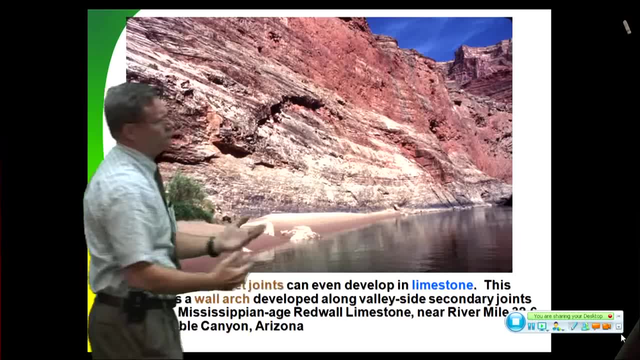 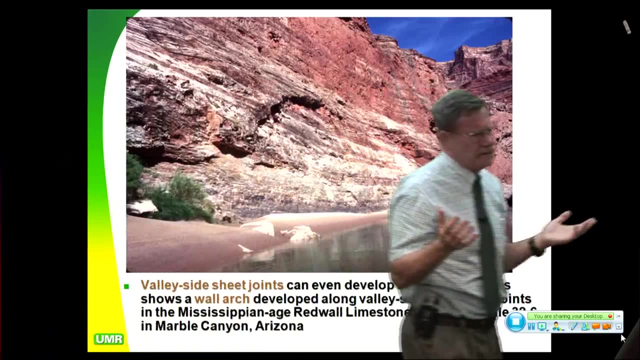 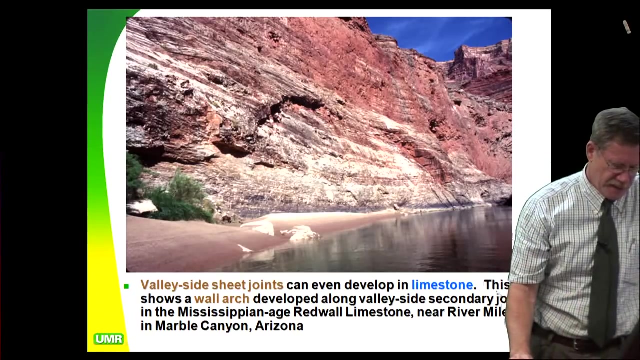 like get in here and show you I can't, but it's good to see I do it like this. yeah, it's pulled out in tension and that's why you get the circle on it the way that you do. and that was in Lime Street, stone, and this is at right near Vasey's Paradise, right down. I can't see, I pull. 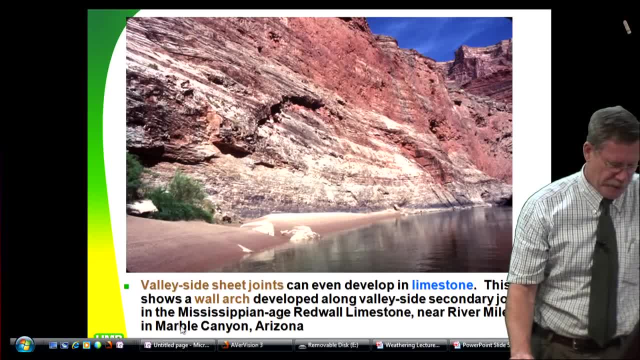 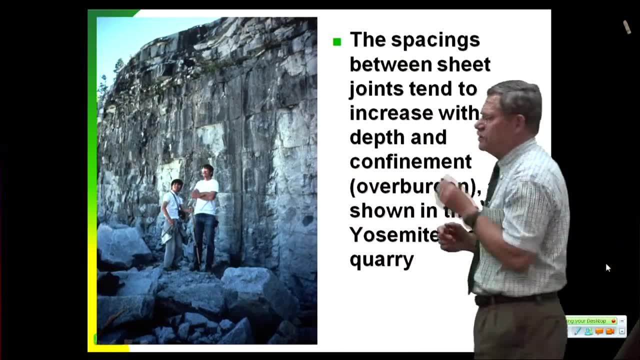 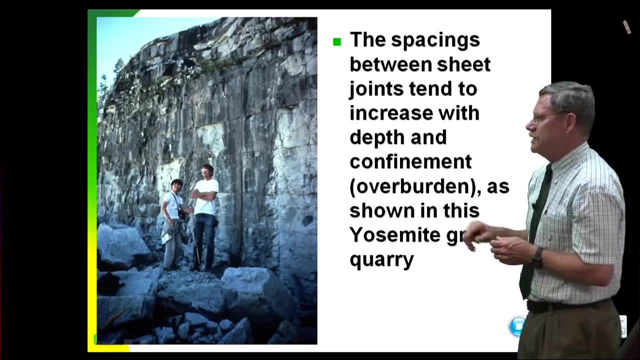 this out of there. yeah, there we go. mile thirty two point six river mile thirty two point six. okay, now here is in a quarry. this is actually at Yosemite National Parks, in the National Park quarry that was built by the Civilian Conservation Corps back in the 30s, and this actually shows how you have. 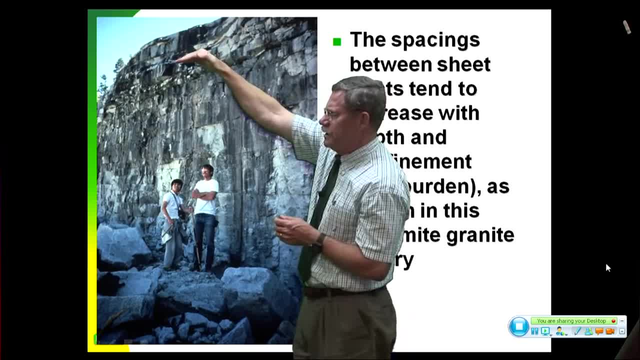 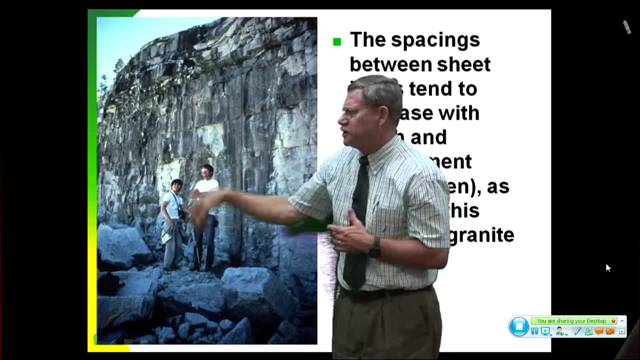 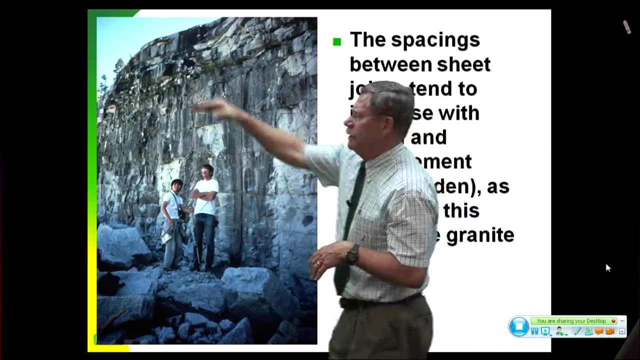 exfoliation joints very close together right near the ground surface, and as you get deeper into the quarry the spacings get further and further apart. now the Romans actually made note of that and use that when they were quarrying. you get your bigger blocks from down here. you get your smaller blocks up in here. 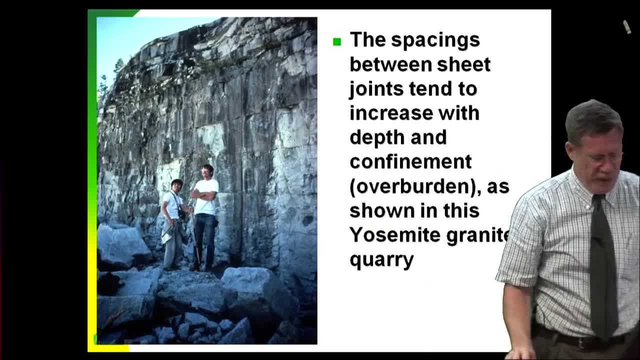 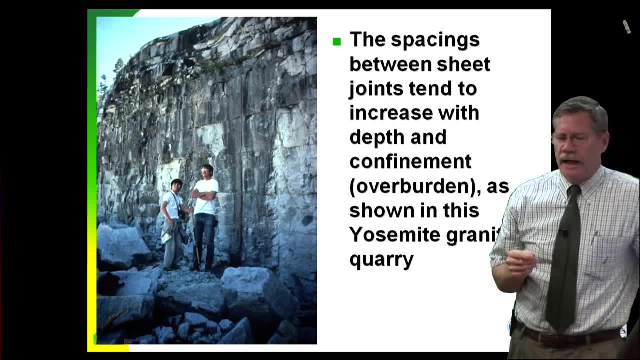 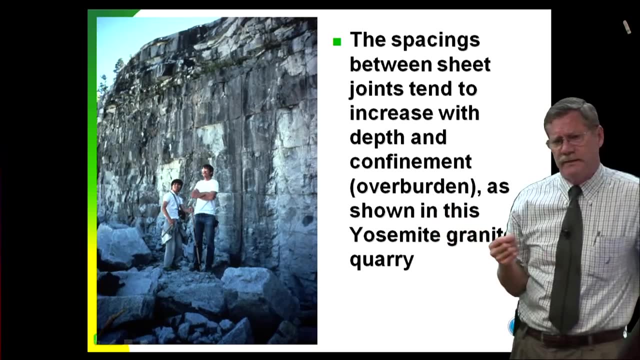 and you make dimension stone out of it. nothing new about that. what the Romans would do, they would use fire and they would use wedges. and remember that guy that came across Hannibal and attacked him from Carthage? well, he came across the Mediterranean, landed to the west of Italy and then 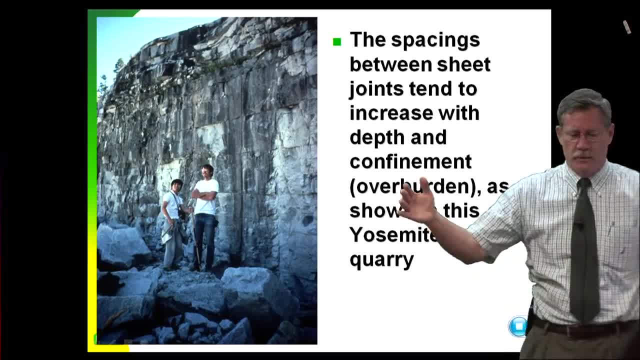 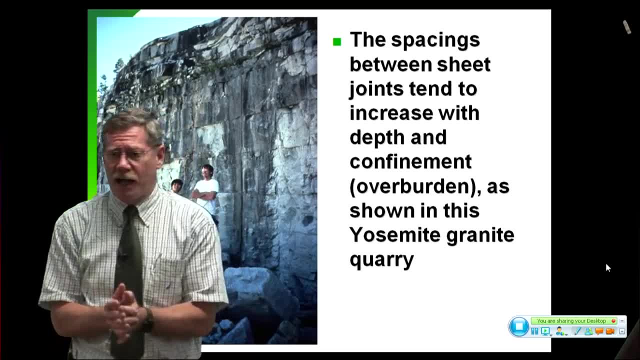 came out through the Alps and in order to widen the road going through the Alps for the elephants, they set these little fires. because if you, if you heat rock and then you throw water on it to quench it, you crack it, you exfoliate it through. 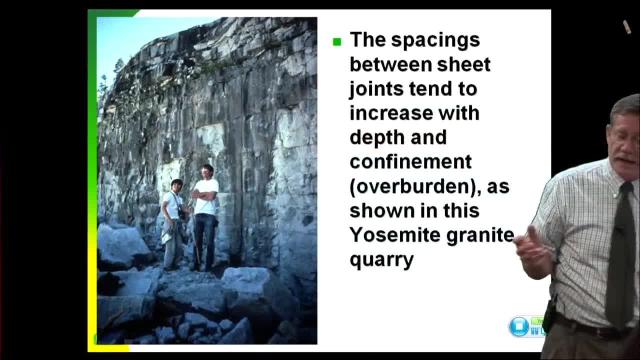 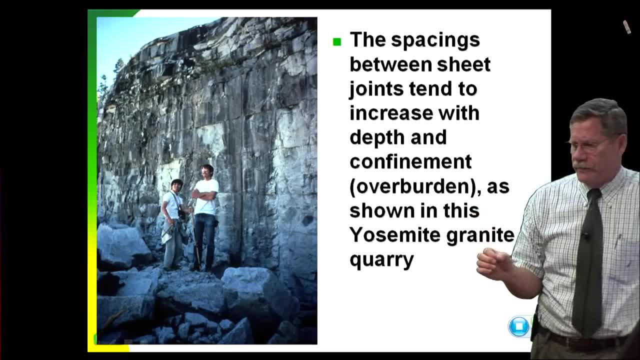 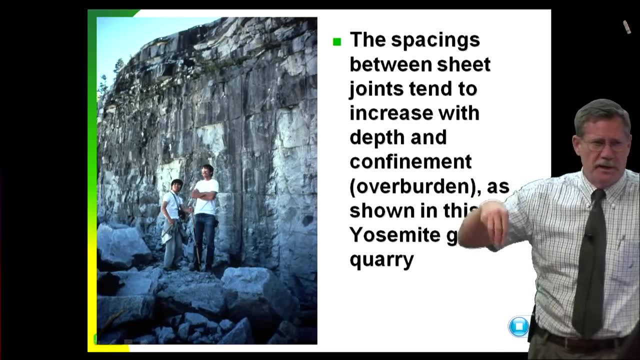 thermal strain, and so thermal strain been around a long time. the Romans used thermal strain with fire and quenching. they might have learned from from the Carthaginians- and they also used wood pegs. so you drill a hole, you put a peg of oak in it and then you 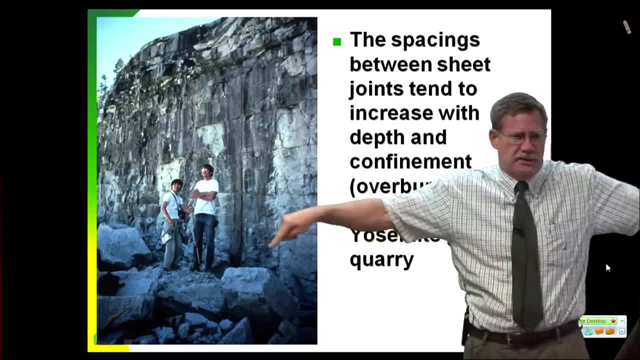 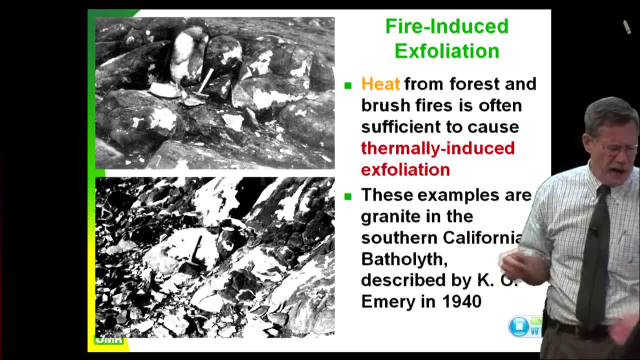 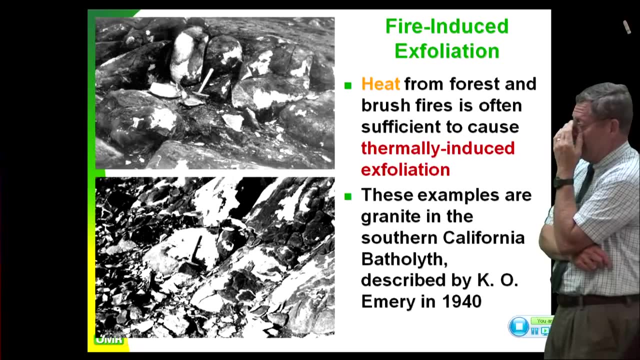 drip water on it, the wood expands and you force a tensile fracture between the holes. the holes are about five inches apart and about five-eighths of an inch in diameter. here's fire induced exfoliation. I saw this when I was fighting on fire crew as a teenager in California with 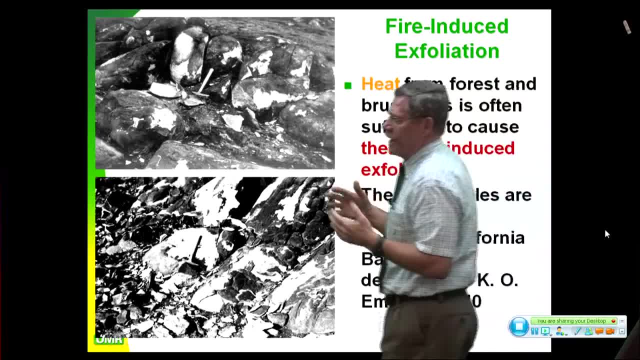 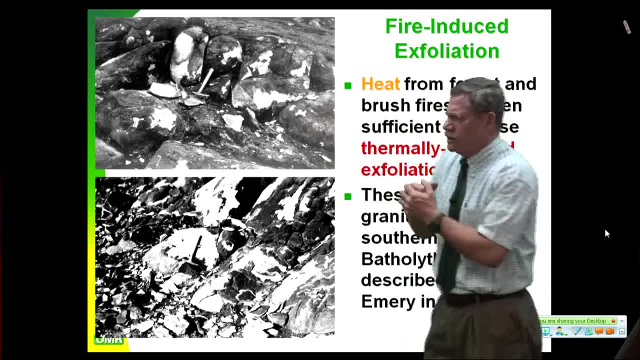 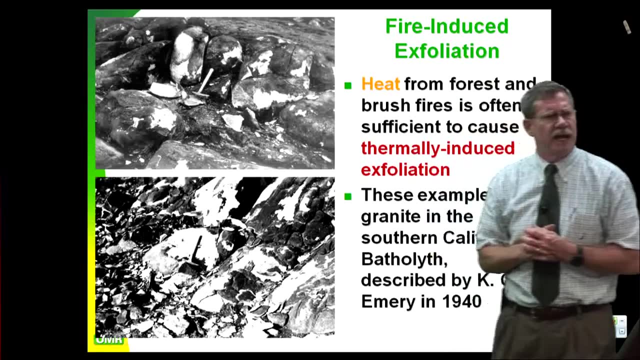 California Department of Forestry. and then I went off and asked my professors at Cal Poly. you know, I said all my textbooks say that temperature doesn't cause exfoliation, it doesn't cause rock. and they said that's right, doesn't? because? David Griggs, who's a member of the National Academy of Science and who 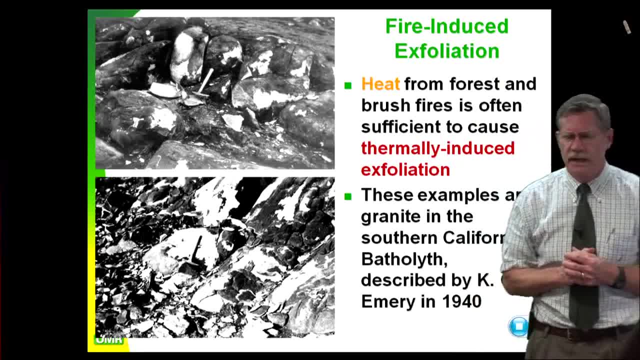 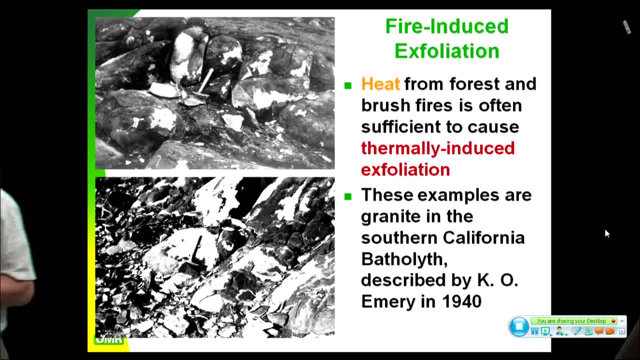 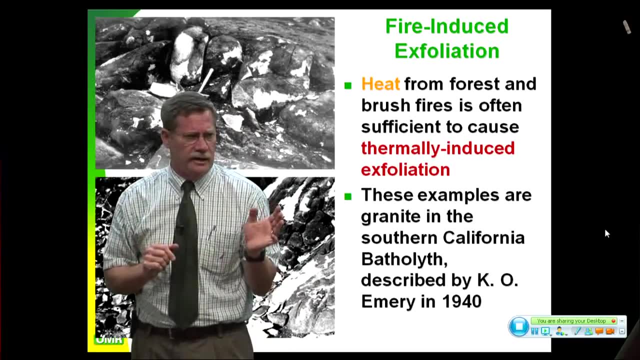 got the Penrose medal from Geological Society of America in 1975. he did tests at UCLA and he was from MIT, and the only those brightest stars come from places like MIT. well, Griggs was a consummate scientist, not an engineer. okay, so I'm gonna go left brain on you now. it's all you scientists, hang on your panties. 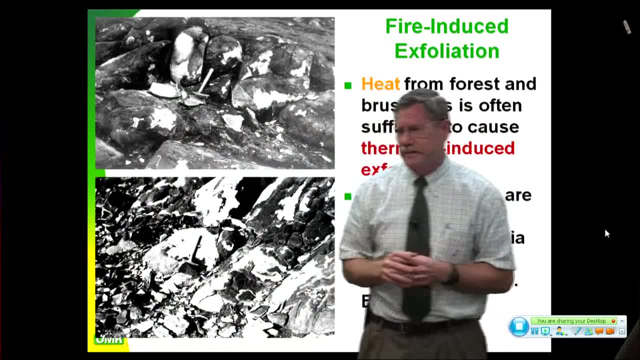 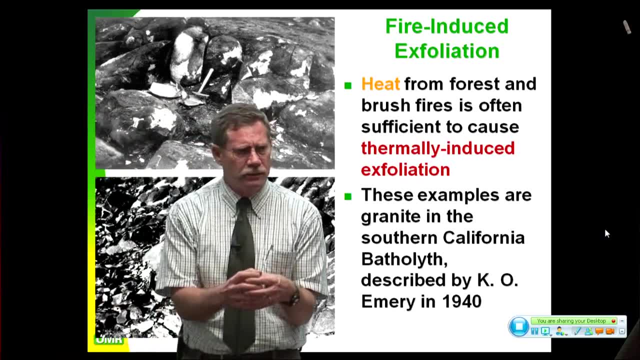 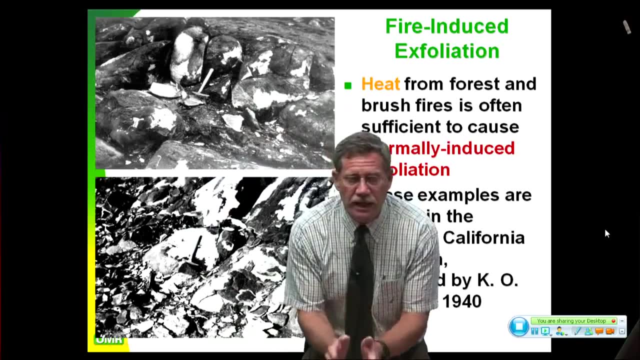 don't get upset at me, but scientists- typical science- didn't have solid mechanics background. okay, it's not an engineer, so he takes little discs. he takes cubes of basalt, granite and limestone. he makes beautiful little cubes out of them. he takes it out here and he heats it up like a scientist heats it up. 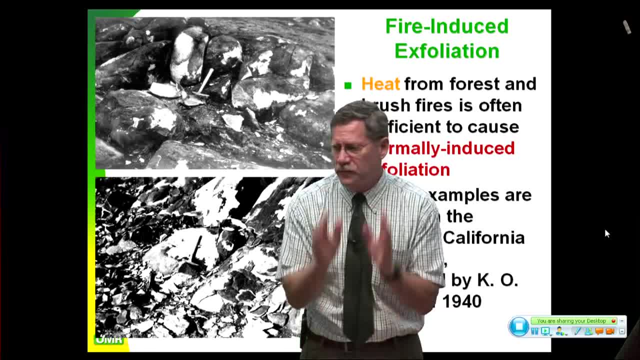 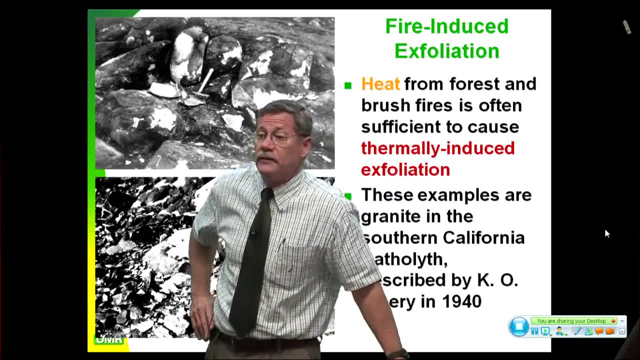 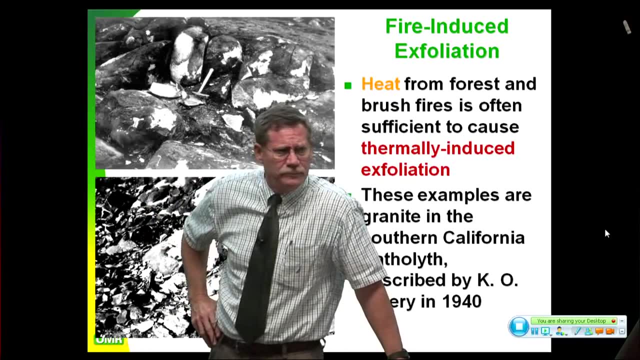 real, real hot. 600 degrees cools it down, does it 400 times, nothing happens. so temperature has no effect on rock, and that's in every geology textbook, even the ones used on this campus by our geology department, even my department. what's wrong with that? what your engineering hat on? what's wrong with? 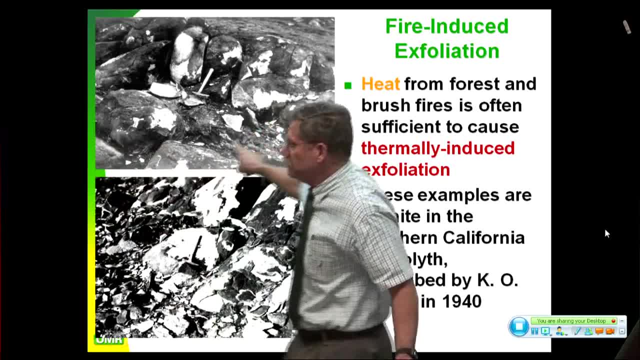 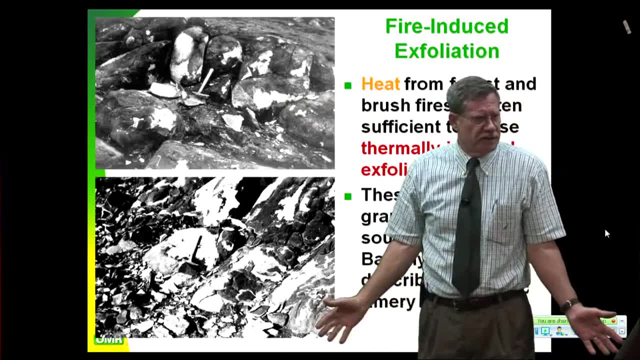 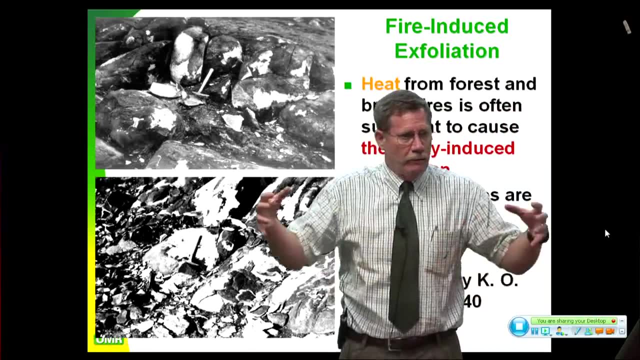 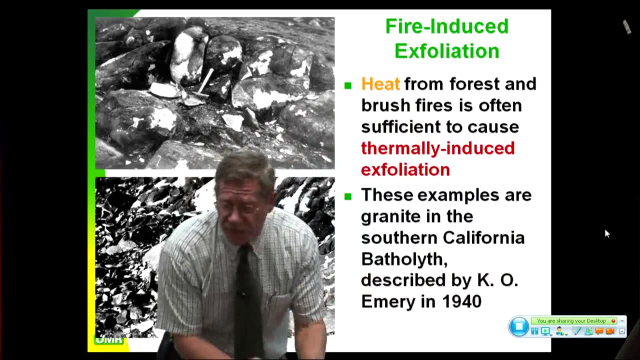 that. does that replicate what goes on in the real world right here? I mean no, what's going on here? what's going on? there's insulation isn't there that that block is never going to develop tensile strain if it's free to expand and contract, expand and contract. but what if you had a long block? let's. 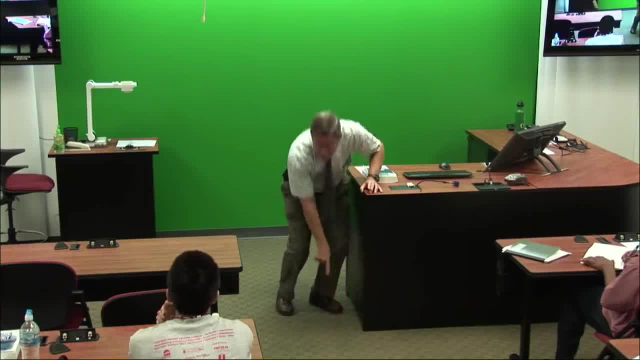 say, you had a block two inches in diameter went all the way down like this for 25 feet, and I stood up here with a blowtorch and went heat it up, heat it up, heat it up. what's going on down here? any thermal strain, you bet your. 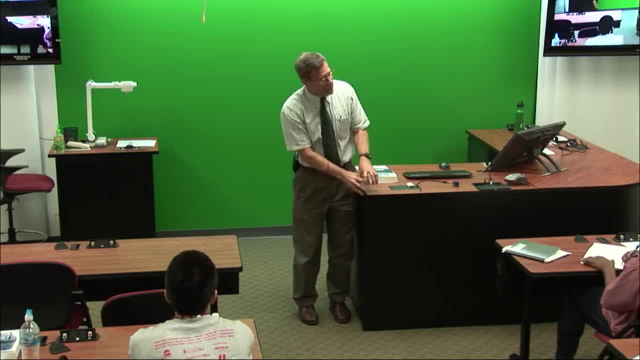 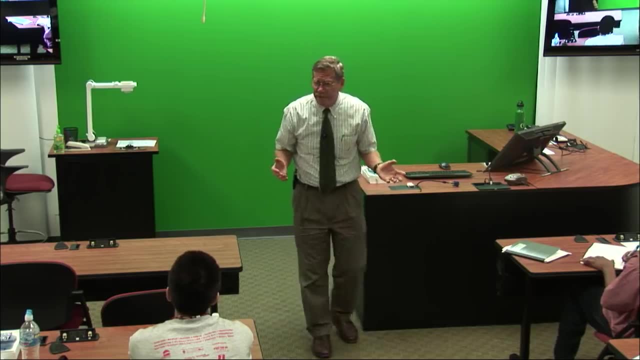 ass. that's his basic solid mechanics. this is going to heat and what's it going to do? it's going to expand. that's how the guy made Stone Mountain Georgia. David Griggs probably wasn't out there, he was at Westwood. one guy made Stone Mountain Georgia. you don't like the Confederacy? 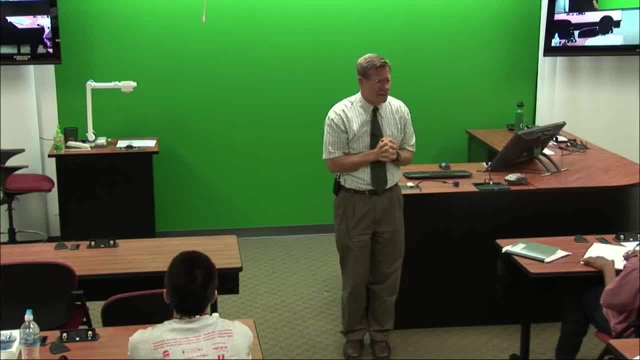 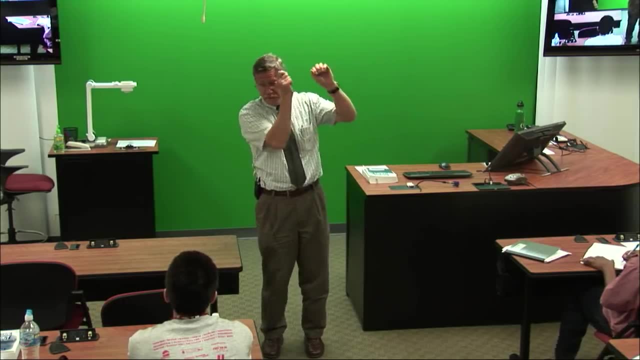 but one guy out there with a blowtorch carved that whole thing. the Vietnam veteran went up there and just turned a blowtorch on and you know this is after. they took him 30 years to build Mount Rushmore, you know, with chisels and dynamite and all the slow. this guy just took a blowtorch, just started carving. 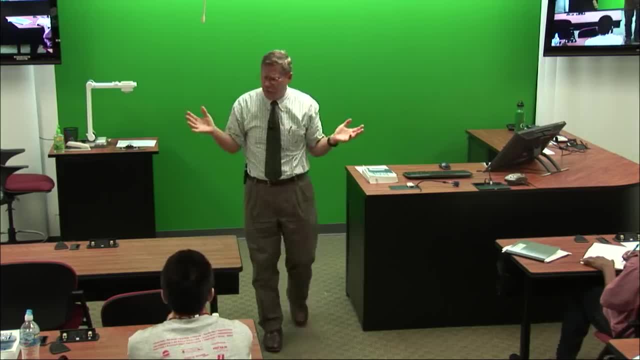 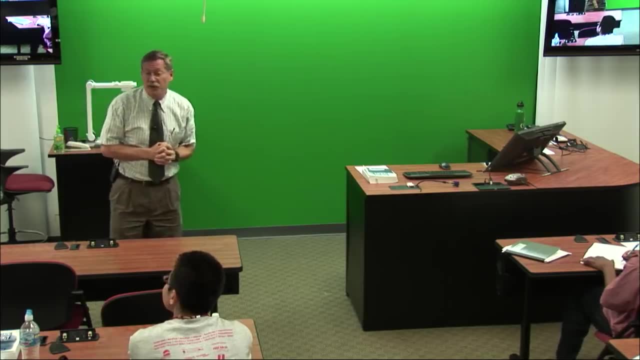 you heat up the granite, real strong granite. you heat it up, it flakes off, it exfoliates. but all the textbooks say heat has no impact. wow, but they're all been peer refereed and put in journals, so it has to be right. Seal of God all. 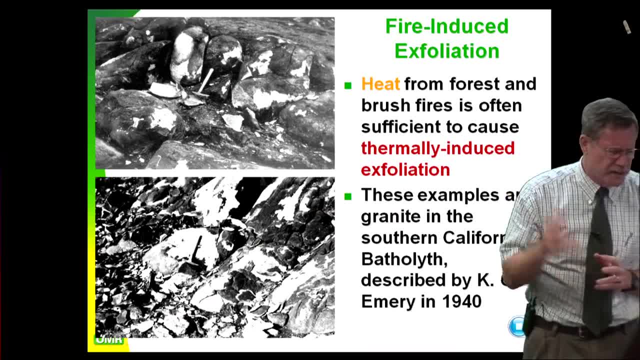 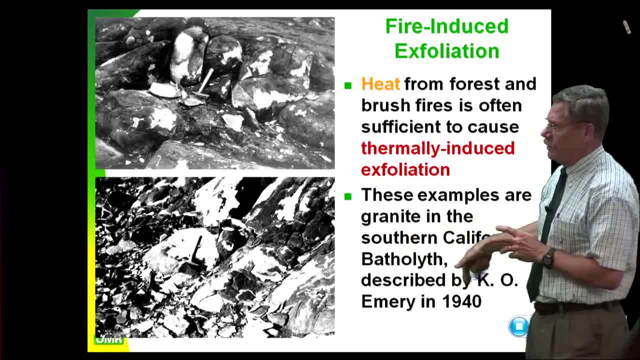 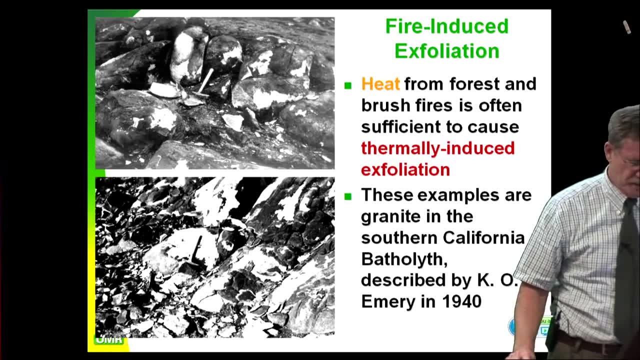 right. so heat from forest fires and brush fires can cause thermally induced exfoliation. there's nothing new about this. it's in the literature, all the way back in 1940, KO Emery's work on forest fires down in San Diego County, that he observed when he was at Woods at La Jolla. this is my own. 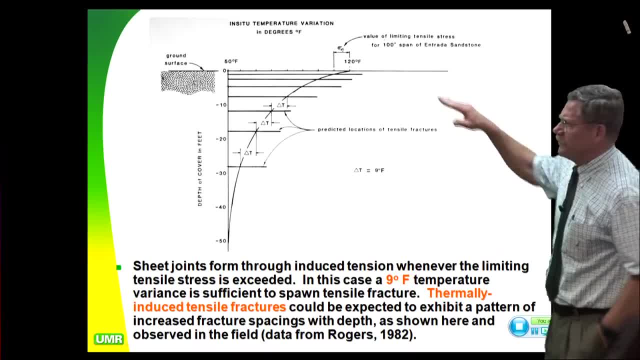 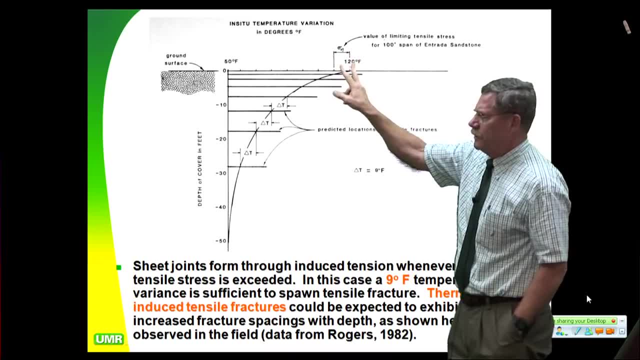 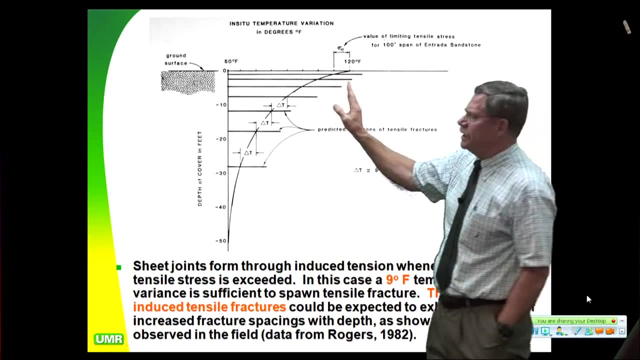 thesis work, some of the some of my thesis work where I actually took a finite element program and looked at the thermal differential to cause tensile fracture and it was nine degrees, I think it was the amount would do it. and what you see is, if you look at it from a solid mechanics perspective, here's the temperature at the ground. 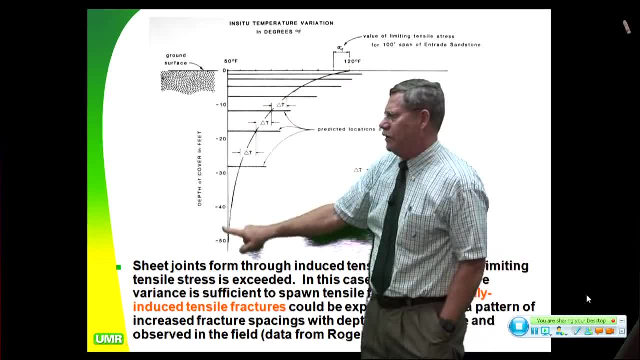 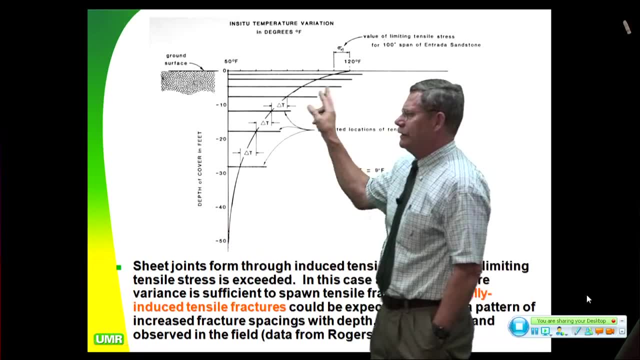 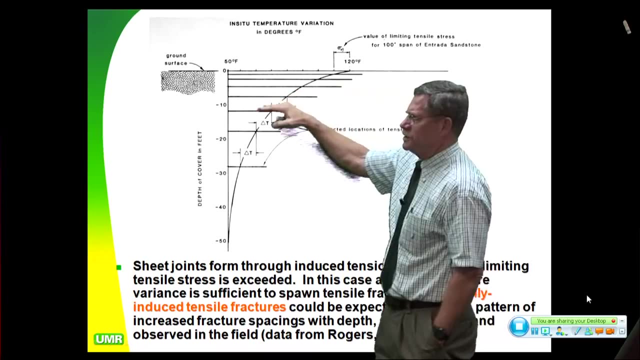 surface on the hottest time in the summer and then going down by the time we get down to 80 feet. we have a constant temperature, something like 55 degrees Fahrenheit, and so if you look at a thermal model, it would predict fractures increasing in spacing, exactly the way we see them in quarries.